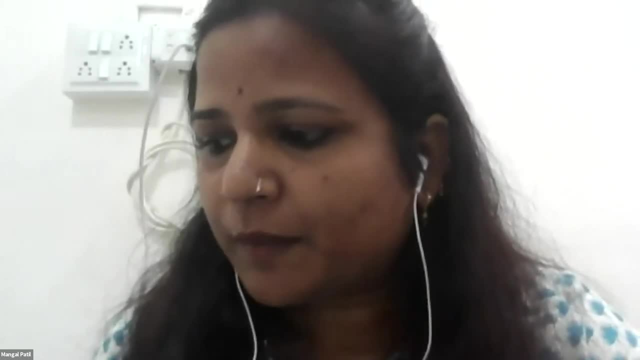 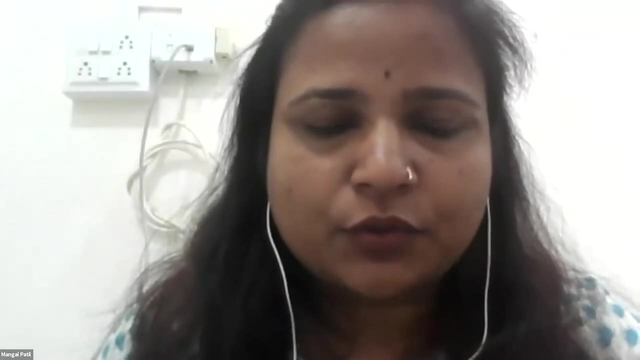 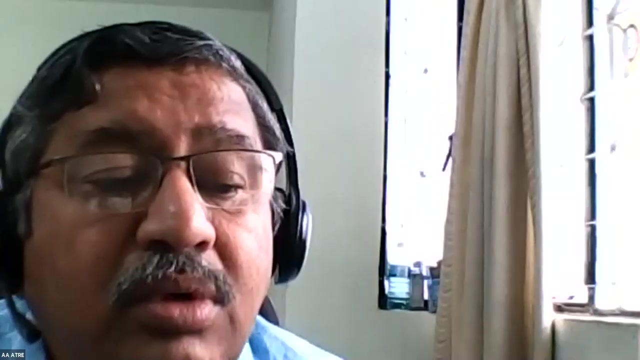 who is the Institute Chair Professor from Department of Civil Engineering, IIT Mumbai. So I would like to request Dr Atre, sir, to welcome the today's keynote speaker and all the participants. Sir, please, Hello, Good morning to all, I welcome. 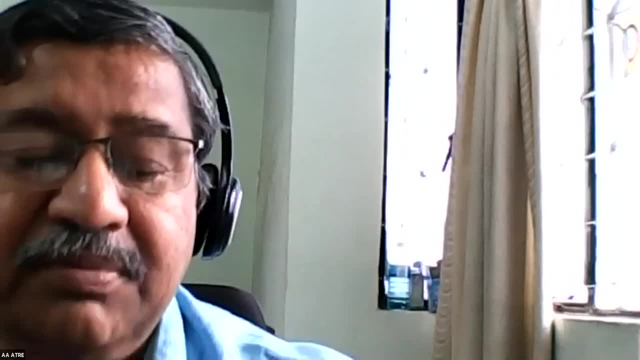 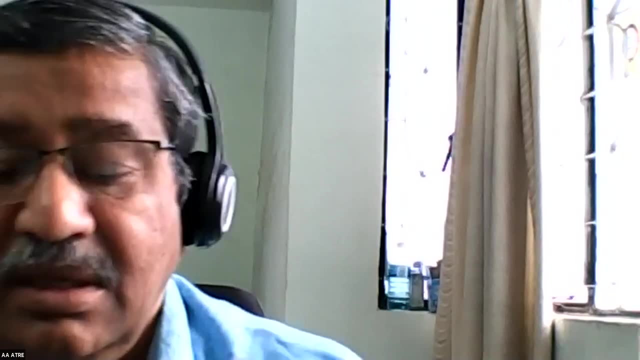 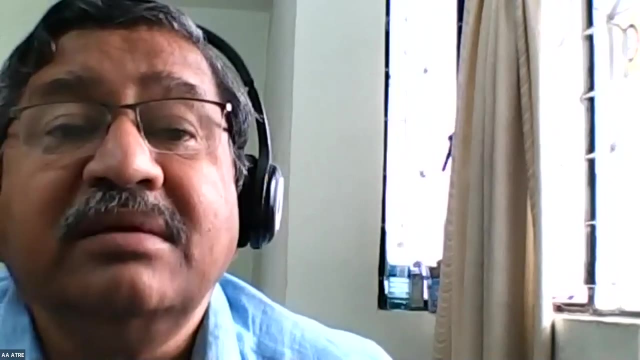 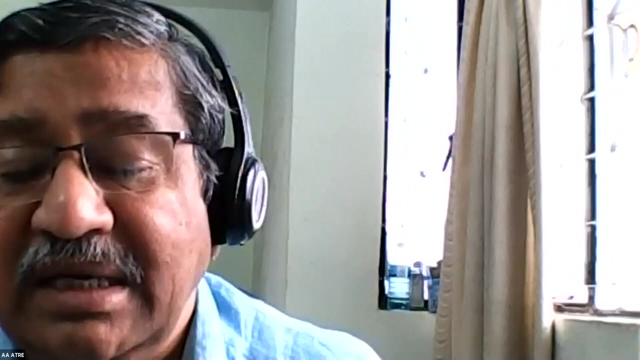 the keynote speaker. today's keynote speaker, Professor Ti, Endo, Institute Chair, Professor from Department of Civil Engineering, IIT Mumbai. This particular training, as already told by Dr Shinde and Dr Patil, This is based on the water resources modeling and I welcome all the participants for this particular training. 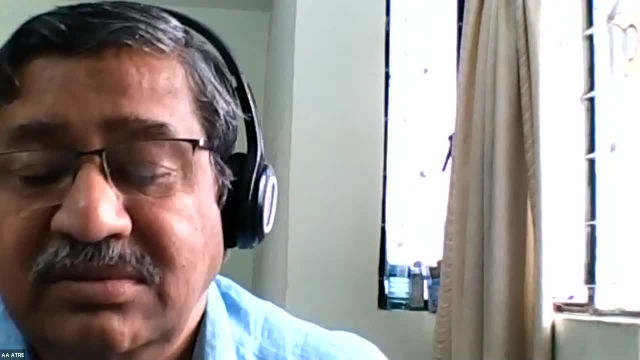 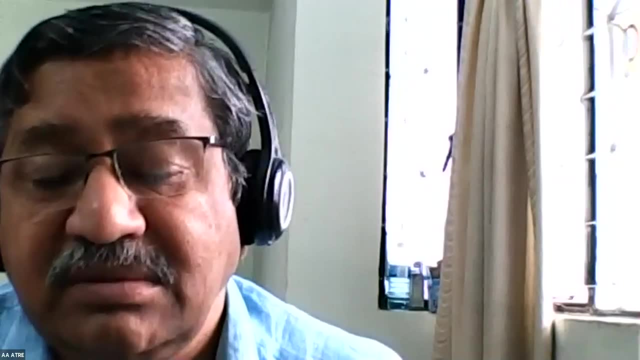 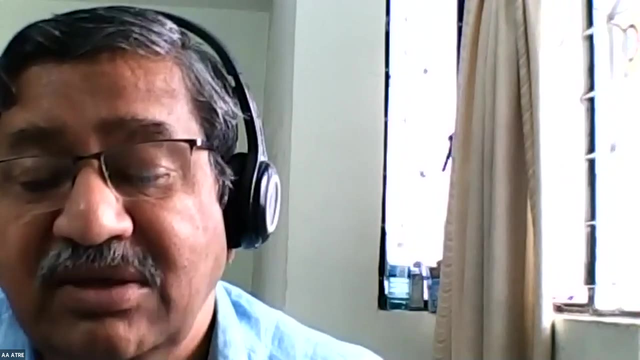 This will be based on the water resources modeling and I welcome all the participants for this particular training. We will possibly give the overview of water resources modeling to other young engineers. This is 64th training in this particular center for Paradigms science and technology. 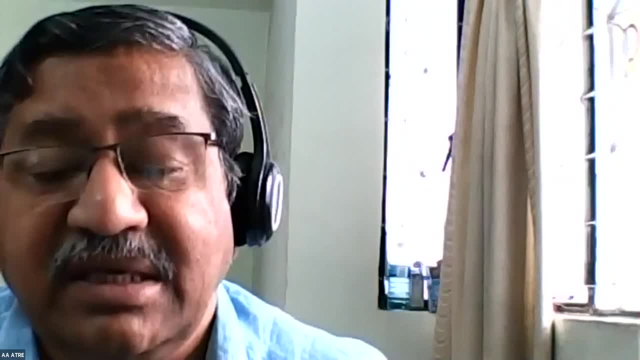 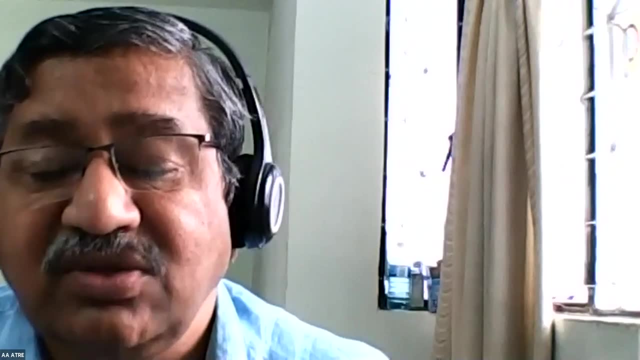 CSaWM, that is, the Climate Smart Agriculture and Water Management. I welcome all the participants for this training on water resources modeling to fit the senses of the water resource, and I organized this training for a few years. and technology- that is the army of science- includes our unto the varies plastic materials such as green specialization, PF, interrogon, velocidad, verm stitches. Está hecho el uno de muchos, obviously de a parte Y fellow se está sosissionando de un producto de Committeea deocused reenkono. 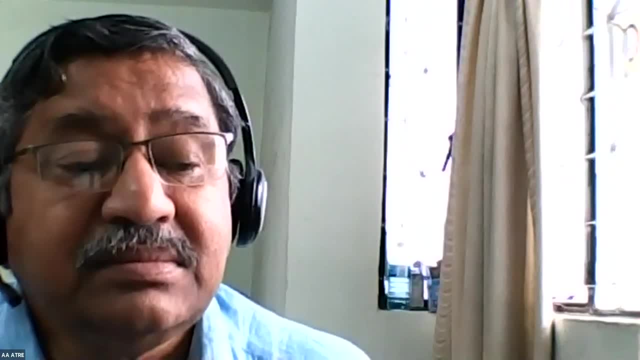 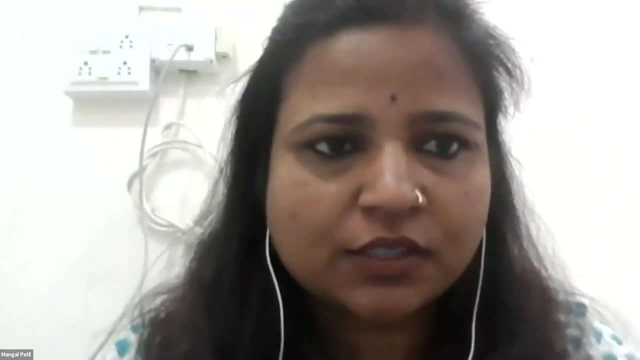 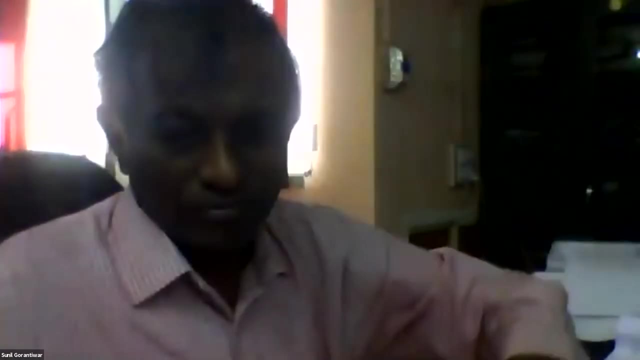 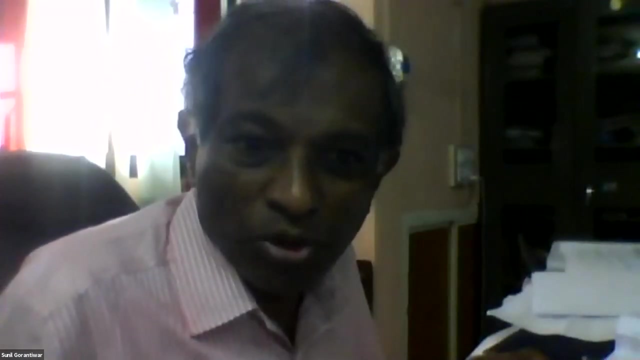 Thank you, sir. Now I would like to request Dr Sunil Gorantewar, who is principal investigator of this project and also the convener of this training program, to give the preamble, Sir, please. Thank you very much, Dr Mangal Patil, The keynote speaker of today's 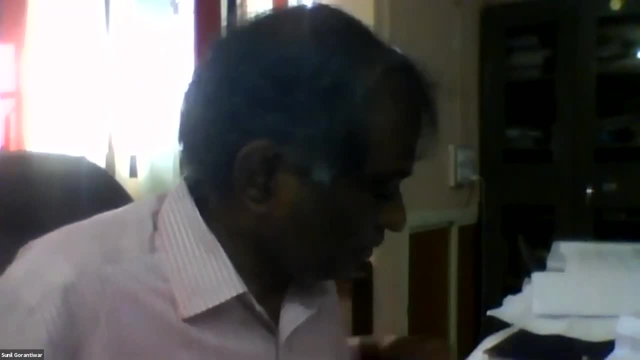 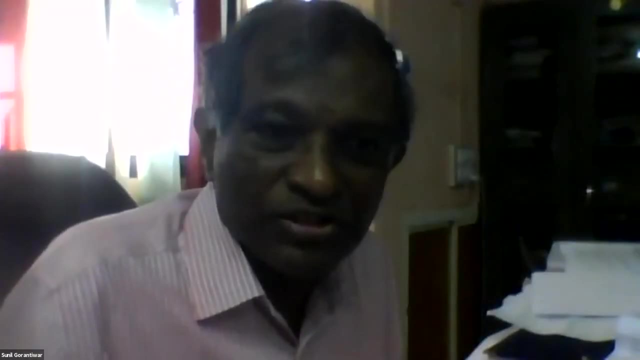 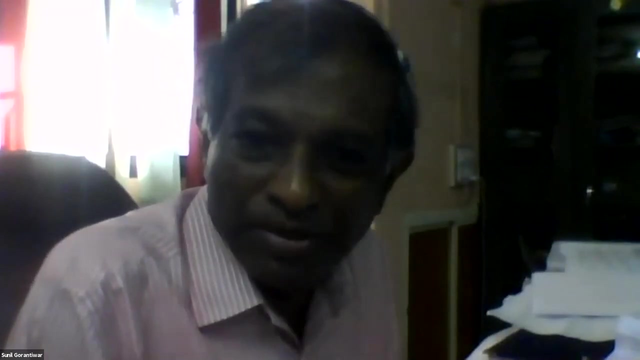 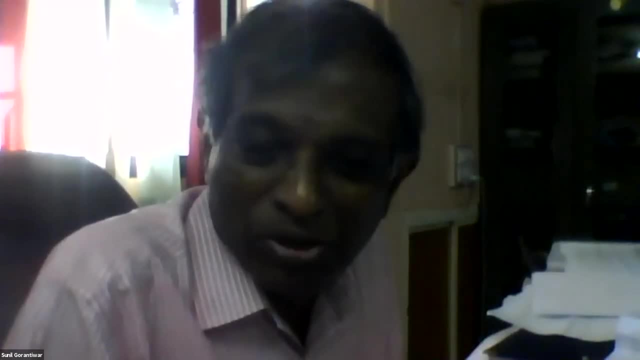 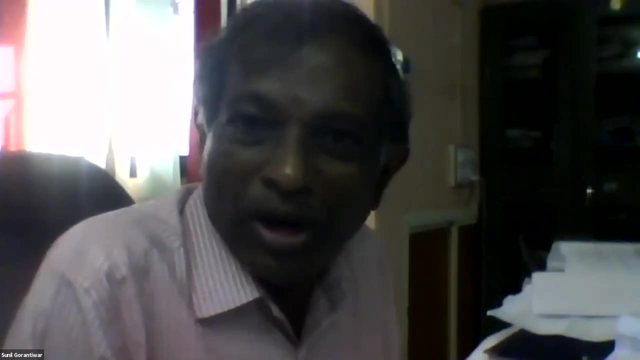 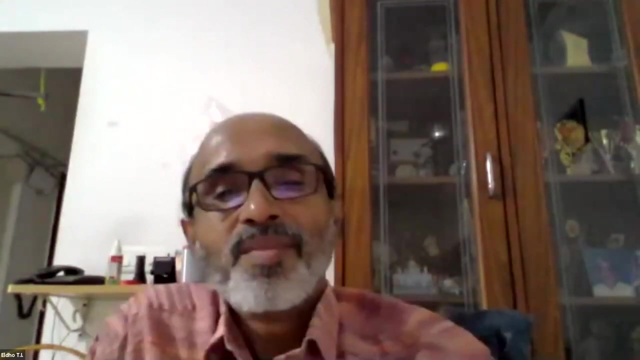 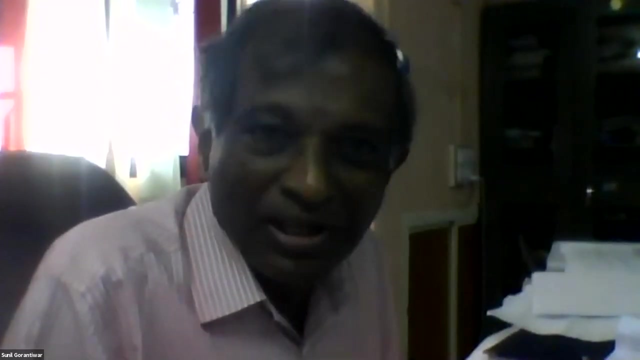 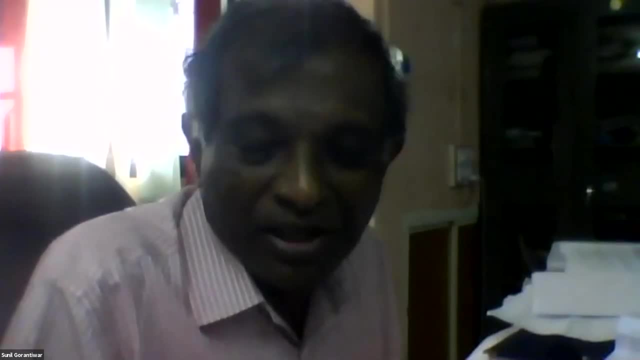 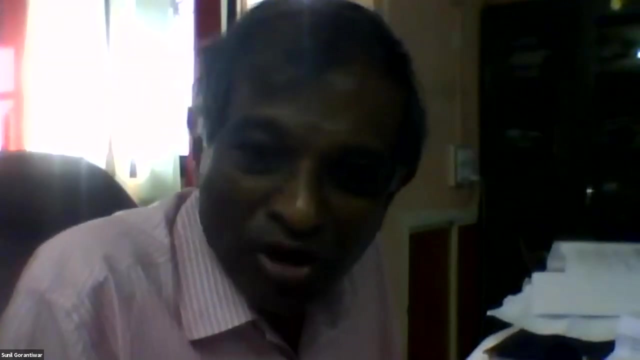 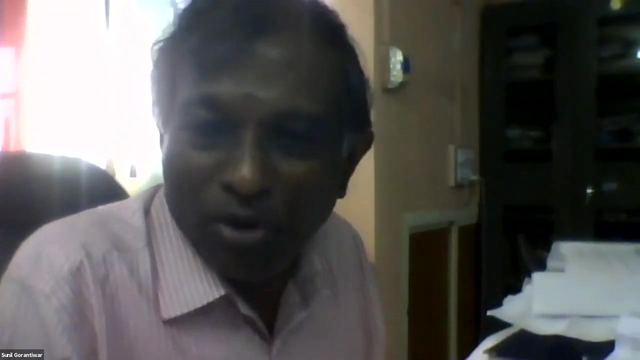 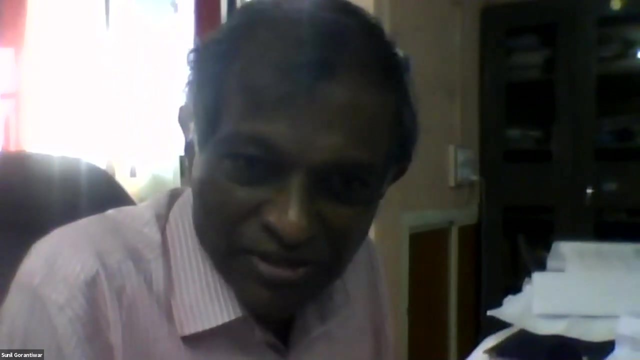 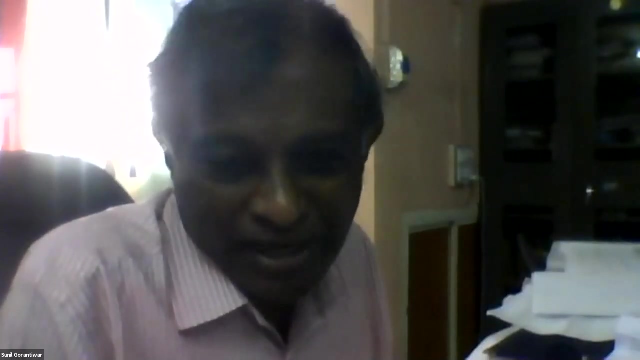 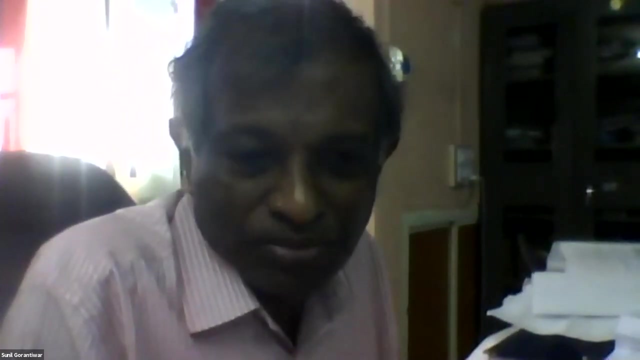 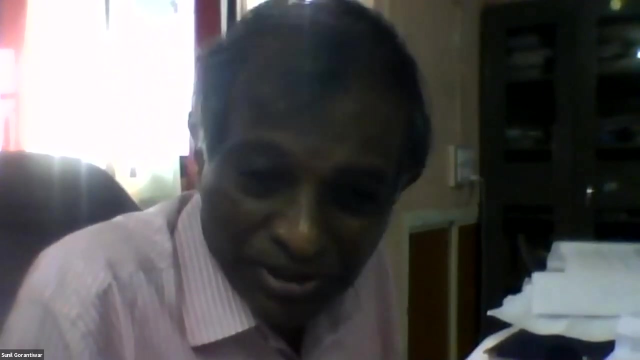 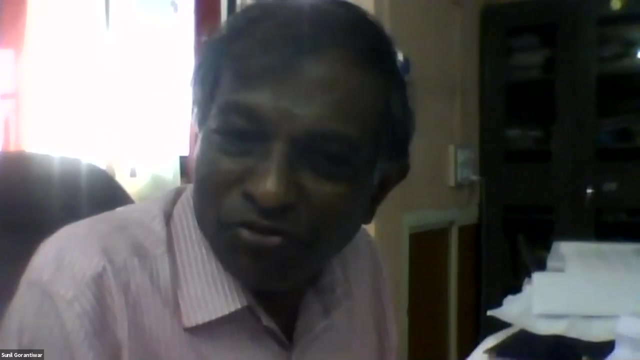 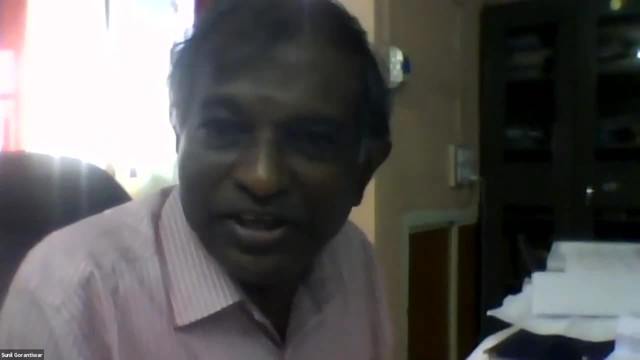 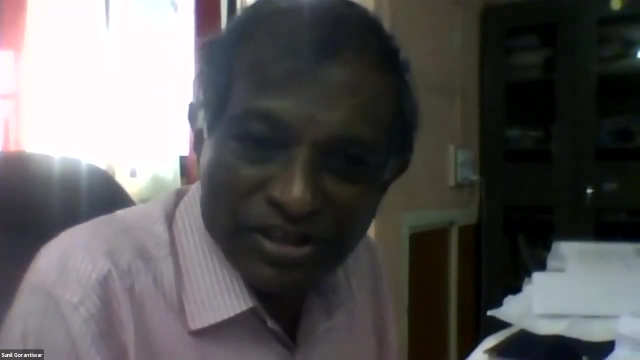 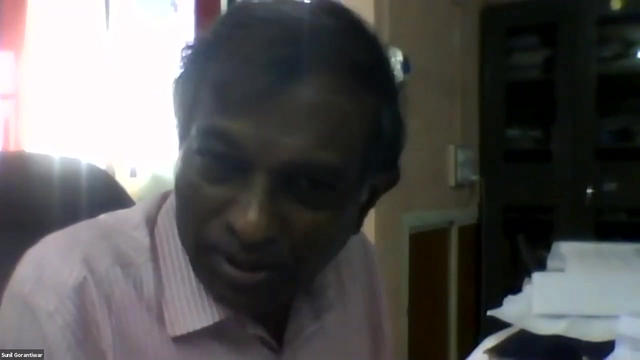 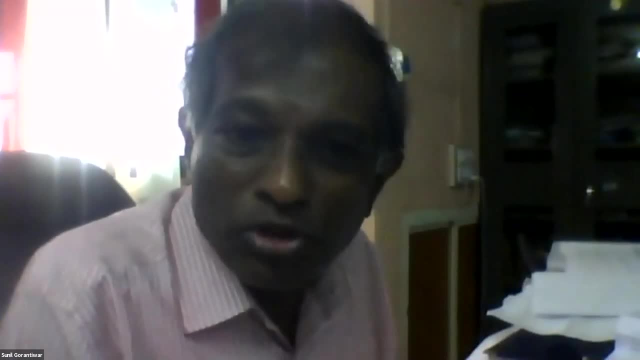 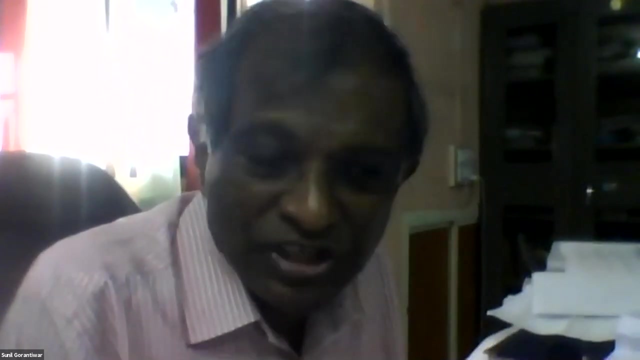 the module-based post-graduate diploma in climate smart agriculture and water management, in association with our national and international partners. Accordingly, we have formulated 12 months module-based climate smart agriculture and water management post-graduate diploma program for basically addressing the thematic areas, such as: 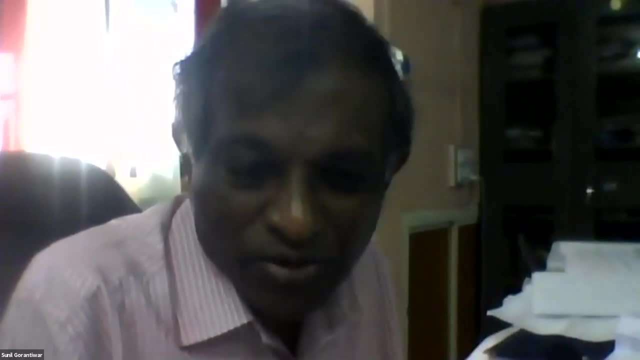 geoinformatics, robotics and drone application in agriculture, then mobile and web-based application, internet of things and decision support system. So our post-graduate diploma program addresses basically these issues, these techniques in context of climate, smart agriculture and water management. 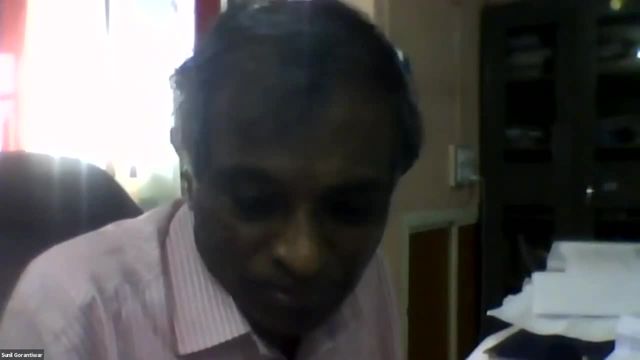 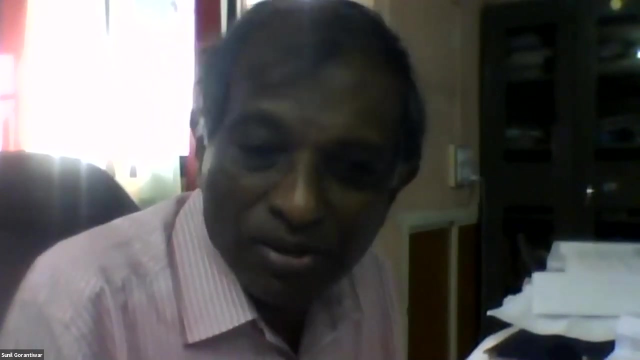 We have also started the post-doctoral research program for the middle level careerist, and already four of the post-doctorate students they are about to join. As far as the post-graduate diploma is concerned, though, we have formulated and framed along with 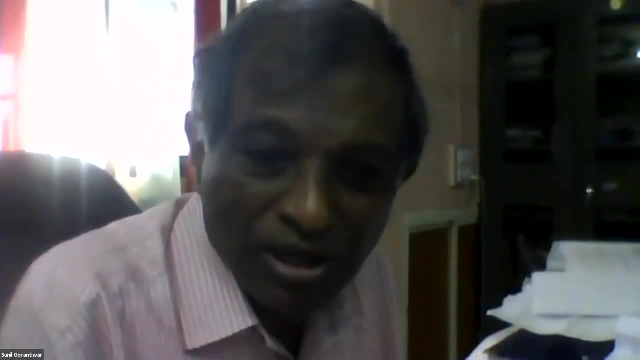 all the modus operandi, but we did not start this program because of the COVID situation, but we are going to soon start And at the same time, we have also strengthened our existing master and doctoral level programs in context of climate, smart agriculture and water management. 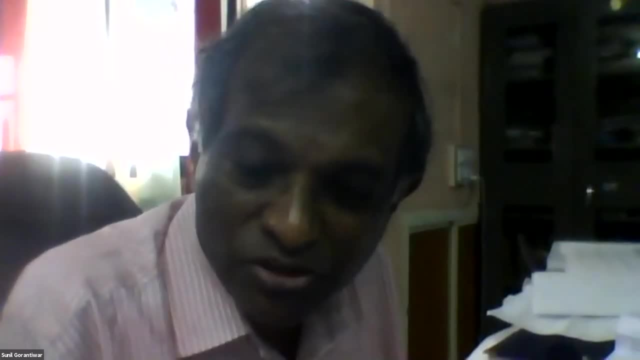 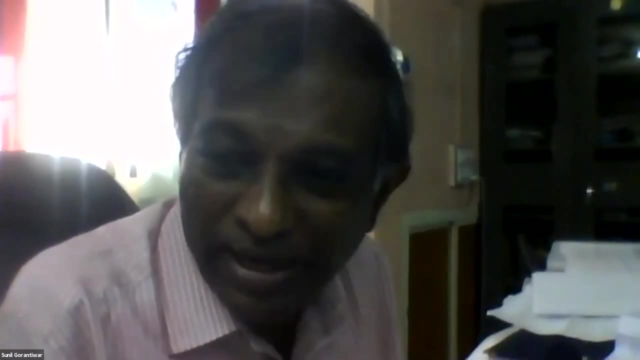 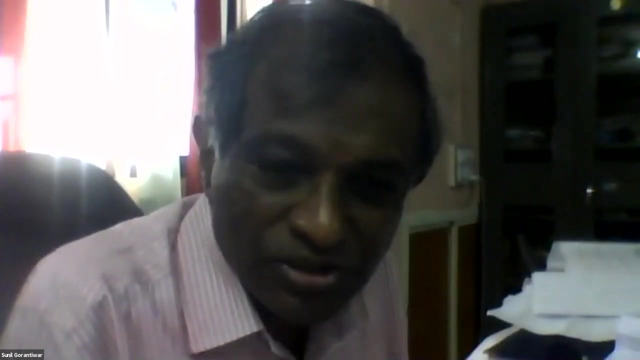 and including all kind of the thematic areas, that is, geoinformatics, robotics, drones, IoT's decision support system, modeling and mobile and web-based application. Our third object is related to research, that is, to develop the tools and technologies, using all those techniques that I have mentioned, for the benefit of the agriculture. 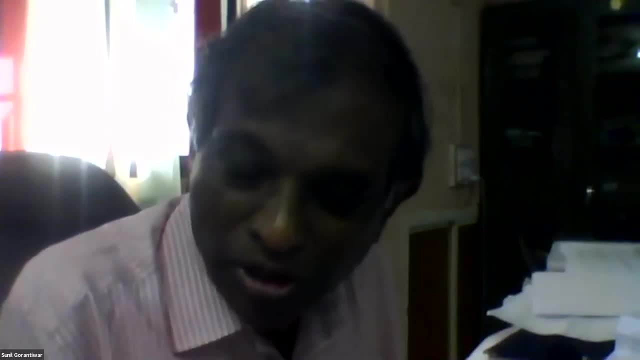 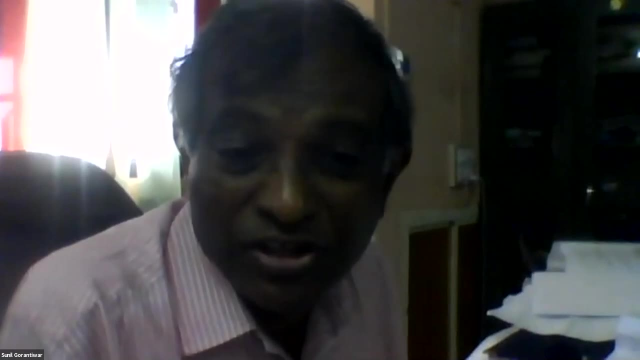 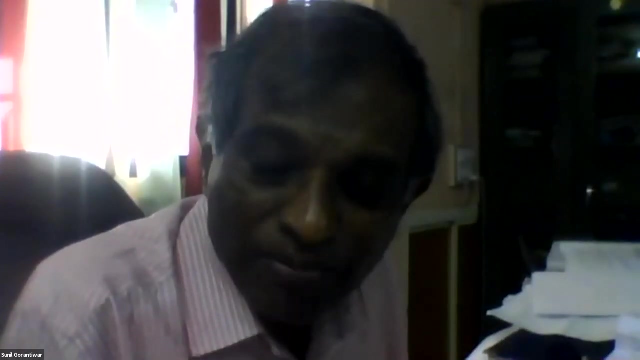 Okay, And then we also develop certain techniques. One such technique which is becoming very popular is that autofillet irrigation scheduler- actually- So maybe I will explain that in detail some other time, But this provides the tool for the precision irrigation water management in real time. 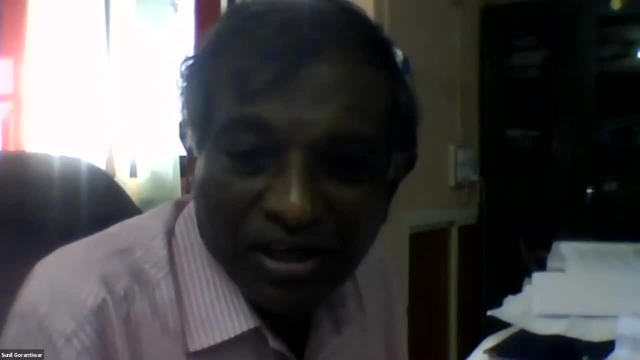 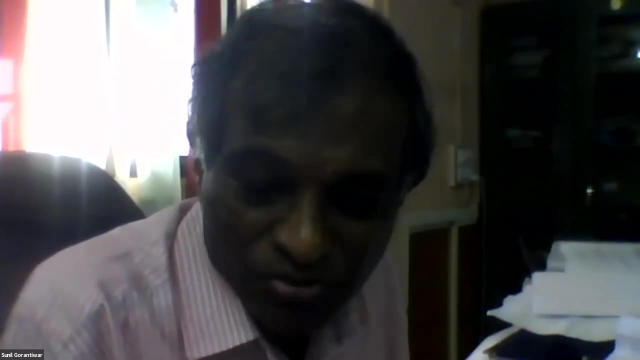 by considering all temporal and spatial variability in soil, weather, climate and irrigation system. So we devise many such other tools as well. And fourth objective is to disseminate this concept on the farmer's field, And for that we developed the concept of climate smart village. 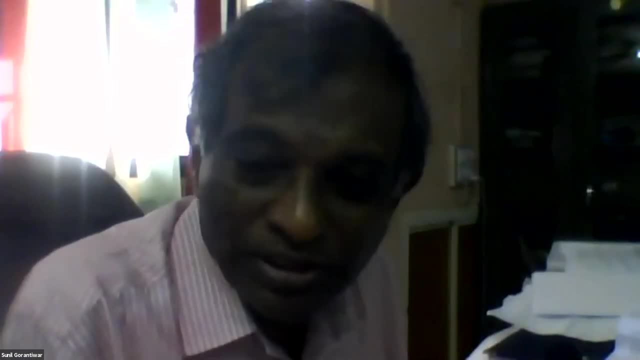 then digital agriculture village and green village, And, with the association of NGOs and other partners, we have started implementing all these concepts on the village level. So, basically, this is, in brief, about our objective And our program. I don't want to take much time. 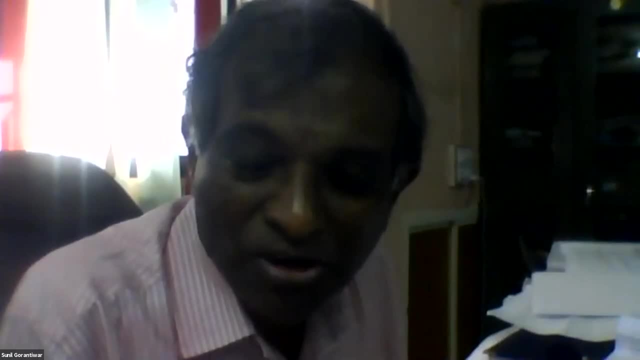 but just I wanted to emphasize upon our special guest, Dr Eldo, today, upon the activities that we are performing in this project, and also to the participants, those who are attending our training program for the first time. So I think, with this I would like to remain. 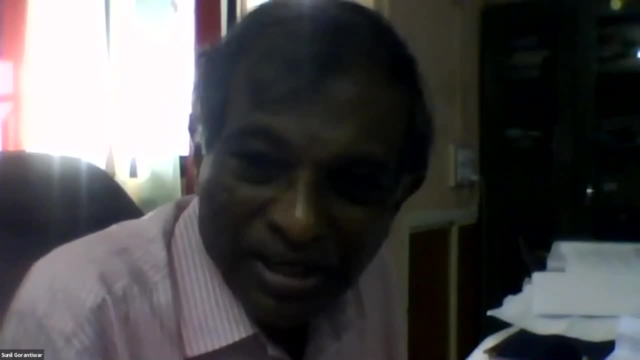 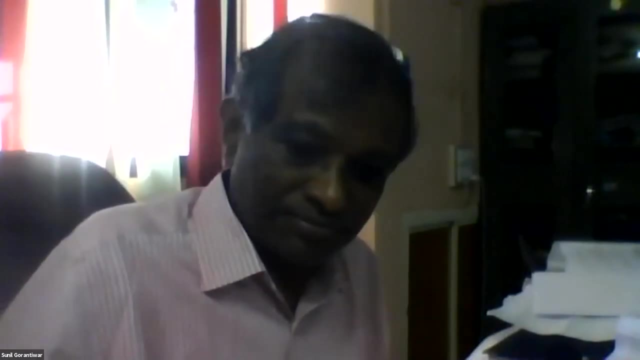 And I would like to welcome our very learned, esteemed expert, Dr Eldo. again, Thank you very much. Thank you, sir. Thank you for your brief preamble. Now I would like to request Dr Mukund Shinde, co-principal investigator of this CAST project. 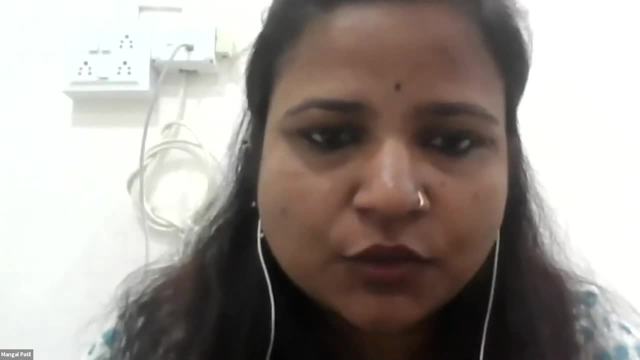 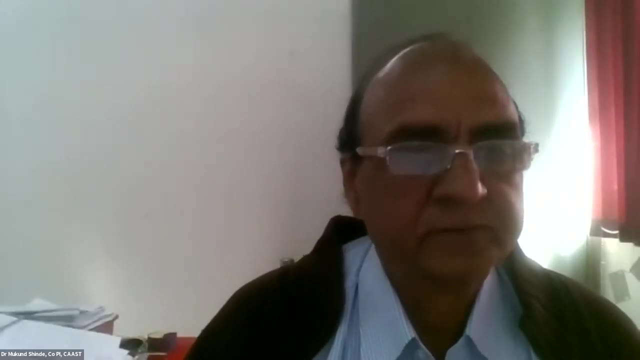 and organizing secretary of this program to welcome or to introduce Dr Eldo. Please, sir, Sir, please, unmute yourself. Yeah, thank you. Yes, sir, This is my privilege to introduce today's keynote speaker, Dr Eldo. 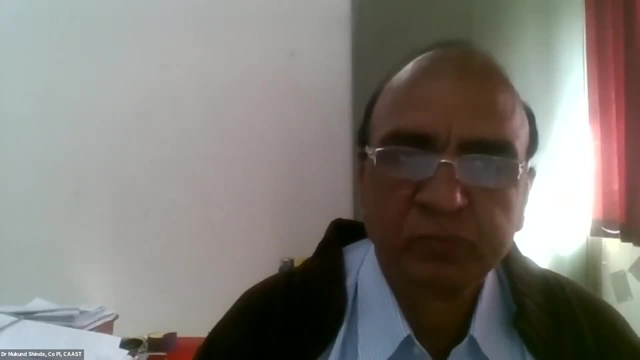 who is an institute chair. Dr Eldo has 28 years of experience in the area of water resources and environmental engineering as scientist, professor and also consultant. He works in the areas of fluid mechanics, coastal hydrodynamics and climate change impact on water resources. computational fluid dynamics. 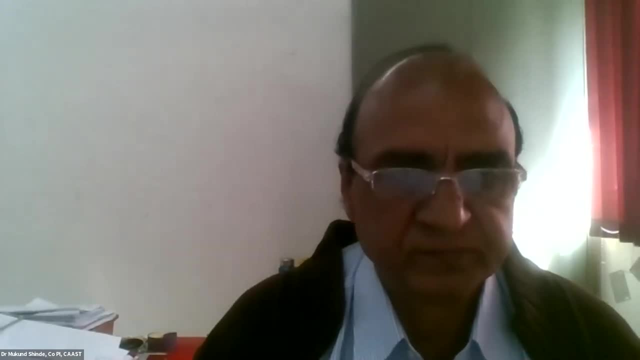 groundwater flow and contaminant transport. Dr Eldo has guided 32 PADs, four postdoctoral fellows and 55 master's theses, And presently he is guiding more than 10 PAD students in various areas. Dr Eldo has published more than 500 research papers in various international journals and conferences. 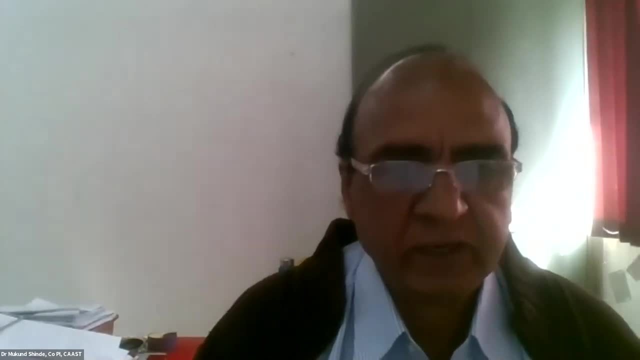 He has developed and offered 25 courses and a number of short-term courses for college teachers and working professionals. He has also developed two popular video courses on fluid mechanics and watershed management. Professor Eldo serves as an editor, associate editor and editorial board member. 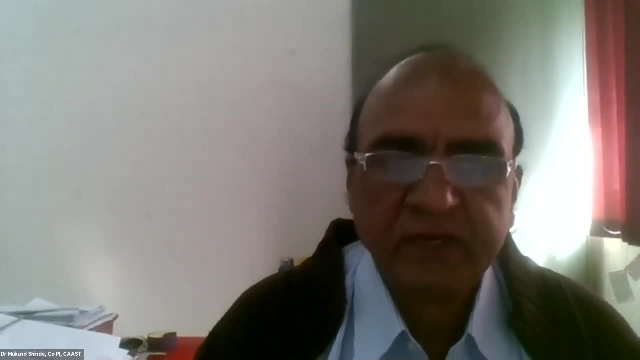 of a number of Indian and international journals and he has worked as a reviewer for more than 50 national and international journals in the recent past. He is also a research proposal reviewer for many research organizations and delivered several invited keynote lectures at various national and international organizations and conferences. 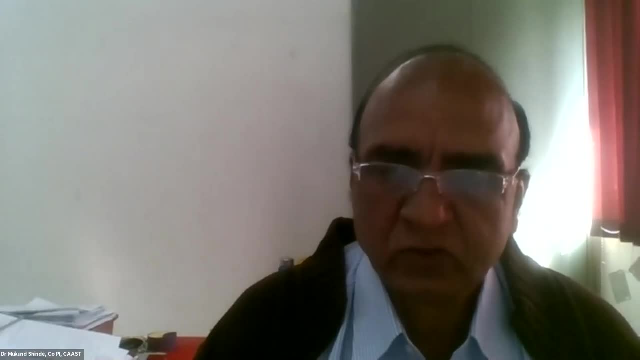 Dr Eldo has co-authored two popular textbooks and contributed 15 book chapters in various edited books. He is a recipient of many prestigious awards, including Eminent Water Resources Scientist constituted by Indian Water Resources Society in 2018.. So with this, I again welcome Dr Eldo and invite him for his keynote speech. 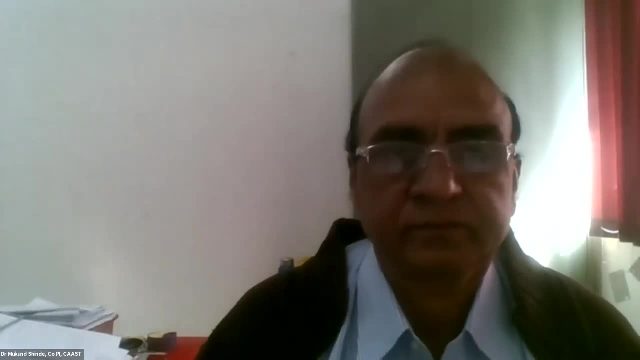 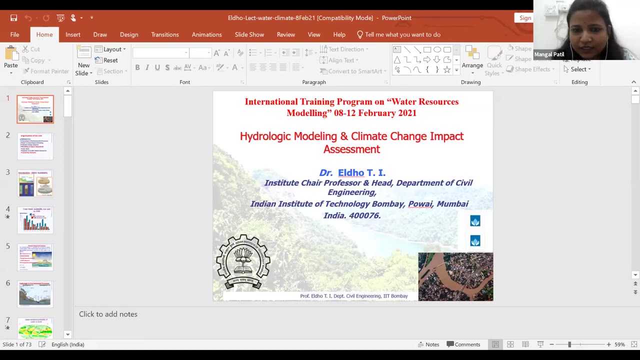 Thank you. Thank you, sir. Before starting the session, I would like to request Dr Gorantewar sir to welcome Garudkar sir. He has joined the session, Sir, please. Okay. One of the PhD students of Dr Eldo. 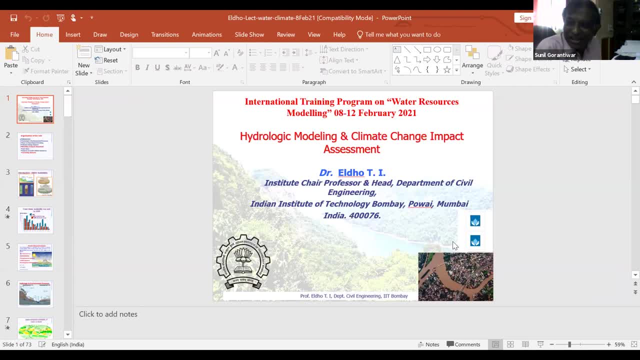 Dr Avinash Garudkar, who is head department of integrated watershed management at Valmy, that is, Water and Land Management Institute, Aurangabad. he also joined specially to take the benefit of Dr Eldo's lecture, So I would like to welcome Dr Avinash Garudkar as well. 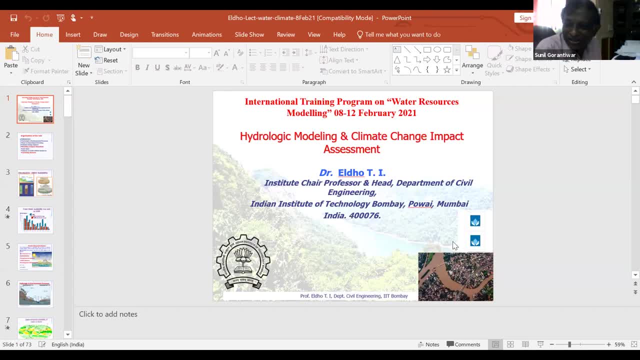 And if he wants to say hello to Dr Eldo, he can do so, And then we'll start our lecture. Yeah, thank you, Dr Gorantewar. It's a privilege for me to listen to Professor Eldo after a long time. 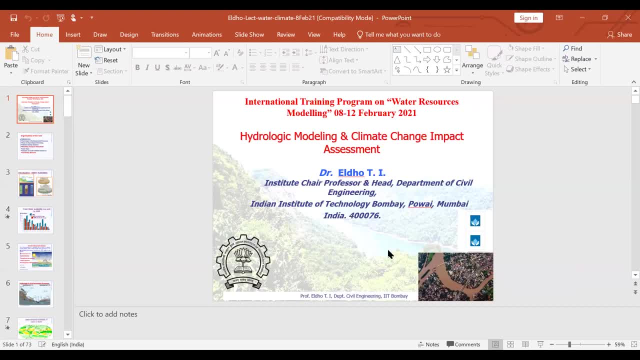 Quite often I'm listening to him And it's great. Okay, Thank you very much, Dr Mangal. you can proceed now. Thank you, sir. Now I would like to request Dr Eldo sir to proceed with the session. 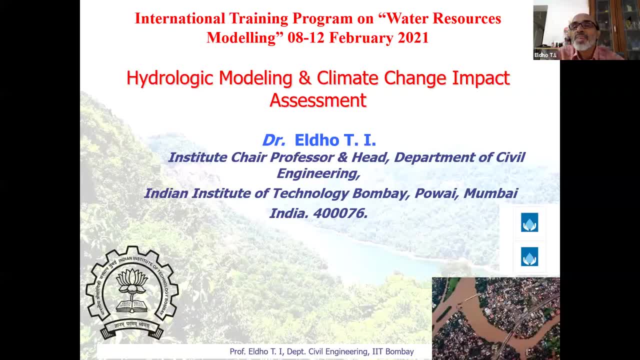 Okay, so thank you very much, Professor Gorantewar, Professor Shinde, Dr Mangal Pandit and all the organizers of this program, So I'm very happy to be here. Very good morning to all participants. I understand that around 200 participants. 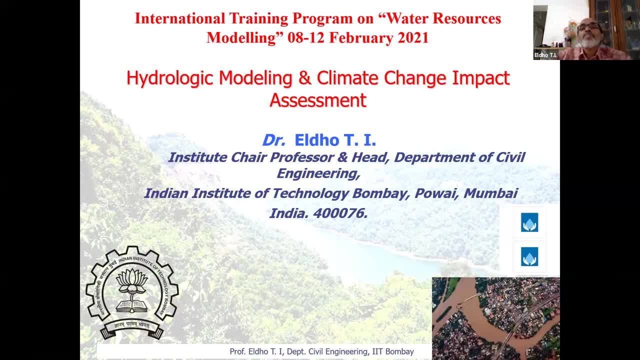 have already joined for this program. So I'm very happy to see that, though we are constrained with so many constraints like COVID-related constraints, and still MBKV is doing so much of- I mean Professor Gorantewar, his team is doing a lot of these kinds of online programs. 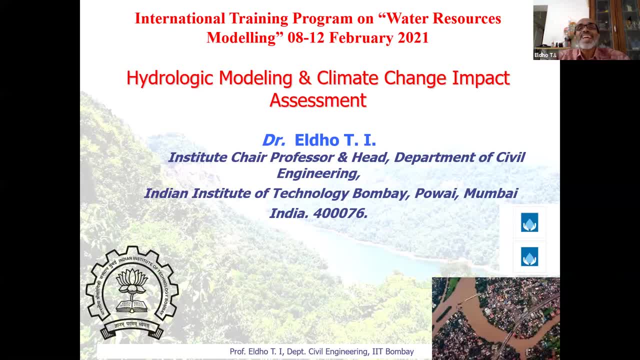 So I think people are doing much more than what we are doing in IIT, Since IIT we are a little bit. of course we do a lot of other things, But these kinds of programs we may be lagging behind. 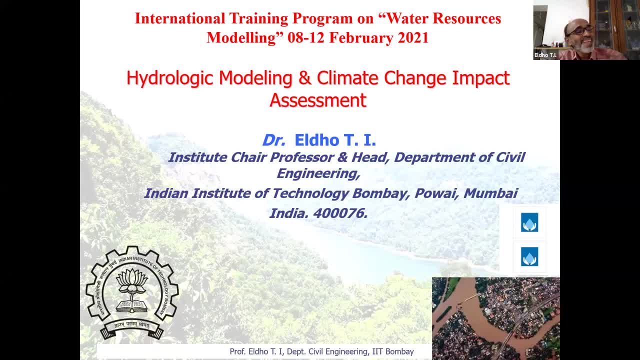 since I'm talking as head of the Department of Civil Engineering, So we generally prefer offline, But anyway, now we have to, everybody has to go these online programs due to various constraints put forward by the COVID and its situation, Of course. you see that that way. 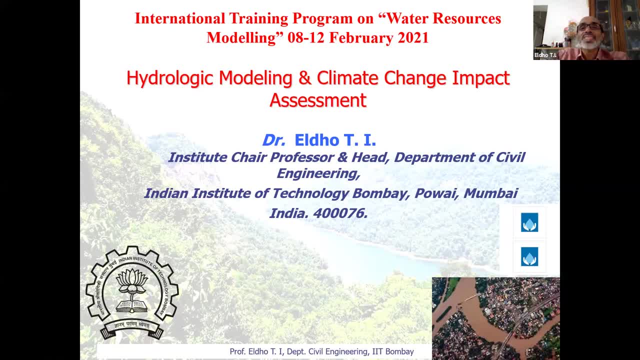 we can. we are getting other opportunities, like now. earlier, say, 30 or 50 years participants used to come to the place and then we used to interact with them And then now- so much of we need to do- a lot of say. 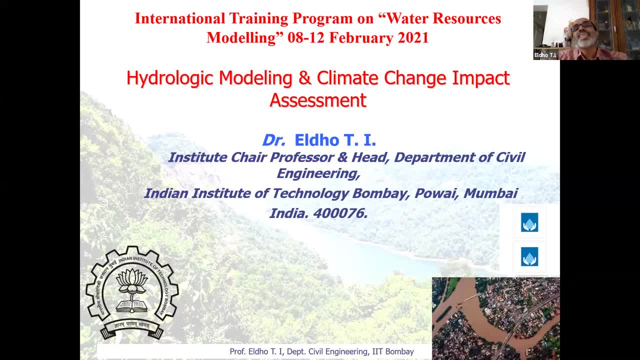 facilitation for all the people coming. But this way the advantage is that anyone all over the world- I mean this program can now become easily international, since all the people, from anywhere they can log in and then they can attend the lectures and then, of course, interact with the speaker. 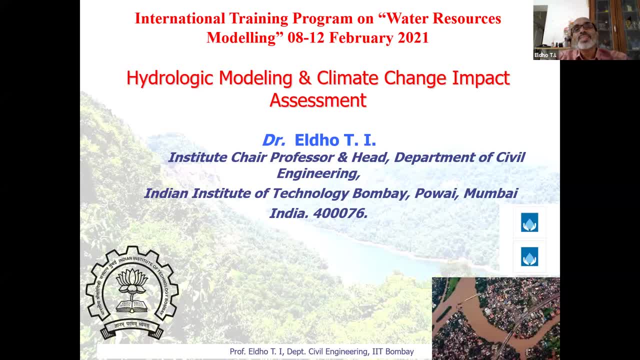 So, that way, I congratulate Professor Gaurandeva, Professor Shinde and all the teams for organizing such a very nice event, And I understand that a number of events are organized by this team, And I congratulate them. And now, without wasting much time, 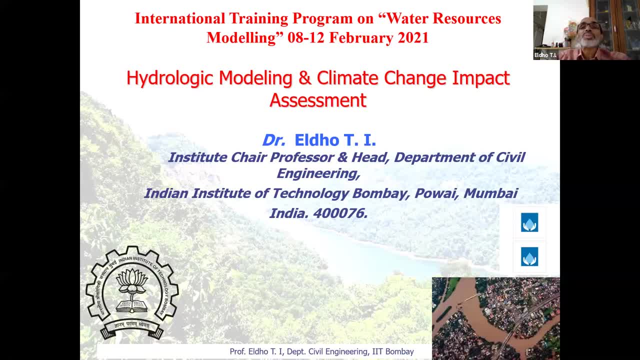 since I have given one and a half hour, only 15 minutes over, so I'll try to finish it within time. So my topic today, what we are going to discuss, is hydrological modeling. Actually, the topic is of the training program itself. 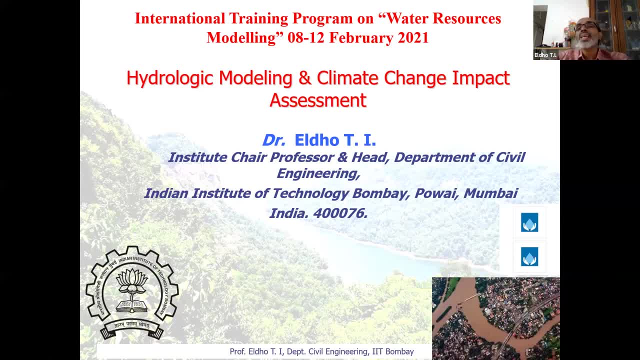 is water. So we'll start with hydrological modeling And then nowadays we are all talking about the climate change, So we are going to discuss what is climate change and how to do the hydrological modeling. as far as the climate change is concerned, 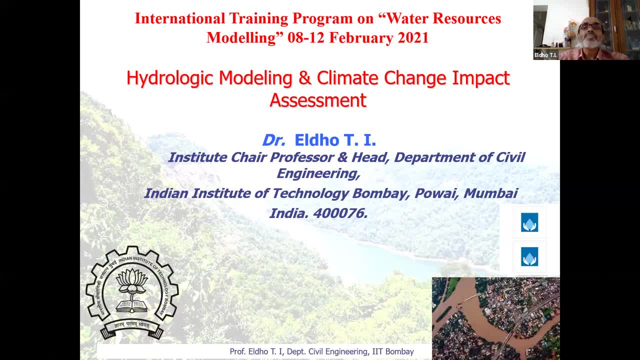 So that is what we are going to discuss today. So the topic is hydrological modeling, climate change and climate change impact assessment. So very similar kind of lectures I have given earlier also to various other programs, But of course we can discuss further. 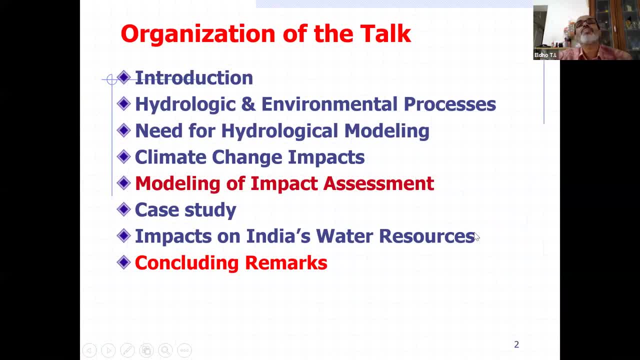 since this is a major topic where now most of the researchers are working, And then, of course, I'm very happy to interact with the participants anytime, whenever they look forward. So this talk will be as I mentioned. we'll be discussing initially what is hydrological modeling? 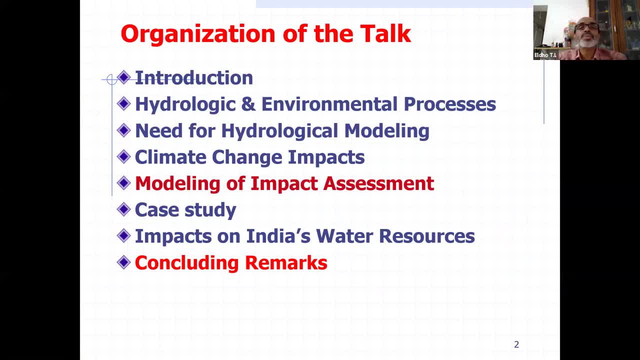 since the main topic of this year's training program is water resource modeling itself. So we'll be discussing what is hydrological modeling and what are the methodologies, or why hydrological modeling is important, Why hydrological modeling is required and what are the methodologies we adopt. 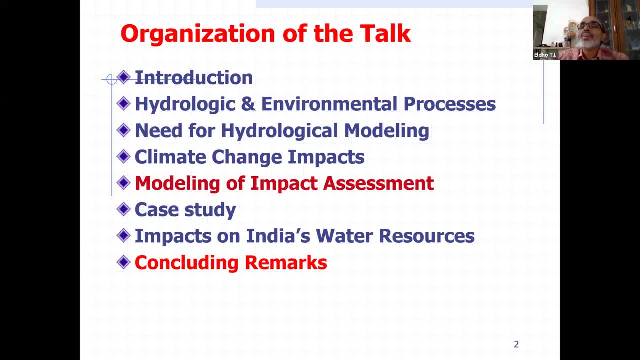 for hydrological modeling And then, of course. so one of the major area where hydrological modeling is required nowadays is the climate change impact assessments as far as water source system or river basins are concerned. So we are going to discuss about the climate change impact. 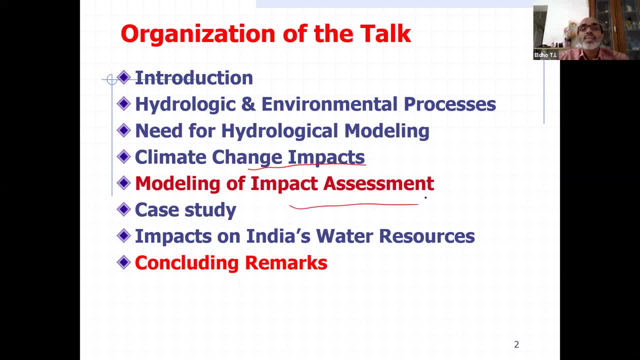 and then also we are going to discuss the say as far as India is concerned, where we are standing and say we'll be discussing, actually, one of the case studies which one of my PhD students has worked on I'll be presenting, and then, of course, the holistic way. 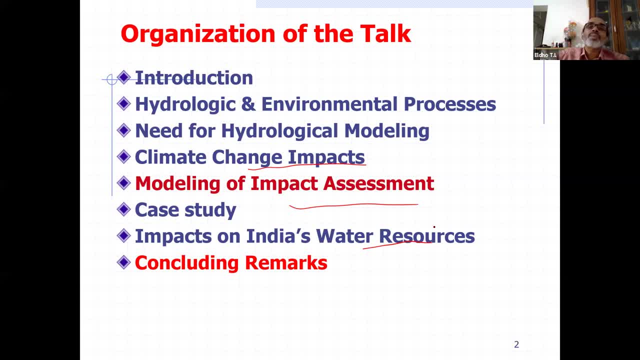 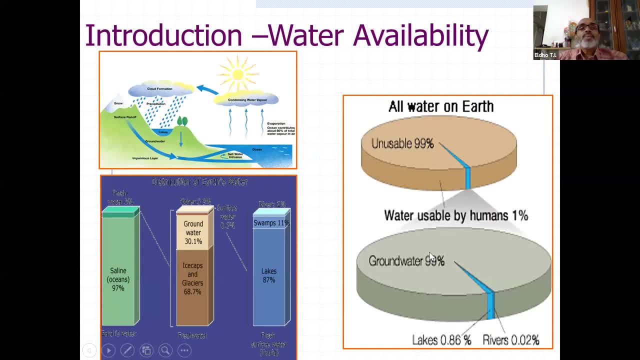 what can happen to India, based upon one of my friend's work, will be also. I'll be just highlighting, for the purpose of completion of this work, Of course, coming back to some introduction. So, as you can see, that say though we have so much of water. 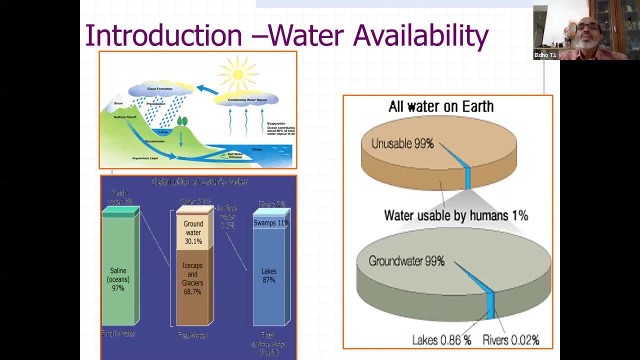 so most of the water available is not at all usable. So though you can see here, say available water, say so much of water is in saline water, and then, out of available usable water, almost 30.1% is in groundwater and then 68.7% is in glacial or ice caps. 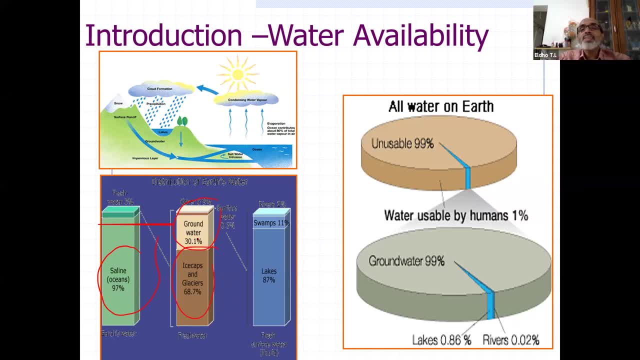 And hardly we are having a say, very less than 1% water or surface water directly we can utilize. So that way out of this is lakes and rivers and this kind of distribution you can see. So this is, everybody knows about it. but for the 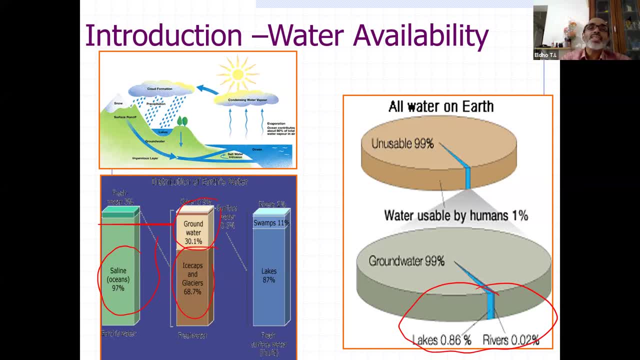 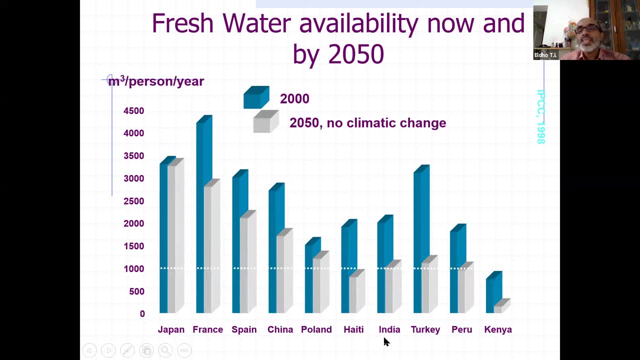 since this is the inaugural lecture, so I would like to highlight some of these points here. And then you see that now you see this is an old estimate but of course still it is valid. So here you see that, say, if you take the 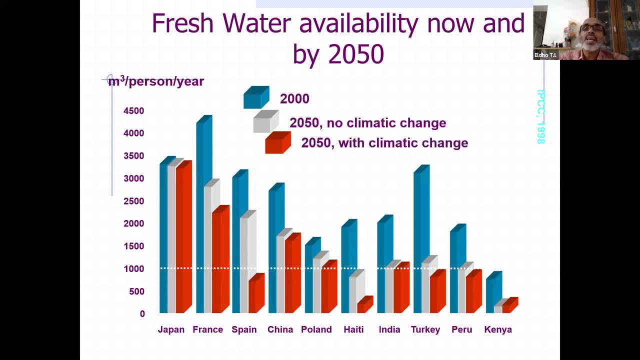 what is the, how much water is available, say, and then how much with respect to the population in Greece and with respect to the countrywide? you see that anyway, I don't want to go other countries details, but India is concerned. 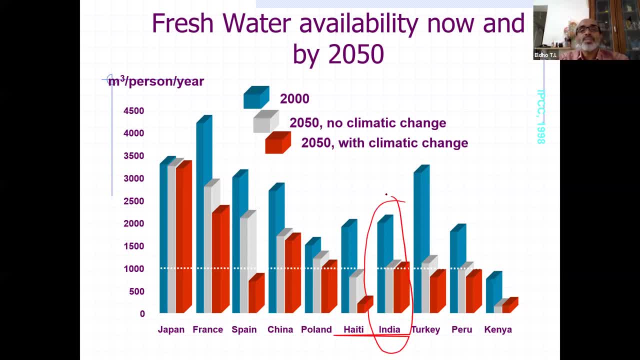 You can see that we are very much constrained with the available water resources. So you can see that in say 2000,- say I mean 20 years back, if you are having around 2,200 meter cube per person per year. 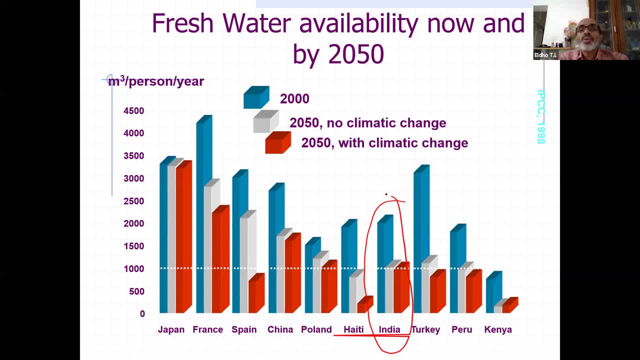 of water is available now by 2050, it is going to become almost half. And then the question is coming that, yes, this here, these kinds of climate change, but it can happen. You see that in Japan, America and France and other places. 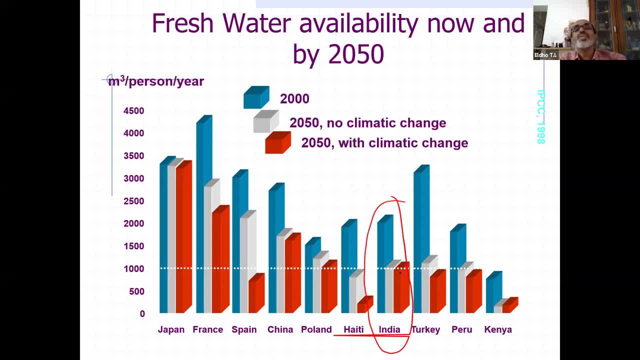 due to climate change. since their water utilization is too much and water availability is also too much, their climate change impact is also very much. But in India, since the water availability is very low, so that way the climate change impacts still there. 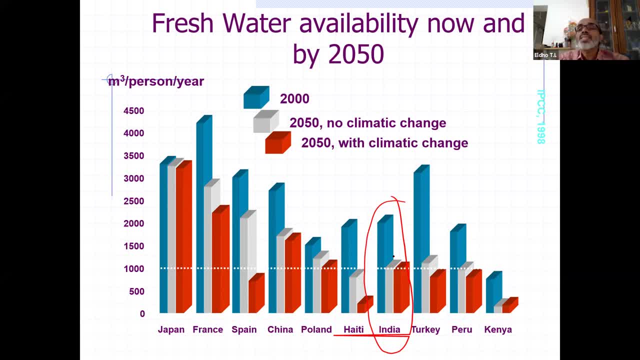 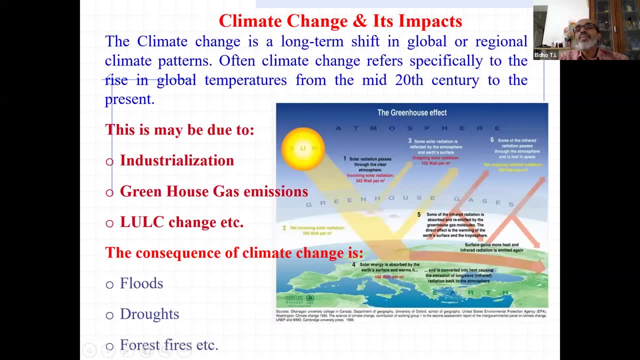 but you can see that that is a small percentage, since the availability itself is very low. So now, as you can see, that say various aspects that we consider as a holistic: water systems, and then river basin management or water resource management is concerned. 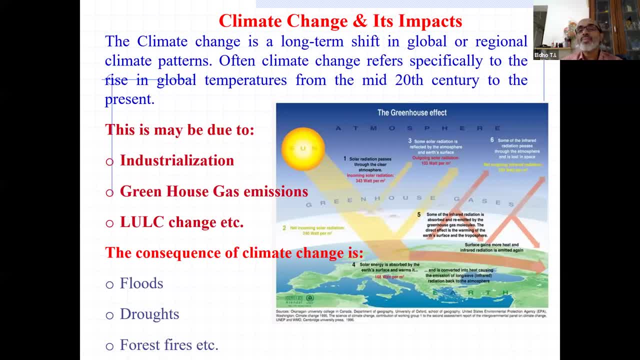 as I already mentioned, climate change is a very important factor which is now governing the hydrological systems And then also, it is already understood, almost the last 30 years. many experts are working in this area And, of course, we are concerned as a country. 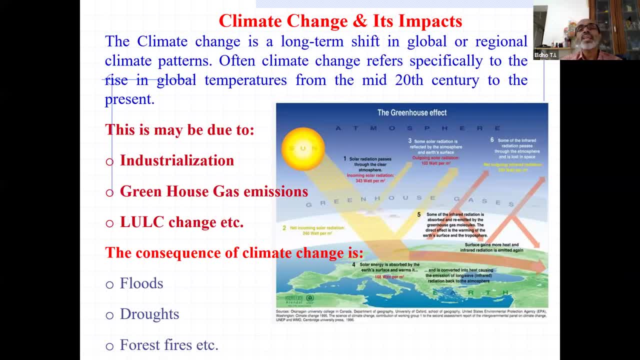 we are last 10, 15 years we are working in this area And actually we are lagging behind. And now, since, with the water resource ministry and various other organizations, we are now taking up various projects to study the impacts of climate change. 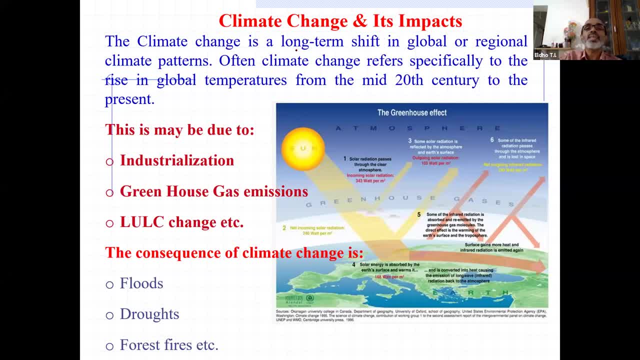 So the climate change impact, as you can see that the long-term shifting global or regional climate pattern often say climate changing. specifically, we say that with respect to temperature rise and then green house gas. So that is the main issues. 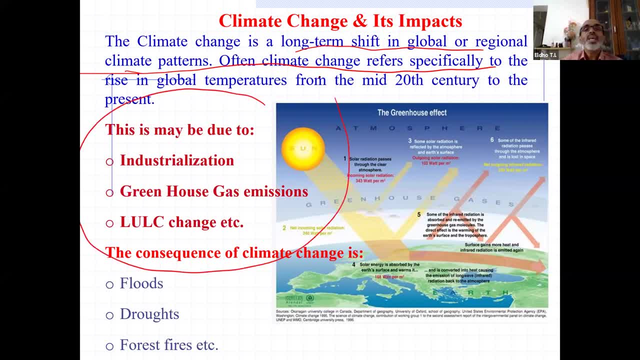 as you can see, depending on the perspective of climate change. So this climate change, of course, if climate change or not, climate change all the years we are having so many water resource related problems, So that you can see. 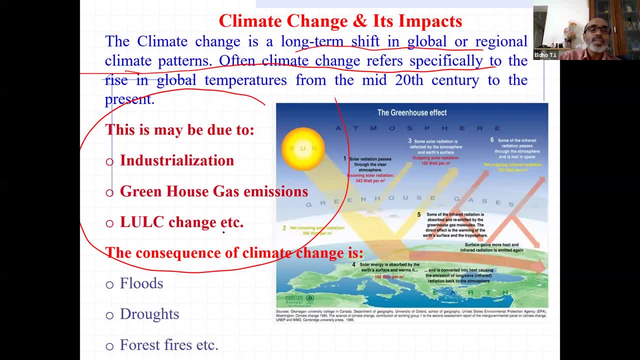 one is plenty of water during the monsoon season, And that is so we call it as floods, And then we can see that it is a major threat as far as one of the most severe threats as far as humanity is concerned. 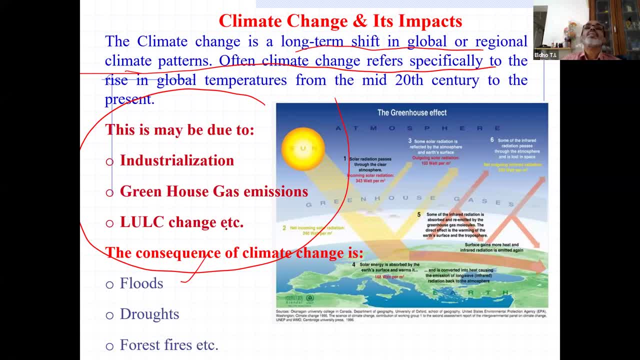 is floods, And then So that way every year, this recurrence, it is happening every year and we have got severe problems, And then of course, the water is available, say, especially of monsoon season, many part of our country is affected by droughts. 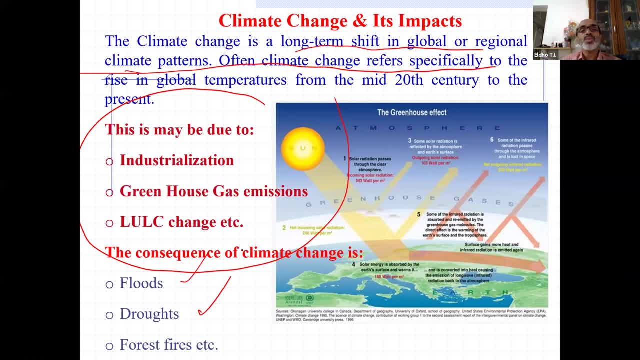 And then, of course, with respect to climate change. another issue is the, the forest fires which is reported in Australia and other countries in the recent past. So now, whenever we look, look all these problems, so we, we water resource engineers. 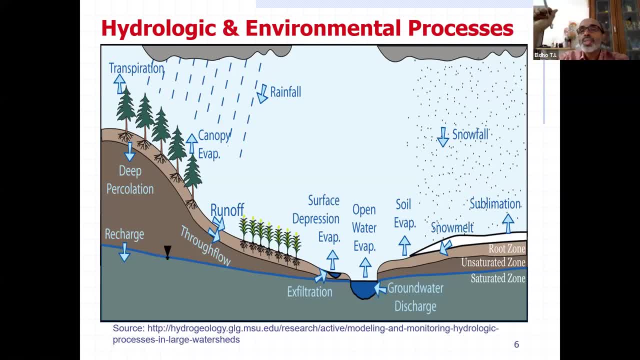 scientists, we always look into the problems and try to get a solution as far as the these issues are concerned. So here, when you take it as a, you can see the total system. you can see that whenever we see the water resource modeling. 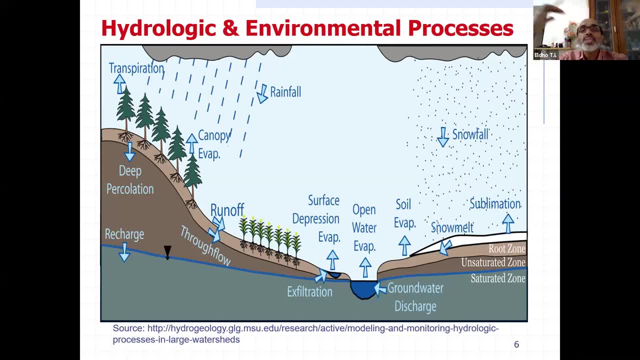 we need to consider, say, total hydrological and environmental system. So you see that this is all part of the the hydrology cycle. So when we start with rainfall, then we are having so many other losses like evaporation. 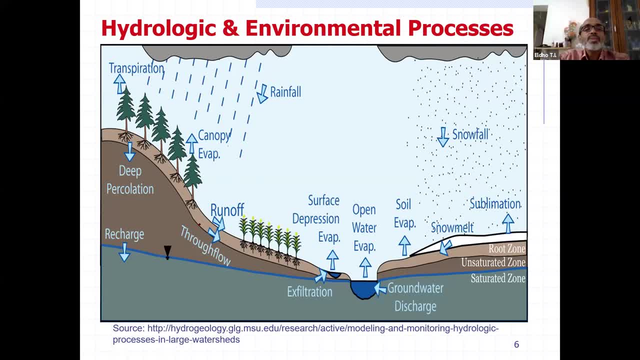 evapotranspiration, then deep percolation and finally coming to runoff and then again going back with the cycle. So so today's newspaper you can see that there is a severe problem of the, the glacial. 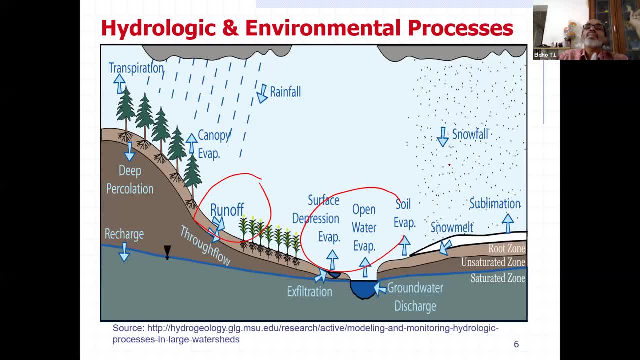 sephar and then then major flood and issues taken place in Uttarakhand. So that kind of system: whenever we think it is in holistic way, we have got severe problems one way or another way. So 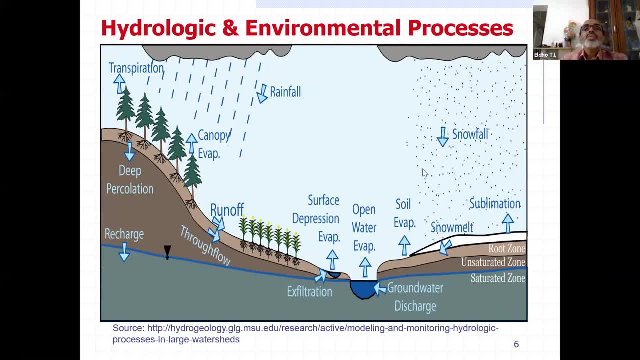 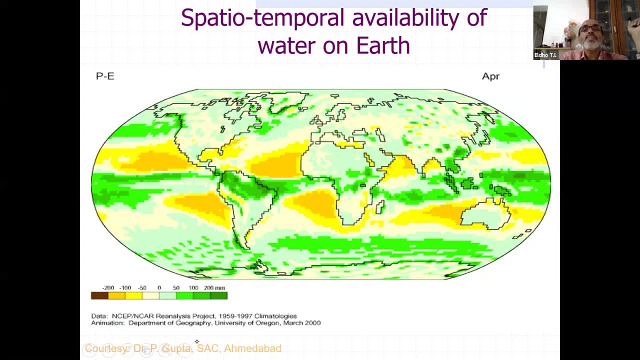 we need to take it in a holistic way and then we need to look into this. So this map generally, it is taken from say of say of so space application in Ahmedabad. So this shows the spatial temporal availability of water. 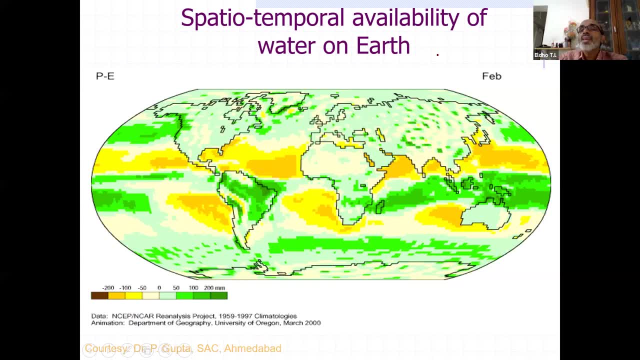 So here, if you are having sufficient water all the months, all the rainfall is uniformly distributed throughout the year, then there is no problem. But especially our country is concerned, as all of you know that we have got the monsoon season starting from June to October. 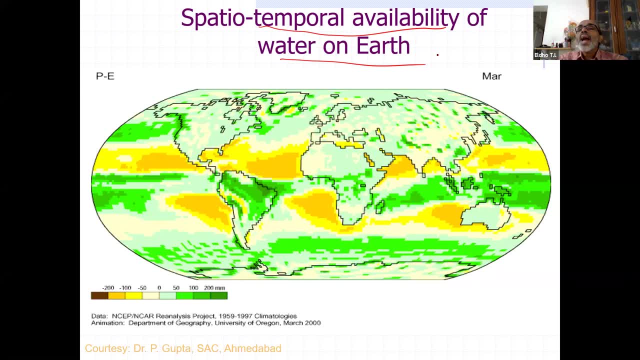 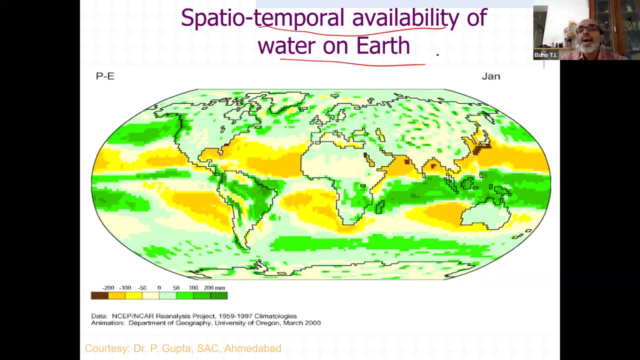 almost only hardly four months of rainfall and remaining eight months we have to depend upon, based upon this rainfall, and then we need to look into how we can manage the, the, the, the water availability, and how, and in a holistic way. 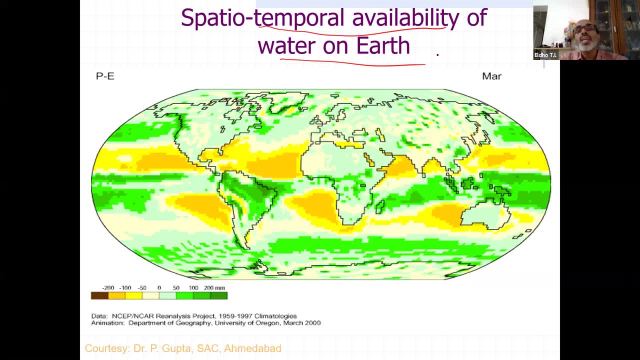 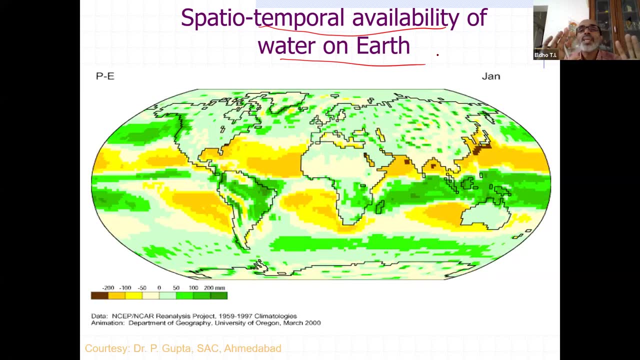 we can deal with the for the various purposes, including drinking, domestic or irrigation or other purposes. So that is the, the temporal variation. So we have only hardly four months of rainfall and eight months we need to deal with. 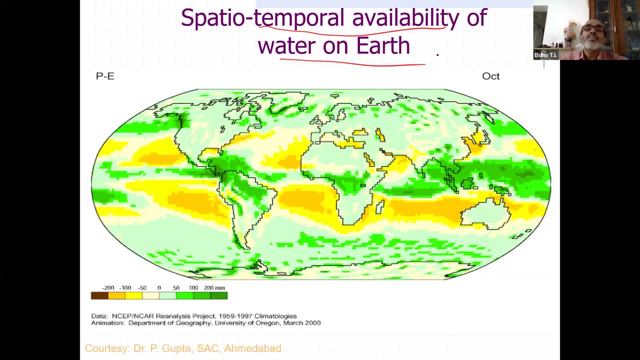 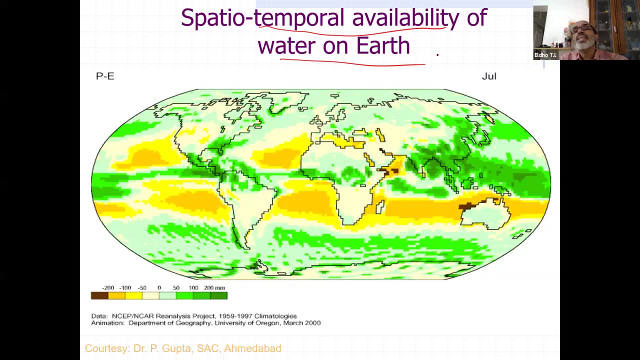 and if there is a shortfall in rainfall then the situation becomes very worse. So similarly the spatial variation. so you can see that, though India's concerned, the average annual rainfall is about 114 centimeter, so some part of the country. 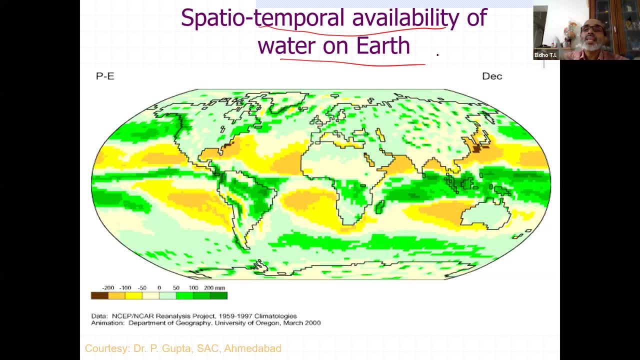 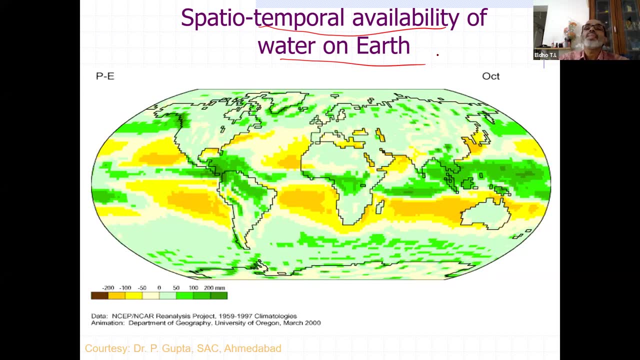 you know the, the, some part of the country. we get around the 350 centimeter 3.5 meter rainfall in the northeast and some part of the, the, the western ghats and but many places. 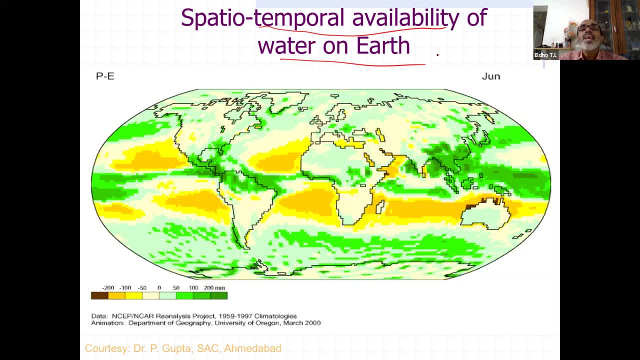 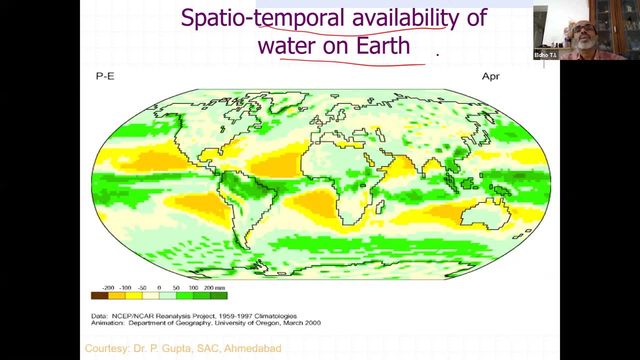 like. including the, the Rajasthan, it is hardly less than 20 centimeter of rainfall. I mean much less than 10 percent of what is the the average annual rainfall of the country. So that way, this is a major challenge. 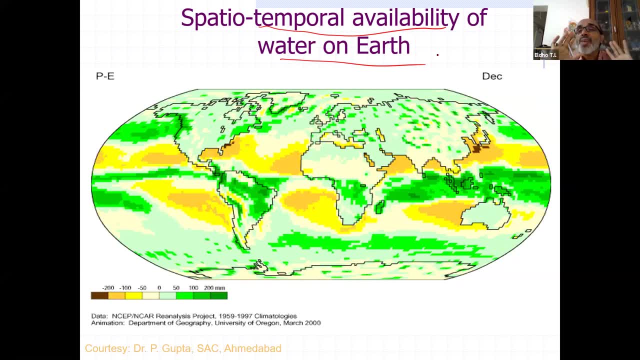 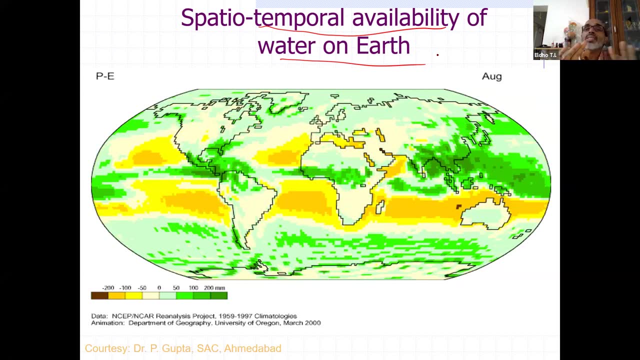 So why, as water resource model, why water resource modeling is required, or hydrological modeling is required, seems the the distribution, especially and temporal distribution, is too scanty. and then we need to look into: 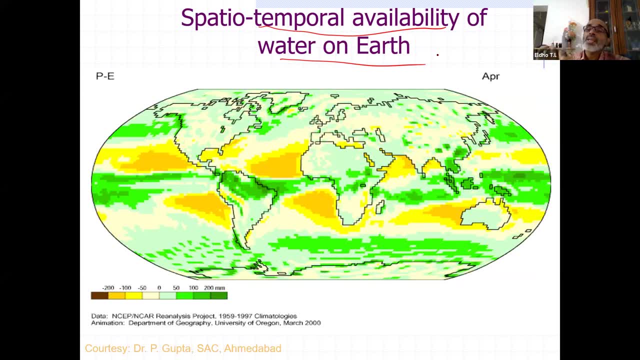 how effectively on a river basin scale, on a on a country scale, we can manage with available water, water resource for for all the needs. So that is why the spatial temporal variation is the the major issue. 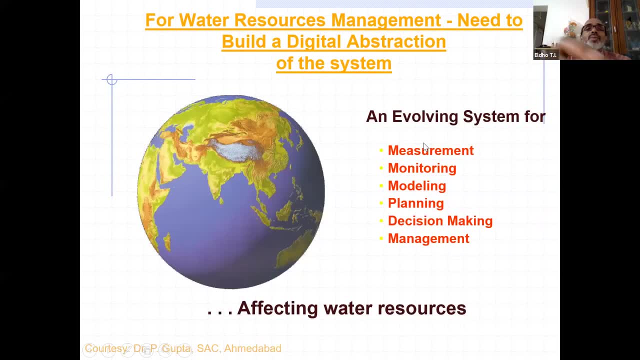 So now, coming back to water resource management and why modeling is required, So you can see that, you see, say, say, as as hydrological system, you can see that it is so complex, and then 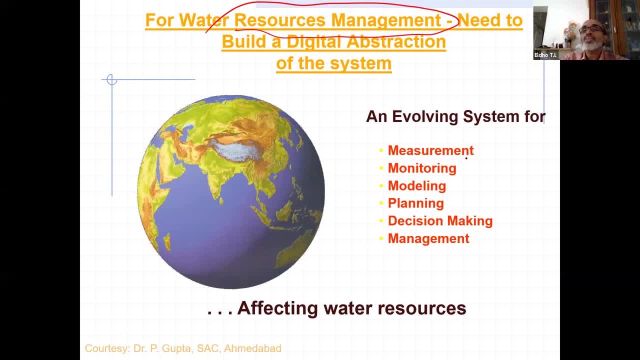 an evolving system, of course we need a measurement, So like we need to measure the, the, the rainfall, of course, in the material department has a series, say a good network of, say, rain gauge stations. 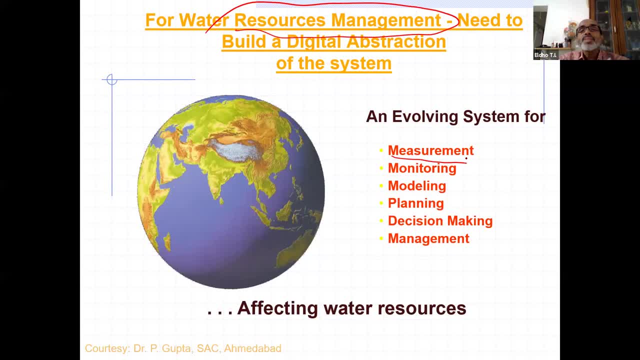 And then we need to monitor, especially the rain gauge station in various river basins, And that way we can monitor how much runoff is taking place. And but these both are very important aspects. but then 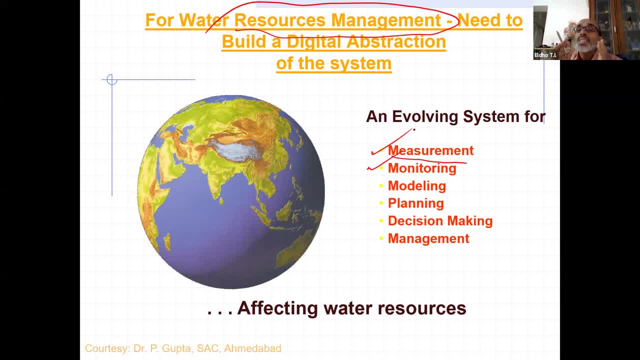 of course, when we want to see, in a holistic way, how much is the what is available, how much is the utilization taking place, and how effectively we can manage. So so you see that, finally, though, we are all scientists. 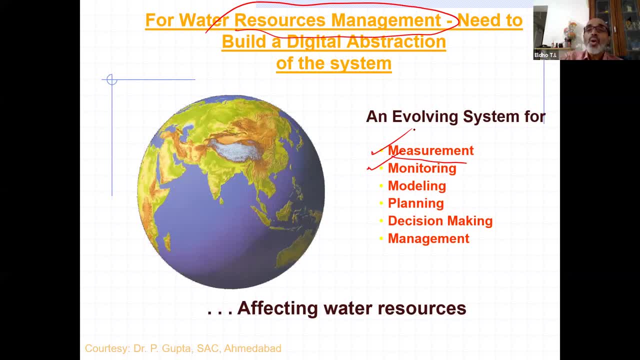 finally, everything is one way or another: management. So this is very, very important. So that is the topic which we are discussing in this five days. I mean this training program And then, of course, 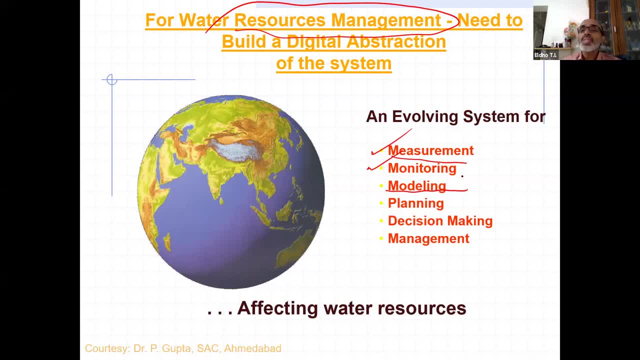 water resource model is so important. So this based upon water resource modeling only we can go for further planning. And then, of course, decision makers, who is either ministerial level or bureaucrats, or who are dealing the decision making. 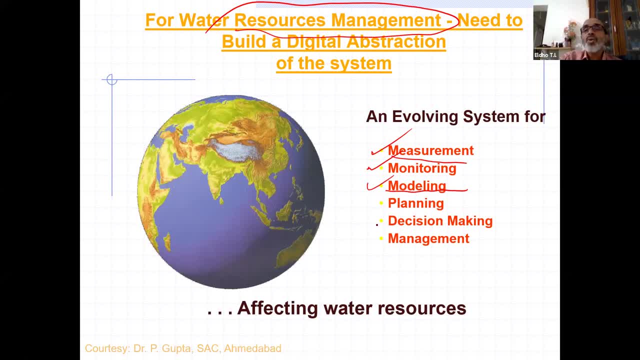 So these are all based upon the modeling And then as far as the decision making or management is concerned. So that way, when we consult the country in a holistic way, we need to take a say. 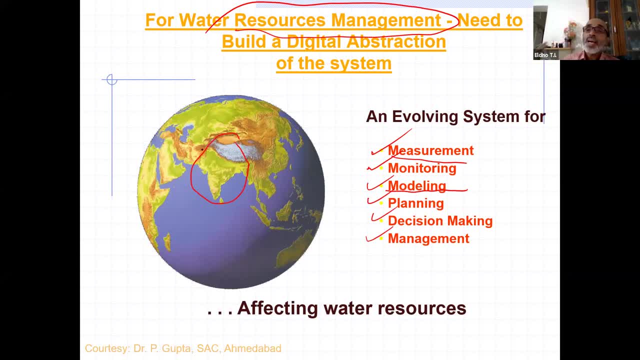 either more basic scale or say the state-wise or the country-wise. we need to do the modeling and then assess how much is available, especially on an annual basis, And then how the system will be behaving and that 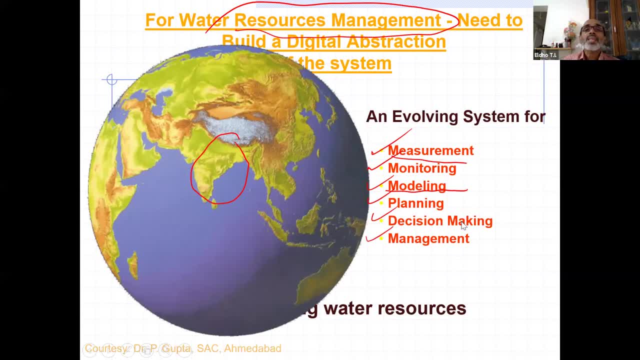 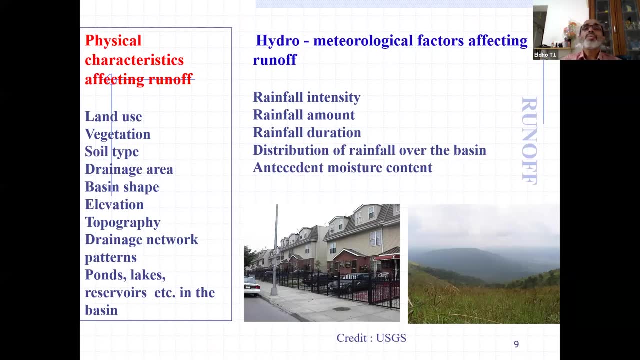 what kind of management, management measures to be taken. So now, coming back to hydrological modeling, we have to, we have to, we have to hydrological modeling or water resource modeling. So we see, we can see that one is the. 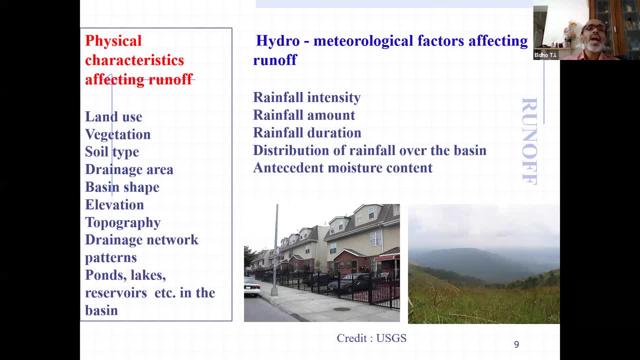 the the meteorological aspect. second one is the hydrological aspect And then, of course, the physical characteristics. So you see that whenever the rainfall takes place, you see, you see that when the rainfall takes place, we need to see what is happening. 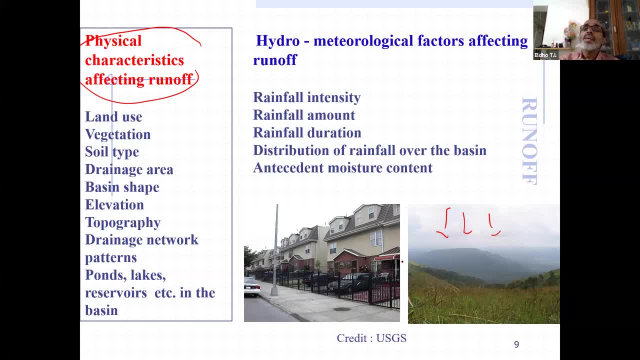 within the system. So the physical characteristics of the river basin or the watershed which we are dealing is very, very important. So as a water resource model, we can see that of course the unit is a watershed. 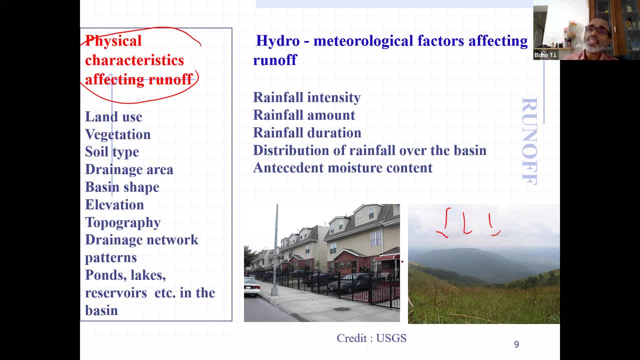 And I don't want to go to the definition of a watershed. I am sure that most of you know So. for example, if this is a river line and then we are having a system like this, we can cook it. 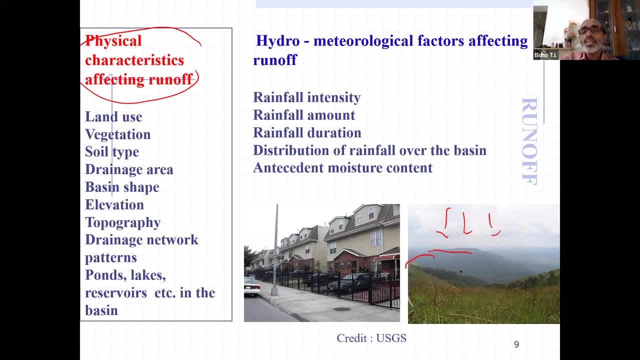 And that is what generally we call it as a watershed. There can be a river like this and all those things can happen. So now to understand what is happening within the system. so we need to see. 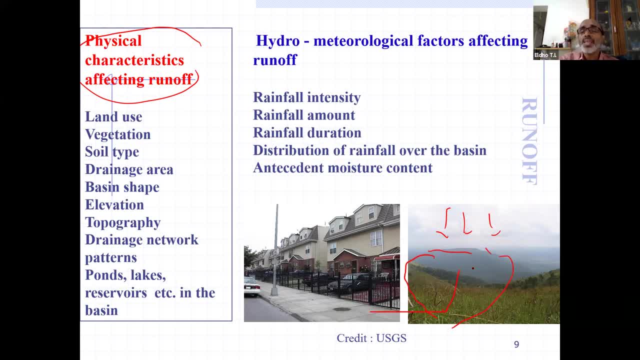 what is say, the geomorphological or hydromorphological aspects of the watershed. And that way, what is the land use, what kind of vegetation is there and what are the soil type? And then 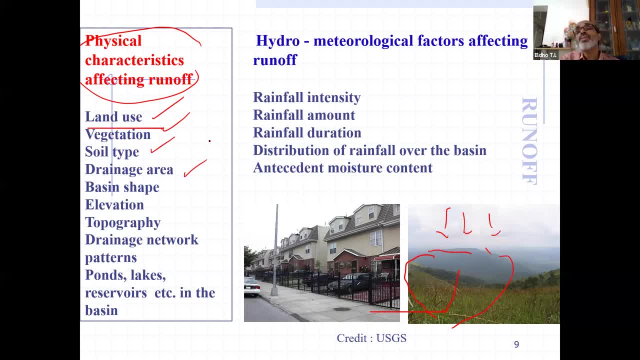 what kind of drainage system is there within the basin And then what is the shape of the basin? So that is also those who are dealing in watershed management, watershed modeling. they know the importance of the shape And 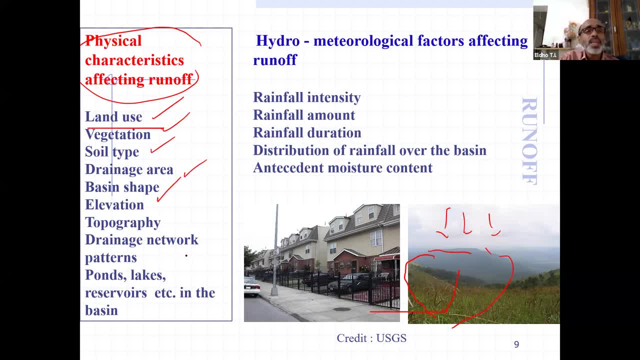 then, of course, what is the maximum elevation to minimum elevation? Then topography- All these aspects are so important as far as physical features of the watershed or the river basin or the geographical conditions- is very, very important. 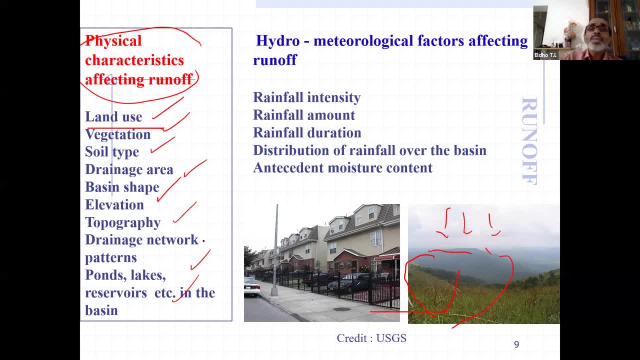 And then comes the meteorological factors. So meteorological factors, of course, you see that the so whenever we- I take lecture on modeling. so we have to see that what we are doing as modeler. 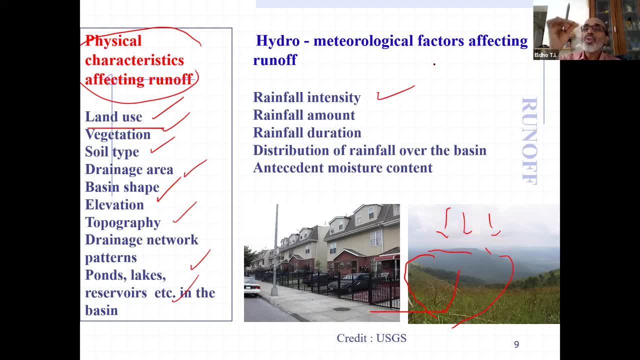 we were trying to see what is the excitation and the response. So, as all of you know that here the excitation is the rainfall. So rainfall I mean rainfall is falling on the river basin or the watershed. 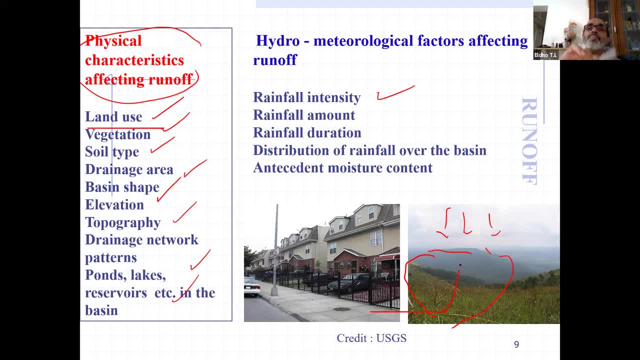 And then the response. we can say that it is the runoff. So the relationship is very important And this depends upon how much is the intensity of the rainfall, how much amount is there and how much is the duration. 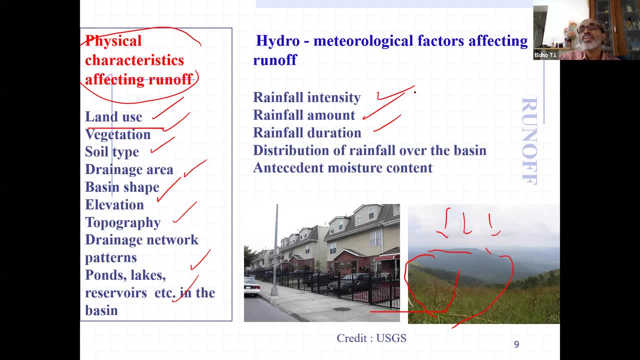 So these are all very, very important factors as far as water source modeling is concerned, or hydrological modeling is concerned, And that way, of course, we need to see, as I already mentioned, this is a hydrological process. 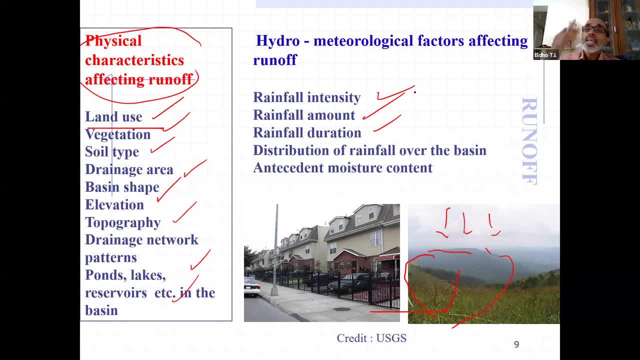 various processes takes place, like evaporation, infiltration. all those aspects will be taking place. So to see, to assess how much water is available, how much the system behaves. system means here the watershed or the river basin. 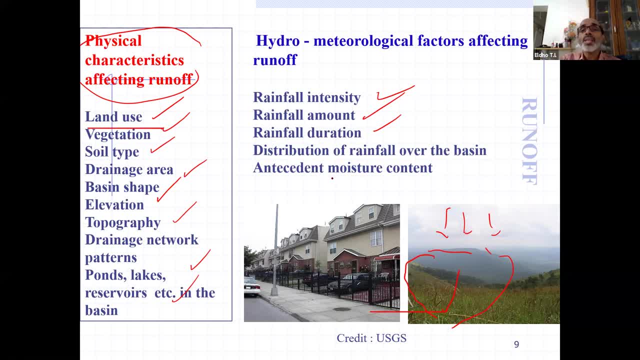 So to understand what is happening, we need to see that the moisture level conditions and then, of course, how much the evaporation taking place within the watershed. So that way, as I mentioned, it is always better to consider a system approach. 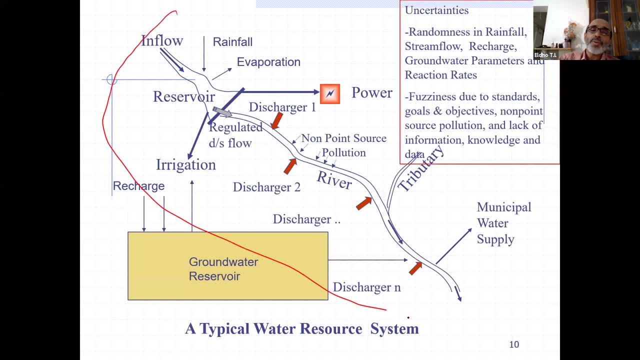 So here I want to call this as a system. So this is the river basin, you can see that, And then, of course, a lot of tributary and you know a lot of then. 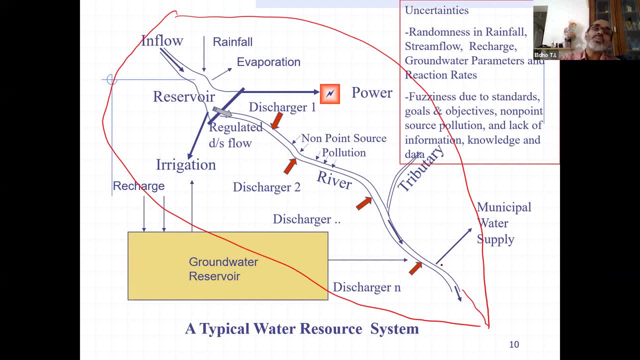 various aspects, how the water is utilized, all those things you can see on a river basin scale, on a watershed scale. So, of course, if the river is continuing from another small watershed down to the second watershed, so there can be an inflow. 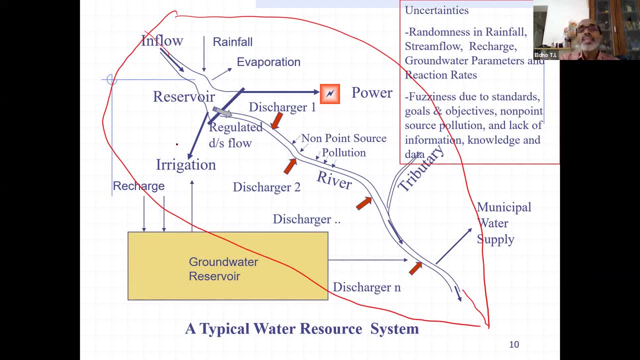 and then rainfall evaporation, all these aspects take place, And then, of course, the some due to the, the rainfall and runoff, discharge the river takes place and then say, for example, if you are going to- let us assume that we are going to construct here a dam- 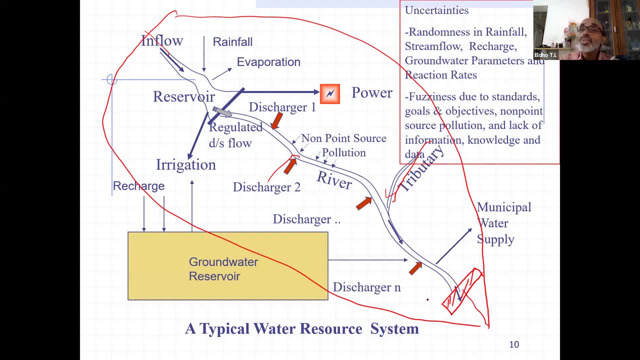 and then we would like to know how much what is possible to store and then how effectively we can utilize these, all those aspects to the study. So, in a holistic way, we need to look into all these aspects in a system-based approach. 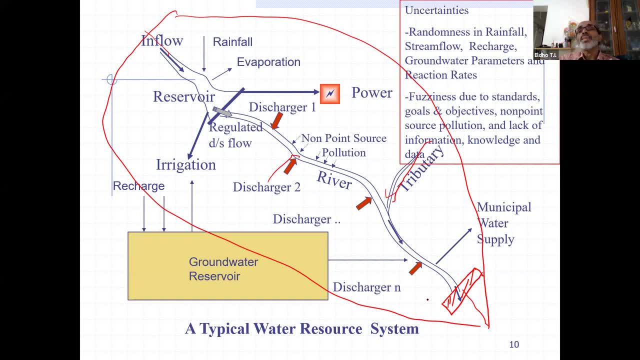 including the surface water and the groundwater, And then say one important aspects: whenever we hydrologists, when we deal with all these things, we need to see various uncertainties, like uncertainties with respect to the randomness in rainfall stream flow. 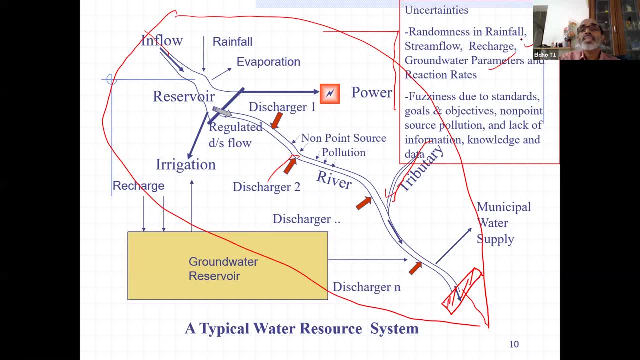 groundwater parameters, reaction rates, et cetera. And there can be also fasteners due to the the various issues. whatever they are, they are taking place within the system. So now, if, if we are going to construct here, 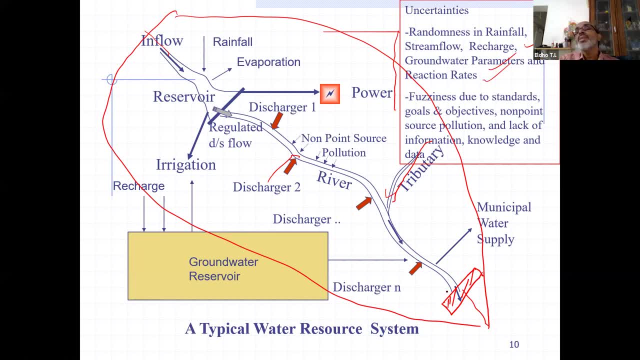 the, the, the, the dam here, or developing reservoir. so we need to see that, to say how much is the possible runoff and how much can be stored and how much is to be released. all these aspects. 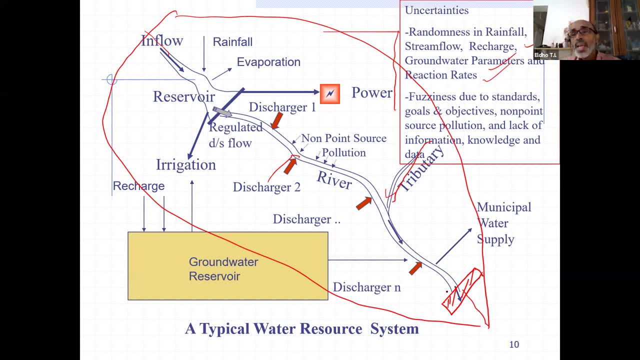 we need to take it as in a holistic way, So that way we can say that the system, it is a in a system approach. this is so complex. So many of my friends here are civil engineers, but 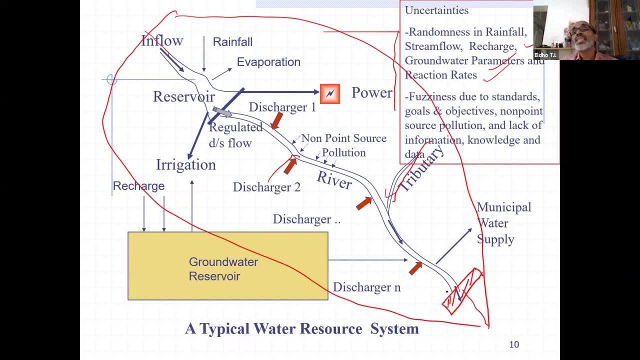 I used to tell the civil engineers. so, though, since civil engineering, structural engineering is the most, people think that there's the, that is the most difficult aspects, and all the civil engineers goes for structural engineering, But I used to say that 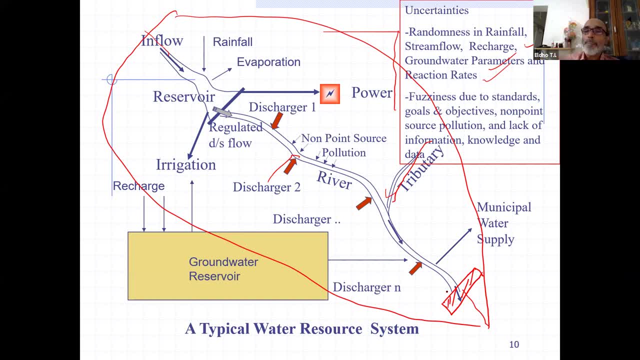 this since we are dealing with the nature, so the nature is so complex. so to deal with the nature and to make a model and to develop a planning and management or management model, it is so complex compared to even. 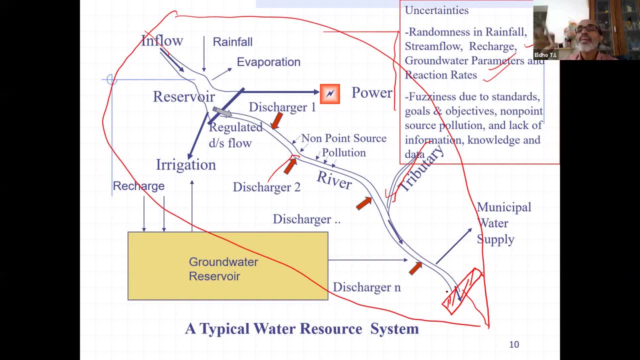 designing a 100 storey building or even planning of a of a city. So that way we are dealing with the nature and there are so many uncertainties involved and we need to deal with these kinds of uncertainties. 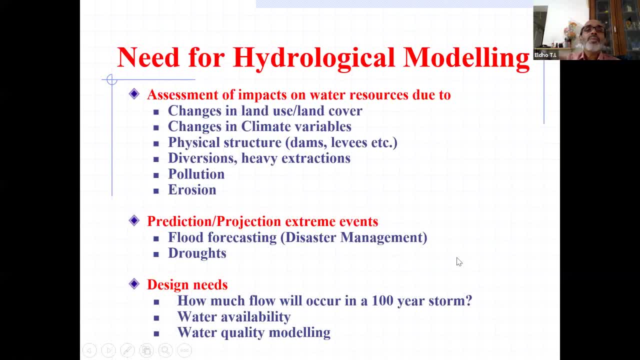 one way or another. So that way, the question I mentioned earlier. when we are dealing with these kinds of problems, we need to ask questions. So the all the engineers, scientists, all the students or faculty here, 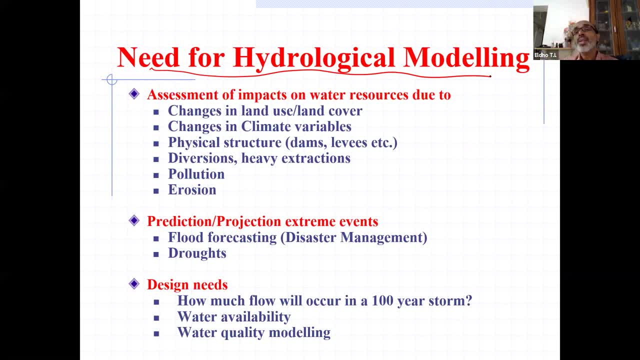 I would like to pose the question what, why we need to go for model and what are the importance of this model and how the model is developed, and then how we can apply such models so that we can. 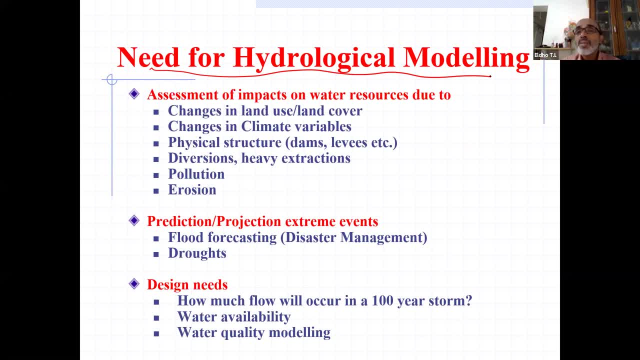 go for further management of the system. the system means here the watershed or the river basin or the underwater source of the country. So that way we need to go for hydrological modeling. the answers I have listed here: 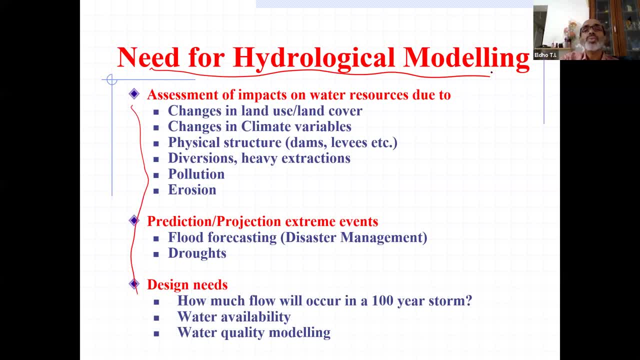 So, first one is the assessment of impacts on water resources due to various aspects. So, as I mentioned, since you see that the water requirement is concerned, farmers need water, the domestic purpose, industry purpose, various needs are there. 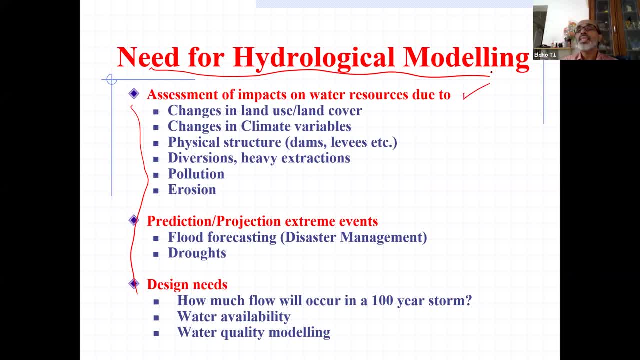 So that way, especially, you see that in a country like India, and the water, the majority of the water, is needed for the agriculture purpose or irrigation purpose. So that way, and you see that the land use. 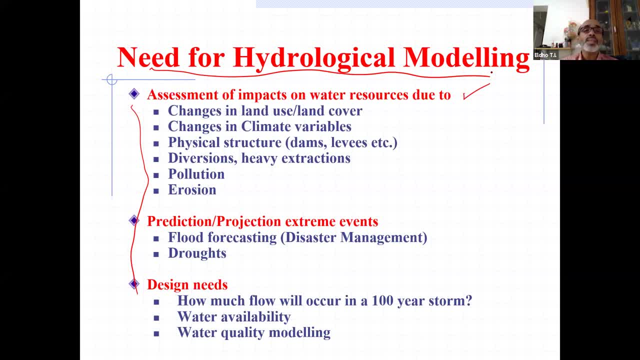 land cover. change in the watershed is so important, So we need to study what are the changes in land use, land cover and then, of course, the major the, the, the. the input coming is from the rainfall. 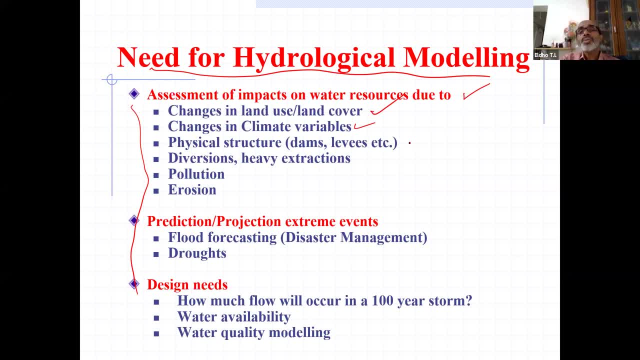 So we need to see the various changes in climate variables. And then of course you see that last say 70 years or 75 years after the independence, we have developed so much of dams and 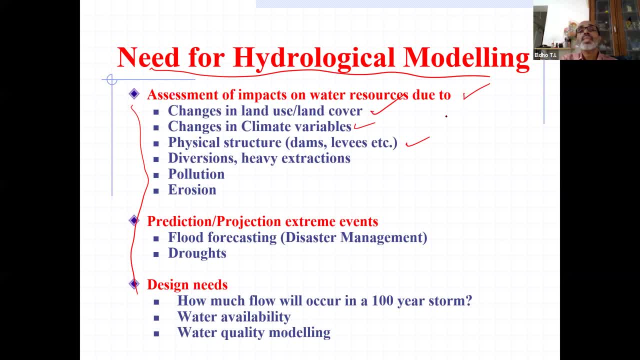 structures were made and where is the structures located? how effectively we are utilizing and like diversions. and then, of course, another important aspect is the pollution. So water resource pollution is a major problem. So most of our rivers are polluted. 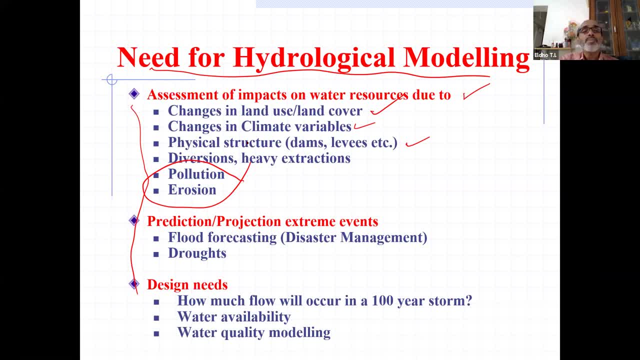 due to the, the contamination taking place from various sources, And then, of course, another disaster is the droughts. There were no water is available for long duration. So in a river basin or in a 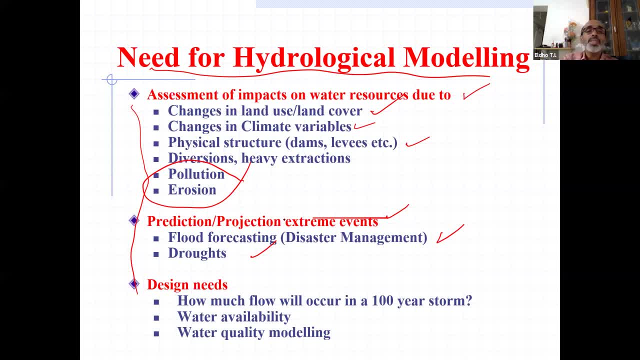 watershed, So there is no prediction or projection of extreme events. And then what are the design needs? So we need to answer these questions since, for example, if we're going to develop an airport, if we're going to develop, 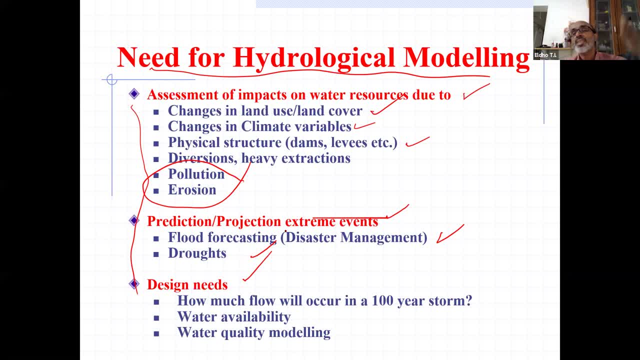 an infrastructure, then we need to make an analysis with respect to the intensity, duration, frequency curves. I mean, in 100 year return period, how much is the maximum flooding can taste? So all these assessments are needed. 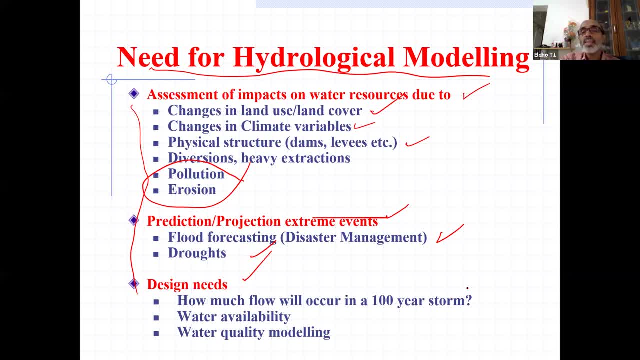 So that kind of design is also. we need to look into, like how much water is available on a river basin, And then, of course, water quality is also important. So, as I already mentioned, my first slide itself: 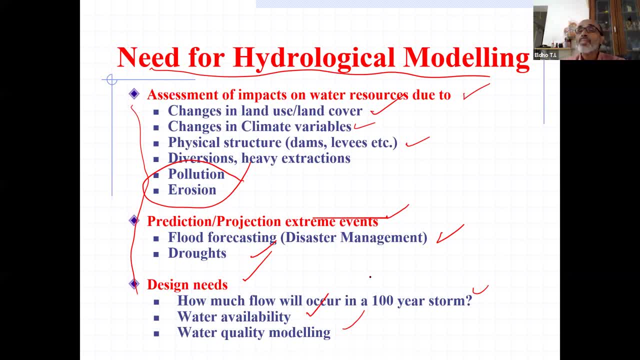 if so much water is available. since seawater or salt water is available, that is, there is no use of it. So that way, water quality is also important. So now, whenever we look into that is, 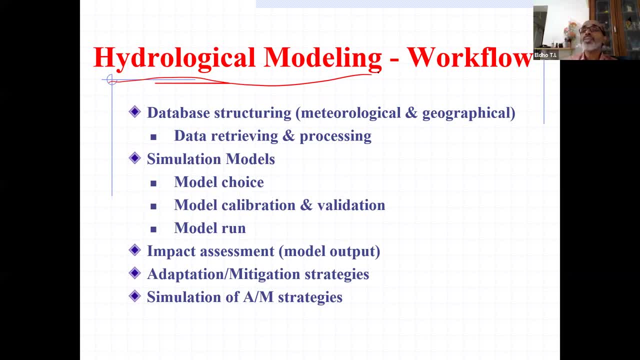 so these slides I am discussing here to show the importance of hydrological modeling. So I hope all of you understood so important is the hydrological modeling and why we need to go for a system-based approach. 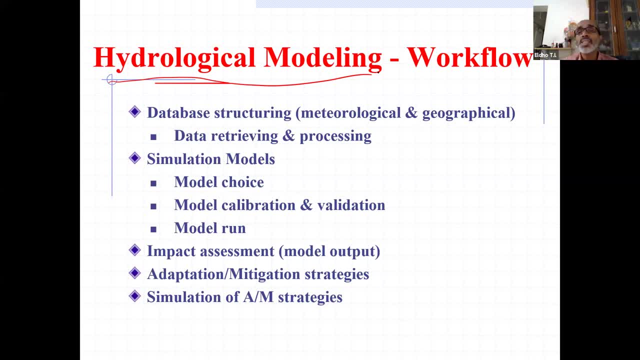 and then what are the important aspects we need to consider for such such studies? So now hydrological modeling. if you go for hydrological modeling here, the various workflow components is already mentioned. So, as I mentioned, 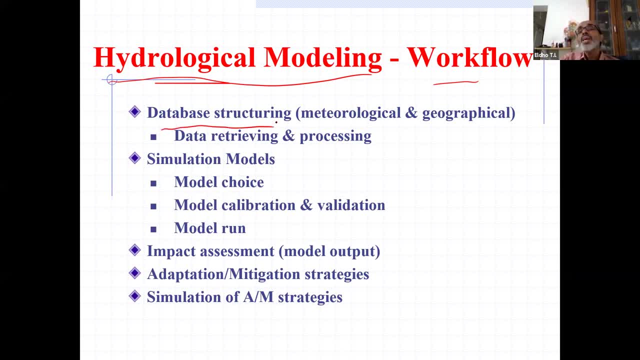 the system is so complex, so that way it is always. we need to have a database structurally, so that can be, you know, geographical conditions databases like your digital elevation model, land use, land over soil. 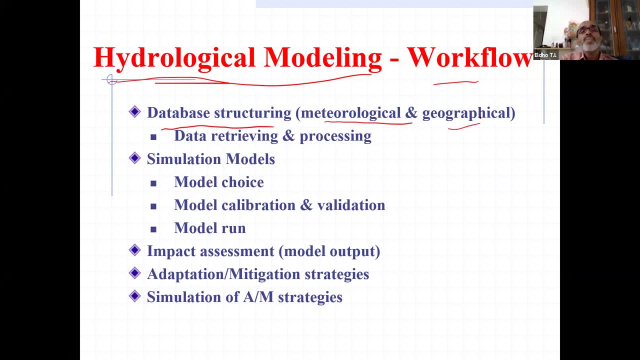 all those things are needed. and then of course we need to also have the meteorological aspects. So that way, depending upon the needs. so now, with various government organizations we are having now, all of you know that. 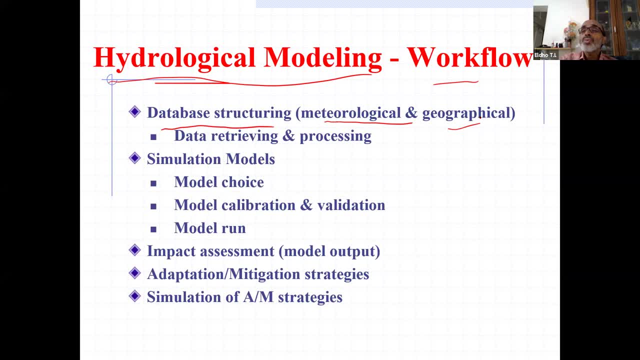 we have got the hydrology project. second or third phase is now going on. so the due to, with the support of World Bank and other organizations, we are collecting the data over the decades, and then that process is going on. 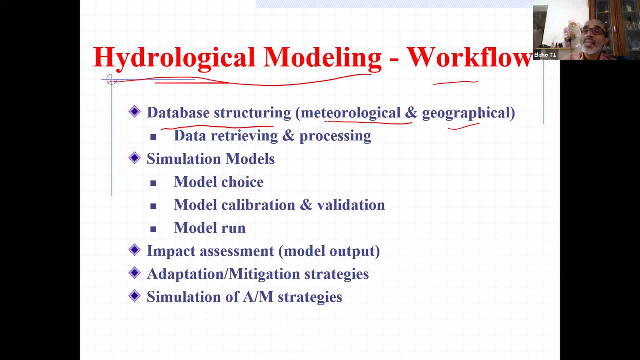 so that data. we have to see the accuracy of this data and then, whenever needed, we need to retrieve the data and then process it so that the, the researchers who are working on this, they can easily. 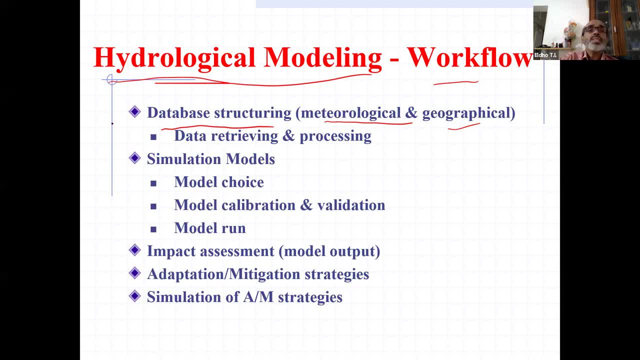 do their research and then study it. And then- so that is the first aspect in hydrology- the database or the data needs as far as the watershed modeling or water resource modeling is concerned. And then 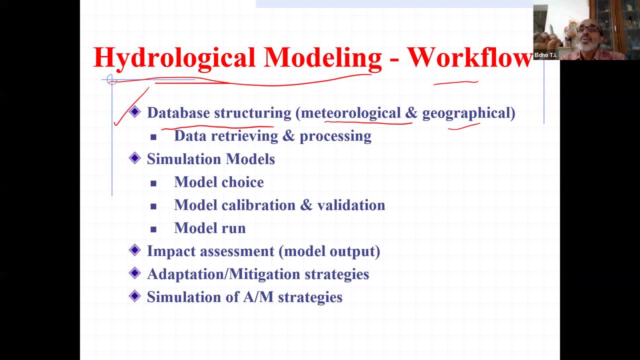 of course, as I mentioned, then the data is either: if you put have the accurate data, then you will get better results, but if you have got the junk data, the your model results also. it is not a problem. 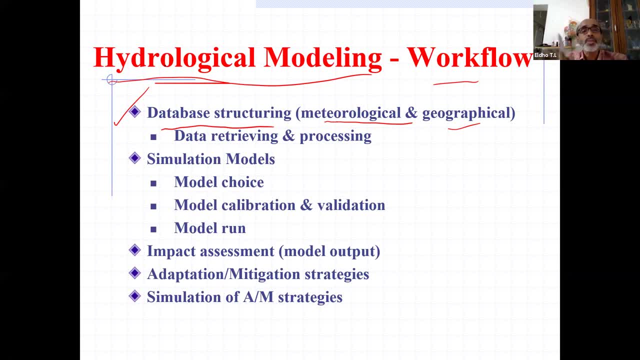 of the model, but if the result, the data, is not correct, then of course whatever you are getting will not be useful. So that way. simulation models. second aspect is simulation models. so database is very important. data accuracy is very important. 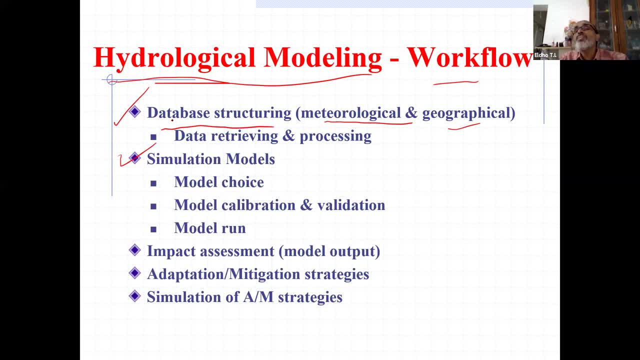 and second aspect is the simulation model. So then you see that this hydrologic modeling, many researchers, many scientists and engineers are working in this area. so large number of models. so, according to the famous Professor, 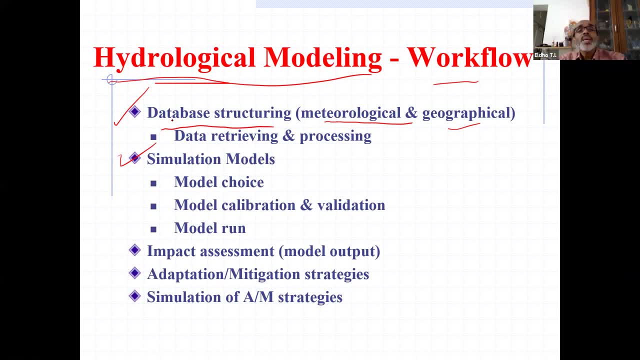 Professor Vipi Singh. thousands of models are available in the hydrological area, so that way we need to choose. some of the models are open source. some of a variety of classifications are also. you can see. 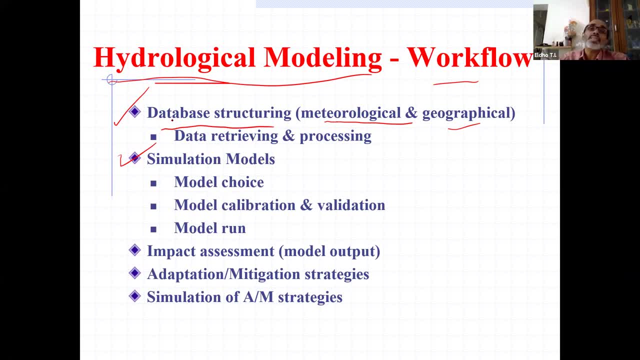 in the literature. so that way, if I talk on that, it will be hours and hours I can need to discuss about it. I will not go into that level, so, but what resources model, what is, what type of model? 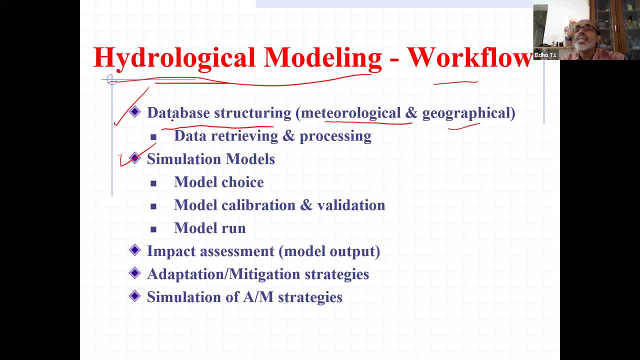 is required so that we need to decide. so that is this kind of training. when you are attending, you will be understanding, you can interact with experts and then understand for your specific problem what kind of the best model. 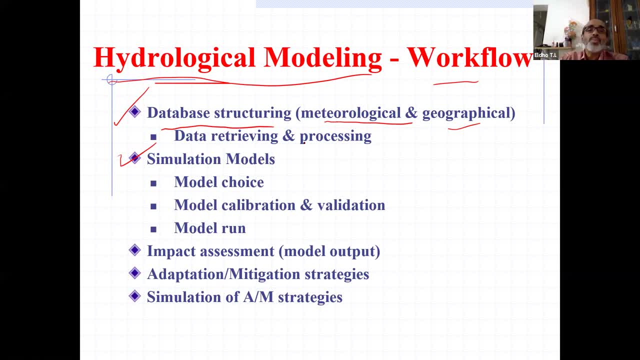 can utilize and how it can be utilized. so model choice is very important. and then, of course, as I mentioned, we are not dealing a building design, so building design is concerned. architect says: these are the. 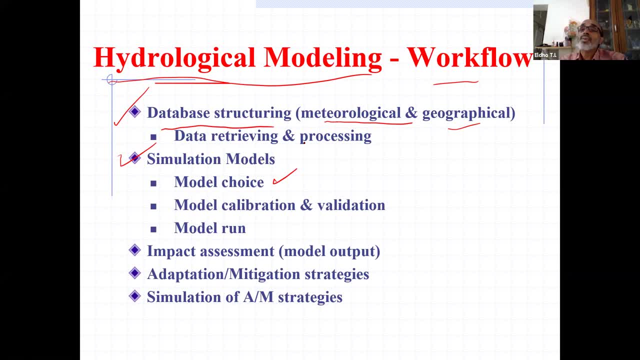 the. we know how much they're loading, loading or whatever they're loading. all those things are to certain extent we can totally predict in advance. but here you see that the nature is so complex. so you see that. 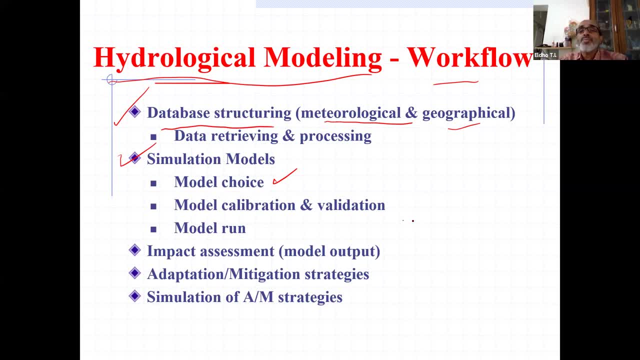 say, for example, hydraulic conductivity is concerned. so whenever I'm going from one foot and one say even 10 centimeter, 30 centimeter away, the hydraulic conductivity is so much variation you can see that everybody knows. 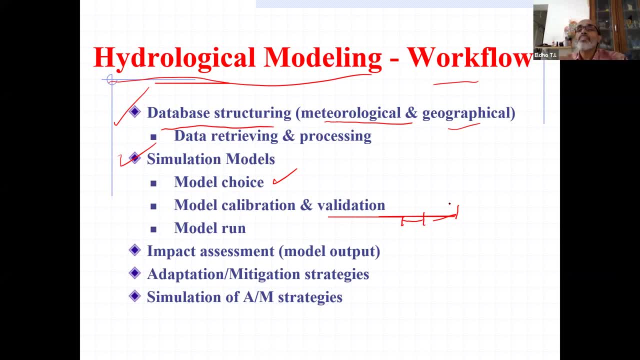 soil is not at all homogeneous, though maybe in some beaches the sand may be some somewhat homogeneous way it may appear, but most of the, the, the, the, the, the soil parameters. 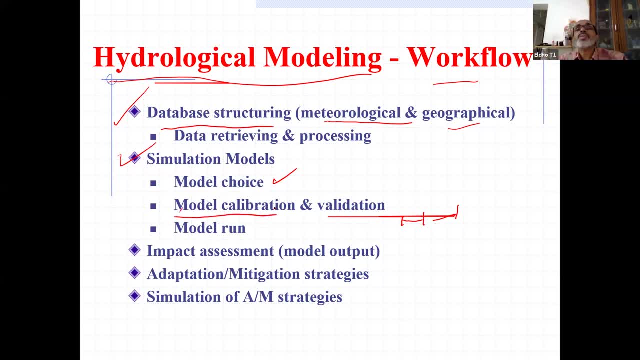 are so much varying. so that way, the with respect to available data, we need to go for model calibration. so many of the parameters we need to identify through model calibration and then we need to validate with respect to the. 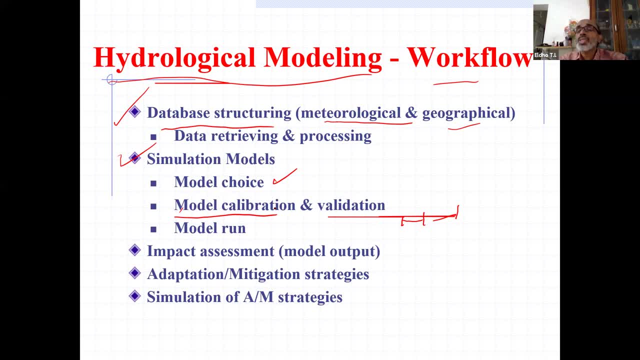 measured data and then, once it is done, we can identify the important parameters or any of the parameters which we are looking forward as far as the model is concerned, and then, after that is done, we can go for model runs. 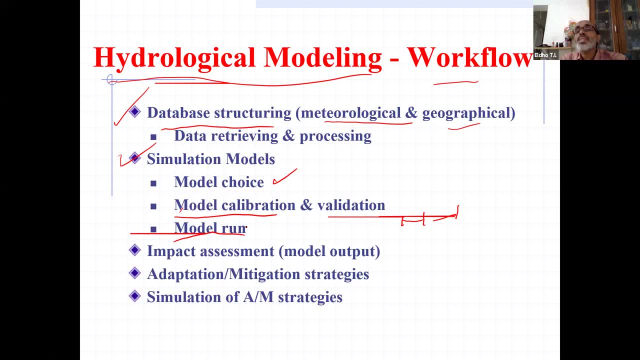 so the model runs means we create various scenarios- the best scenarios, the worst scenarios and then maybe normal scenarios- and based upon this we can come to certain conversions or recommendations saying that this is the best possible solution. 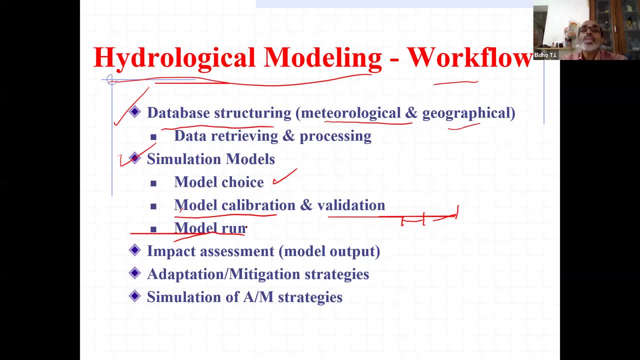 as far as this particular area is concerned. so, as I mentioned earlier, if you are going to develop a dam, and then you see that maximum rainfall concentration and then you see that maximum rainfall condition, how much water is available? 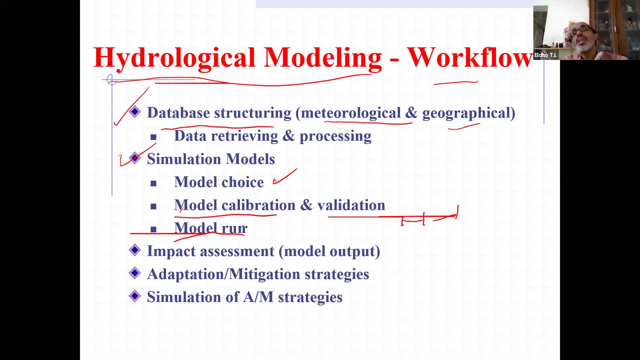 in that particular location. the worst condition- drought season- how much water is available? so accordingly we can design the structure and then its operation can be designed. so that is the way we do so, the various scenarios. 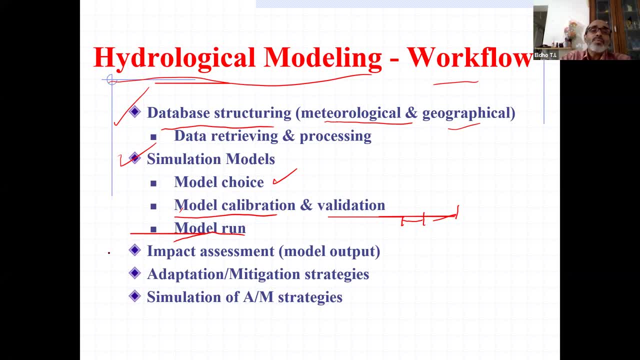 we generate and then, based upon that, we go for the impact assessment. so impact assessment means coming from the model outputs. so if the best rainfall condition is there, then what can happen? how much water is available for irrigation release? 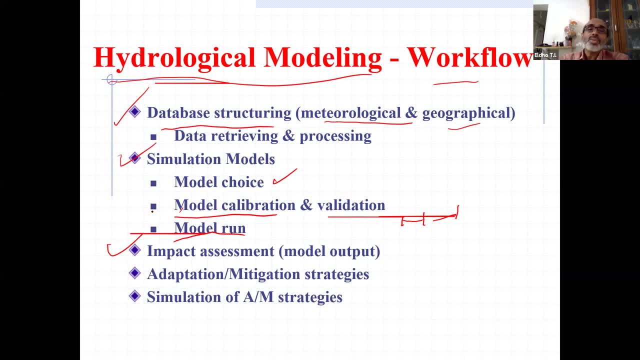 how much what is available for various needs. so that is based upon the model output we can design impact assessment and then, of course, adaptation and mitigation strategies. so once it is that scenario is implemented, what can happen? 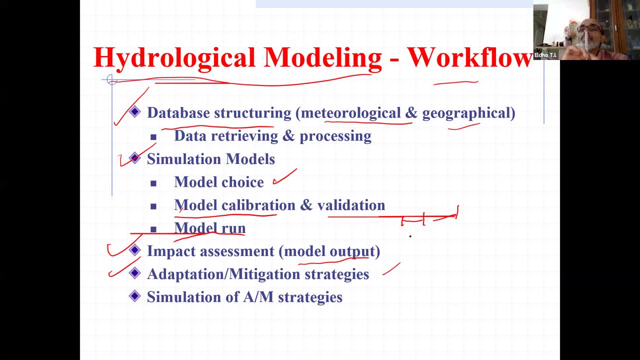 again, we can come back to the model and then see that how it is behaving and how the whatever we get we can observe in the water and that way we can do, and so that way the simulation. 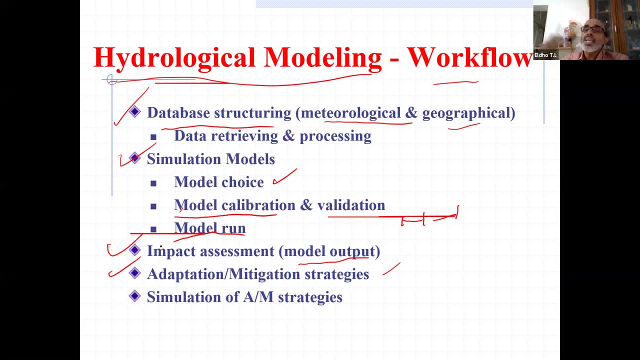 of adaptation and mitigation strategies can be further studied. so this is a process. so especially we used to train the water resource engineers in Maharashtra. I used to give training program earlier also, so that way I always tell that. 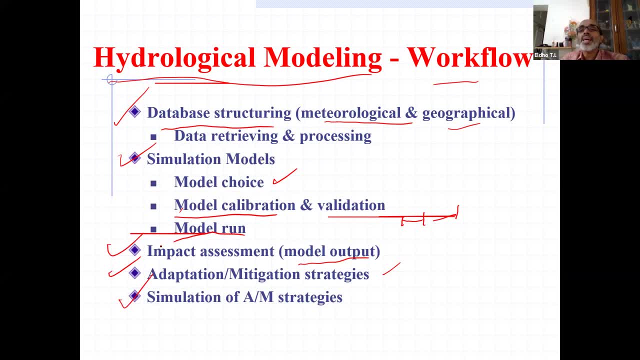 you are all controlling. as an executive engineer, you are controlling this particular area, so you need to see that. say it is not say one time a model is concerned. it is not simply developed and get some output. 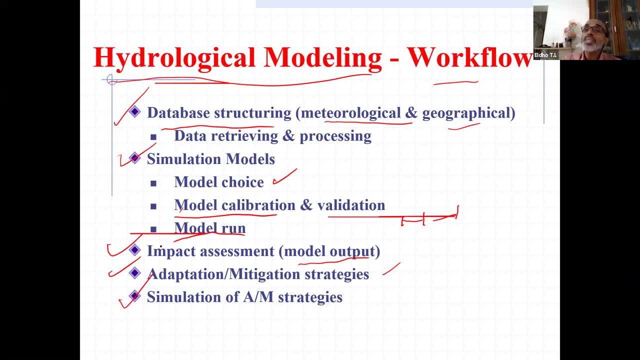 and then you are running away. no, we need to see that in a long time: how it is happening, how the behavior, how it is behaving and what kind of corrections are required as far as 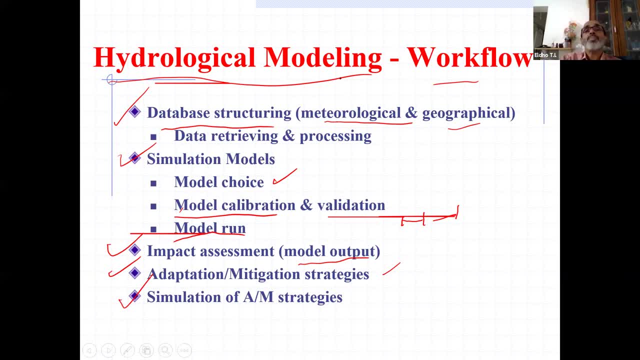 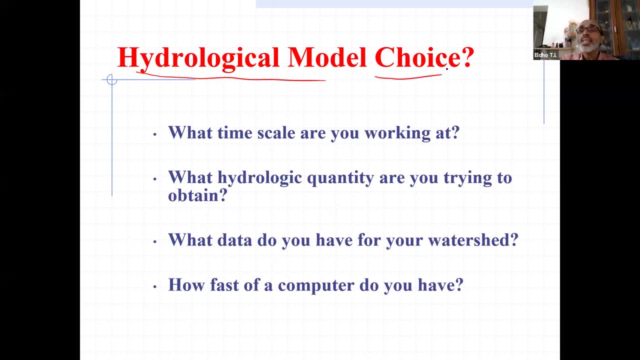 the modeling is concerned. so now the major topic of this training program is on hydrological model. so now the question is what kind of hydrological model we can? what are the choices as far as the hydrological modeling? 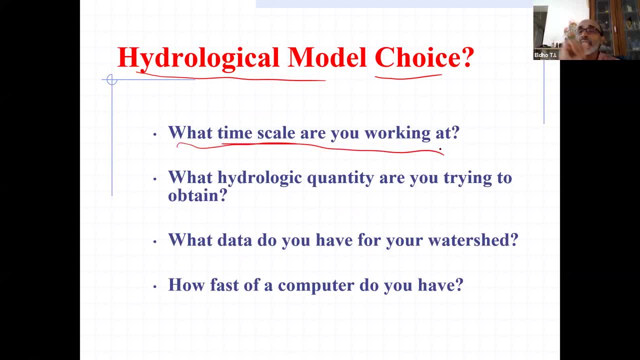 is concerned. so, as I mentioned, what time scale are you working at? so, to the students and the practitioners here, I would like to say: whenever, depending upon the needs, depending upon what kind of so we need to. 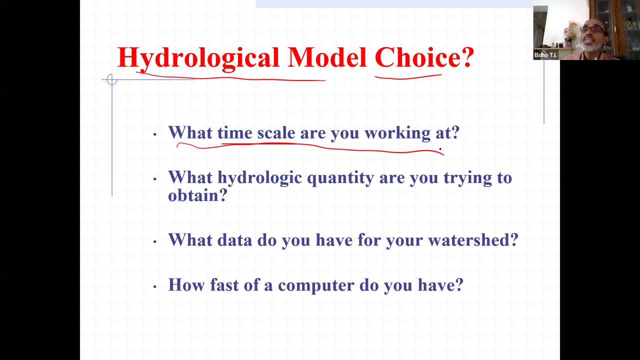 take a decision. this is your time scale, so it can be annual basis, it can be monthly basis, it can be weekly basis, it can be daily basis or it can be hourly basis. so, for example, 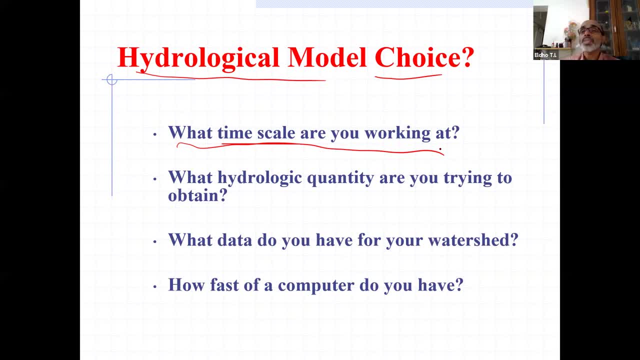 say, if you are going for a drought assessment. it can be even monthly or season variation can be captured, but you see that flooding, flooding is concerned even daily basis simulation is not enough, since 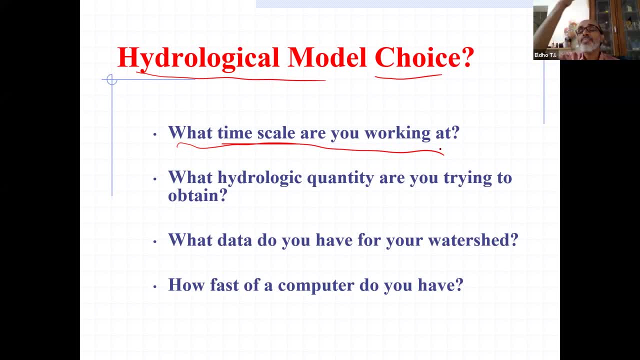 many times you are hearing how the, the, the flooding is rising or it is receding, so that all kinds of things are here. so that way, time scale is very, very important. so the students. 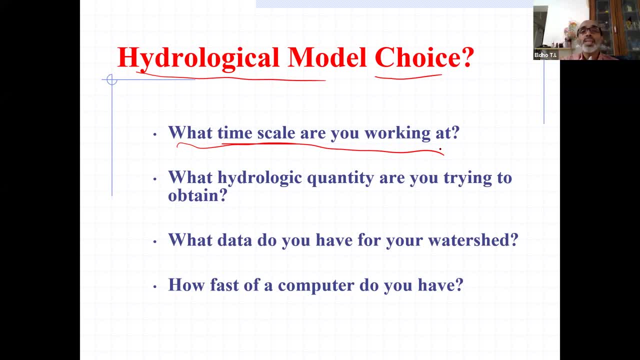 who are hearing from me, I would like to say you have to assess what kind of model you are developing and what is the time scale. so that is very, very important. and then the second aspect is the water. 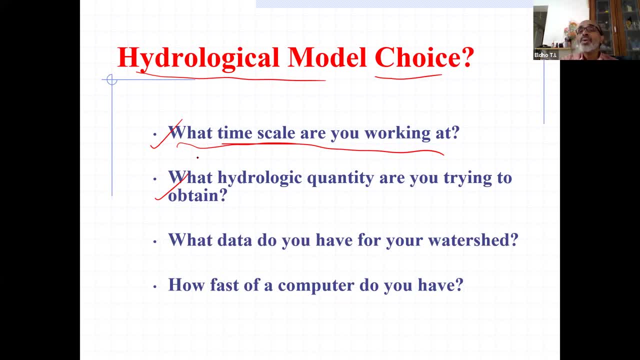 the? what hydrological quantity are you trying to obtain? so that is very, very important so much many times say. especially agriculture engineers are concerned, they need to also assess the soil moisture variations and then also. 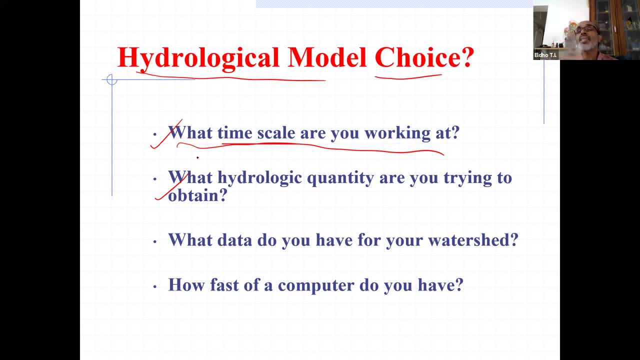 the groundwater variations we need to capture. so what kind of hydrological quantity you are doing? and then, of course, evapotranspiration is also very, very important. and then third aspect is: what data do you have? 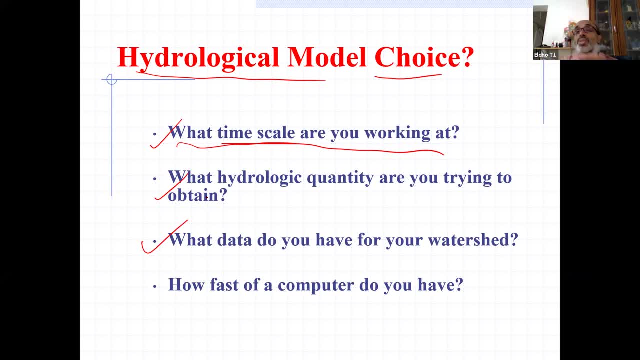 for your watershed. so, as I mentioned, if you put the young data, you get the young output. so your data should be accurate and what type of data you are having. so that is of course we are dealing. 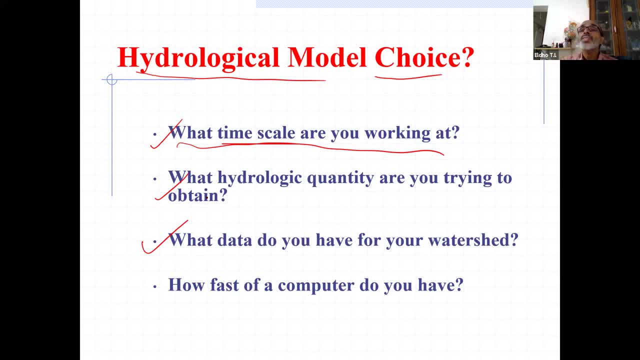 with the very serious kinds of modeling. so this model needs, say, some kinds of models, needs hours and hours or even days of simulation. so what, how fast is your computer? whether you are having on a simple PC. 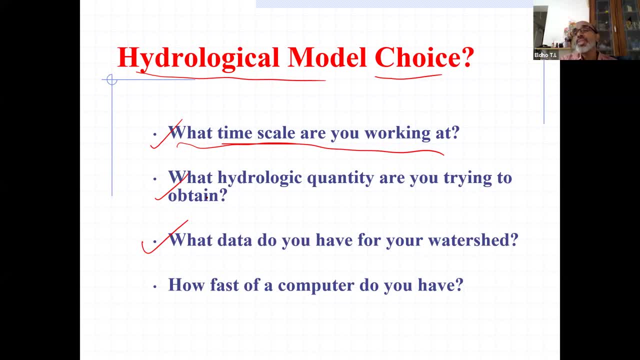 or you have, you are having, or sometimes, especially now, climate modeling, all those things are considered, we need even many times the supercomputers, so that that kind of you need to also before taking up. 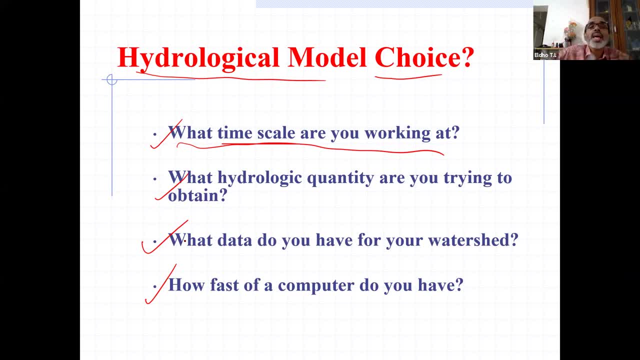 any particular study. we need to get look all these aspects so that the particular model which you are choosing we can take accordingly. and then comes, of course, as I already mentioned, thousands of models are available. 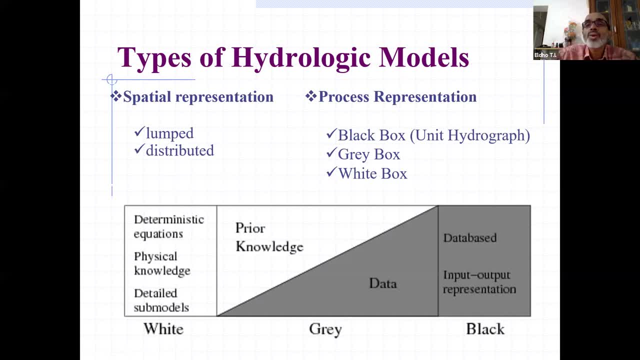 so those who are studying hydrology- you would have already looked in, studied about it. so we have got like a simple black box model. so we have like a simple unit hydrograph or even artificial neural network. 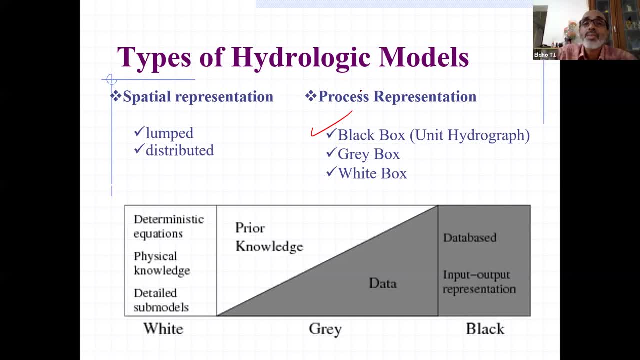 which is simply giving rainfall runoff, that kind of relationship. so we have a gray box, black box or a gray box means it is a between, in between. I mean say some parameters like mass balance. 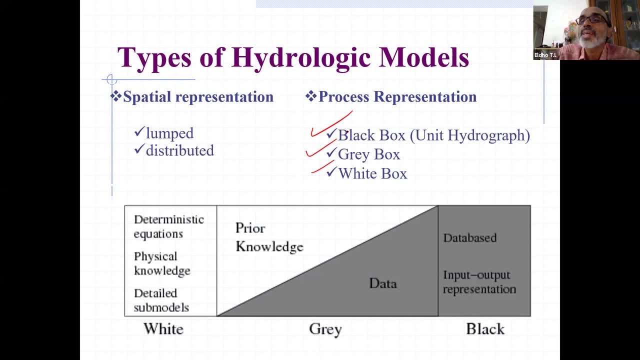 all will be taken care. and then white box means it is directly all the aspects, like a, say, distributed model where we consider the conservation of mass, conservation of momentum. all those aspects will be considered and then 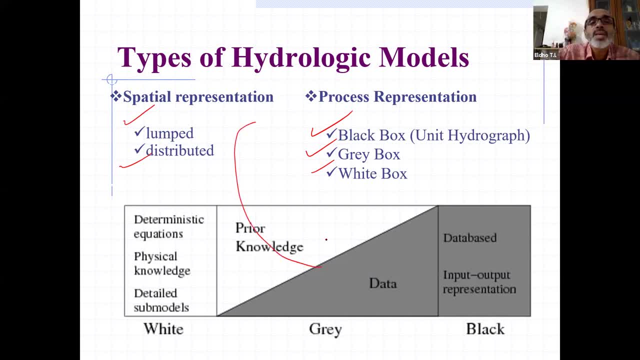 also, the modeling can be lumped or distributed. so lumped means say so, this is a thousand square kilometer area, and then we say that okay, we consider only one land use, one land use or one soil parameter. 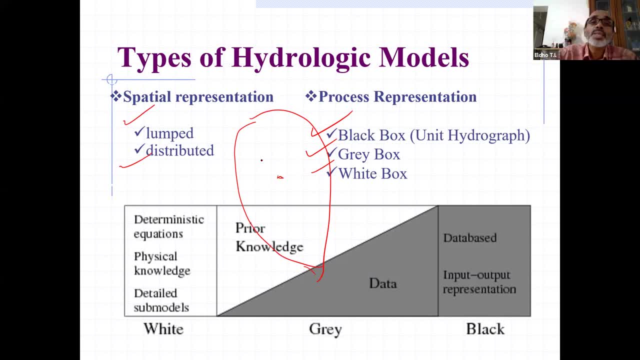 or that kind of lumping. all the parameters is lumped for that particular area or a sonar wise. we can lump it like that: various zones, you can put it, and then these are the parameters. so that is called. 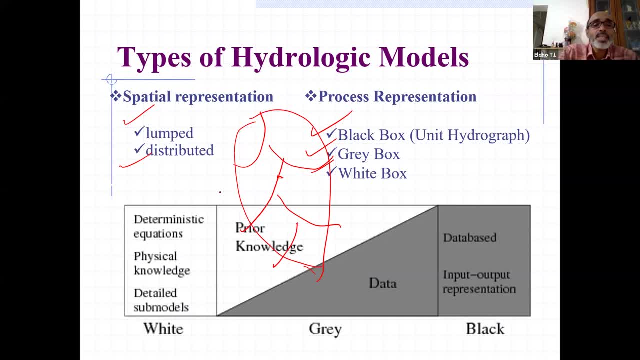 lumped models, and then, of course, you see that this, as I already mentioned, we are having the white kind of model, physical knowledge, everything is available, and then gray is in between. some are 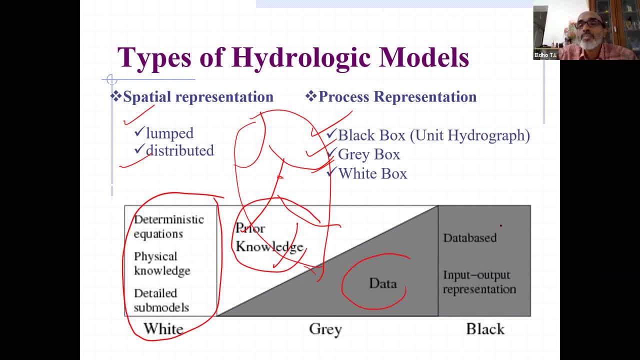 some of the things are prior knowledge and some is based upon data. and then black box model means simply based upon data, like artificial network. simply, if you have got thousands of data points, based upon that, we are getting. 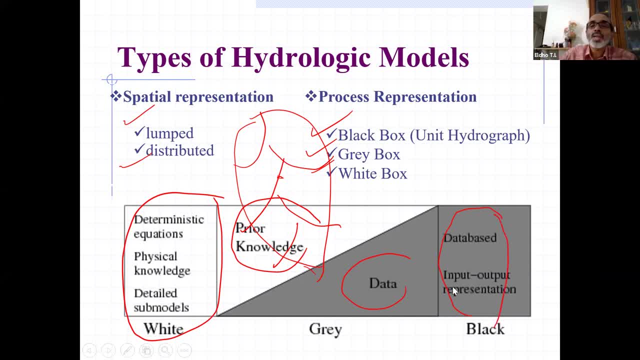 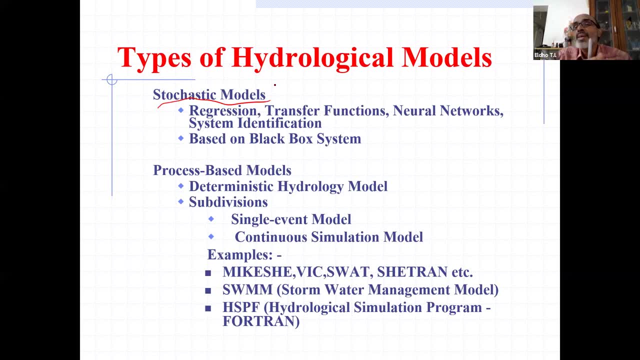 an input output relationships, so that way the types of hydrological models are classified and then also we can have stochastic model. you can see that many times the rainfall prediction surface. various aspects of stochasticity. 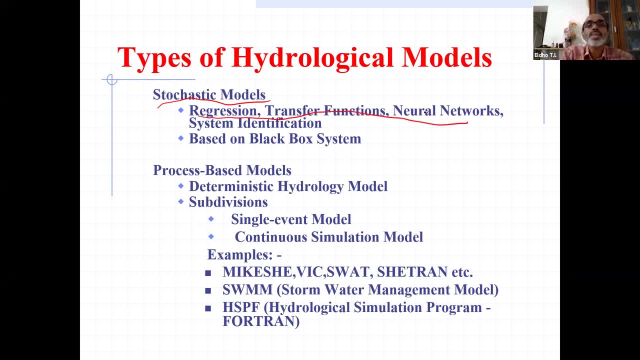 and then regression transfer function. all those things will be coming to picture. and then of course we go for process-based model. so like a deterministic hydrological model, subduction, single event or continuous simulation model, 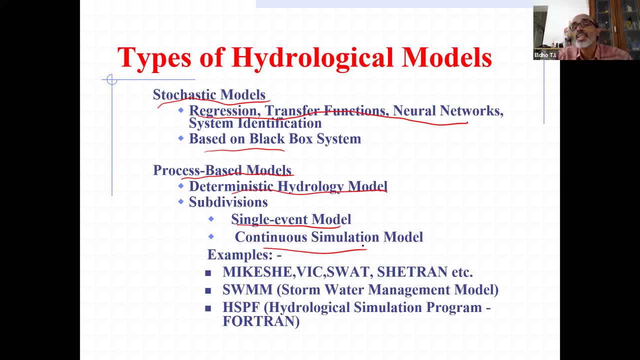 or depending upon the needs. so, for example, if you are going for a prep simulation, it can be even single event based model. or if you are going for water source, agricultural aspect is concerned, we can go for. 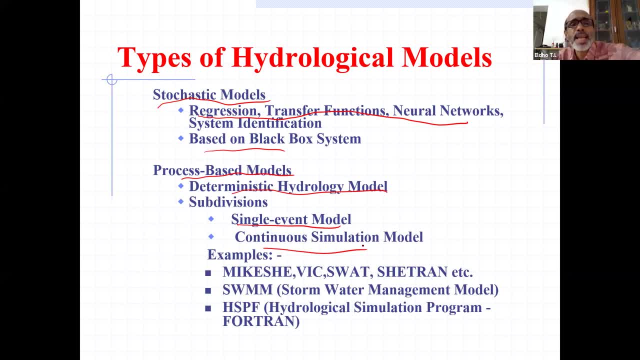 continuous simulation. so here some of the examples, like Mike Shee, Swatch, Sheep Can, et cetera. these are all somewhat. Mike Shee is fully a distributed model. Sheep Can is also a distributed model. 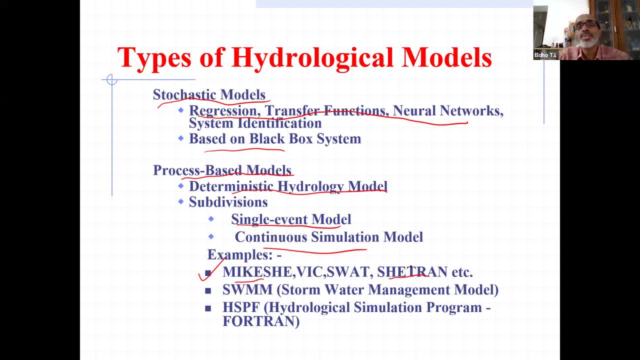 Swatch is a- you can see in between, since some of the parameters we lump, and I understand that there is a Swatch training also in these five days of international training and then, like storm water management model. 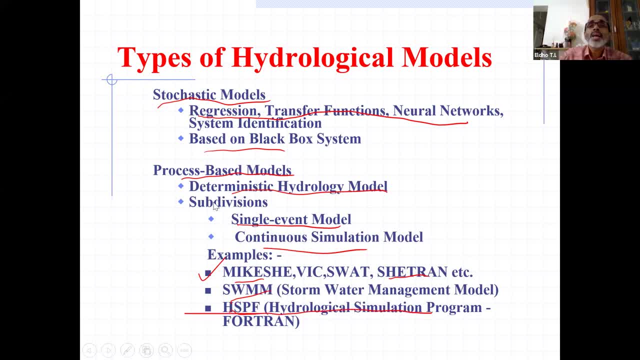 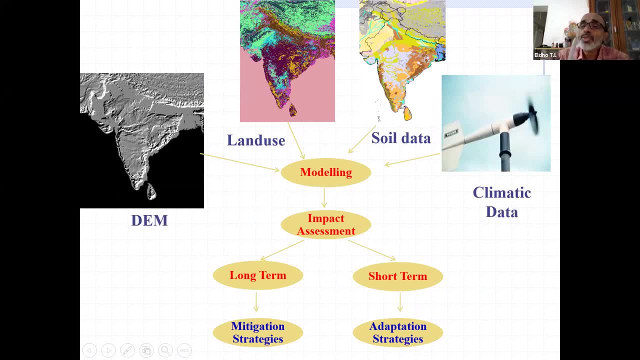 then HSPF, like hydraulic simulation program. so there are so many models are available in the literature, the needs. we can choose particular model and some of the models have open source. I mean directly. 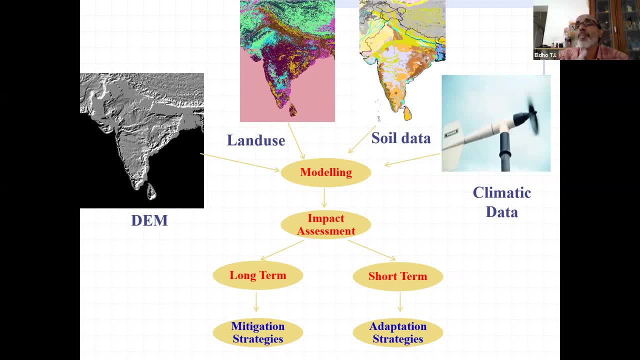 you can like Swatch to VIC very, very inflection capacity models. so these are directly open source model and which you can download and then work with, but some of the more like Mike models. these are: 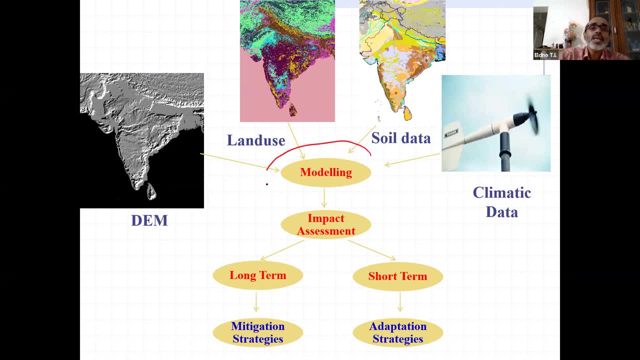 we said we are paid model, we need to buy the model and then, of course, as I mentioned, modeling is concerned, so the geographical features will be coming, and then the land use we need to look into. 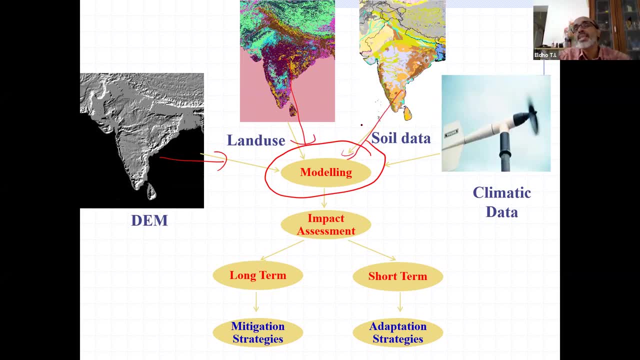 and then soil data. so you see that India is concerned. at Magpur we are having national bureau of soils. the center is there, so from there you can get the soil data and then climate parameters. 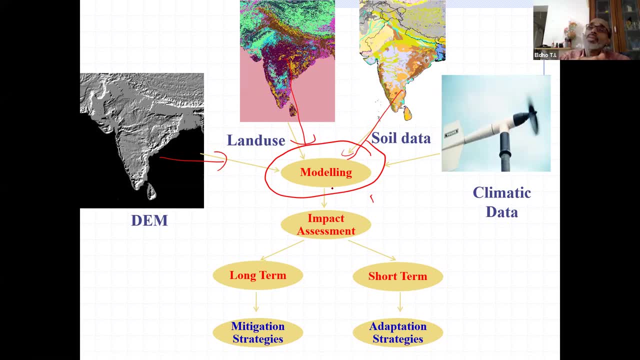 all we can get it, and then everything will be put into a model and then we, as I mentioned already, we can go for various scenarios: generation. so, as I already mentioned, whenever we look into these kinds of problem, 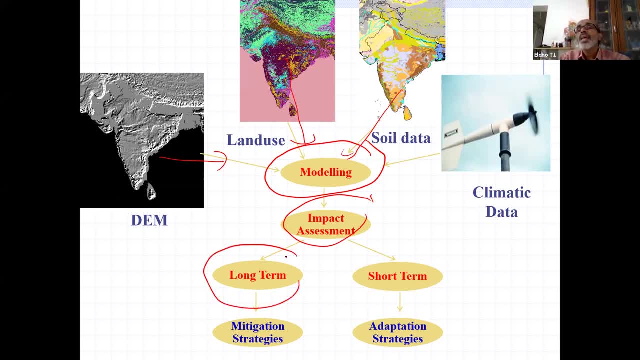 whether it is, we are going for long-term simulation. so, like many months or even years, say, for example, in climate change projections are concerned, we run the model up to even 2100,. I will be presenting: 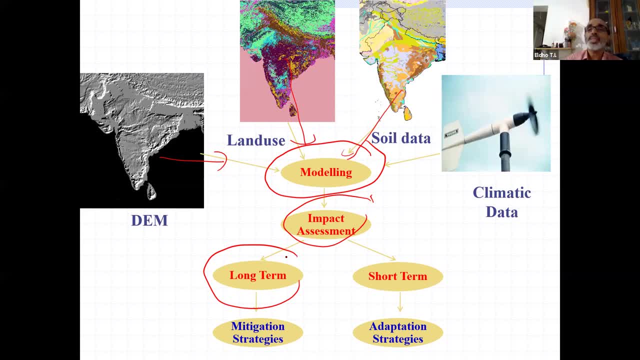 some results here using SWAT or other kinds of models. so we do very long simulation and the short-term means you say, especially flood assessment is concerned and we can. we'll be running the model for a few hours. 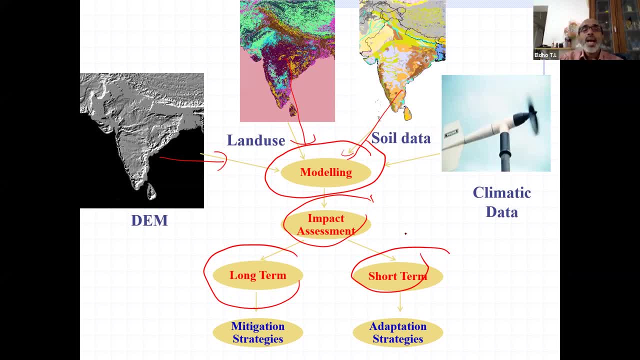 we'll be looking for the, the, the impacts, and so, long-term is concerned, what kind of materials and strategies we can look into and, short-term, what are the adaptation, immediate adaptation strategies we need to? 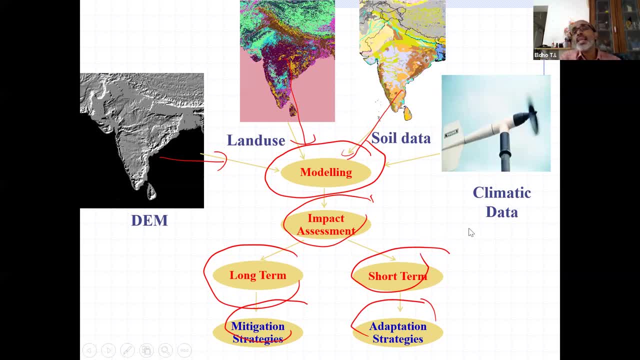 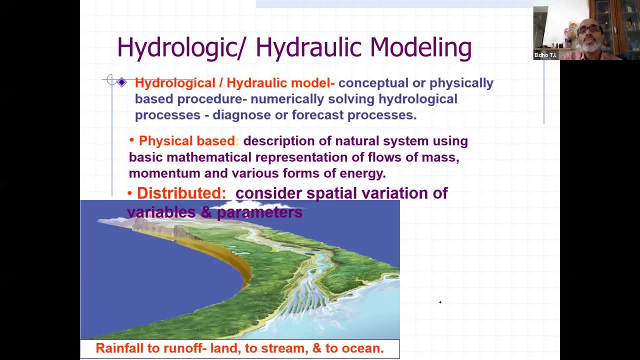 look into. so that way we'll be looking. and then again coming back to the hydrological and hydraulic models. the hydrological model means, of course, you see that say, for example, this is here: 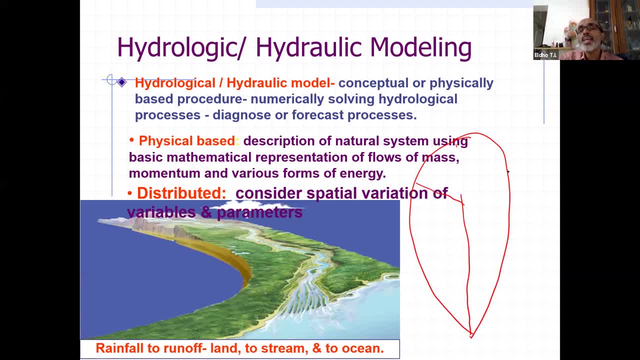 watershed and then a network is there, so you can see that various small, small drains will be joining here and then it will be routing. so this, whatever is happening on the overland. so 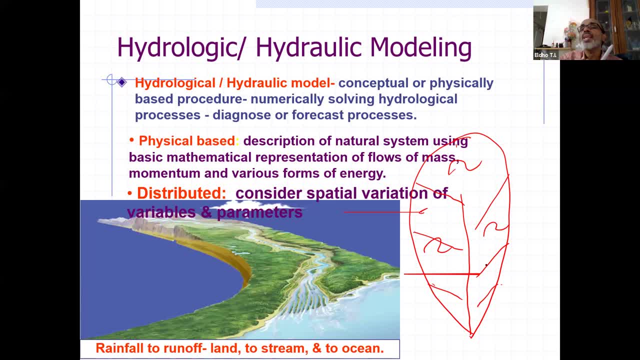 here. these are this area are called overland area. so in this overland area, how much is the rainfall and population? we call this hydrological modeling and then hydraulic means. so here we have. 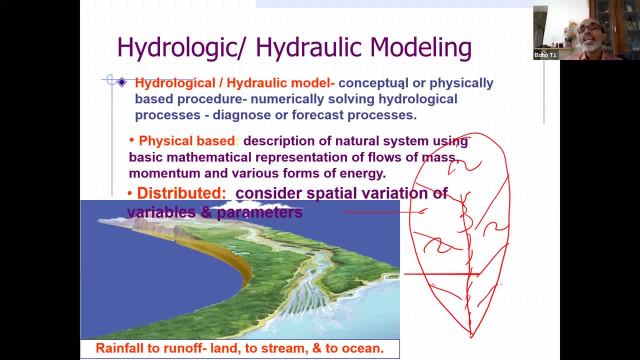 all these different concepts of physically based distributed, physically based procedure we can adopt and especially physically based means we need to solve partial equations, so we need to go for the numerical methods. so physically based description. 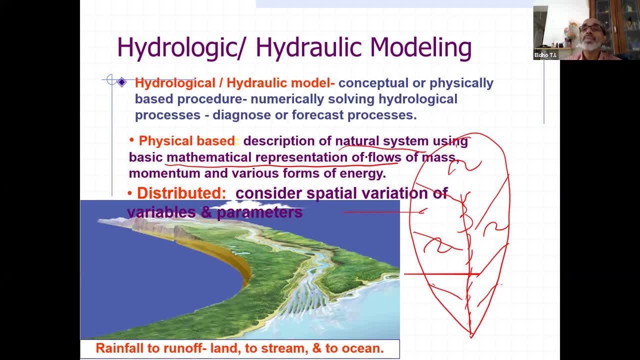 of natural system using basic mathematical representation, like your many of all. of you know that we use saying we had equations. so that is the distributed model, consents in the variables. and now here, this is the river passing and then you can see that radius and the overland, the 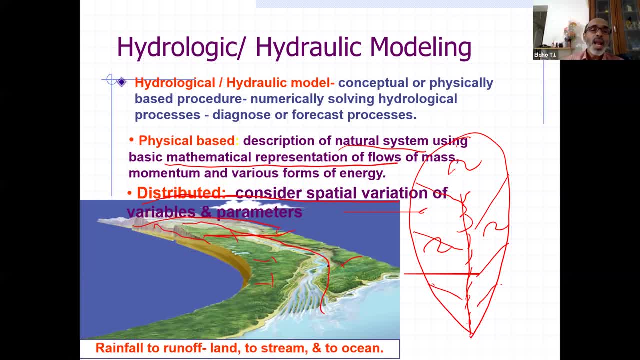 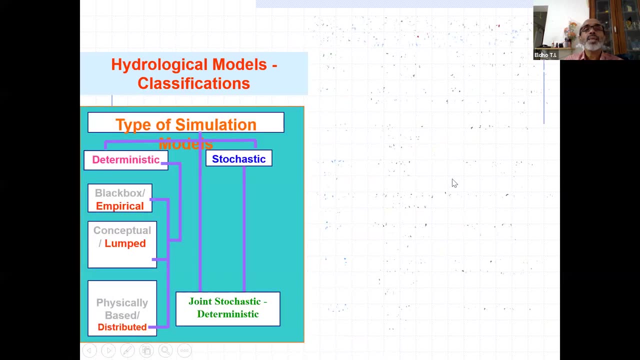 component will be coming, and then we need to route through each and finally rainfall runoff, so land to stream and finally to ocean. so that way, the hydrological modeling is to be done, and then routing is to be done, or hydraulic modeling is also important. so now, that way, now, as i mentioned, 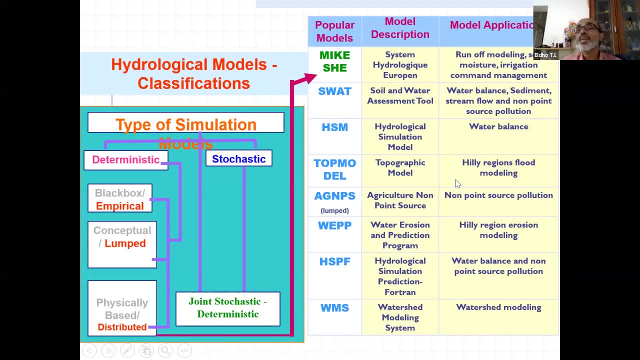 earlier and we are having a number of variety of models are available. so depending upon the objectives of your study you need to choose particular model, particular kind of systems and so that way type of simulations again in the product. i have book here. so here, between this big model or forecasting model, then models are considered kind of black box or empirical. 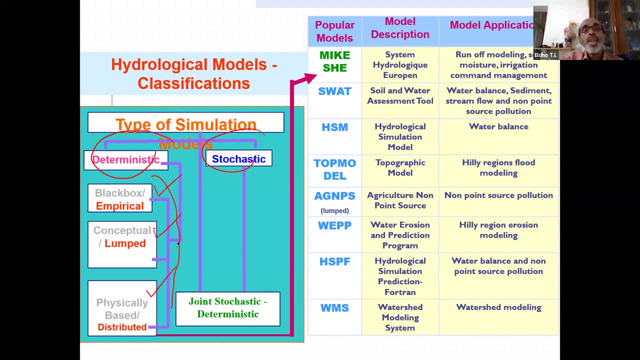 models, or conceptual lumber model or physically distributed model, and then what type of model? and then a variety of models. you can see, as i mentioned, like a mainstream model which gives uh runoff modeling of soil, moisture irrigation, all those things. we can use it, and that is a somewhat a paid model. i mean the the uh uh mike models, and then swat model soil water. 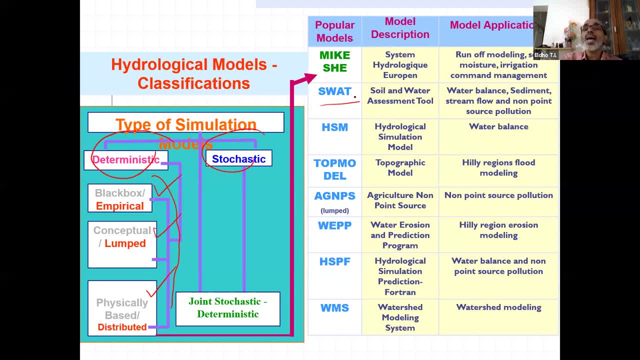 assessment tool- so this is a freeware- so where water balance and then stream flow and all the parameters can be obtained, and then hydraulic simulation models you can see here and then top of model agnps, web model, hsps and watershed modeling system. so, like that number of 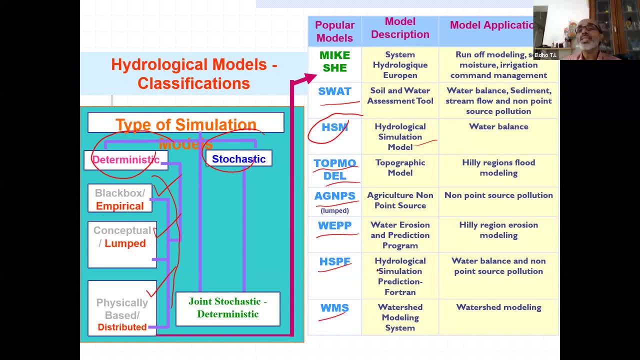 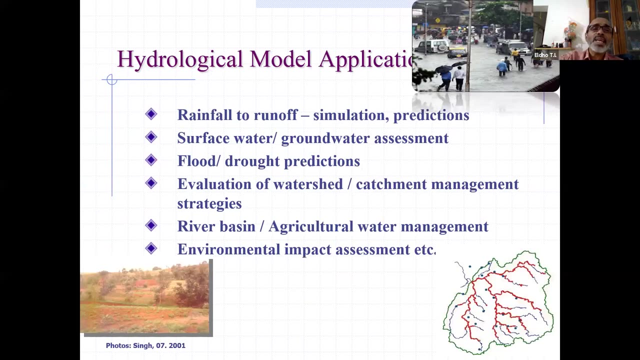 paid or open sources are available. so, depending upon the needs, uh, you can choose particular model and then go for the, the, the particular, depending upon your objectives and depending upon the data available, you can go for the particular model and then coming back to the hydraulic model applications. so so far, we are discussing so many aspects of hydrological modeling. so from this you 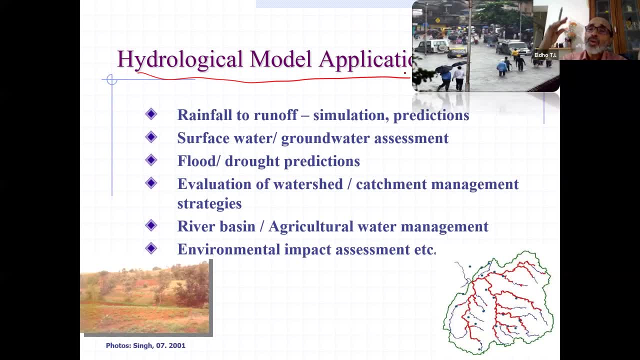 can see that, uh, say you already, we have already discussed all these. so what kind of applications are there? so many applications are there. so, as i only mentioned, rainfall to run off. so assimilation predictions we can do using the hydraulic model and then we can go for surface water, groundwater assessment. 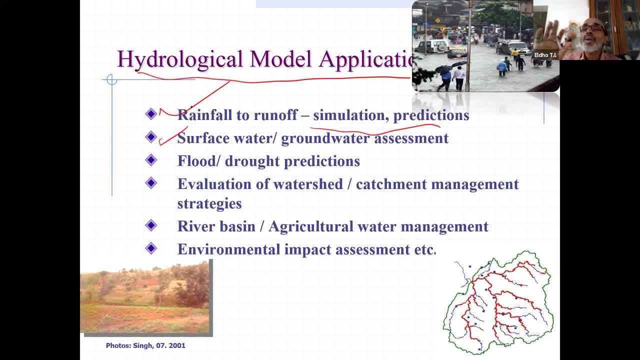 so for a on a river basin scale, on a watershed scale, how much water is available? or annual basis, and then we can say that, yes, this much is the water available and this is the utilization and this is so for this much uses. we need to work for storage or a check down or what kind of development. 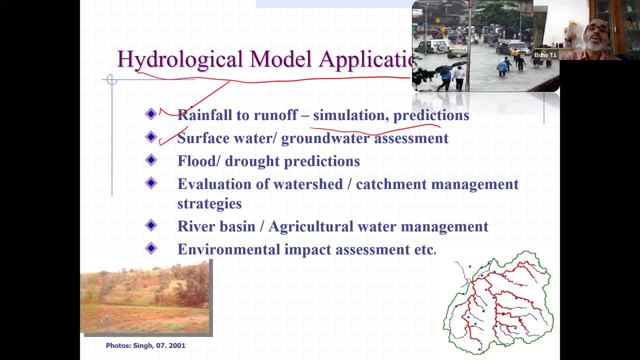 is required, or rainwater harbour, so we can go for the hydraulic model, so we can use the hydraulic model for the harvesting measures to be done, and then, of course, we can go for groundwater assessments and then, as i already mentioned, the hydraulic model we can use for the flood simulation, or 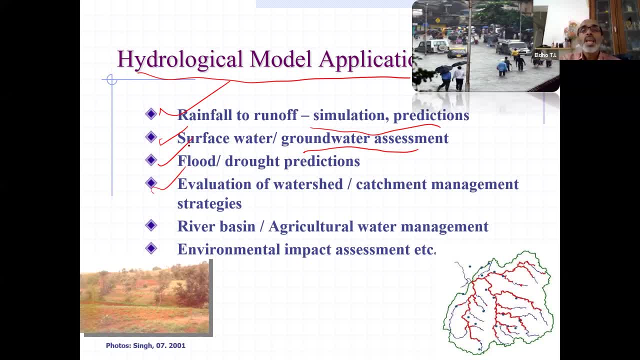 drought predictions, and then we can also use it for evaluation, watershed or catchment management strategies, and then we can go for river basin agriculture, water management. so river basin scale. so what kind of farming is there, agricultural practices are there? so accordingly, we can- uh, you look into. 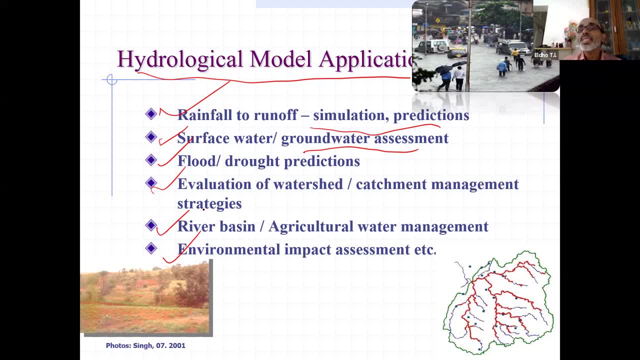 all of these things, and then we can go for the hydraulic model. and then, of course, whenever we are developing a large scale investment, like a larger dam is we are constructing, then we need to see environment impact assessment. so, with respect to hydrological parameters- uh, what kind of uh? 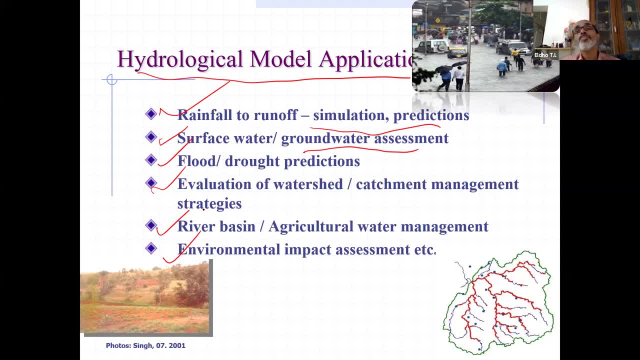 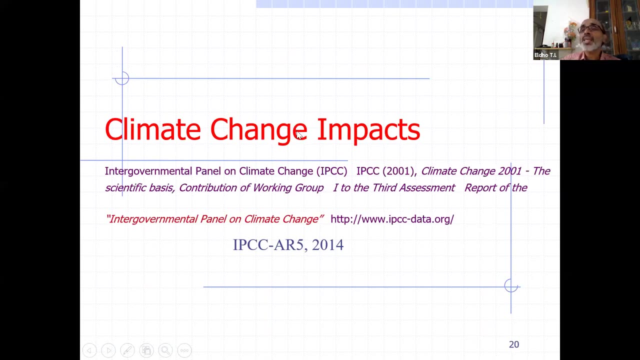 assessing that can take space, how much area we affected and what kind of flooding can take space. all those things, uh, we, we need to be the support of the, the hydrological model. so, uh, that way, uh, you, all these aspects. so this was the first part of my lecture, where the hydrological models we discussed. 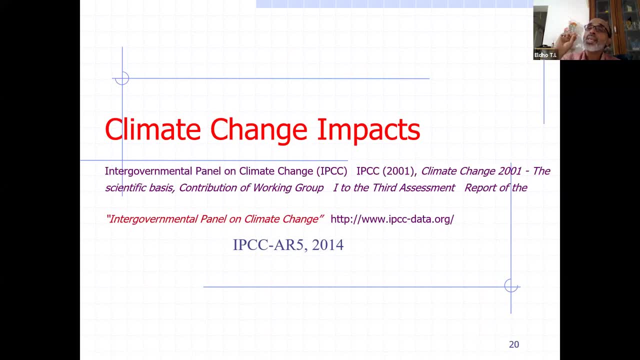 so so far we discussed why hydrological model is required, what are the importance of hydrological models, and then how we develop a model, and then what kind of models are available and, uh, what are the applications. so that was the first part of my lecture and now second part is uh. so, as i mentioned, 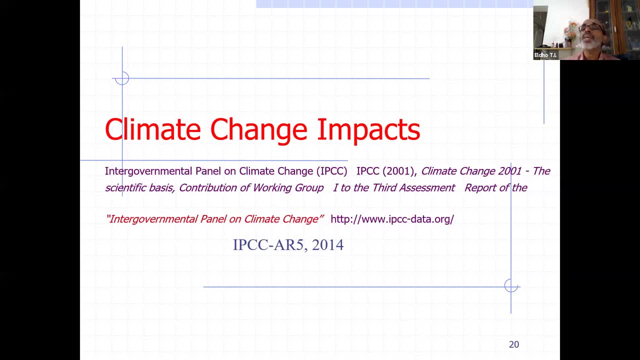 now the most important aspect is the climate change, what is happening, and then, with respect to climate change, what will be the impacts? of course, here also, as i already mentioned, the hydraulic models are required, so we'll be discussing how we can utilize the hydraulic models are concerned. 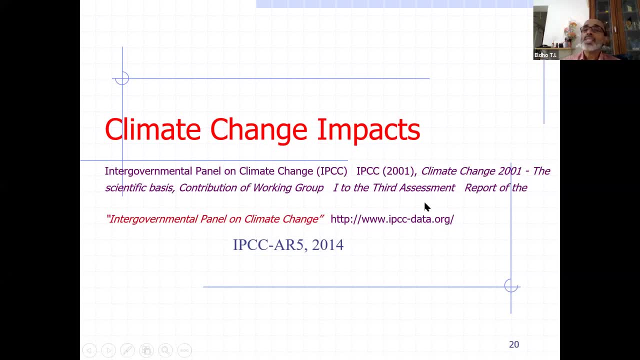 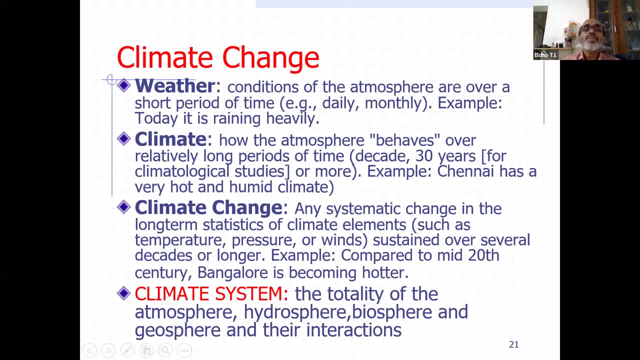 how we can utilize for the, the impact assessment, especially had all these concerns. so climate change, the time, so um, all of you heard about the height climate change and many of you may be working in this area. so climate change. so whenever climate is concerned, we put the two. 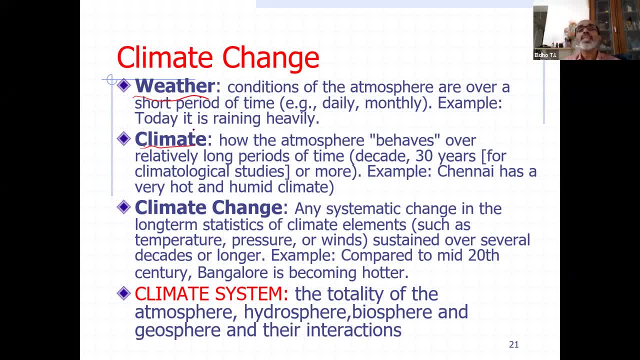 times one is available. the weather second is the climate. so weather means what is happening, the conditions of the atmosphere over a short period, like a daily basis, so the today it may rain or tomorrow it will be sunny, so like that when we call it a city's weather. so that is not the climate is concerned. 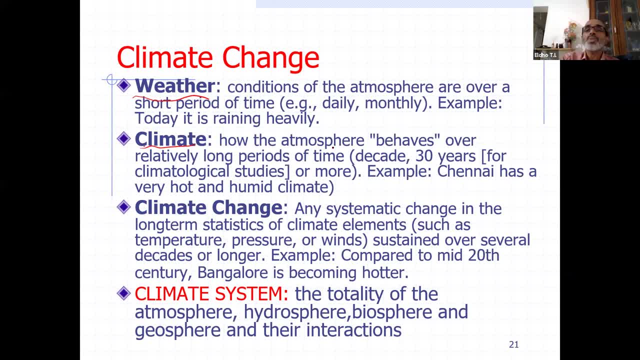 so when the terms of climate is concerned and how the atmosphere behaves over a long period of time, like two decades or three decades of time, how the variations take place. now chennai is very hot and humid nowadays, so that is based upon we can assess for last 30 years of data, or bangalore. 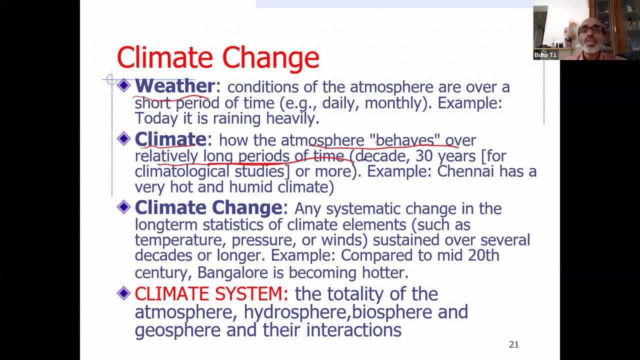 a few years back. now it is becoming hot, so that kind of variations we can say that is called a climate climatic variation. so then the change means climate change, any systematic change in the long-term statistics of the climate elements such as temperature, pressure or winds sustained. 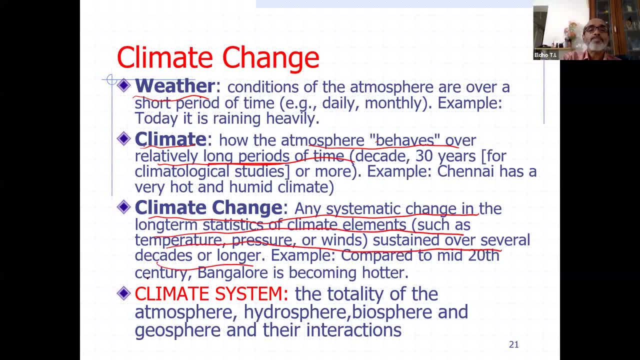 over several decades or longer. so then we say that is climate change. so what is weather, what is the climate and what is climate change? so that way, we need to look into so why we are discussing this. this hydrology is concerned, it is very much affected due to the climate change, so that is. 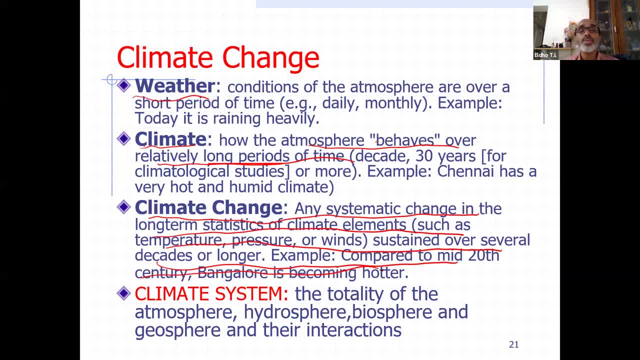 already grown and then so much of our assessments also show that. so that is why we need to look into what is climate and how the changes as far as climate is concerned, how it is affecting the ideology. so now, climate system. as you see that whenever we talk about, climate change is concerned, 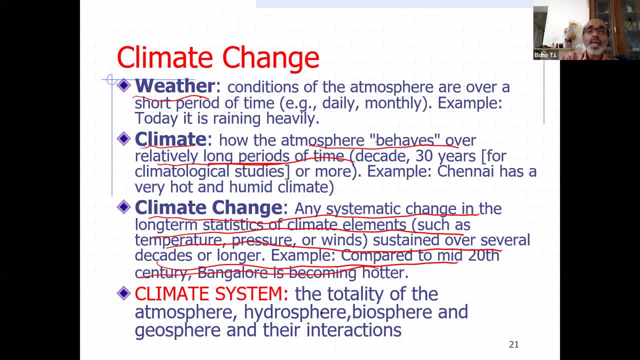 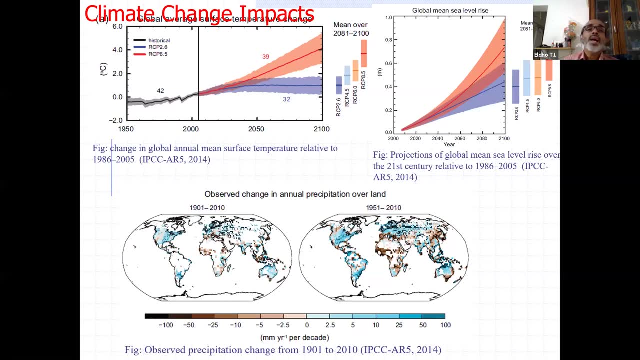 we need to talk about the climate system, the totality of the atmosphere, atmosphere, biosphere, all those things we need to look into. and then, of course, now we are having a very sophisticated model like the gcm- global circulation model, or general circulation models- are available so that we can definitely utilize it. and now coming back to climate, so climate change impacts. 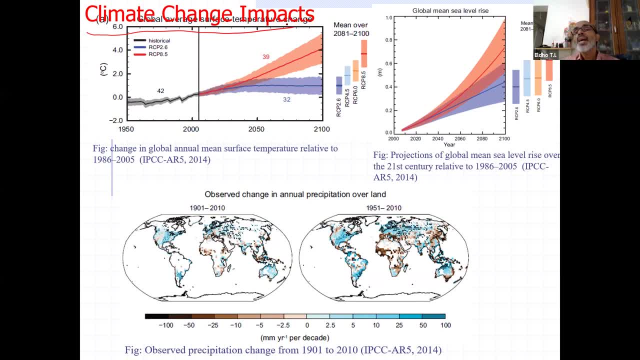 so you see that. then say the temperature: so this is all. so last hundred years of data, ipcc has all already analyzed. and then they come with these kinds of charts. so if you compare startup on 1950s, you can see that the temperature there is a uh, so a change, the rise is taking place, and then you can. 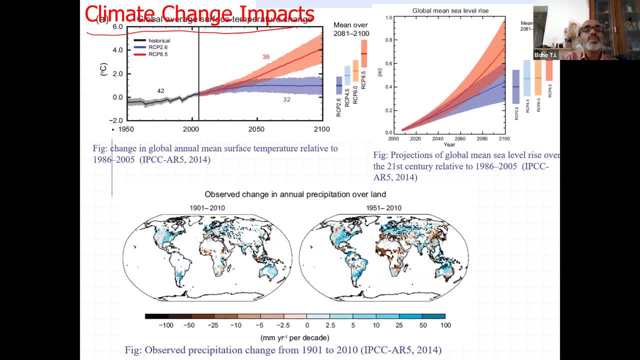 see that if it is currently 2020, you see that with respect to 1950, uh, there is a almost same two degree centigrade changes. it can take place. and then now, when you are projecting to 2100, so ipcc has come with the radio scenario like: 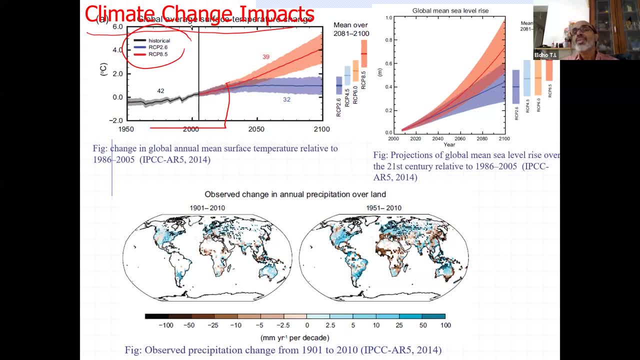 the same kind of pattern is taking place. what is the situation? uh, so generally called just rcp 4.5, and whether, if you can stop the, the, the greenhouse gases, or the, the rise of temperature can be, then i just generally call it just rcp 2.6 and rcp 8.5. it is: keep on increasing the, the carbon emissions. 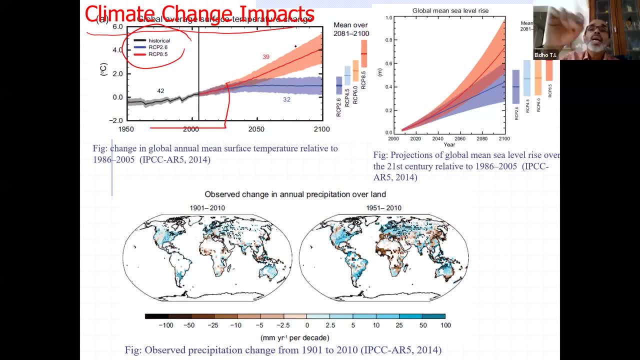 keep on increasing, then these red line shows. so that way we will be projecting what can happen in future. and so that is as far as the ipcc norms are concerned. and then of course you see that whenever the the temperature is rising, then of course there is: 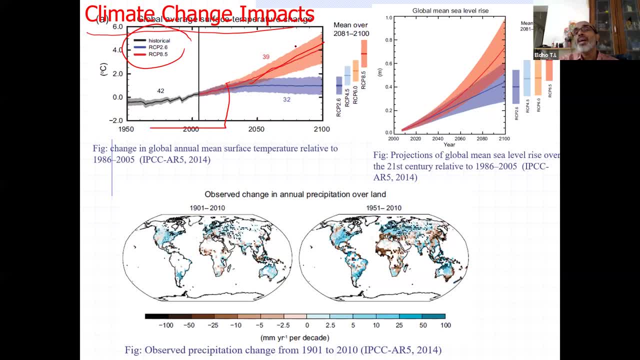 a means level resource. you can see that is also well proven by measurements for the last hundreds of years. so you can see that now, if it is 2020, what is the situation? uh, here, uh, so, now, uh, so, so, if you're not on the condition, so there is a slow raise. you can see, um, you know, various 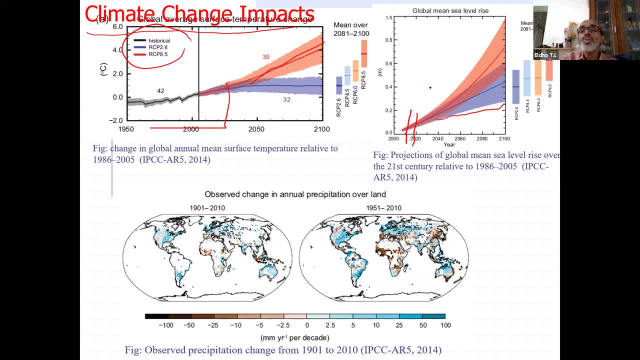 scenarios. so that way, uh, what is the impact of climate change on ocean is concerned? a global means see. and then here also, this shows the observed precipitation changes from 1901 to 2010. as far as ipcc 2014, you can see observed changes: annual precipitation over lunch. so even this is that. 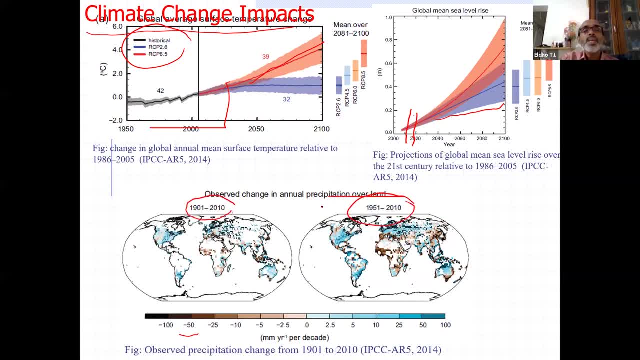 1901 to 2010 and 1951 to i mean 100 years changed and the last 50 years of change with respect to 2010- how the changes are taking place. so that way, when we look into, we can see that the climate is. 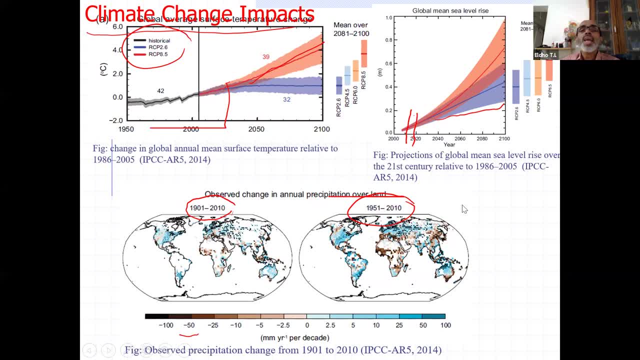 changing and then that is the, the, the, the after effect is, as i mentioned, the hydrology is the most the vulnerable system as far as the climate change impacts are concerned, since the everything they want the rainfall to run up of the hydraulic cycle is concerned, it is depend 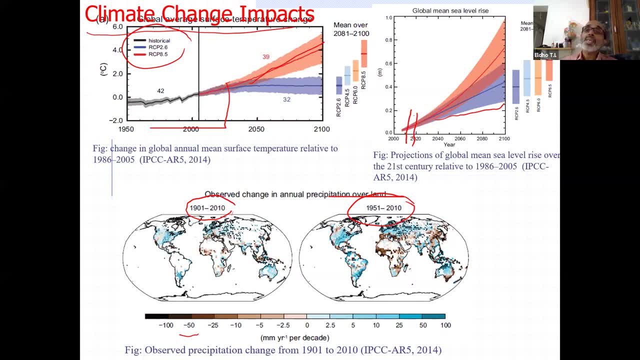 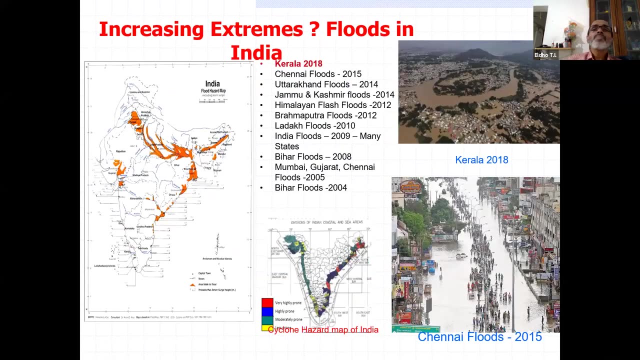 upon the temperature, or it depends upon the, this type of carbon emissions, and then you can see that the evaporation can change, evapotranspiration can change the little temperature variation, and then the the rainfall pattern can change and all over, all over, the system can change. so now, um, you may ask whether actually say even still. 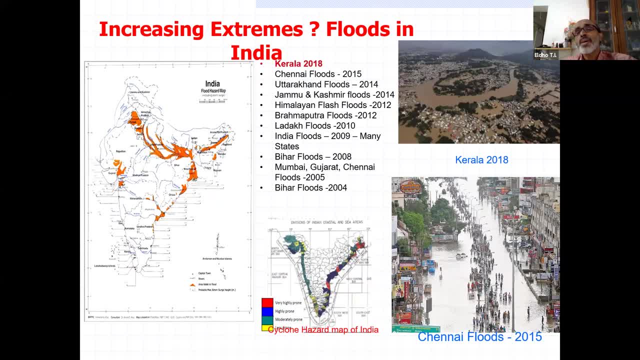 some of the scientists or some of the decision makers, or some politicians or some of the people are still skeptic whether climate change is really happening. but whenever we look into in terms of hydrology, when we look into indian situation for the last 20 or 30 years, we can see a series of events taking place. 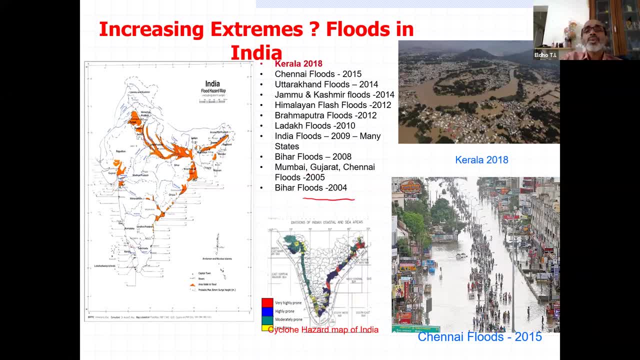 so, starting from- and we have 2004 funding to 2005, number of flooding: where i was, i was in mumbai in 2005 and when my family was affected in 2005 flooding, and then we have 2000. so, like that, you can see a series of events taking place and latest. 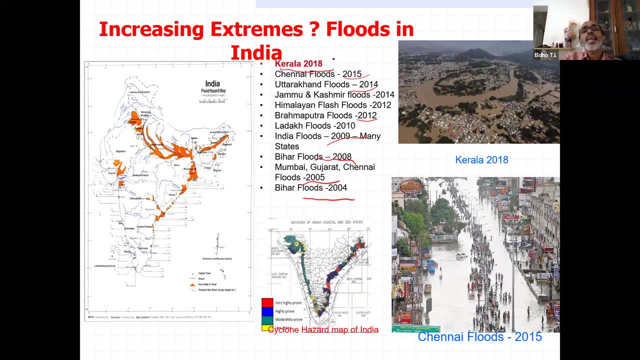 severe fund was happening in 2018, uh in kerala and chennai 2015, and then, though it was not severe, last year also, there were issues of the uh, these kinds of flooding events. so the so that way, and the the extremes. so that is one of the major aspects of climate change. what 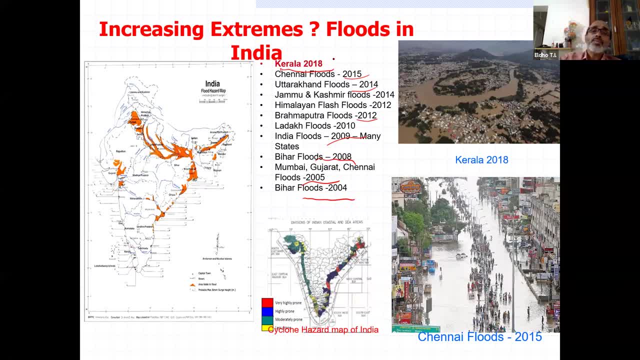 is observed, so the extremes are increasing, uh, so you can see some of the pictures here. uh, and then also post is concerned. you can see that that is every year and many kinds of, even many events of cyclones are taking place. so cyclone means severe rainfall and again flooding. all those things can 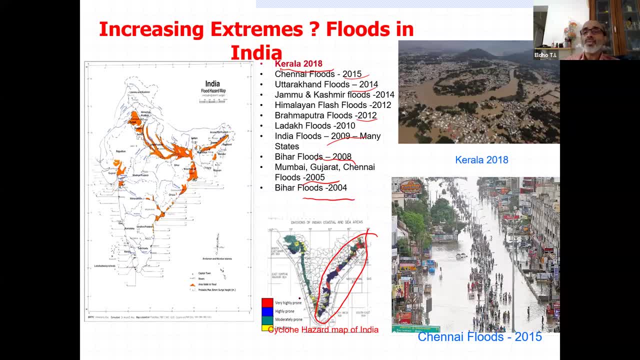 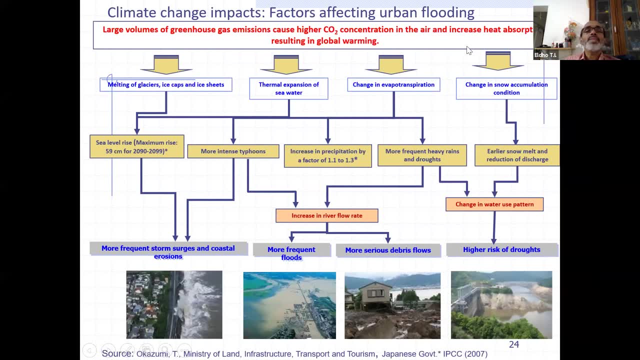 happen and then also, uh, even, uh, western cost also. you can see these kinds of problems. so now coming back to these kinds of issues, so climate change impacts, factors affecting the say, for example, cutting, is concerned. so you can see that now large volumes of greenhouse gas emitted and then it's after. 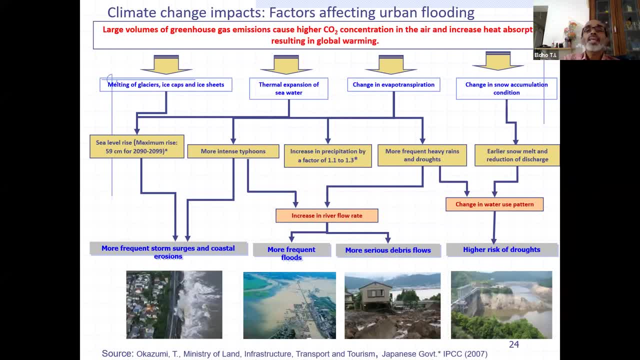 impacts is on the temperature raise and then the the climate change that we have already seen, and then, uh, one impact can be melting of lucy is then thermal expansion, sea water changing, evapotranspiration changing, snow, melt, all those things, and then, as we already seen, there is sea level, uh, rise is observed, then, uh, most of the 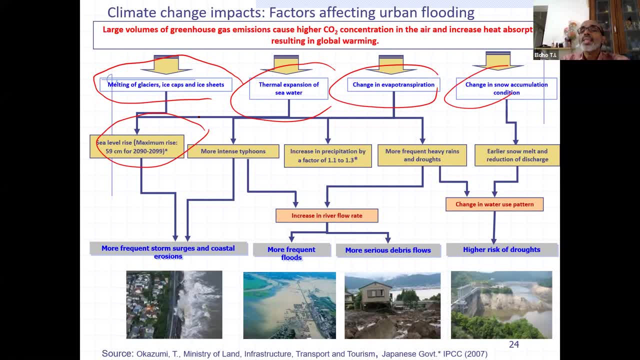 predictions so shown that more intense um, like typhoons or cyclones, are keep on increasing. and then many places the projections show that, or the the total rainfall variation shows that there is a precipitation is increased by one point one to one point. three factor and more frequent heavy rains. you see that. then of course you may ask that so much rain is there. 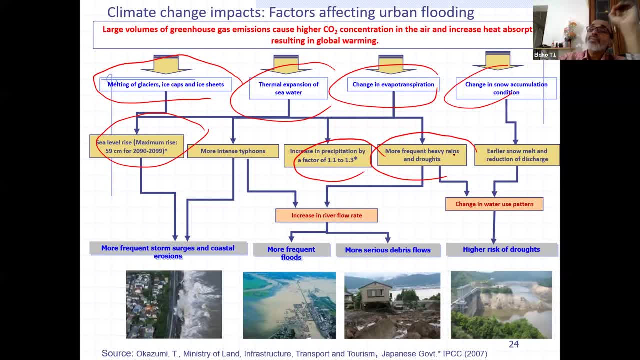 then by drought. so much now you see that normally there is no um climate change impact. then the normal rainfall events in in our place, in most of the places, are like 30 to 50 or 100 events of rainfall space. then that will be drastically reduced to 20 or 30 and then, whenever it stays, 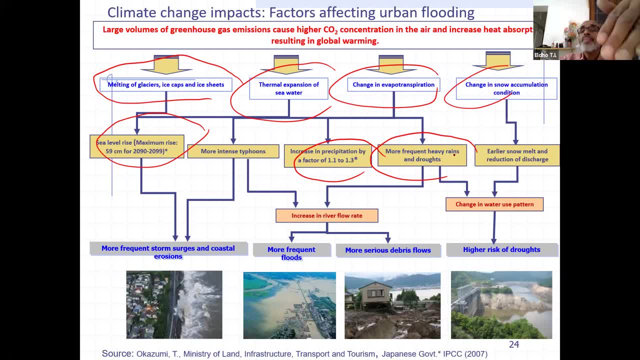 space, it is severe rains happening, so that is um the flooding, and then afterwards there is no way. so that is where the clouds, what kind of situation can take place? and then, after, impacts can be more frequent storm surges and coastal erosions um more frequent floods, more serious debris, etc. and like whatever we are, today's, yesterday's reported in. 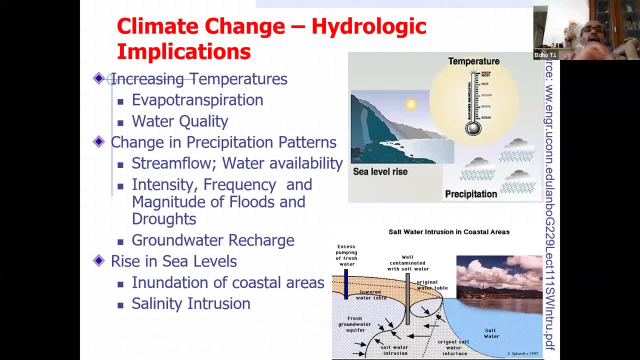 utah. so that kind of issues, uh, you can see and now, as i mentioned that, so one of the, the very, we can see with our naked eye what is happening. so that is what we can observe with respect to the. the climate change and hydraulic impact implications are so severe. 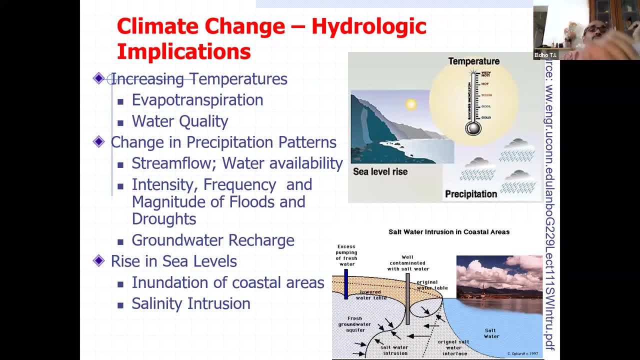 we need to study it in details. so as you can see, uh, as i mentioned, the climate change is concerned, temperature increases the major effect. so temperature increase is concerned, so you can see that evapotranspiration will be increasing and then, due to various other aspects, water quality also can be affected. then, second aspect is the, the change in precipitation pattern. 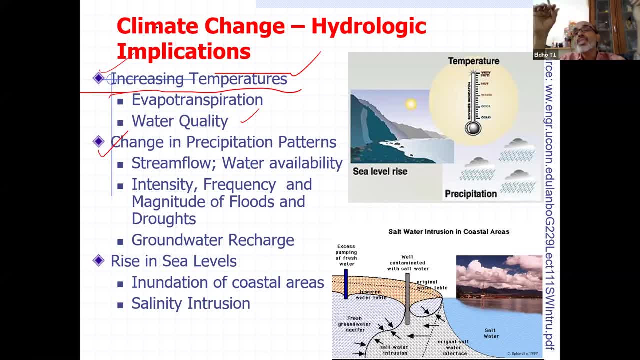 often for climate change is traces, and the latest report tells us thatatta are most off days or after dry season, for example, and also this change of conditions, of course, is very similar. so, yes, the temperature change impact that we already mentioned, the climate change impact, shows that whenever rain stays space, it will be severe rainfall day space, and then uh, uh. 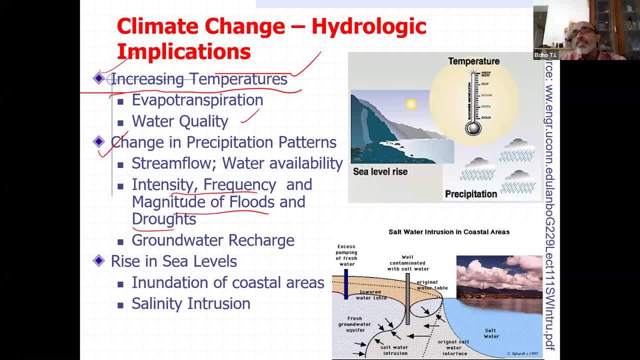 kontrollation, high intensity, so that use tozos, and then afterwards drought. so in men city, frequency and magnitude of floods, all this all depends upon the yield path, precipitation pattern, And then of course after effect can also be on water feature. And then another aspect is rising sea level. 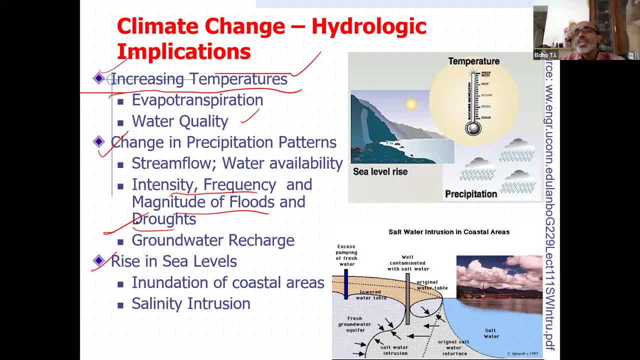 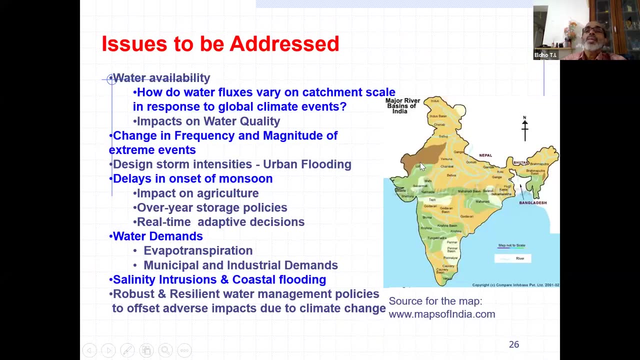 So sea level rise means most of our population living on the coastal region and then sea level is rising means then there can be frequent floods with, say, an association with the rainfall. So that is, that can be. that are the implications as far as the climate change is concerned. 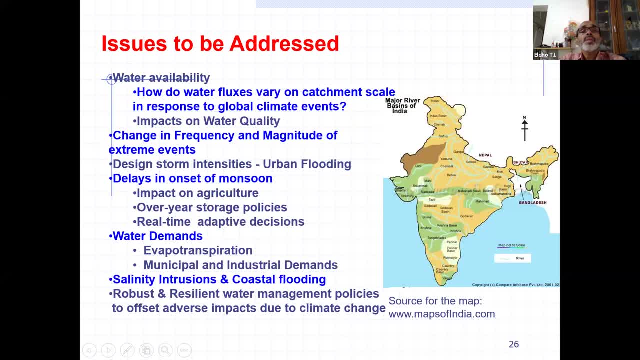 So that way we will say, as a country, we need to address a variety of aspects. So one aspect is, when you talk about water resource modeling or hydrological modeling is concerned, we need to assess how much water is available. So how do water fluxes vary on catchment scale in response to global climate events? 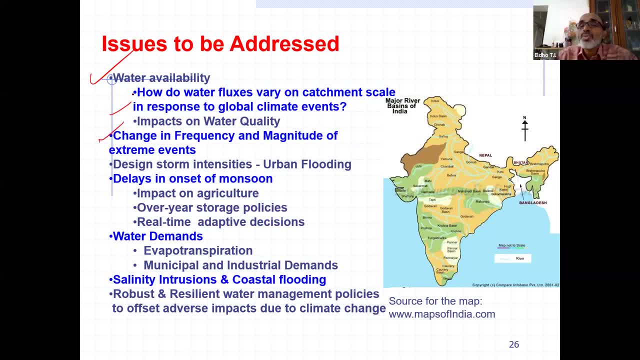 Then what are the changes in frequency and magnitude of extremes? So that also we have seen, And then especially urban due to climate change. So that is one aspect And then, as I already mentioned, especially agriculture is concerned. we raise the onset of monsoon and then water demands and sanity inclusion, cost of funding all those things. 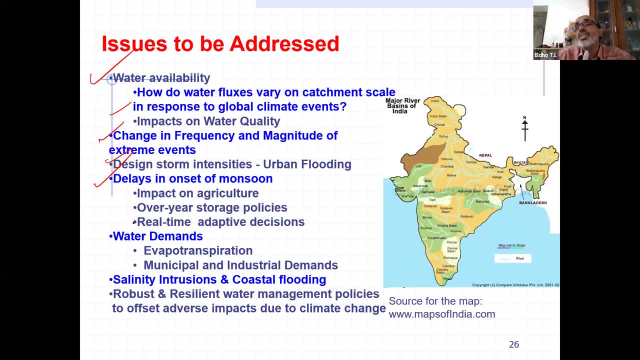 can lead to this various variety of issues. So this is this I am putting to the scientists, engineers and students: who is dealing with the water resource model? So there are so many issues that we need to deal with and then we need to go systematically. 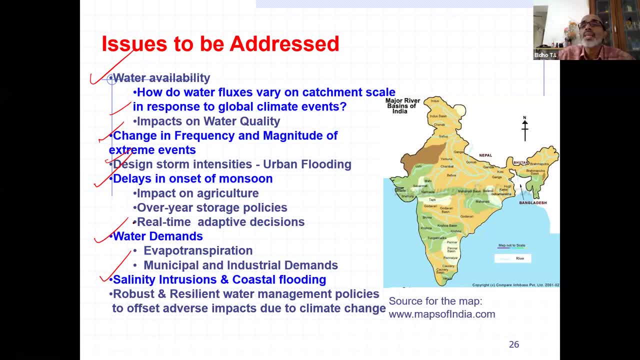 we need to deal with these kinds of issues and then each and every aspect, even one, to our basis scale. we need to see the, how much water is available, what will be impacts of the climate change in future. So that way, we need to do the hydrological modeling, we need to do the climate change. 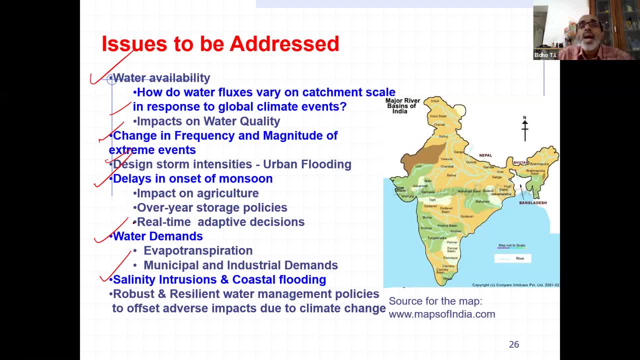 impact assessment. So that is very, very important. Am I audible and everything is going fine, Dr Patil? Mangal Patil, everything is fine, Yes sir, Yes sir, We are perfectly audible, Okay, Okay. 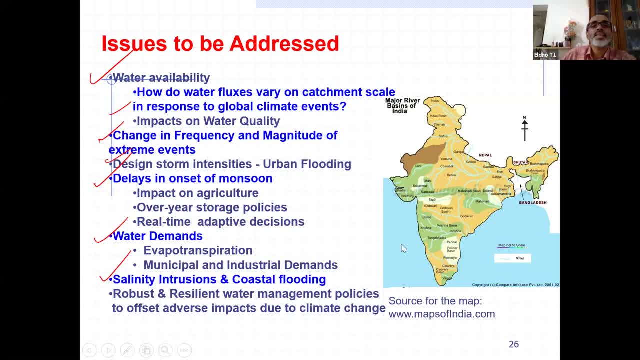 Thank you. So now we are going to move on to the next question. We are going to move on to the next question. We are going to move on to the next question. Okay, So whenever we say the climate change impacts of water resource is concerned, as I already 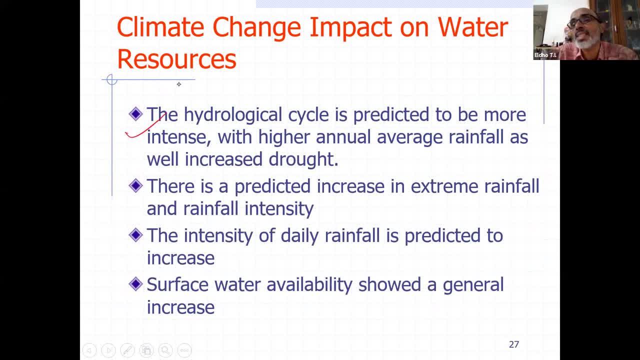 mentioned, the hydraulic cycle is predictably So many of our studies even. we are also conducting a number of river basins, especially in Western Gujarat region. My research team is working on this, which I will be presenting one case study here. 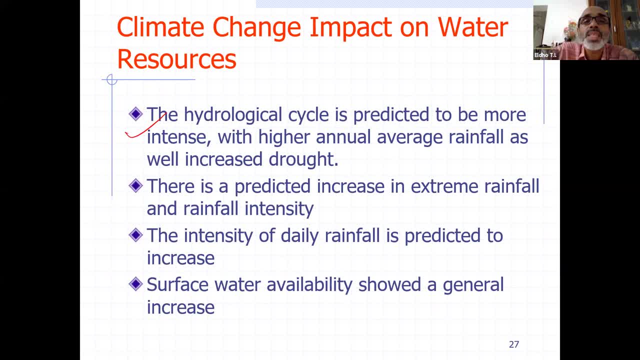 So most of the studies show that the hydraulic cycle is predictably most intense with the higher annual average rainfall, and then there is a predicted increase in extreme rainfall. So that is what we can observe. Like the Kerala floods, Chennai floods, all these flooding indicate that the extreme, even 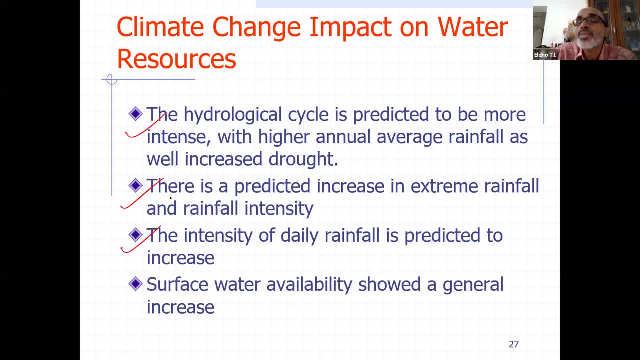 stay space And then the intensity of daily rainfall is predicted to increase, but the number of events may decrease, And then surface water availability showed a general increase. but that is holistic. But if you have sufficient storage, then that is good. But if the storage is not there, then immediately the water goes to the sea and then in the 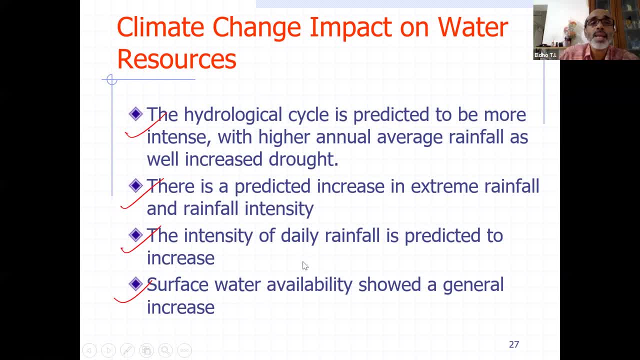 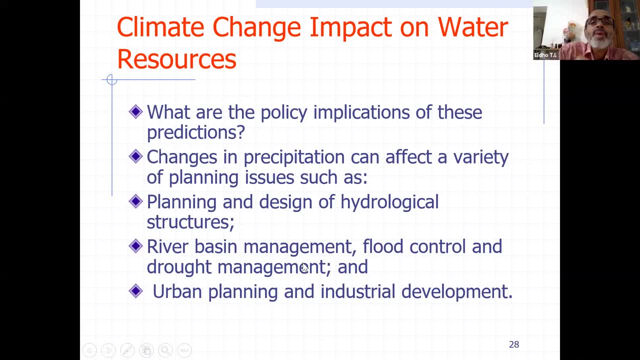 off-season, there will not be sufficient water available. Okay, Okay. So whenever, in terms of when we discuss in policy matters or management is concerned, what are the policy implications of these predictions. So you see that, so, as you can see, the change in precipitation can affect a variety of planning. 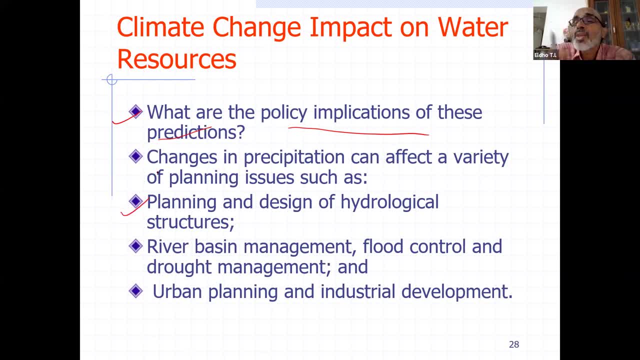 issues like planning and design of hydraulic structures. So you have a large number of dams, but you see that in Kerala 2018.. So it was, though we thought that, okay, we can store all the water whenever the severe flooding rainfall stays space. 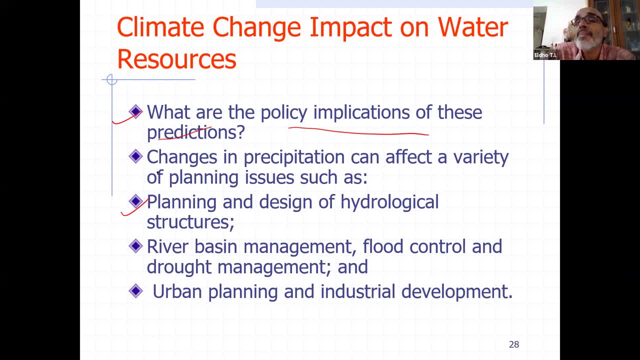 But then we are forced to really look at the water. Then we are forced to really open the dam, open the reservoir. The reason is that we need to. we cannot sustain that much water coming in few days time. So that way, even though storage is there, we will not be able to manage. 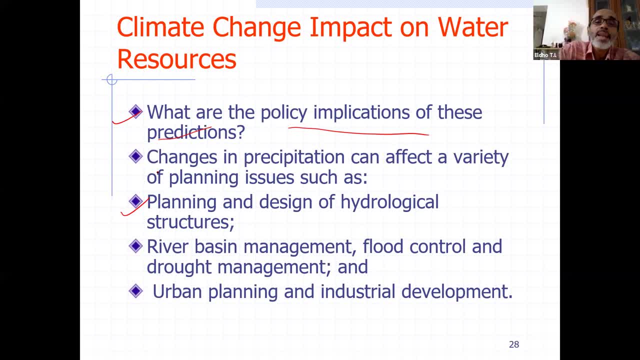 So the planning and design of hydraulic structures is very, very important. And then river basin management, flood control and drought management. as I mentioned, whenever rain is taking place in few events, or floods kinds of situations will take place, And then afterwards drought kind of situation takes place. 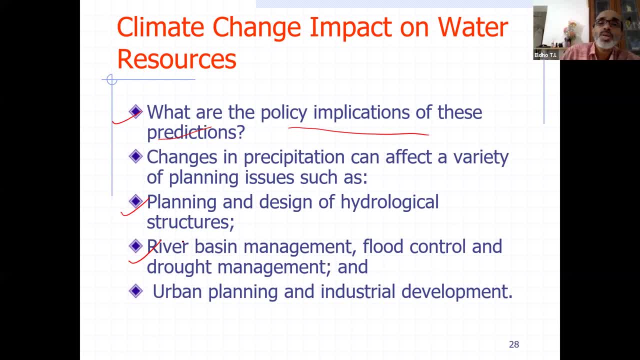 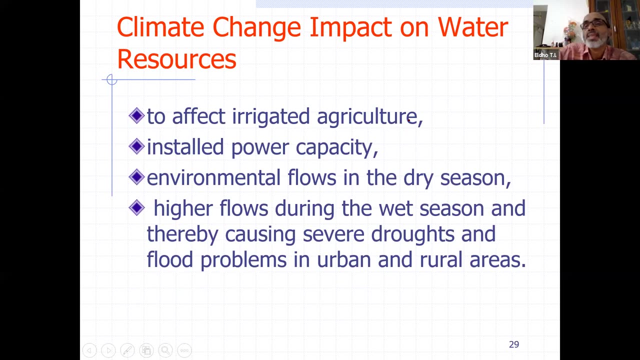 Okay, Okay, Okay. And then we need to also look into urban planning and industrial development within the perspective of climate change. So then you see that many of the irrigation engineers or agriculture engineers, so how this is going to affect the irrigated agriculture. 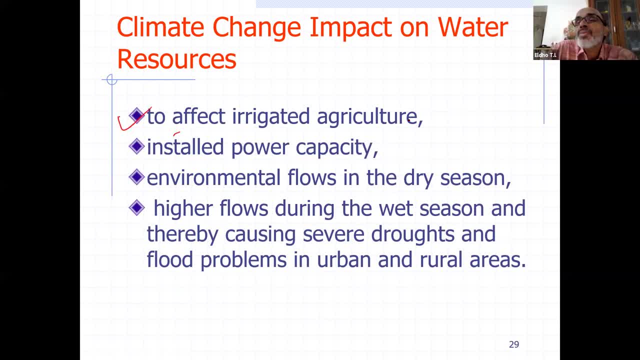 So you see that in India hardly the 35 to 40 percent only irrigated area is. the remaining agriculture is done based upon the rainfall pattern only. So that way, if it is irrigated agriculture, how will it be affecting the irrigation area? 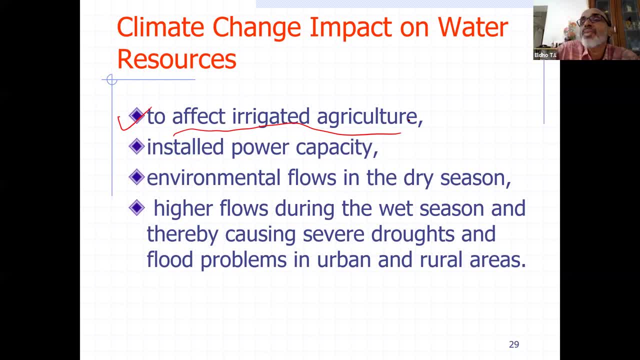 Okay, Okay. and if it is unirrigated- I mean no irrigation is there- then what are the problems of climate change that also we need to look into? And then also another important aspect is that in India, around 20% of the power. 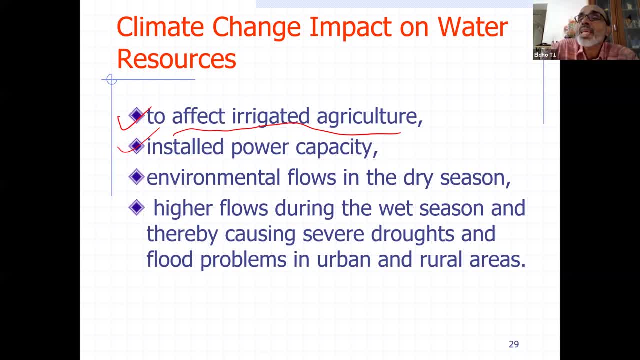 is coming from hydro power projects, So that also can get affected, since there is no sufficient storage and then power capacity will be decreased. Then we also need to see that, these reservoirs, we need to see the flora and fauna. what is happening with the environment? 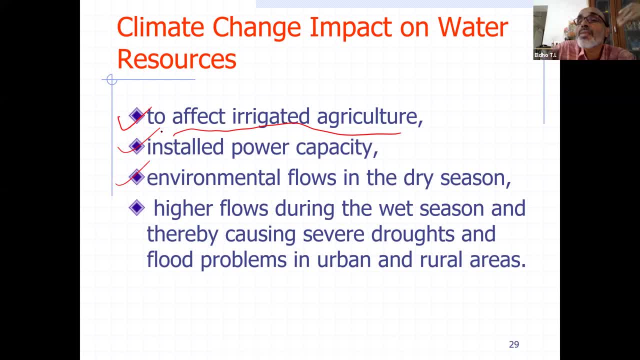 before is very, very important. So how much? if the water is not available reservoir, then we cannot release the water, and during the green season or the summer season, So environmental flows in dry season and then high flows during the wet season and thereby causing severe drought and flood problem. 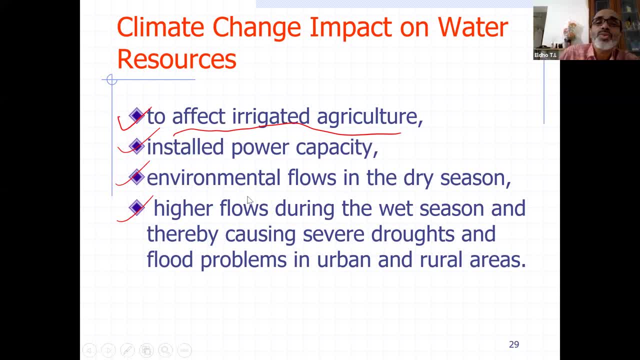 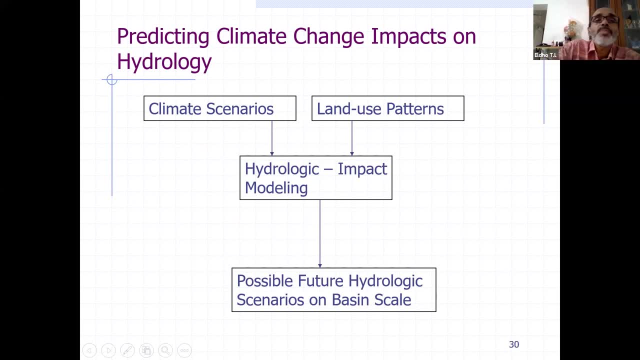 So all these issues- climate change and hydrology is concerned, so important and we need to look into So that way, when we look into, say, predicting climate change impacts on hydrology. so there is two aspects. One is the climate scenarios. 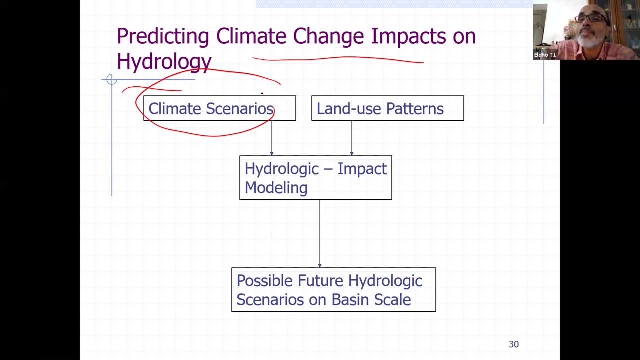 So we need to see, as I mentioned, RCP 2.6, 4.5, 8.5, like that- various scenarios we need to assess, And then we need to see that if a particular watershed or river basin is concerned, 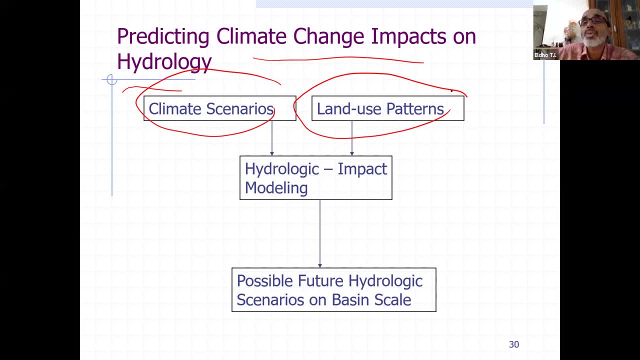 we need to see what are the land use pattern and how it is going to affect with respect to hydrology. So we need to do hydrology impact modeling using SWAT, VIG or whichever model you are preferring And then, based upon that, we need to come into the possible. 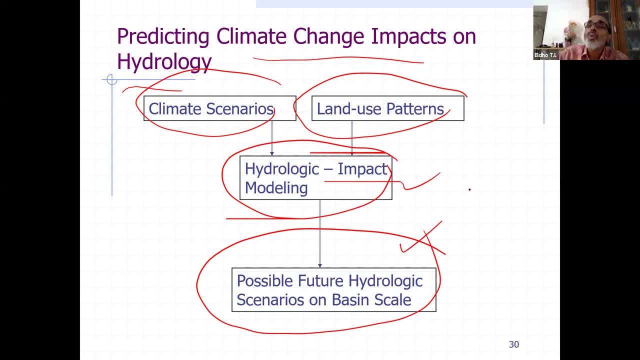 future hydrological scenario, and then we need to look at what is going to happen in the future. So that way, all the river basins in India, we need to assess, with respect to the climate change, what can happen, what is happening in the past, historical 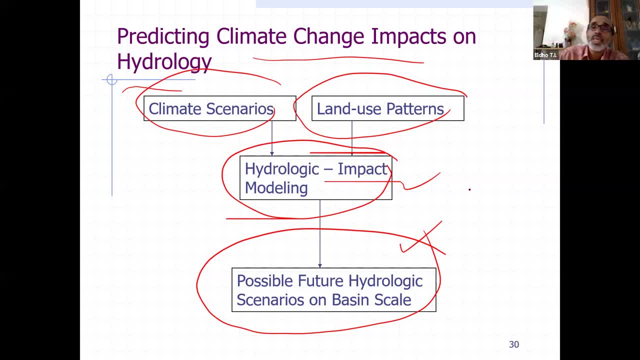 and then what can happen in currently what is happening, and then we need to project what can happen in 80 years, like it only went up to 2100 now the scale put by IPCC, So that also we need to look into So that way. so first we want to be 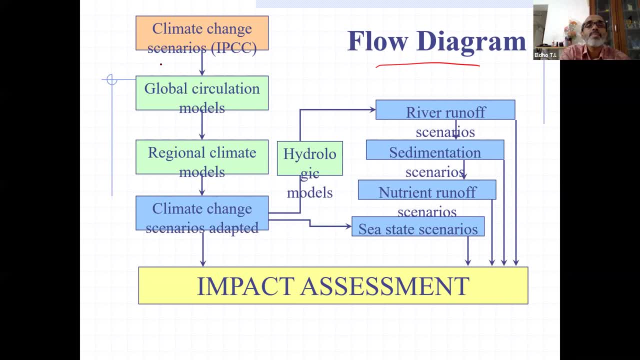 this kind of assessment. how we do. the flow diagram is shown here. So first, the climate scenarios we need to study. So, as I mentioned, we have a very sophisticated system like global circulation models, So using that we can have regional climate models. 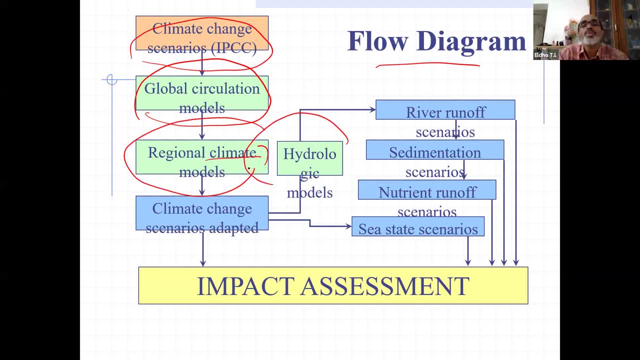 and then this will be from here. we will be having input to the hydrological models and hydrological models will be giving the river runoff, then sedimentation, routine runoff, then the various scenario, like sea state scenarios, all those things can be obtained. 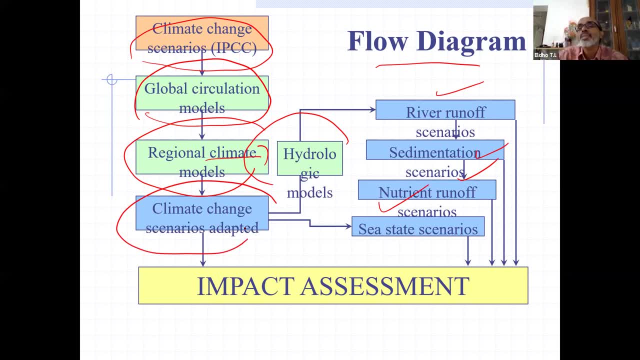 And then the climate change scenarios adapted, So like, if you are going for, like now after the Paris Agreement, whether we'd be able to go to keep the same kind of pace, like whether we can sustain to at least 4.5. 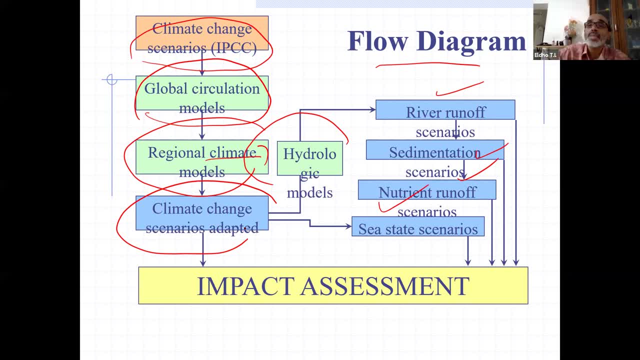 instead of going to the severe condition of 8.5.. So that is what we need to look into, though we may not be able to achieve 2.6. I mean the very low emissions compared to what is happening. So then, based upon all those things, 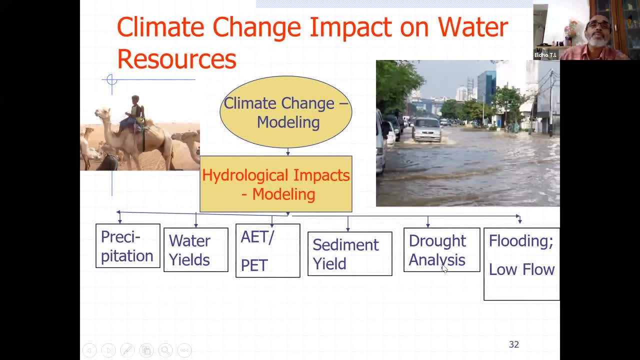 we need to go for the impact assessment So that way, when we come to discuss the climate change impact on water source, the climate change modeling is very important. So, as I mentioned climate change models, we can use general saturation models and then, based upon that data, 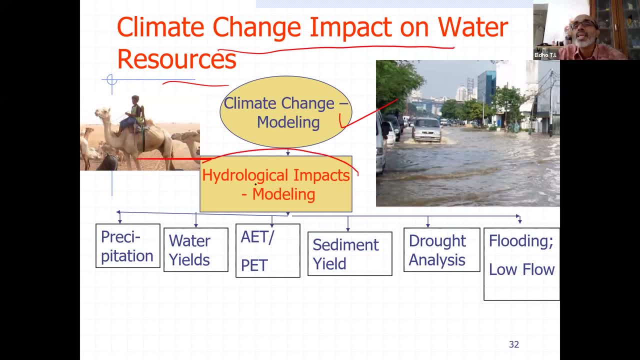 we can put into hydrological models And then the hydrological models will be giving the precipitation, water release and the evapotranspiration- sediment, drought analysis, flood water, low situation. all those things can be obtained With respect to climate change and the hydrological modeling is concerned. 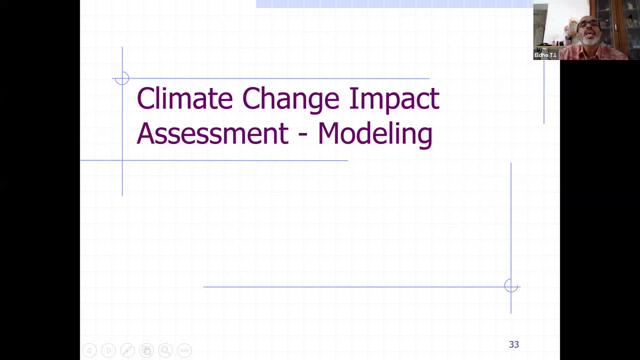 So now the next part of my lecture. we will be discussing a few case studies: climate change impact assessment through modeling, So how we can effectively utilize the hydrological model as far as the climate change is concerned. So the model which I'm going to discuss is SWAT model. 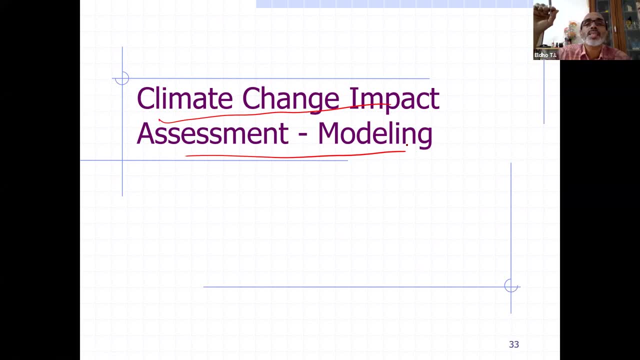 So of course I understand that there will be a training program on SWAT later in this one week program itself. So that way now you can see how it can be effectively utilized for these kinds of studies. So as far as climate change is concerned, 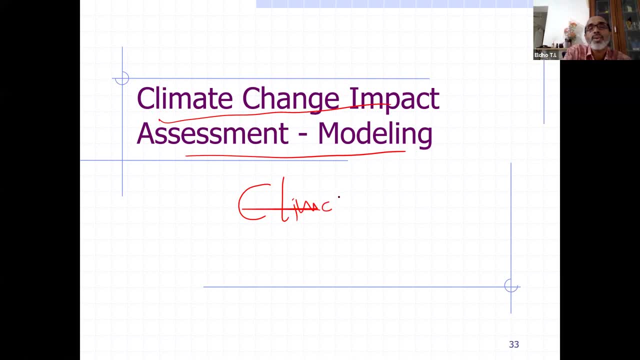 so there are two aspects: One is the climate change and the second one is the hydrology. So climate change is concerned, as I mentioned, and we already see what is hydrology and hydrology model is concerned- The climate models are concerned. 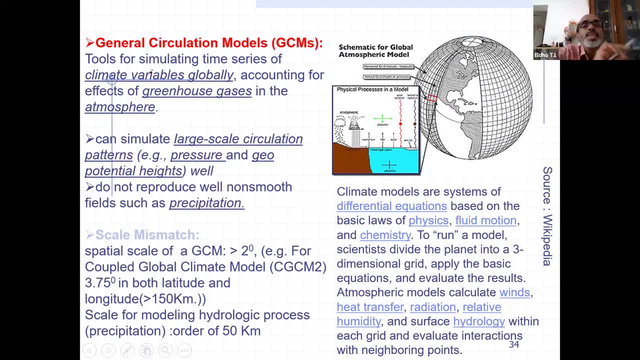 You see that the most reliable model is general saturation models. So these are the tools for simulating time series of climate variables globally, according for the effect of greenhouse gases. So they can simulate large scales, saturation patterns. And then you see that the total hydrosphere, total system will be modeled, as you can see. 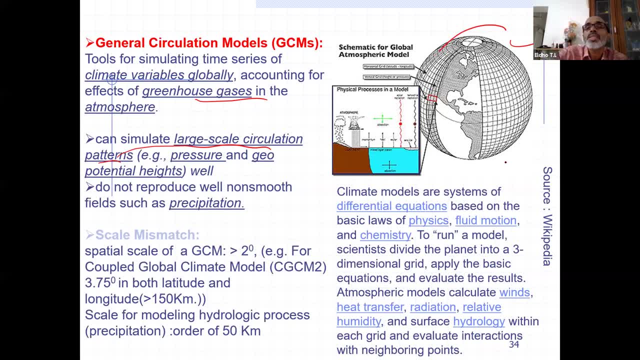 here, in this figure here. So you can see that the holistic model is based upon the mathematical modeling is done. So that way you see that we cannot go for a very final scale. So you see that most of the scale mismatch is there. 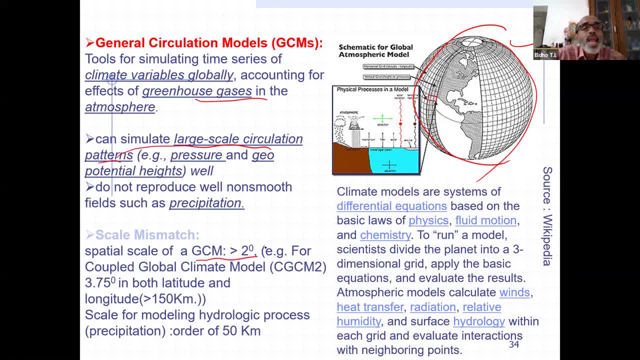 The spatial scale can be more than two degrees And so that way it is more than 150 kilometer, even in the polar regions. and the scale of models- Generally hydrology model- is concerned, we need to get a very finer scale. 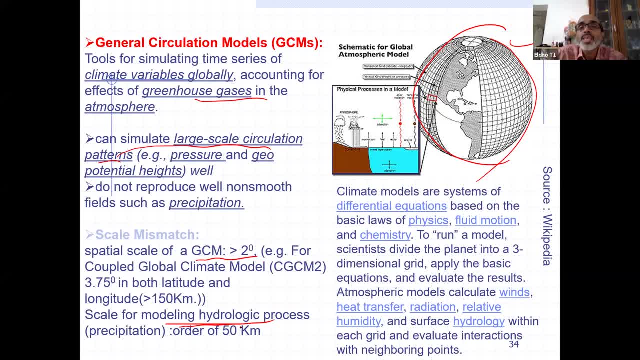 So at least 50 kilometer scale we need. So that way the climate we need to go for. the scale mismatch is a major problem. And then, as I mentioned, climate models are systems of different equations. So this is how the GCEMs are developed. 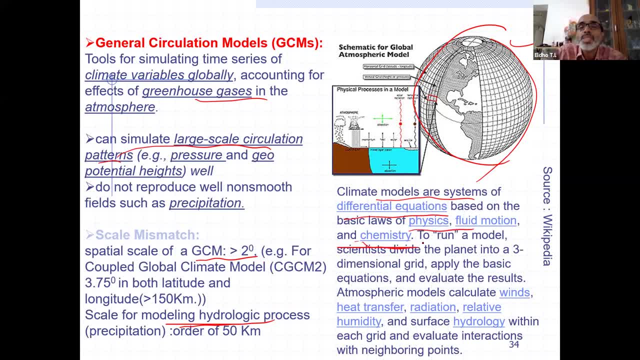 I am not going to detail so that I can't say that. So in our country- physics, food, motion, chemistry, etc. These models are available. Unfortunately, in India we don't have our own models, but we have to depend upon American. 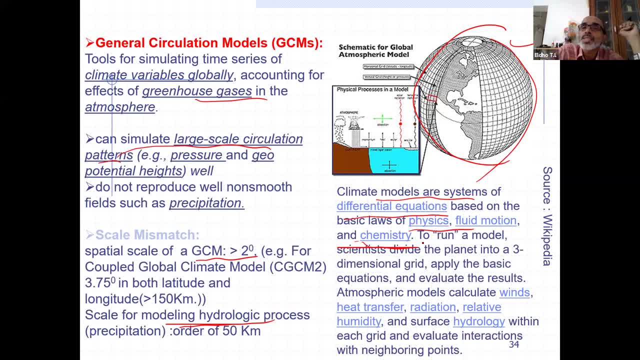 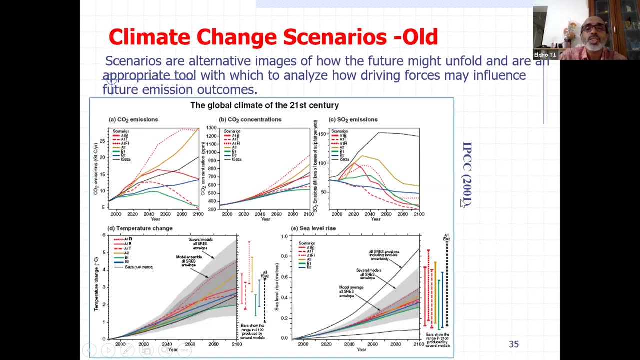 Japanese or the European or Canadian models. as GCEMs are concerned, though, we are having some regional climate models with IRPM and other organizations are developing, So now using these climate models so we can go for the various scenario assessment. So, as I already mentioned, 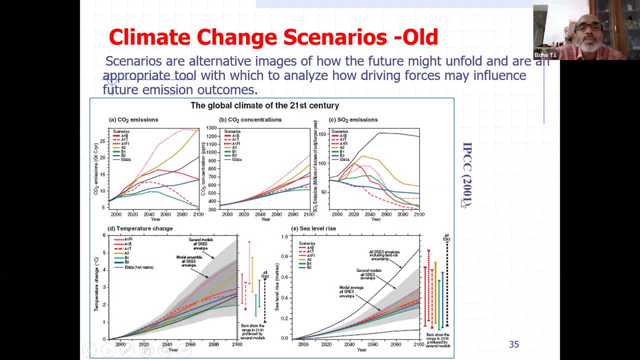 with respect to climate, various kinds of emissions, how the system is working. so there is. so those are working. this area we you may remember that the cvcv5 cmip three models were there earlier. now we are going for cv6, cmip, spy models, and now later what is going to come is cvc might be six more kinds of things. 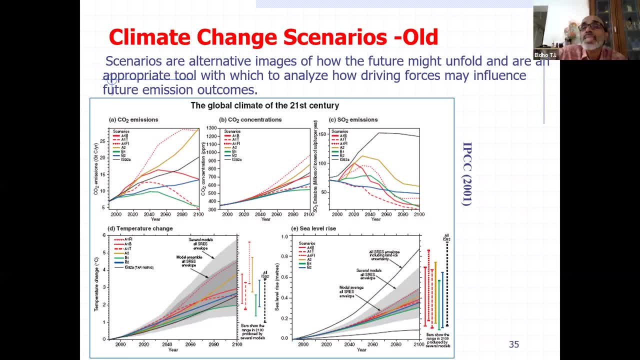 but of course these are all some kind of improvement. like when we write a book we say addition, one, addition to like that. this is further improvement. so earlier scenarios like, if you remember, a1b haven't even like that- various scenarios, but now we are going for accordingly. 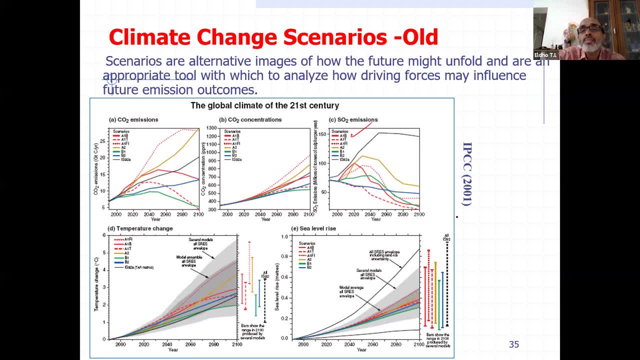 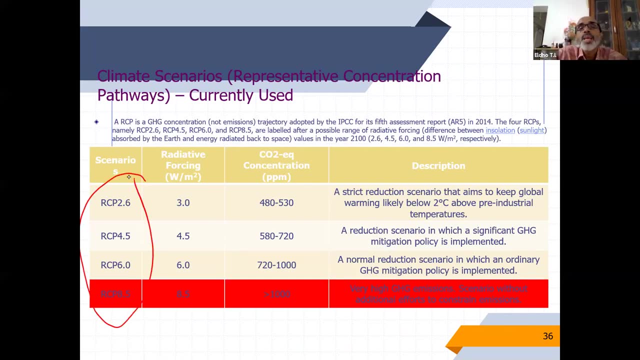 they are. they see me for three ipcc, which was published in 2001 and the corresponding scenarios we can see here. but now we are going for cmip for five models. so there, as i mentioned, that we based upon rcp 2.6, 4.56 and 8.5. so here, as i mentioned, currently we can say that what is? 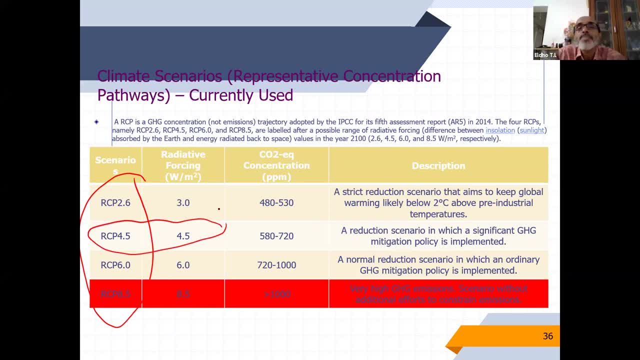 happening. maybe we can put in this level, rcp 4.5, and then if you can further decrease the emissions, then we can go, even come back to rcp 2.6, but if you can at least maintain what is happening to be here, but if it is. 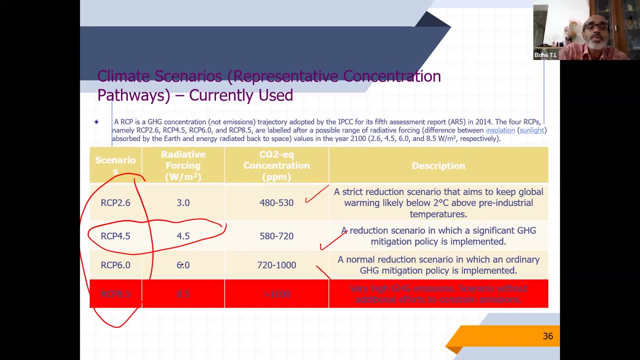 say, very high emissions, continuous, then it we can get to 8.5. so that way we can see that in these all those kinds of models generally, when we climate model is, or hydrological model, we assess two kinds of systems. one is rcp 4.5 and rcp 8.5, and then, if you want to see a better future, then we can also assess 2.6. 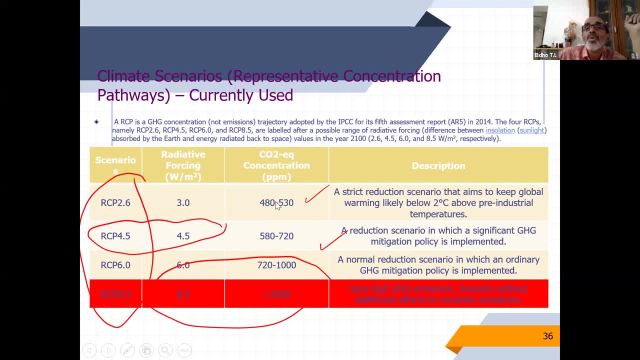 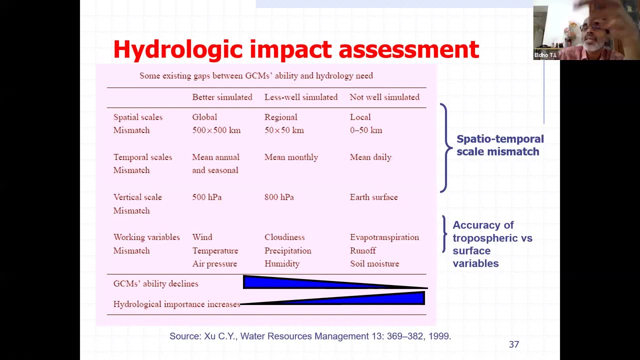 so that way the the current simi, simi 3, simi 5 models we can utilize and there is not much mismatch between simi 3 models. it's only thing is that the some improvement will be there and then coming back to hydrological. so what are the issues? so some existing gap between. 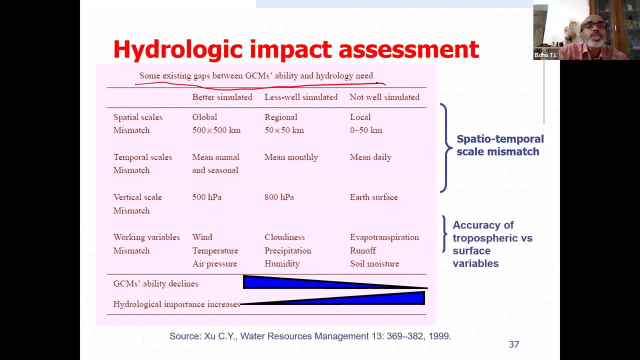 dcm ability and hydrological model is there. so spatial scales are concerned. but we can see that. we can see that there is a gap between dcm and hydrological model is there. so spatial scales are concerned. as i mentioned, global scale, uh, climate models are, say, 2.5 degree or sometimes even 500. 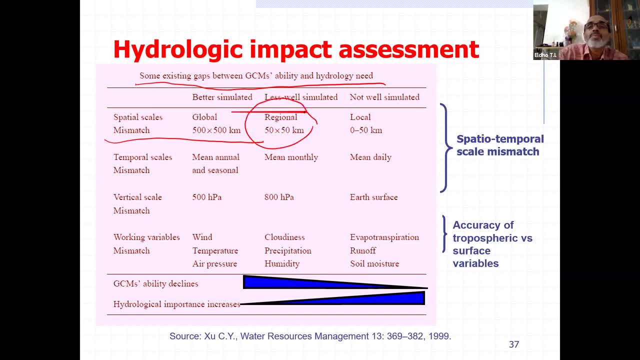 kilometers by 500 kilometers and regional scale models can test by 50, but the hydrologis concern we need to grow comfort is smaller still, so less than 50 kilometer basis is recurred. and then the temporal scale is concerned. it can be mean, annual or uh. so whenever we say normal hydrology it is better to get a daily basis and a vertical scale. it is larger when working at the water level- more than 50 kilometers a day, that would change and normal hydrologic scale is better seen. it is better to get monthly logical scales. other modified. your annual look at the schedule power view average is: better than a full day annual law e year or 3 year. but Plan något we say normal hydrologic scale. guess is better. chances are lower than a 30 day, see on 20 days per week. librarian can have significant to travel, so at once we leave facility laser don't have really a lot of water supply transport. 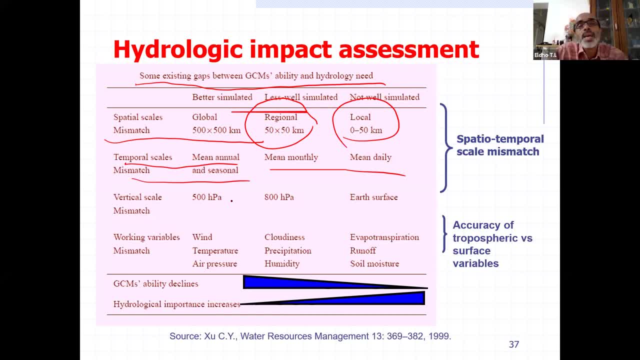 and a vertical scale match, like the GCMs are based upon high 500 hectopascal kinds of pressure variations. But then, if hydrology is concerned, we need to see what is happening on their surface. Then working variables like wind temperature- all those things are there here, evapotranspiration- are not. 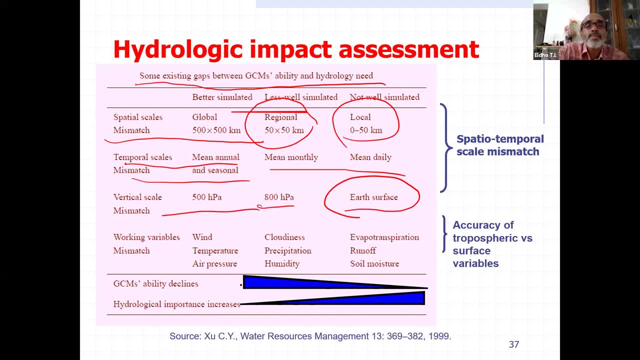 So these kinds of issues are there And GCM scale is very high, So the ability of GCM, everything declines on small scale And hydrology is concerned, we are having with high scale we don't get anything, So we need a smaller scale. So this is the special temperature issues. as far as the climate is concerned, 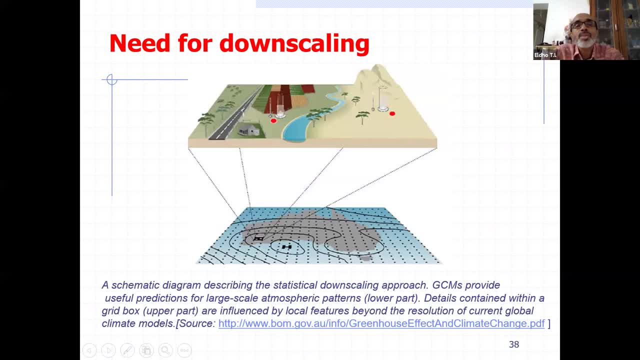 So that way we need to go for downscaling. So downscaling is concerned, Generally, we are having two kinds of So this is where the systems are now coming to, Normally what is happening. we need to look into smaller scale. 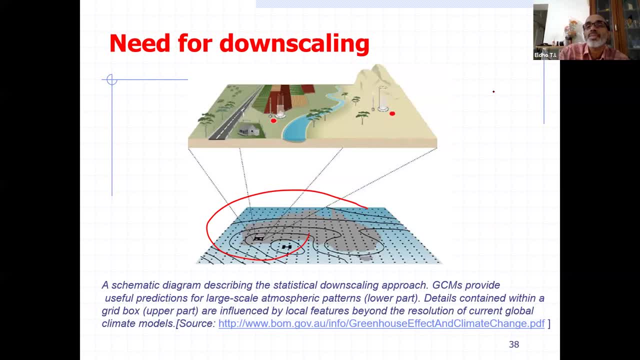 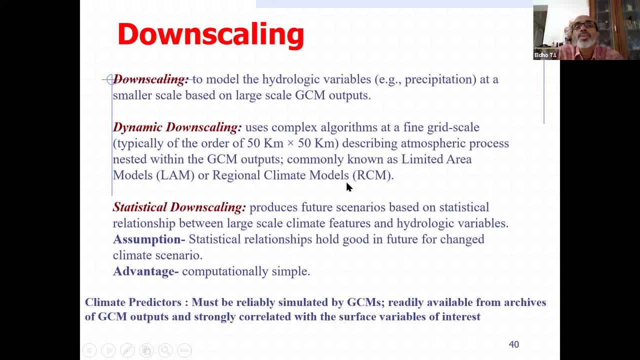 One is the statistical downscaling and dynamic downscaling. So dynamic downscaling based upon the local conditions, We can say, for example, 50 km by 50 km, we can come like RCM, regional climate model. RCM can be developed. 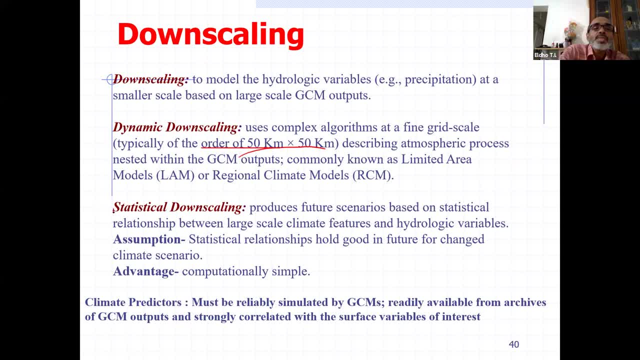 So, like IATM is doing, as I already mentioned, And then statistical downscaling is concerned: Based upon the data, we check the aspect and then we do appropriate changes As far as the bias correction will be done in the results. So that advantage is that computation is simple but dynamic modeling is. downscaling is computationally intensive. 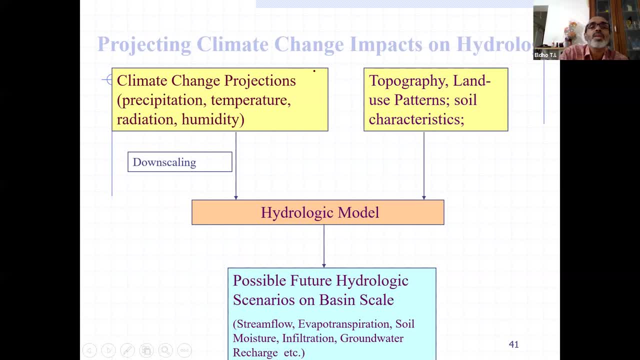 So now coming back to the project, climate change impacts on hydrology, climate change projections are concerned mainly precipitation, temperature, radiation, humidity, all those things. what we are getting, That is the input getting from the GCMs and through downscaling we can go for the river basin scale. 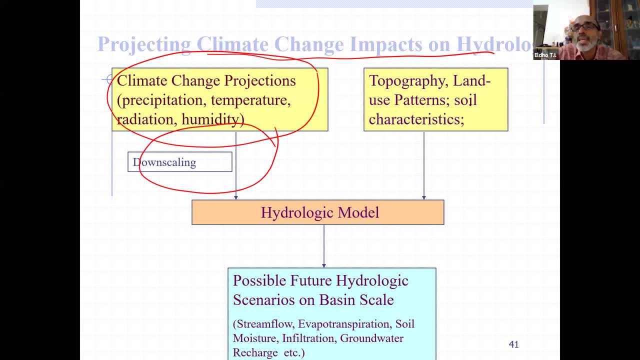 And then from the topography, land use pattern, soil etc. That are the inputs coming from the geographic features and the deterioration model etc. And then we run the hydrological model And then finally we can get the pure possible future hydrological situation scenarios on basin scale. 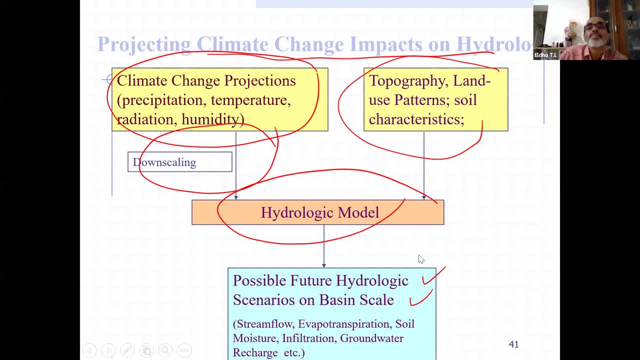 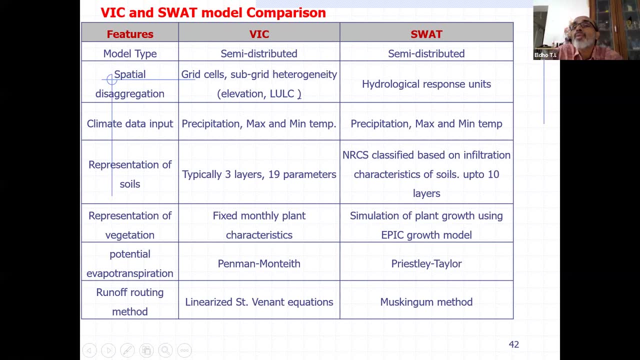 like stream flow, water transpiration, soil moisture, etc. So that way you can see that, as I already mentioned, different hydrological models we can utilize for this kind of assessment. Two commonly used models are. one is called BIC, Variable Infiltration Capacity Model. 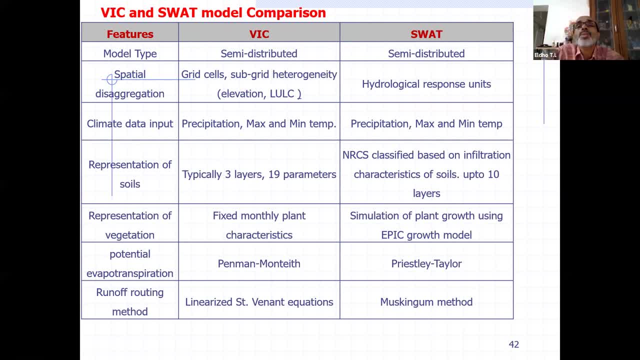 And another one is called SWAT model Soil Water Assessment Tool. So both models my research team is using currently. So BIC is generally a grid based system, So like a 0.5 by 0.25, by 0.25 degree, I mean 25 by 25 kilometer grid. what is happening with the assessing? 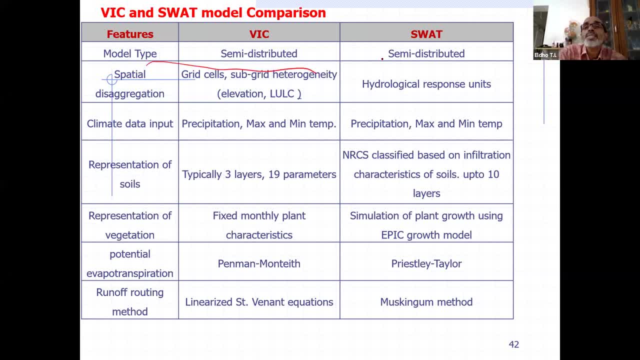 And so it is a semi-distributed model. But the SWAT is concerned, that is also a semi-distributed model, but that will be specifically for a river basin scale, Or a basin or a watershed is concerned. So then, so BIC, generally we deal with the grid cells or sub-grid scale. 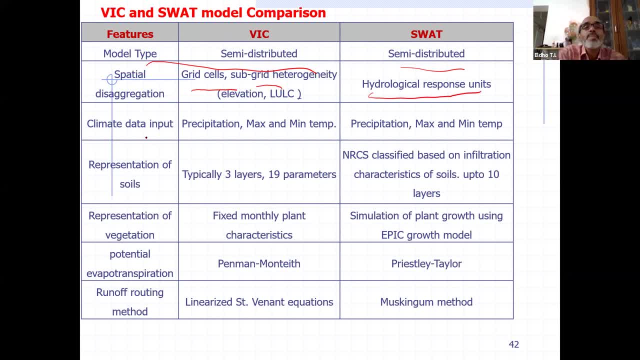 And SWAT, we generally do Hydraulic Response Unit And climate data input. what is needed for BIC model is precipitation maximum minimum temperature- So we are also winning in the same- And representational soils. typically three-layer models and 19 parameters are concerned in BIC model. 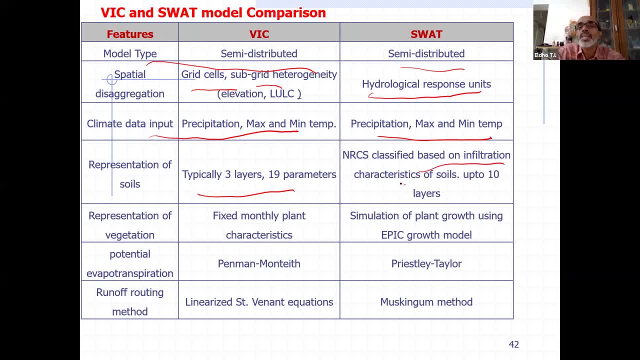 And here we can have. even up to 32 parameters can be there, And in SWAT we can go- for I'm sure that you'll be getting training later- so up to 10 layers we can do, And the representational vegetation is concerned. 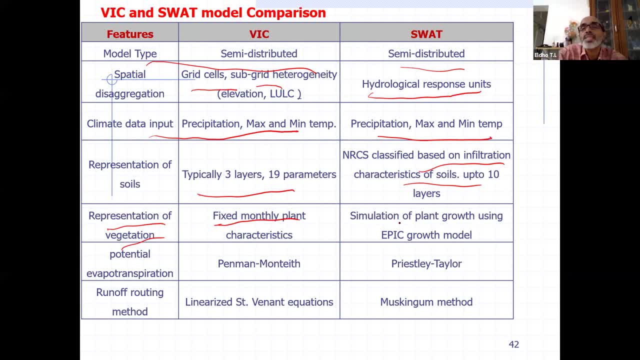 In BIC model we do. pixel plant characteristic simulation of plant growth is also concerned. SWAT model And evapotranspiration. various variety of models can be there. Generally Penman model is used in BIC model And here basically or Harvey's. different kinds of methods are available in SWAT model. 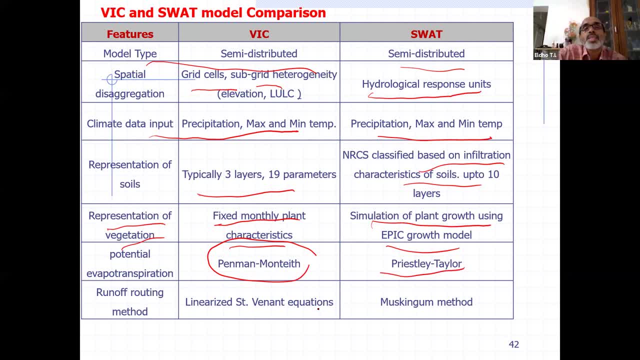 And runoff routing. we have to say generally, we can use in BIC model And runoff routing. we have to say generally we can use in BIC model And runoff routing. we have to say generally we can use in BIC model. 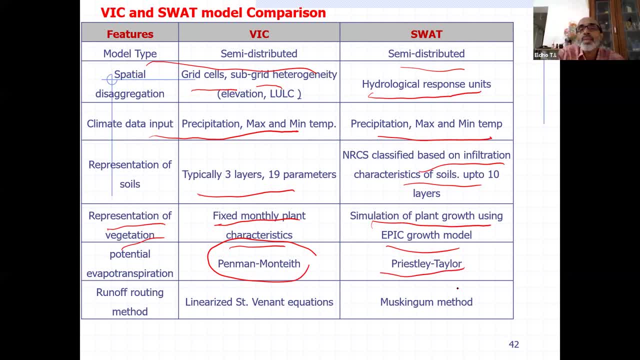 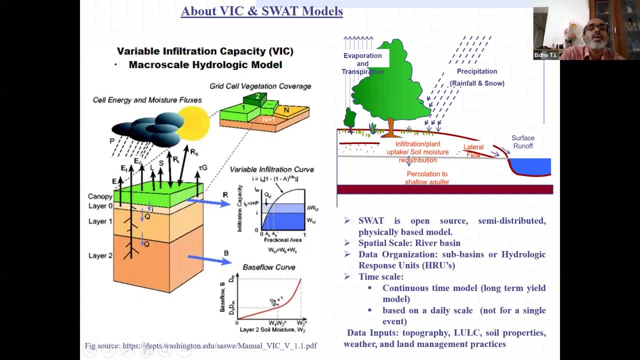 And runoff routing. we say generally we can use in BIC model And here linear, nonlinear Muskingum model, that kind of methods we can use in SWAT model. So this is – this pictorially representing what is BIC model. 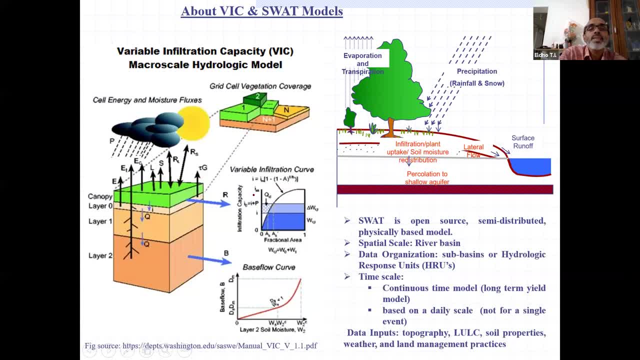 So here is the grid we are considering, And then three layers- soil layer- and then these various parameters are considered, Those who are interesting. you can see all these aspects in these website And then how the variations are taken there in grid basis. 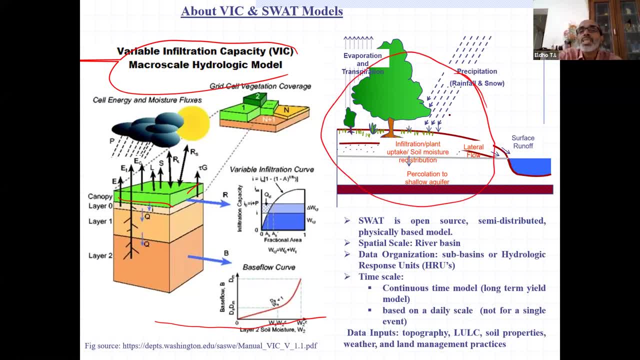 But in SWAT model is concerned, we take as hydraulic response units, with respect to vegetation, the parameters and uh. so it is an open source, semi-distributed model. uh: spatial scale, river basin that organizes some basins, scale and time scale. continuous time modeling is possible and 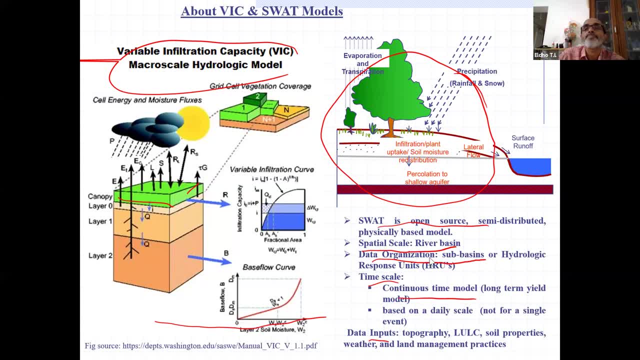 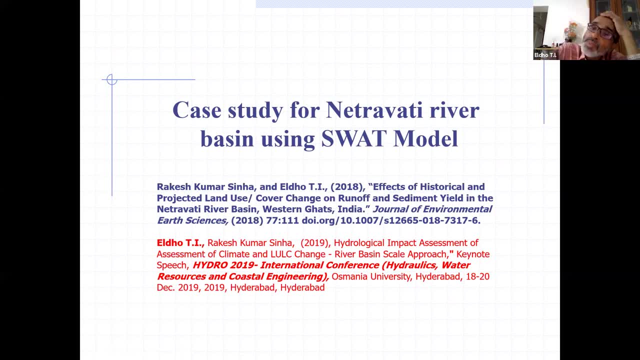 that time, books in growth, topography and years is all properties, etc. so now, uh, next. so this is about the hydrological model and then two important models which we use as far as the climate change impact assessment is. one is a basic model, second one is the, the, the swap model. 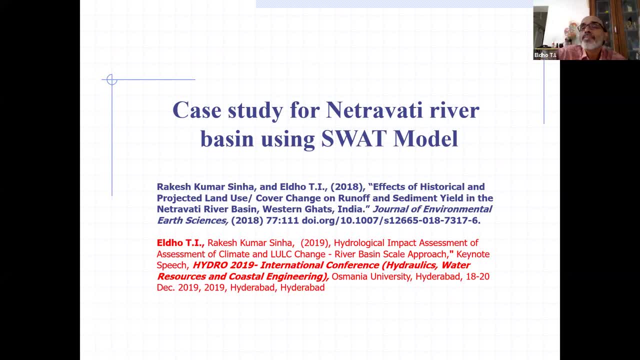 okay, now i will just show- anyway i'm not going to details of this model. so i'm sure that the SWAT model has a training program and vic models also. a lot of literature is available. so now how we can utilize for particular reason, how we can utilize it for an assessment, for 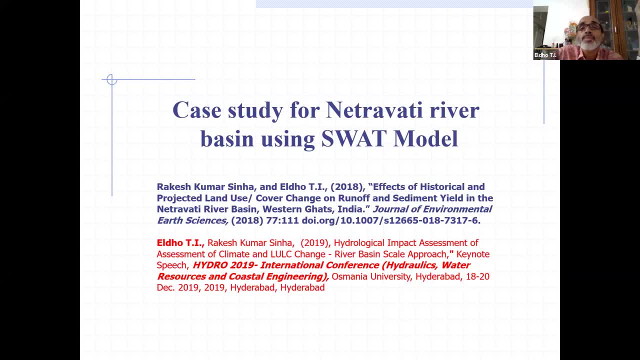 climate changing impact assessments for, say, for example, using swat model. so that is what we are going to discuss in this case study. so this case study we have published in general environmental systems analysis Science 2018, and then another paper, also in 2019, and then Hydraulic Science, then another. 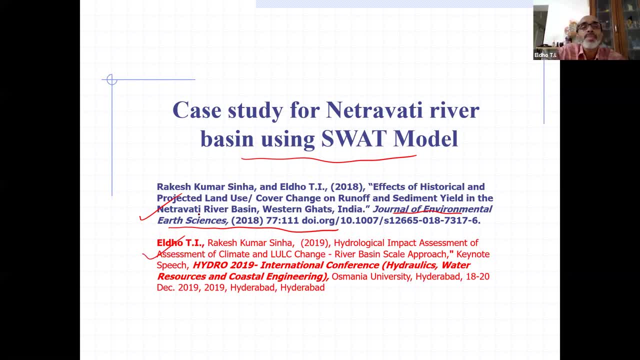 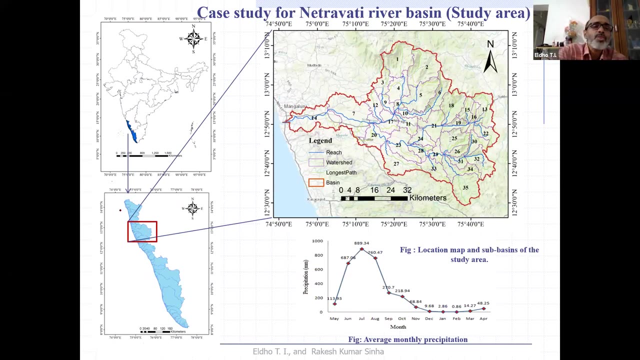 case study you can see, published in last year by my student, Agish Kumar, and myself. So these papers gives a lot of information how we can use SWAT model as far as the Hydraulical Impact Assessment of Climate Change. So here what I'm going to project, actually as part of Ministry of Water Resources, INCC. 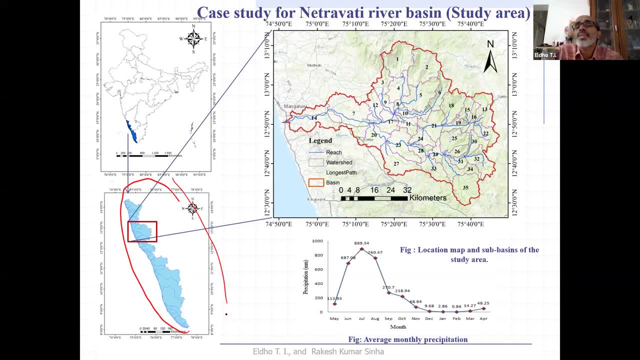 we have got a project to study the Climate Change Impact of Tadri to Kanyakumari, the Western Ghats River Basin, So that study is in progress. So as part of that study, one river basin is done by my student, Dr Agish, who has done 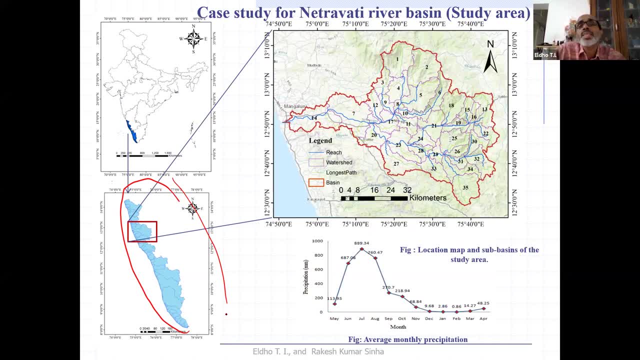 PhD with me, So that is the results I am presenting. So here the case study is Netravadi River Basin. So here you can see, this is the Netravadi which is located in Karnataka region, and then this is the outlet and here this is the basin boundaries. 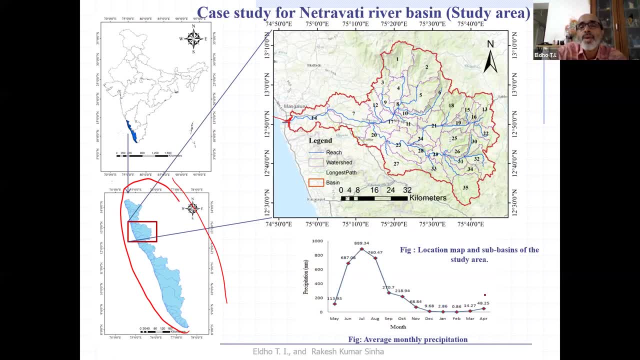 And here the rainfall. You can see that mainly monsoon season heavy rainfall is there and this is a good rainfall area with around 2,500 mm per year. So here the details of the study here in Netravadi River Basin, approximately 3,500 square kilometer. 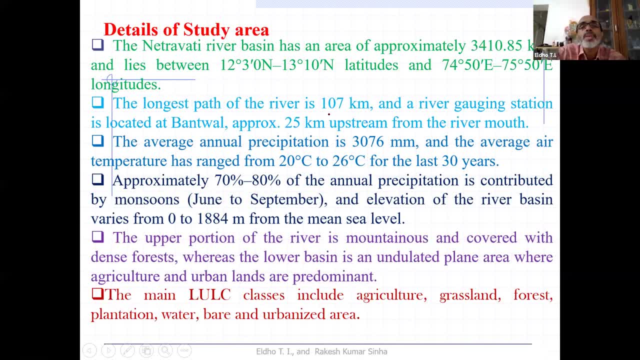 area and the longest part of the river is about 107 kilometer, and then the average annual rainfall is more than 3,000. sorry, it is about more than 3,000 is the rainfall per year, and temperature variation is 20 degrees to 26 degrees. 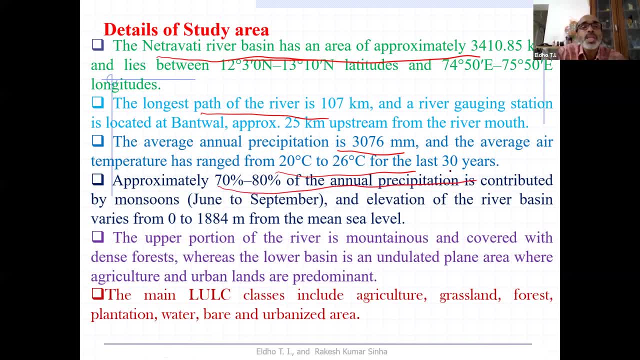 So the average annual precipitation is approximately 70 to 80 percent during the monsoon season and the upper portion of the river is mountainous and the lower portion is like mangrove city and other area. So the ELIRSI classification include agricultural, grassland plantation, water layer and urbanized 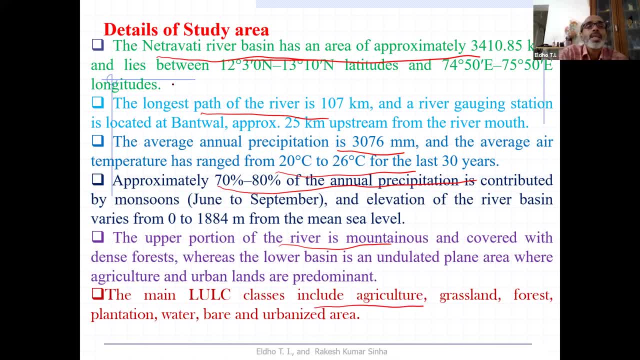 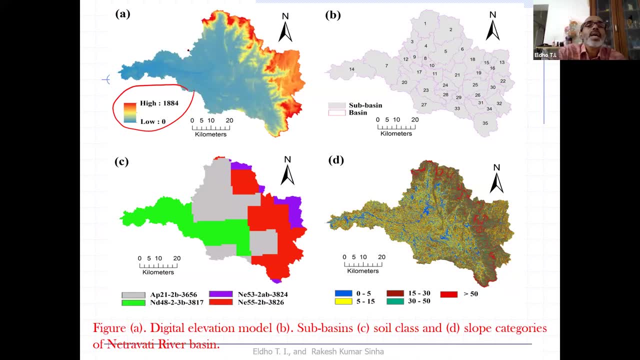 area. So this shows the deep elevation model. The deep elevation model is: we are using the CARTOSAT data and then it is: maximum height is 1884 to 1,800 meters. Okay, So it is 1884, and then it is told in the C that is low. and then here you can see the 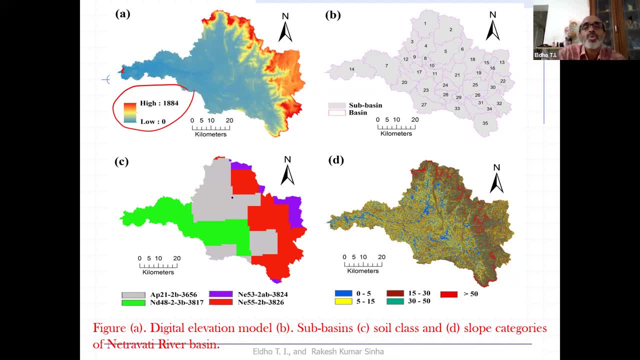 soil map, soil classification. a variety of soil location, like the sandy loam or some area is clayey or that kind of soil pattern is there and this gives the hydraulic response which we have done using the swatch. So various numbers automatically in our swatch we are getting and then this figure shows. 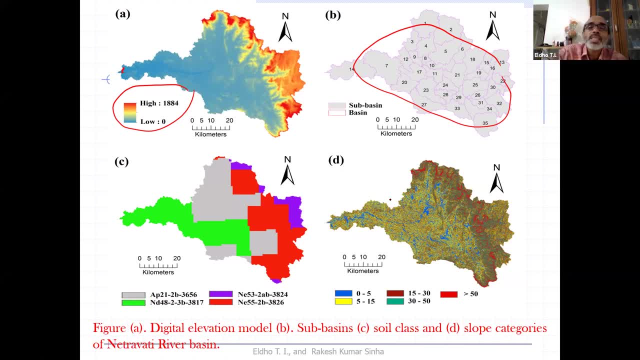 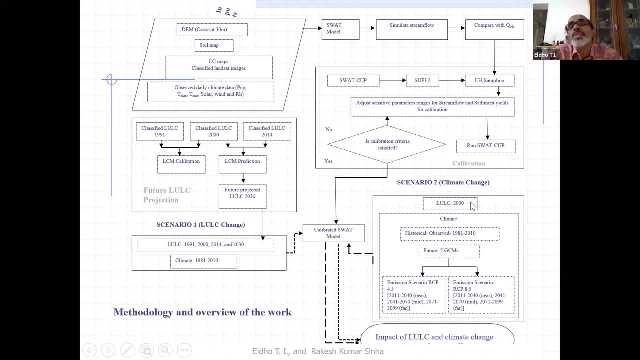 the slope categories. It is high slope for how the water level is Okay. So this is the range in which the radiations are taking place, and also the drainage pattern of the nethra of the river basin is shown. So this is the methodology which we adopted. 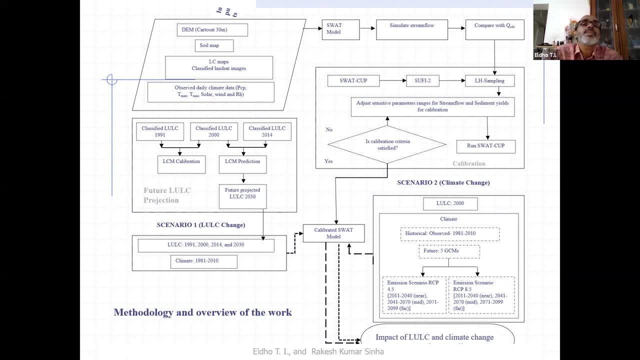 So for this particular Tadriti Kanyamari and their studies, we are using the same kind of methods. So the method in which we started with the deep elevation model soil map and ELIRSI map, for the historically is concerned, we use the Landsat data and then we get the classified. 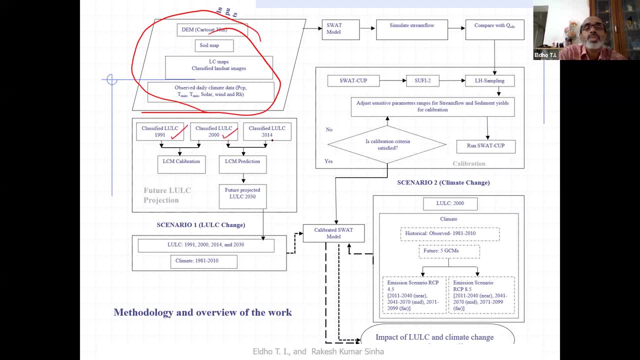 ELIRSI for historical, like 1991, 2000,, 2015.. Okay, So this is the map. Okay, Okay, 14 or 15, and then we go for. so you see that either you can keep the same kind of lulc and 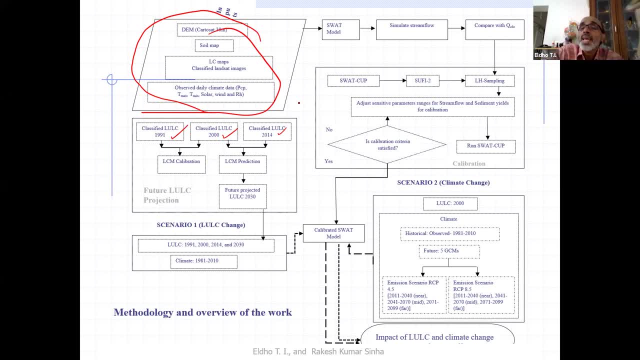 then project for the hydrological impacts for the future climatological impact for 2100, but you can also project the lulc changes using land change model, so that also we are done. we are projected to 2030, 50 up to 2100. so, though, i'll be putting the results up to 2030 and then 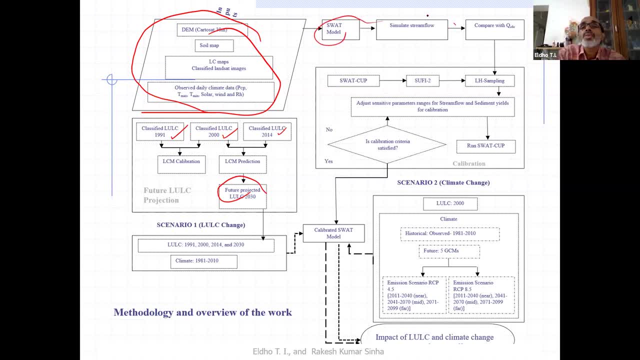 uh, we will be using swat model model so to simulate the stream flow and compare the runoff so that company is used for the calibration and validation purpose. so calibration of various parameters- about 50 parameters are there- and start model out on that around 12 parameters. 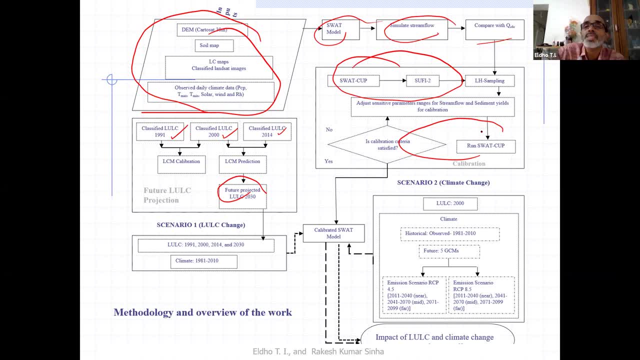 we use for the calibration important parameters based upon the pressure studies, and then we study like a scenario changes, only the lulc change. so, as i mentioned that, what is what is happening? and then there is uh, lulc, land use, land cover change, what is the impact? and then 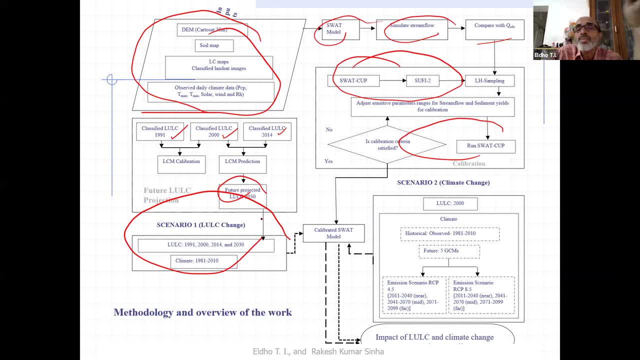 we study um the the scenario to the climate change with respect up to the only 100, what kind of like rcp 4.5 scenario, rcp 8.5 scenario, how the changes are taking place, and then we can also combine both land use, language change and the climate change together. what is happening? so this is the way the 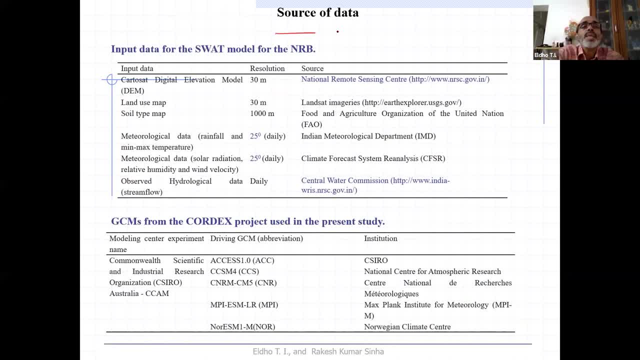 typical studies are carried out and here the source of data is already mentioned, like, as i mentioned, is obtained from cartosat and language map, from the landsat imageries, soil type data from nbs and fao- that also we used, and then material data in imd data we use, uh, and then um like, um, uh, the. 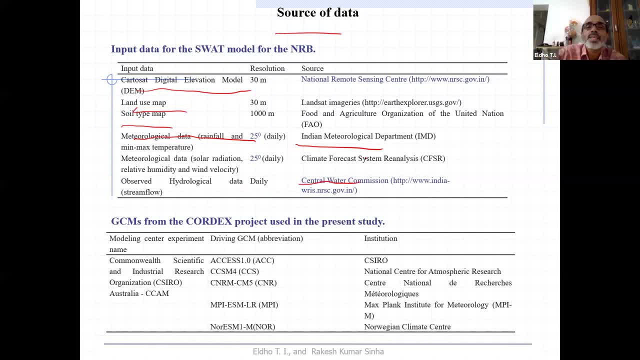 observed runoff data from central water commission, the rain gauge, river gauge stations and there are some of the gcms which is used by this doctors of the rakesh, is cortex data. so currently we are using other data but the early of the studies results is based upon cortex data. so cortex data and various 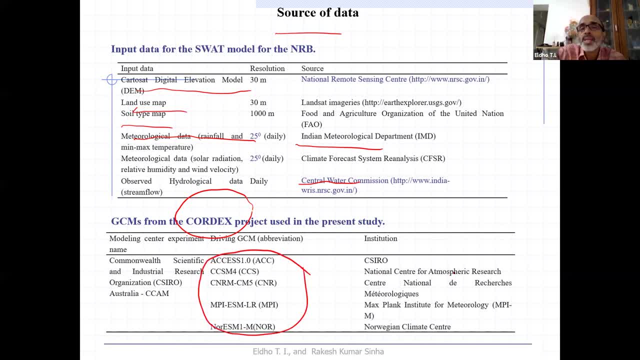 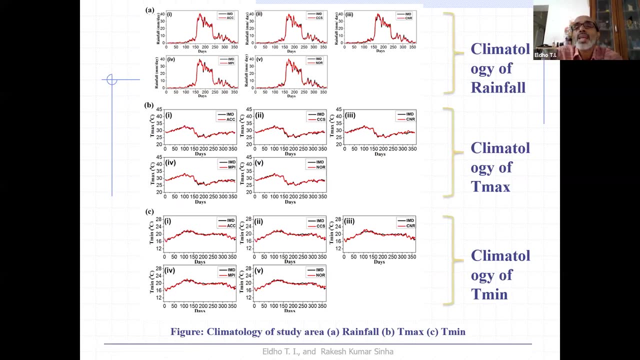 gcms used are listed here, like a national center for atmosphere research, ccs, m4, like that, cnrm, etc. these are the gcms which are used for uh, the studies here. so then, as i mentioned that um, we need to see the, the climatology of the rainfall, climatology. t max, t minimum, maximum temperature. 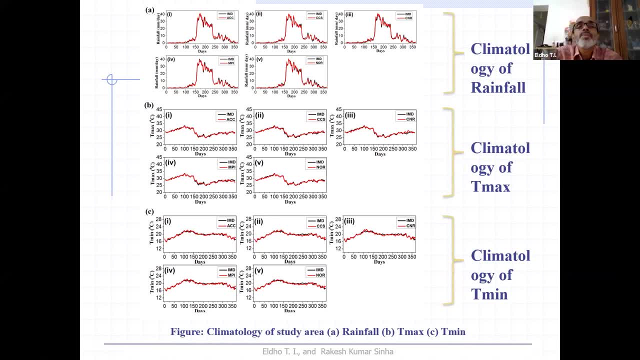 minimum temperature. so these all holistically, we need to assess by using the past data: uh, so now, uh, and then also from the gcms, uh, those data we need to see. you see that, whatever the data coming from gcm, since the statistical downscaling, we need to see that we. 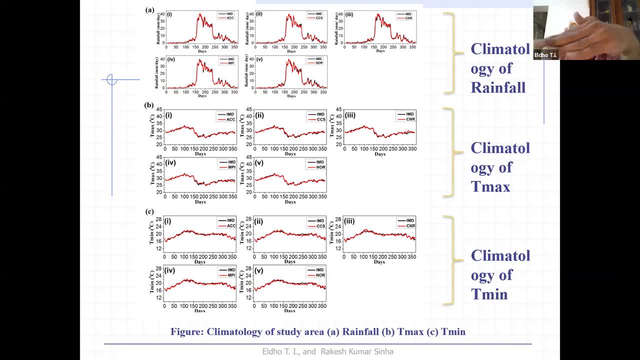 need to do some bias corrections and then uh see that it is matching with the historical, then only we can go for uh further projections as far as these uh hydrological parameters are concerned. so this shows like a climatologist area- rainfall, t max and t minimum- how the variations are taking. 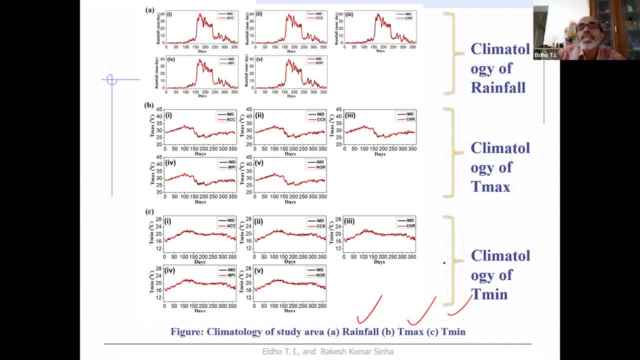 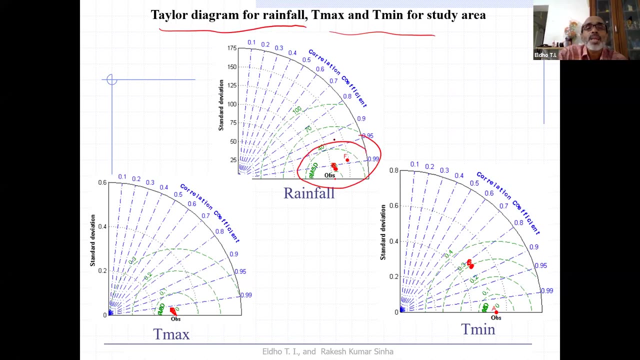 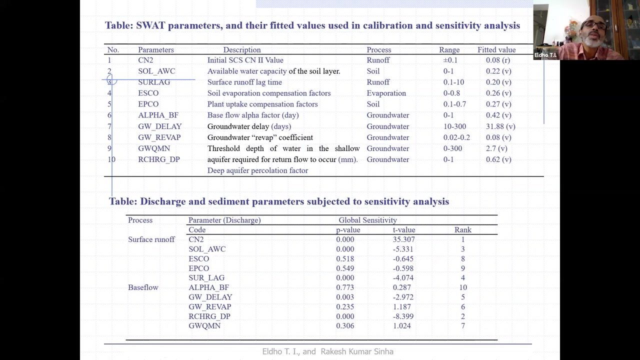 place Kelly. mandatory индinum has two model around 32 parameters are there. so some of the important parameters. you see the available runoff estimation from the cwc sites are shown here and here the parameters. i don't want to view it further. you can look into that. and then the fitted values are obtained based upon the. 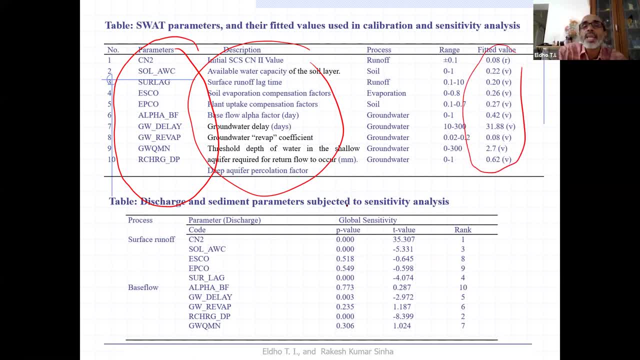 calibration, and then we started sedimentary studies, also carried out in this river basin, and the publication, the paper which i mentioned. all these data are available and let you determine parameters, like various parameters are listed here, and then running of these parameters is done and then, accordingly, the model is developed and then 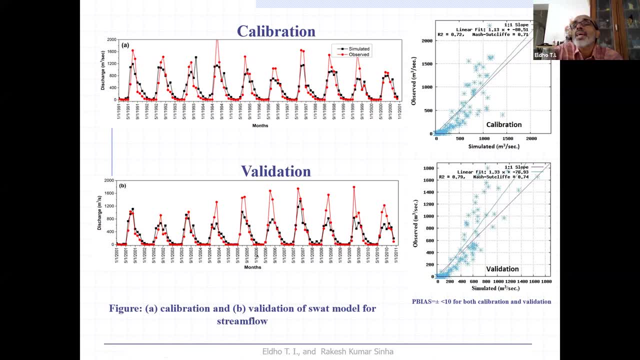 here. this shows the calibration. so of course you see that we will not get whenever we are doing, starting from 1991 to 2001- 10 years that is used for calibration, and that you can see that there is a. the peaks are not the type drawing the model, getting peak is so difficult, but 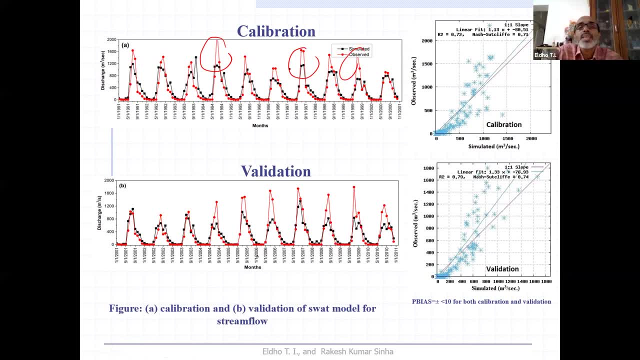 you can see that there is a good match around 0.79 or 0.8 um nsc coefficients, um variations obtained, which is found to be very good. so you have to point 871 for calibration and then further. we used from 2001 to 2011. 10 years ago we used it for the validation of the model. so there also 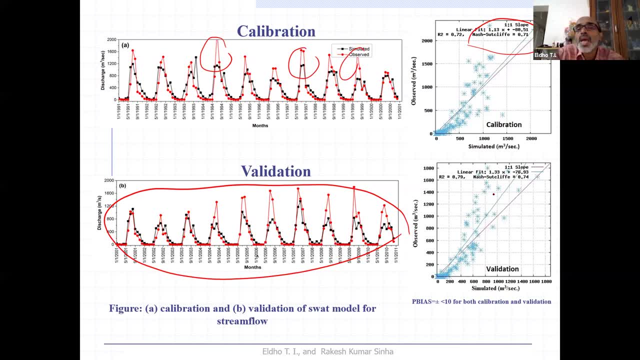 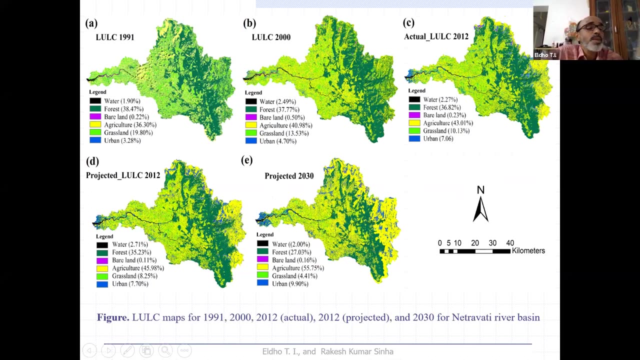 we. we got reasonably after 0.79, and then nsc coefficient almost 0.7, etc. and that way we calibrated the models and then validated and then, as i mentioned here, a land use. land power change is very important as far as hydrology is concerned, so using landsat. 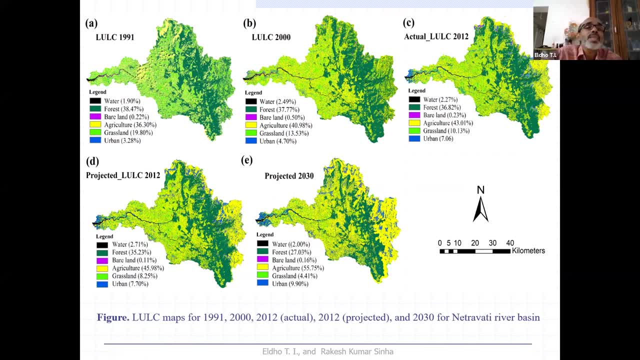 data. we analyzed. what is the, what is happening in the river basin, netra river basin. so this shows elliots in 1991, 2000, 2012 and then here you can see that the 2012, 2030, etc. so we are using so here. 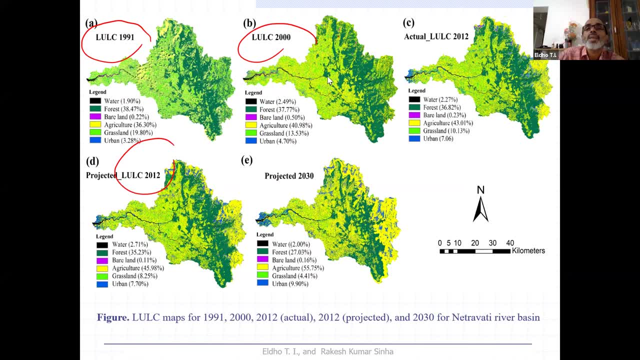 up to 2012, uh, so we are using the data for um, uh, the, the, what is happening in the, the historical, and then we are projecting 2030. so, though i am showing only up to 2030, we we have projected 2450, 75 and. 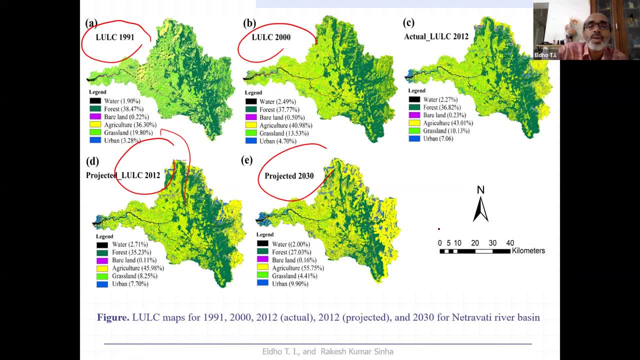 2100 as part of this project, and the results are available here. i am putting only up to 2030.. so that way, uh we we get the variations using land change model as far as land use, land cover is concerned. so here you can. one important aspect is land use, land cover is considered, so here you can. 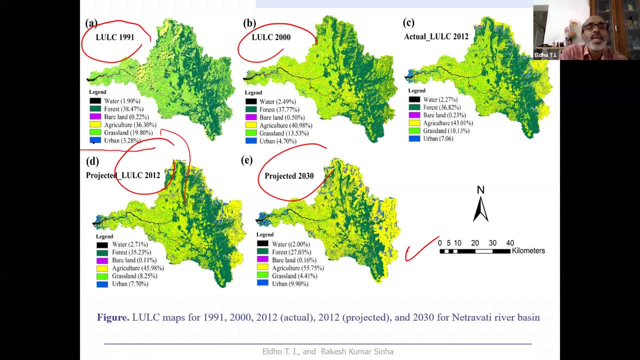 one important aspect is land use. land cover is considered, so here you can. one important aspect is: in 1991 the urbanized area was 3.28, then it is increasing to 4.7, then by 2030 7.06 and then uh. 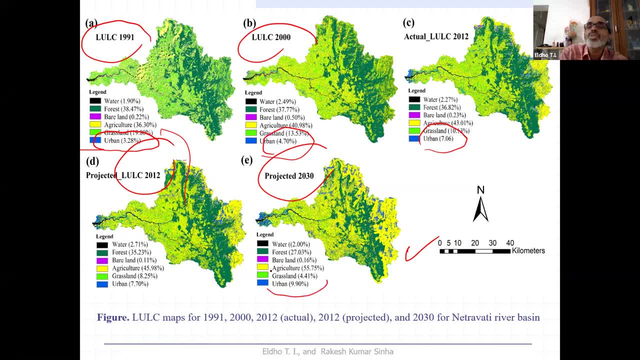 say another 10, 10 years, it will be going to 9.9. so this is people increasing, and then that is especially organized flooding, how all those things can take place. and here this shows the spatial distribution of change of the surface runoff for land cover, map 1991 to 2000. and you so, in comparison with the 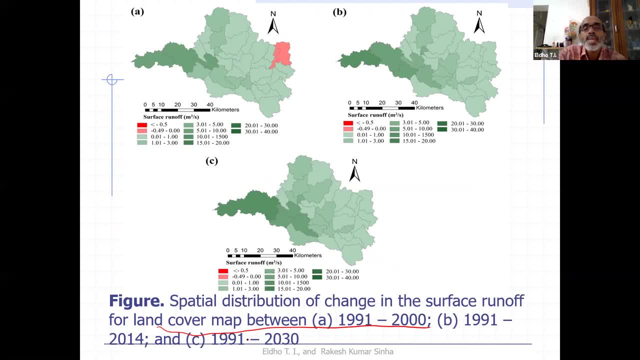 1991 to 2000, 1991 to 2014, 1991 to 2030. so this is based upon the swat model and we we compared and how the variations taking place, so even atari basis, special variation- we are capturing and which hru is on which location. 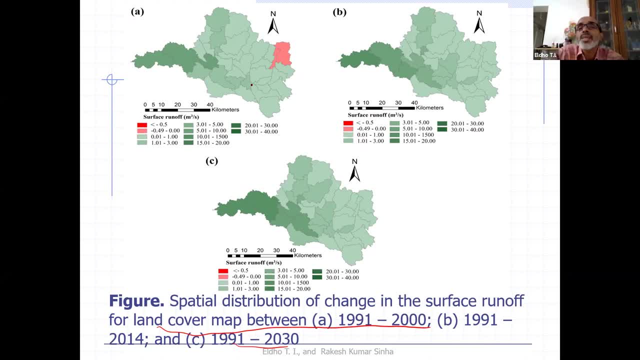 is severely affected. you can see that here. upper region is that much effect is not there but a lot of regions is much affected. we can see with respect to the runoff is concerned. and then this next figure shows the changes with respect to seasonal. you can see that. 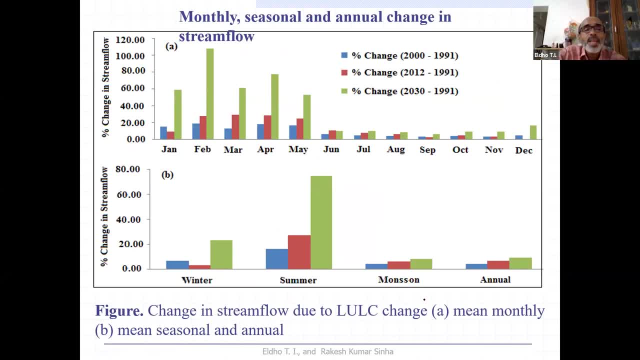 the change in the stream flow due to lerc change, with the mean monthly and mean seasonal you can see. so you see that this basin, especially the western, even summer rainfall is there, summer season rainfall is also there. so there you can see that, the summer, the rainfall. 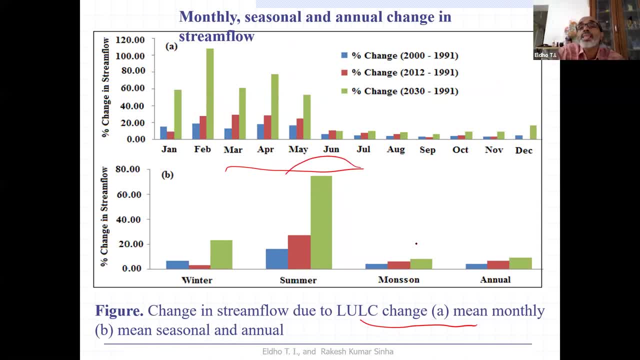 is increasing and runoff is also increasing and monsoon actually there is a small changes only observed. so that is, uh, what you can see here with respect to percentage change. so but, um, starting from march, april, may, this season the the effect, so, but please understand that the summer 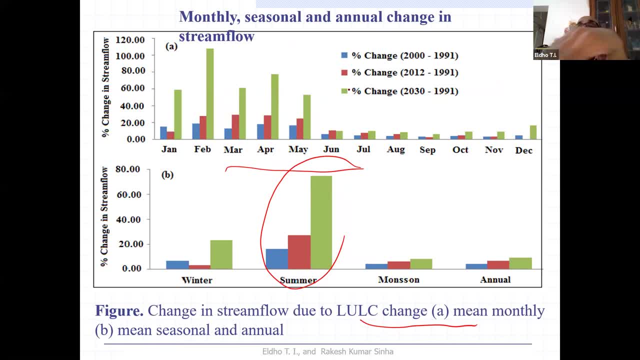 this is increasing, but when the further monsoon comes this will be caryo carryover effectively there. uh. so here that is due to that impact. you can see that as a type of care Lafr Fuk tinha. there was severe rainfall during the summer season, like march, april, may, and then whenever the even. 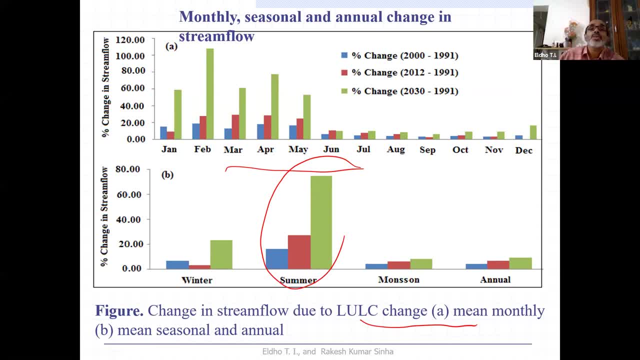 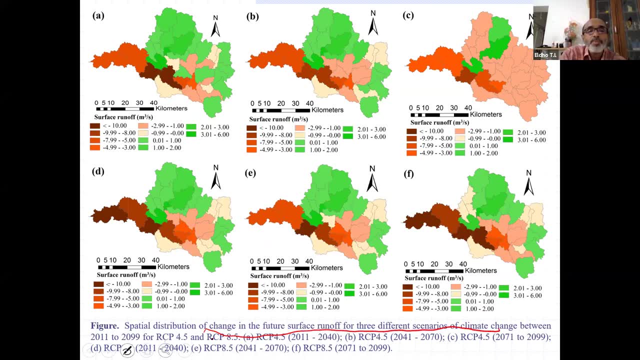 rainfall and spreading phase space, so that you can see these kinds of phenomena and this shows the spatial distribution of changes in the future. runoff for three different scenarios, like rcp 4.5, 8.5 with respect to 2011 to 40, 2041 to 70, 71 to 90. by using it to 2030, um lurs changes and then like: 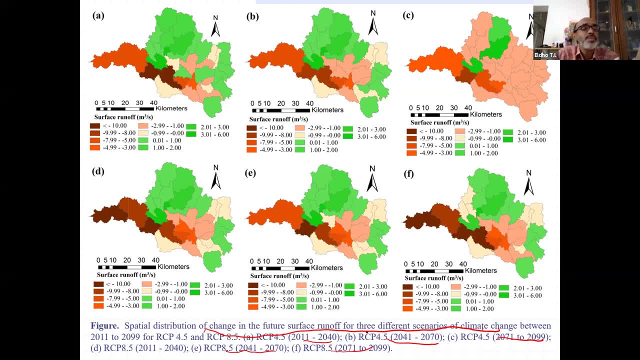 various time sizes. so i mean, there is no time, therefore, to explain all those things, but what is the way we do this climate change impact? as far as hydrology is concerned, we take various scenarios like rcp 4.5, 8.5, and various time slices are taken and then, based upon that, 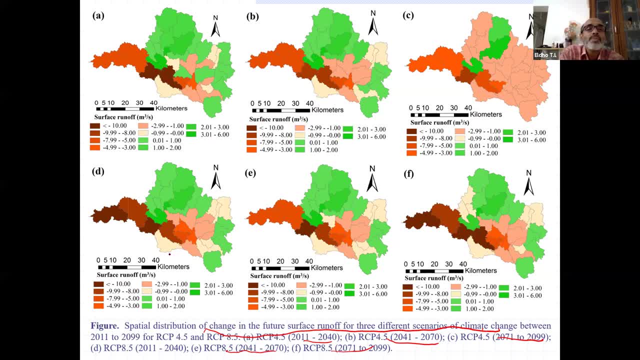 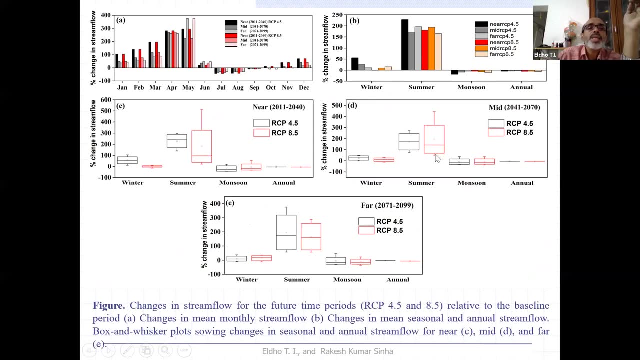 we see how the variations are taking place. so you can see here the surface of variation, and so some part is severely affected, some part is less affected. so then, rcp 4.5, 8.5- how a typical kind of studies can be done. that is the purpose of uh projecting uh these slides here. so now, 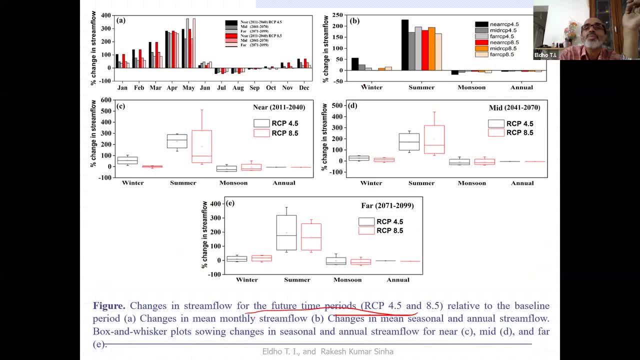 then this shows the change in such stream flow for rcp: 4.5- 8.5. the situation, how the changes. you can see this black indicates 4.5 and this shows 8.5. 8.5 means it is severe variations. you can see. 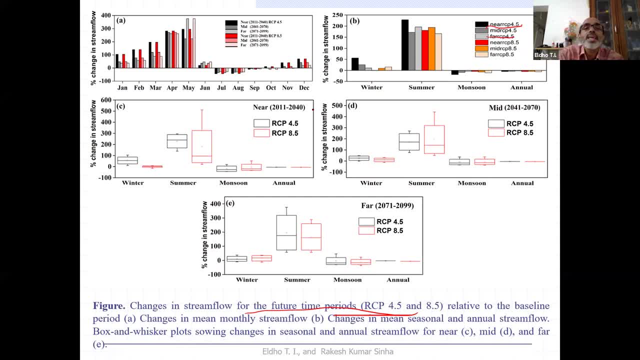 depending upon the monthly and depending upon the season variation, and then we show the box plots correspondingly with respect to 4.5 and 8.5 and how the behavior is taking place, so that way we can see with respect to the various time slices and then 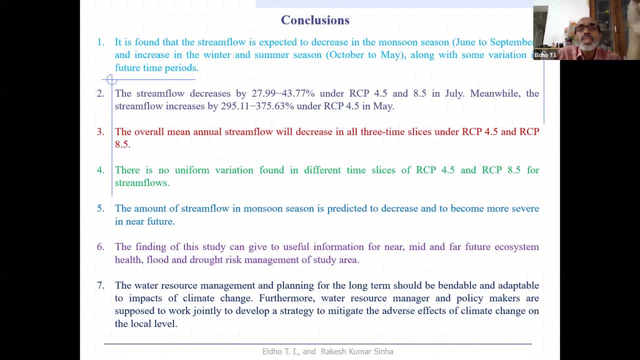 aspects are concerned. so, finally, based upon this case study, what are the conversions? it is found that the stream flow is expected. this is not overall conversion, but a particular river based is concerned. it is found that stream flow is expected to decrease in the monsoon season, but increasing the summer season the stream flow uh decreases. uh, this much percentage in 4.5 and 8.5. 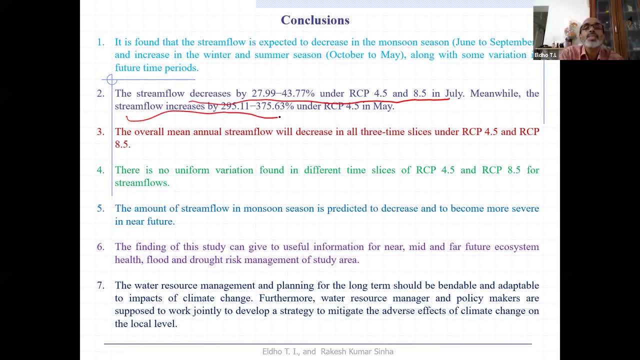 about uh 50 percent in july. stream flow increases by two to two to two ninety five uh percentage. i mean large increases of in the summer season and overall mean annual stream flow will decrease and there is no uniform variation found in different time traces with the rest of the 4.5 and 8.5 the amount of stream flow. 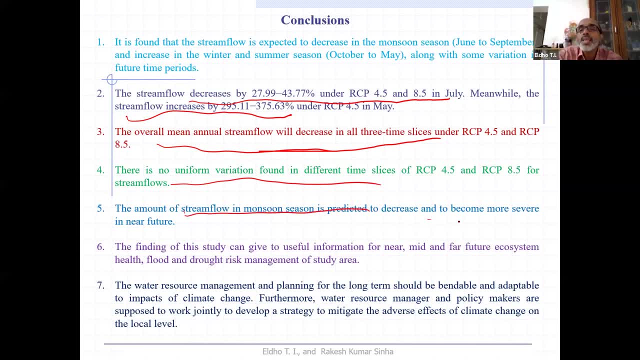 monsoon season is predicted and to decrease and become more severe in near future and finding this study can give a useful information for near or mid future or future ecosystem is concerned and these kinds of studies we are supposed to do for all river basins, and then we need to look at 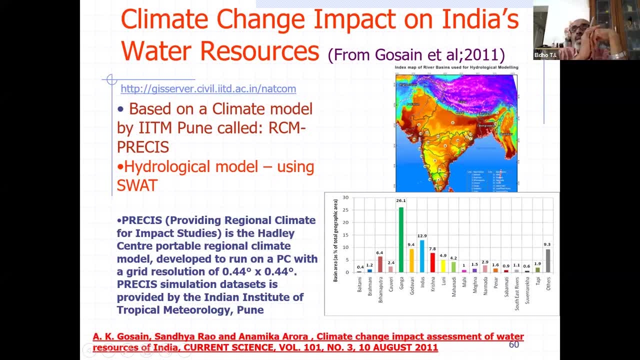 it and, before concluding, few slides i would like to show, based upon again these uh details fromIt was the Gossain studies in 2011published in some journal. uh, so you see that, again, this is also based upon SWAT model. they are used a regional climate model, so holistic. 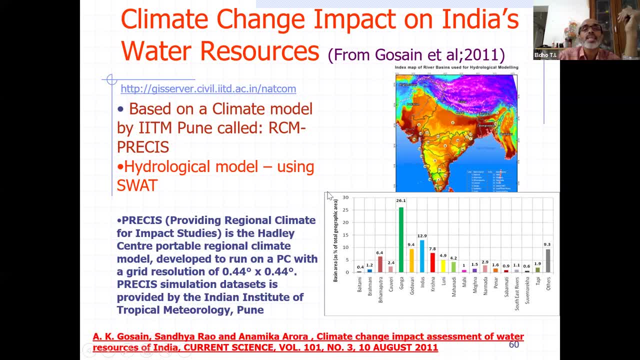 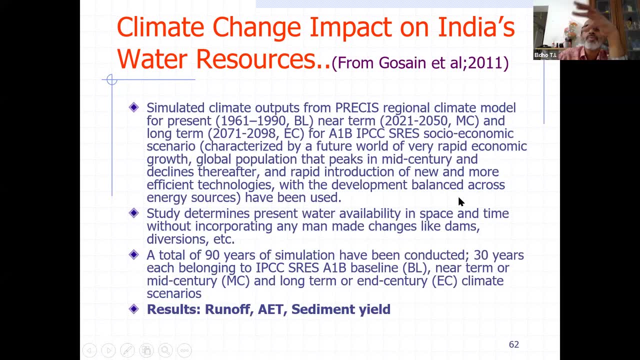 modeling studies. consent for entire india. you can see similar strength is concerned, so they use the precise. i don't want to go over the details since time is almost getting over. so very similar kind of scenario, but here existing see that it was at that time. it is a semi-three model. similar might be three models, so every. 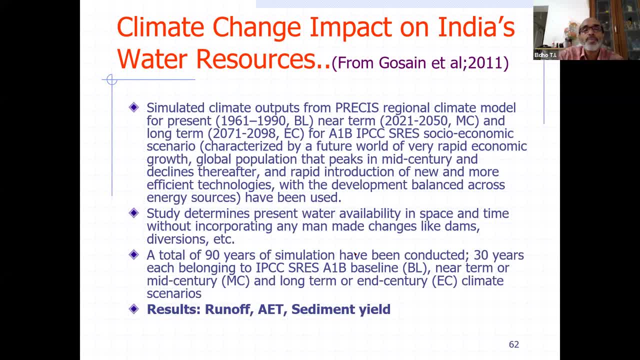 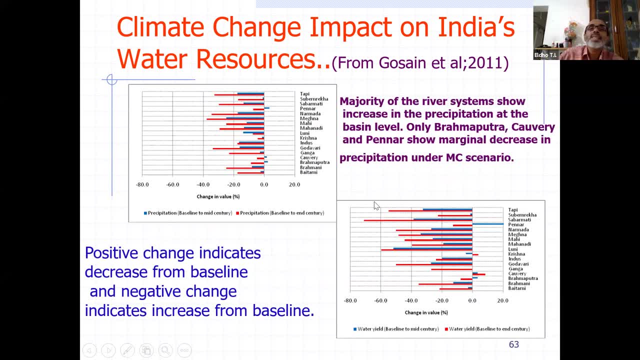 scenario you can see, uh, that kind of uh variations you can see then, because to run off uh, aet and sediment d. so here again that study is also shown a very similar kind of trend which i i projected earlier from the natural basin. so positive change indicates decrease from baseline a 90 change. 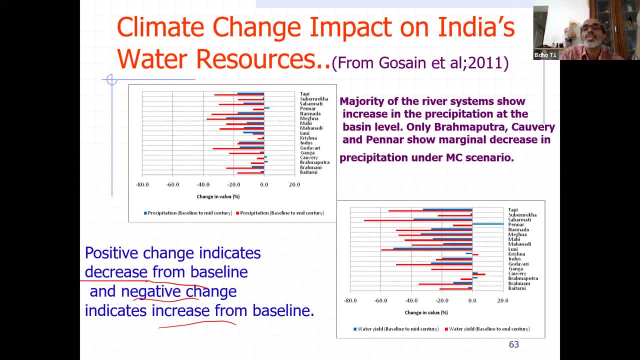 indicates increase from the baseline. so here see that the majority of the river system shows increase in the precipitation. so here you see that all over india's concern, only there is increase in the the precipitation and, uh, some river basin, only short decrease and here correspondingly, of course, rainfall is increasing. total runoff is concerned, this concept, it is. 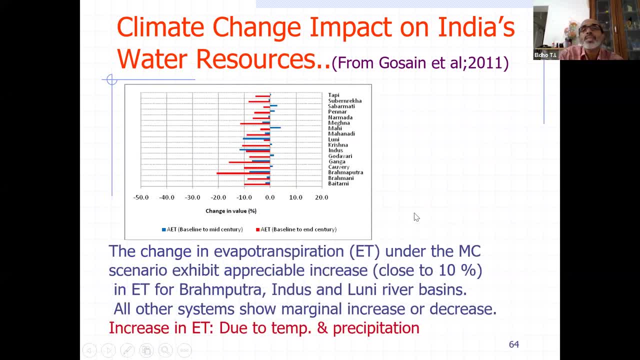 increasing and you see that with the changing evapotranspiration, of course the temperature is increasing. so this is based upon the science study. so you can see that here you see that the, the actually evapotranspiration with respect to that, is also increasing. uh, with respect to the the future, 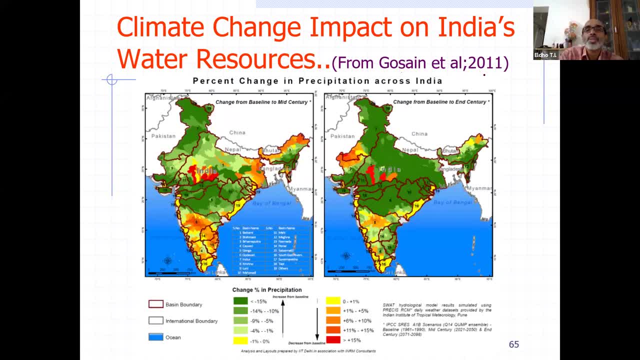 scenarios are concerned. so this is again. i have taken from the science for all over the whole our industries. my research team has not conducted so, but i have taken from this to just to share the details with you, those who are going through. that is this. one paper is there published in current 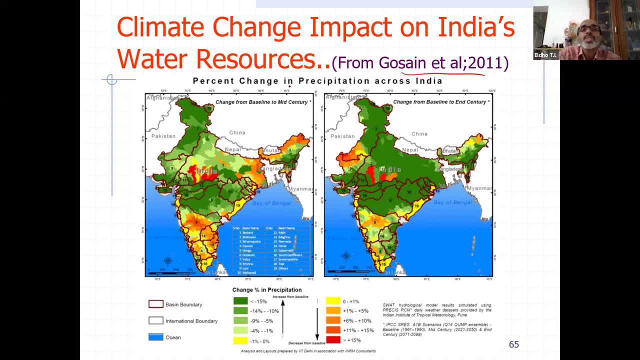 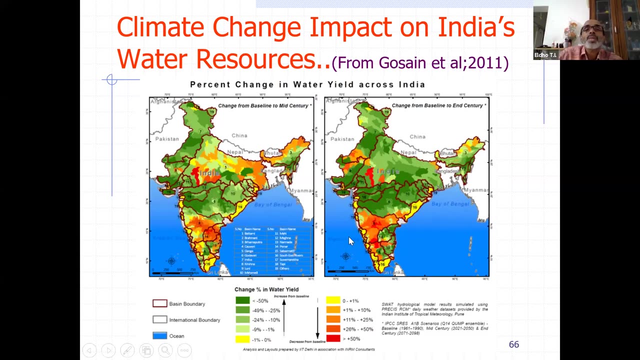 science. so here you see that the change in pattern with respect to present a person, changing precipitation across india. so that is uh. this green shows it is increasing and uh, red shows the decrease, the decreasing trends and increasing trends you can see here, and then simultaneously, similarly, a percentage in water yield, also obviously with respect to rainfall, you can see. 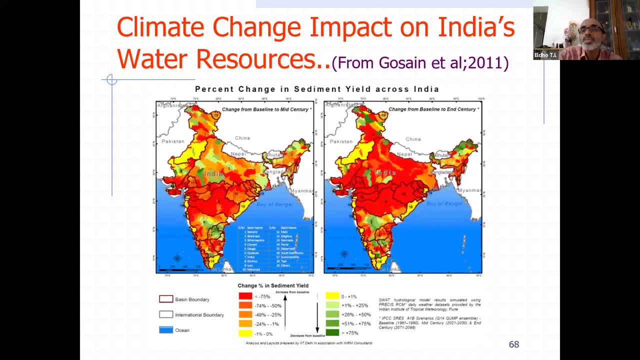 and then evapotranspiration and then the person is sediment yield. so you see that one important study is that whenever rainfall test space, severe rainfall test space, so that way the sediment will be increasing throughout the country. with respect to the, the future scenarios up to 2100 is concerned, 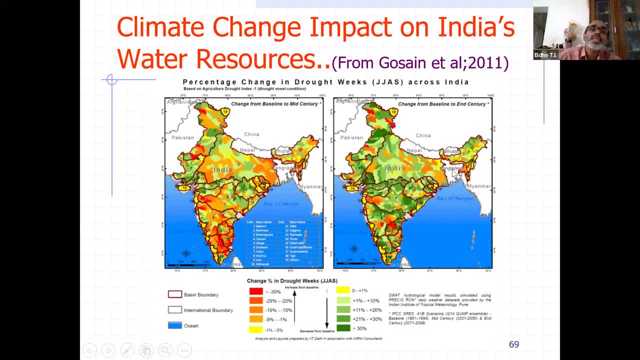 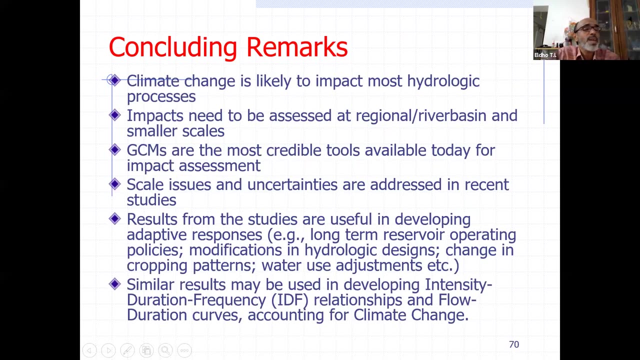 so that is, uh, the studies done by uh professor gosan team. and then, uh, these are also increasing, as i mentioned, when the rainfall space- it happens in few events- and the the many, many areas, the drought situation also, uh, increasing. so, finally, to conclude this lecture, though i have just crossed, 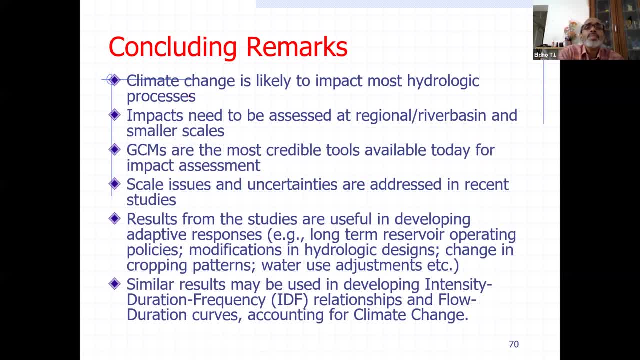 the five minutes. i'll be just quickly concluding. so climate change is likely the most hydraulic process. so that is very we can feel it, we can model it, we can do. we can last a few years, or even six years, which we are going to be doing even in the next few years, that's, and we should. 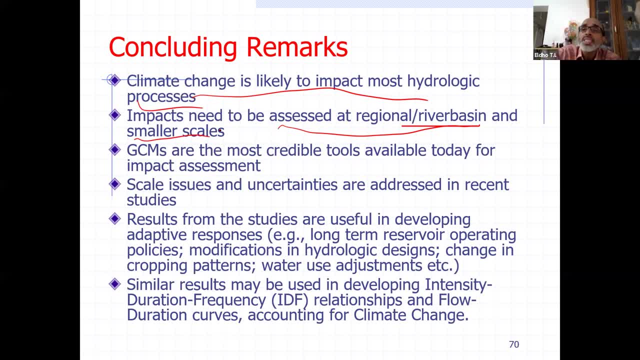 be able to go down to a much more effective schedule. but it is. Monte Carlo is going to be very, very difficult to come to very, very rapid planning. it may be very difficult to uh model it, but in our case we have a very, very rapid planning and this is going to be. 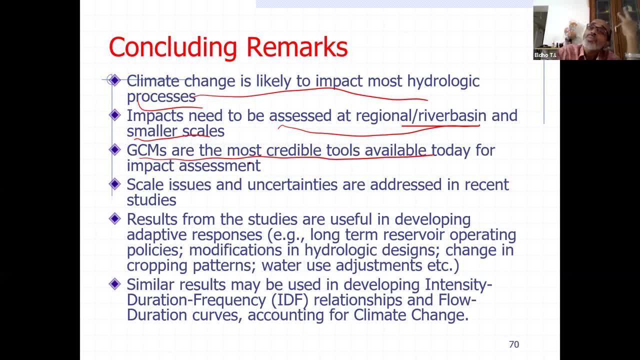 very, very sensitive, so that this is true for the the whole of the country. and the technology is going to be very, very flexible and therefore we need to have a slow and flexible planning for the different kinds of water, so that the climate changes and we can be able to have 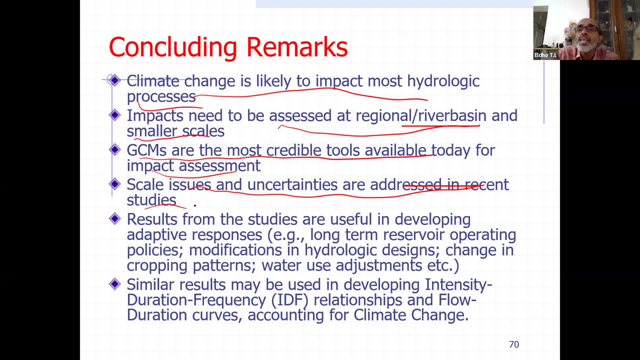 like the statistical downscaling, dynamic downscaling, all those things can be done and then get a better perspective And results from the studies are useful in developing adaptive responses, long-term or short-term- like that we can look into And similar results may be used for developing. 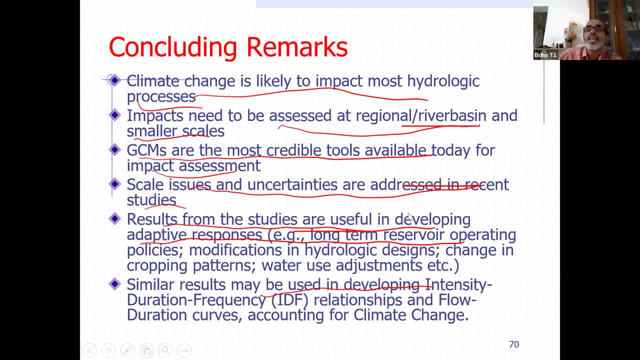 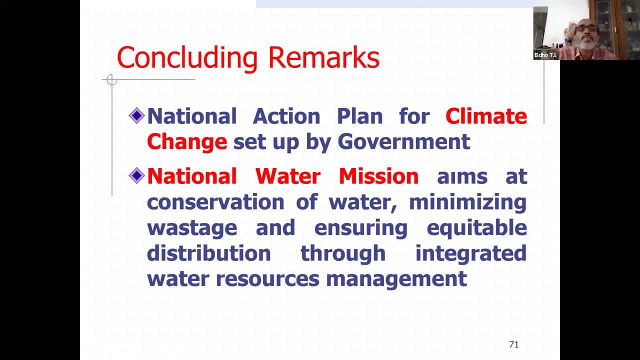 idea of goals for the future. So, based upon these studies, we can make it. and then what will be the impact we can assess. And then many of you know that Government of India started National Action Plan for Climate Change, and then there is a National Water Mission. 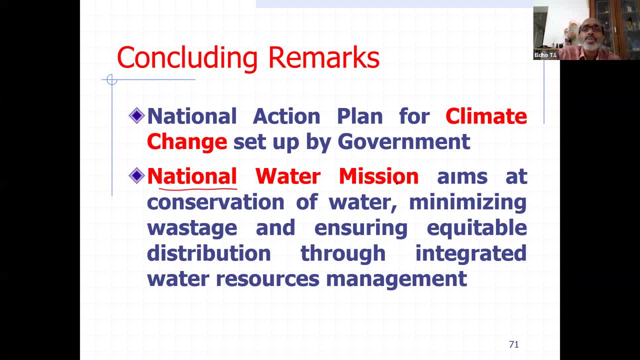 under Ministry of Water Resources, or Jalasekti, is there. So the purpose of it, like a conservation of water, minimization of wastage, ensuring equitable distribution through integrated water resource management, So this is very important actually. Professor Goran Deewar and his team. 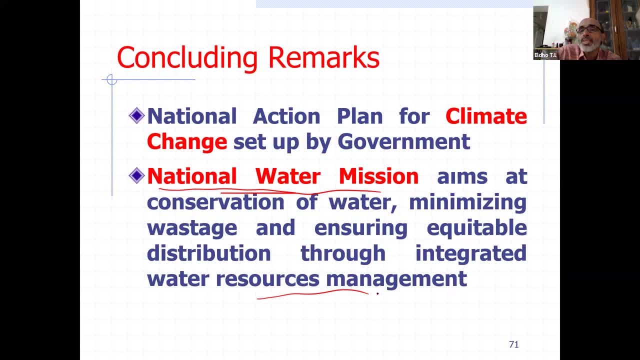 or most of the agricultural team said. we are need to look into the irrigation demands, whether, how much we can decrease, how efficient irrigation can be done and whether we can so now currently around 75 to 80% water is used for irrigation- whether we can decrease, reduce that. 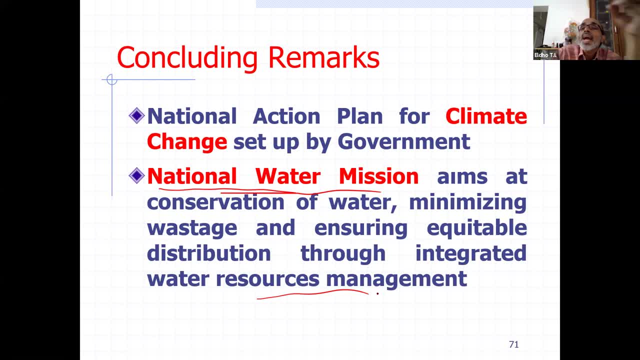 to 50%, So that all of our water scarcity can be decreased, and the per crop, per drop of water, how much efficiency, efficiently, we can utilize it for the increase in crop production. So that is what we need to look into And then, under the National Water Mission, 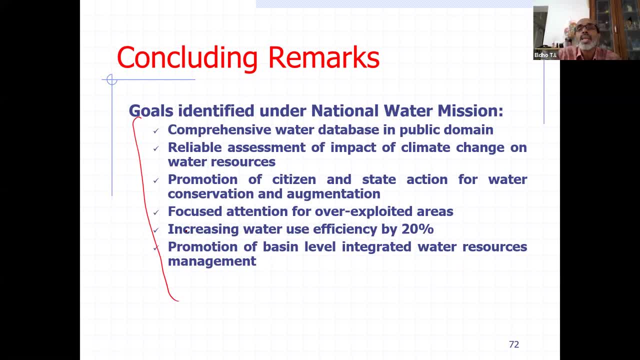 some of the important aspects which are listed, like water database, in public domain. So that is now happening. So most of the data. all researchers hearing me, you can see that through hydrologic project, various protocols, we can download the data. It is 10 years back. it was very, very difficult. 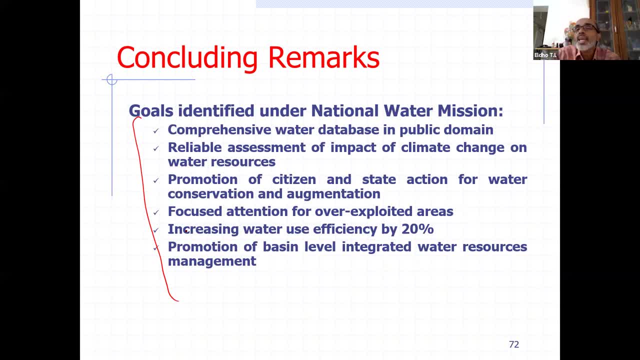 but now it is much easy And then, like you said that it is readily available, with ISRO or as a space application centers, it is readily available And then we can go for reliable assessment of impact of climate change part of the system. So like a very sophisticated tool, like a SWAT. 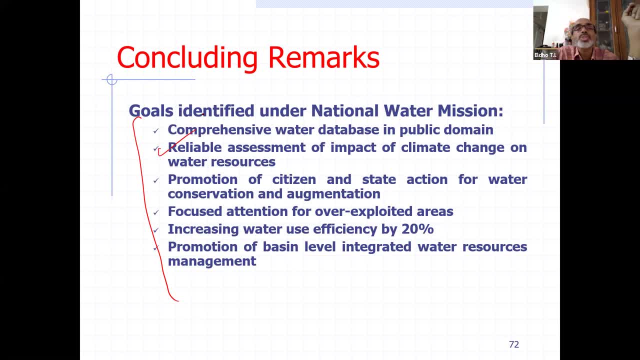 or EIC models are available and even each open source is available. So, researchers or the students, you can easily utilize it. Then promotion of citizen state action for water conservation augmentation. So we need to go for, like water management, rainwater harvesting. 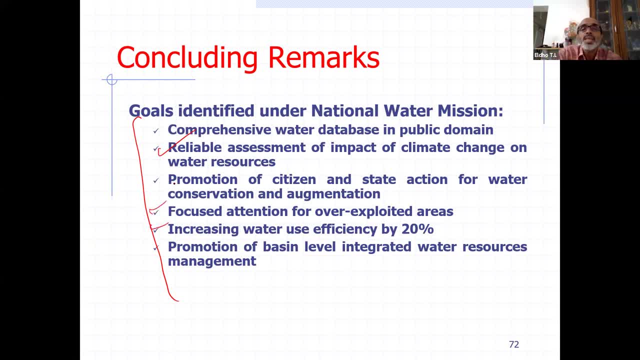 then focused attention for over-exploited areas and increased water use efficiency. So this is very important as far as agriculture sector is concerned. Then promotion of basin level in near to water resource management, That is, we always advise for the near to water resource management available. 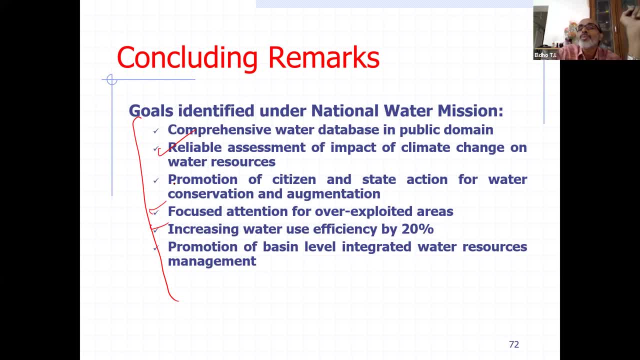 We need to first assess how much water is available And then, based upon that, for what are the various- you know- uses, and then where we need to decrease, reduce the usage for agriculture purposes, And then we go for integrated water resource management. 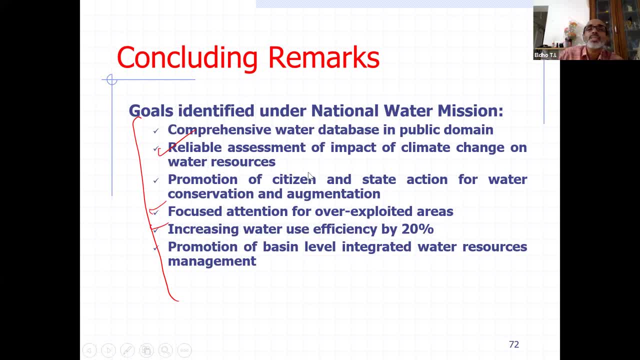 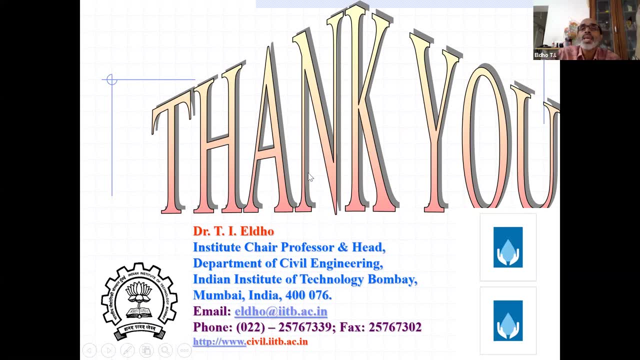 with respect to surface water and groundwater. So that is what we need to look into. So that way we need to go for integrated water resource assessment and management. So with this I'm concluding here. So if you have got any questions, I'll be happy to answer. 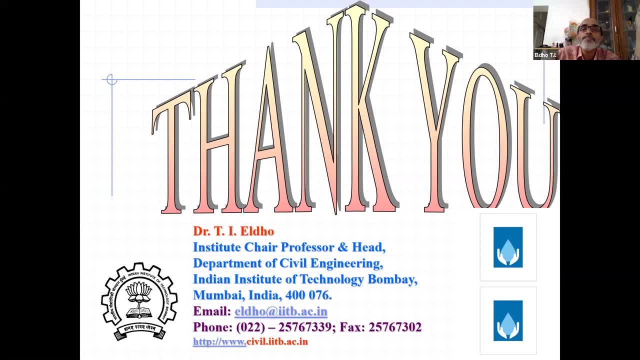 I'm very thankful to Professor Gurandeva, Professor Shinde and their team for inviting me for this lecture And I hope all of you got a glimpse of what are the issues, what are the problems to be addressed and what are the research needs in this area. 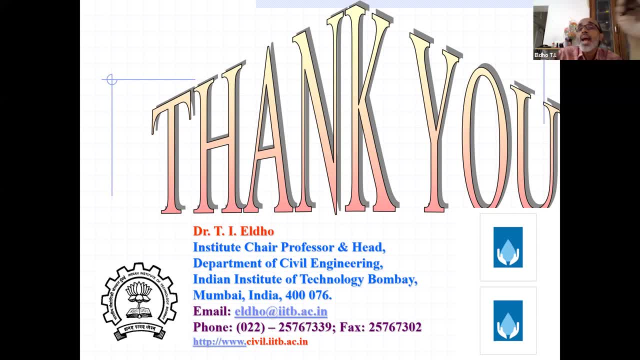 and how the hydrology model or water resource modeling, is very, very important and how we can contribute as a water resource engineer or an agriculture engineer, how we can contribute in all these studies. So with this I conclude here. Thank you very much. 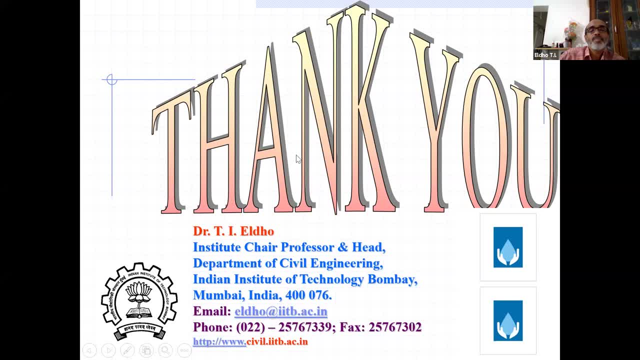 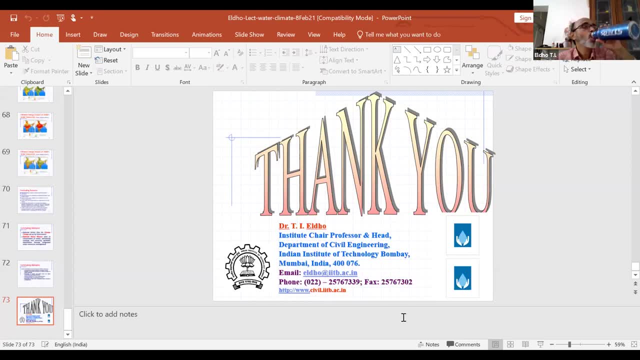 Yeah, thank you, Professor Aldo. In spite of your meeting schedule, you are deliverable. You have a very nice lecture on hydrological modeling and its impact and impact of climate change. So there are a few questions in the chat box. 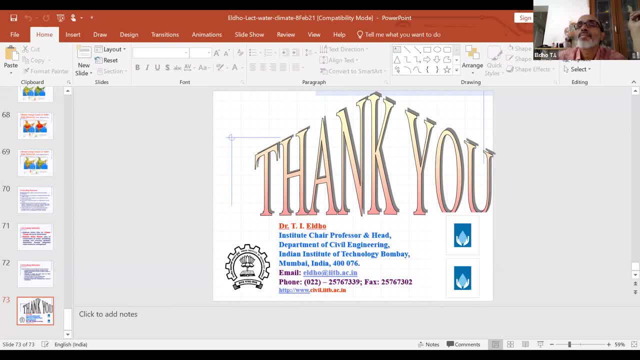 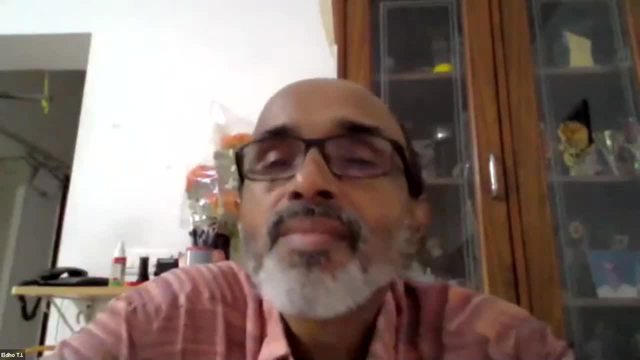 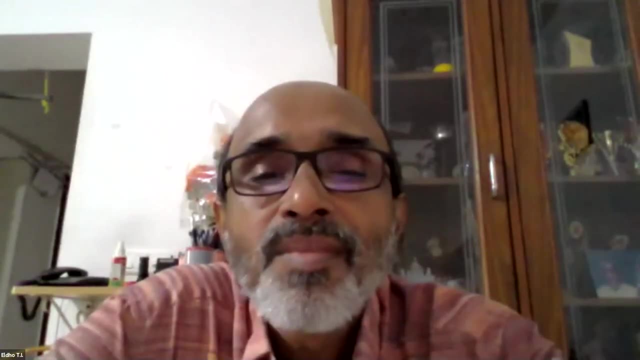 Can I take? Yeah, yes, please, Yeah, thank you, sir. The first question from Professor Ajay Singh. Many research papers have been published on hydrological modeling during the last 20 years in India. Based on your experience, which hydrological model? 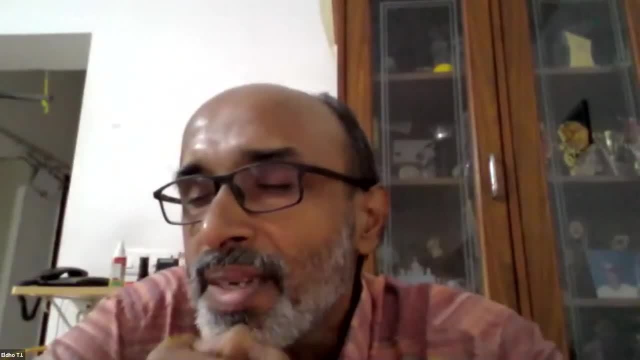 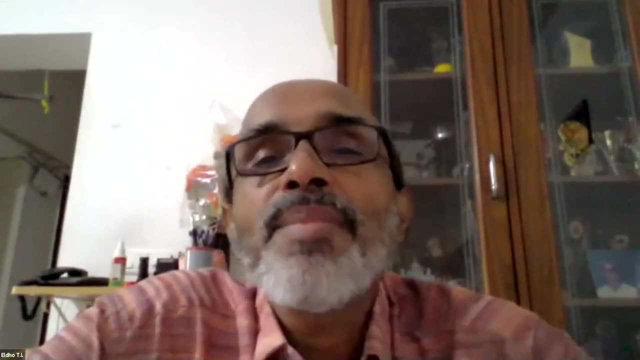 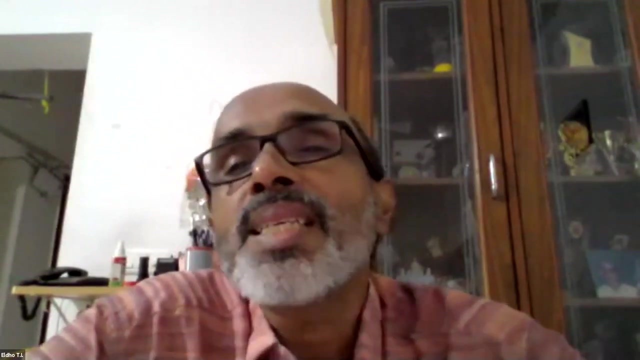 you find applicable in field conditions? Right applicable, Which one? In field conditions? of course, as I mentioned, this climate change impact is concerned by type to all. the aspects of models seems to be very useful. And then if you're going for flood kind of simulation, 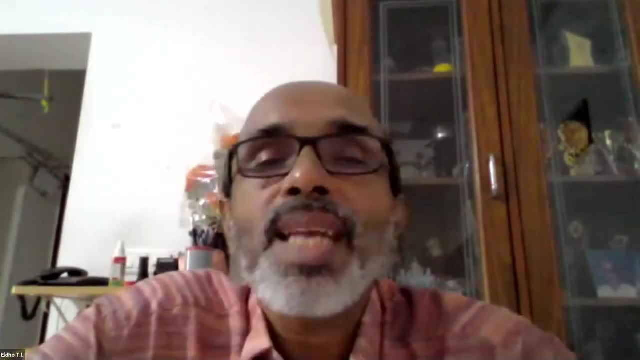 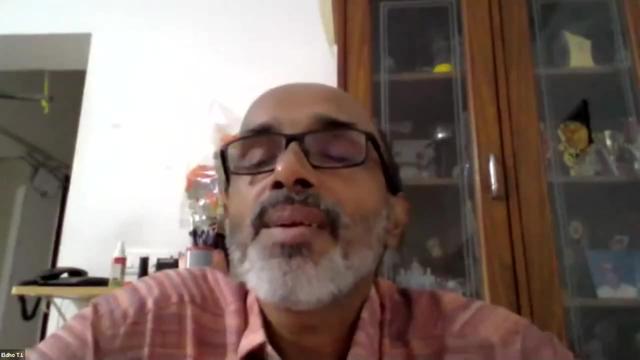 even to open sourcing, like HGC, HM, HGC rice. all these models can be utilized. but then if you are looking for a very specific video, very intensive modeling- that the Mike models- we can use it, but that is a paid model, so we need less time. 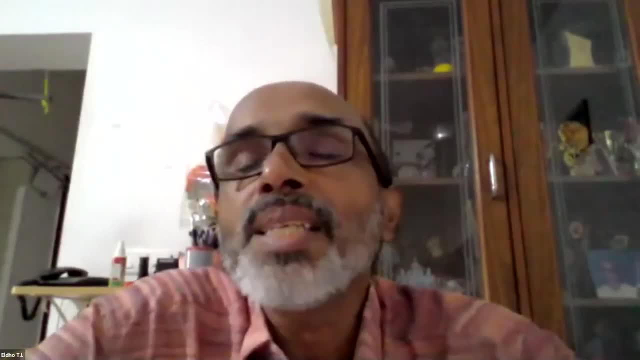 But that can be for at least, and that is for the goal here. All right, then take questions, you can use these, You can do so. Start, And then we have another complaint so I might tell you what the� to look into that kind of models. Otherwise, the SWAT model can give you many of the required. 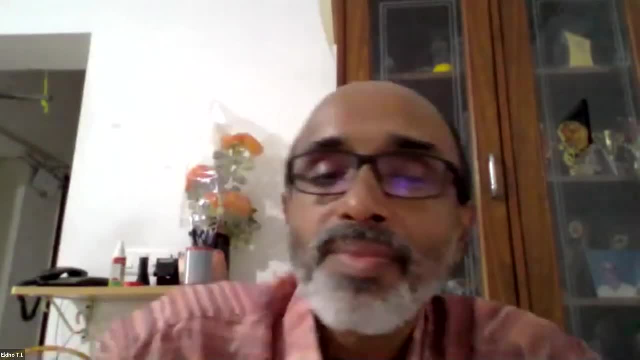 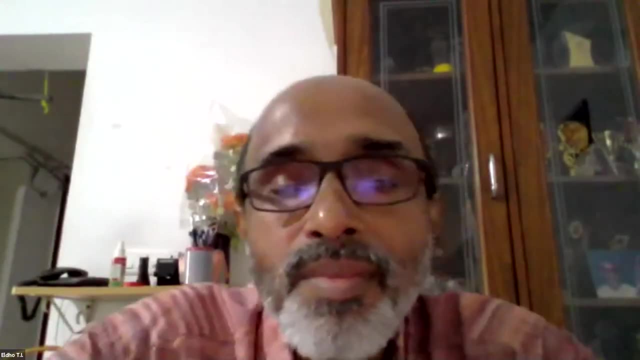 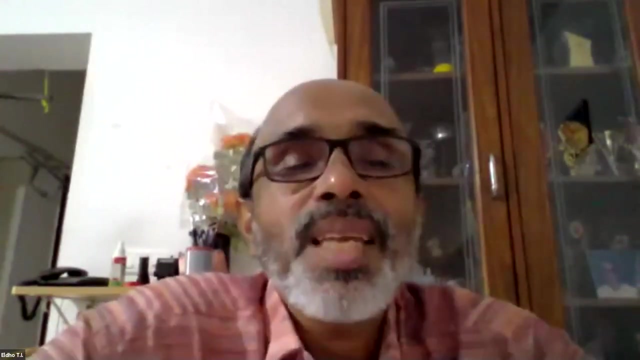 data as whatever we need to look into. Okay, Thank you, sir. Next question from Dipesh Machivar: In absence of observed runoff data, can hydrological modeling be developed and used to estimate runoff in an un-gauge catchment? Of course, observed data is very, very important. 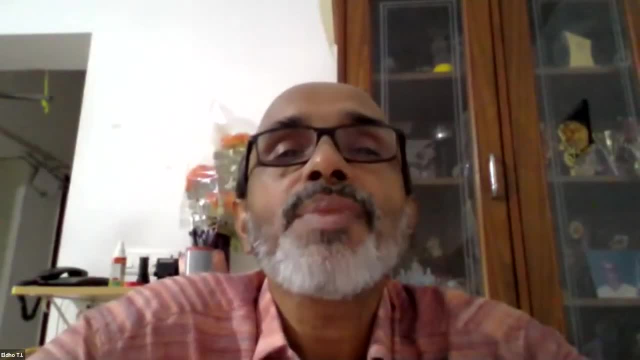 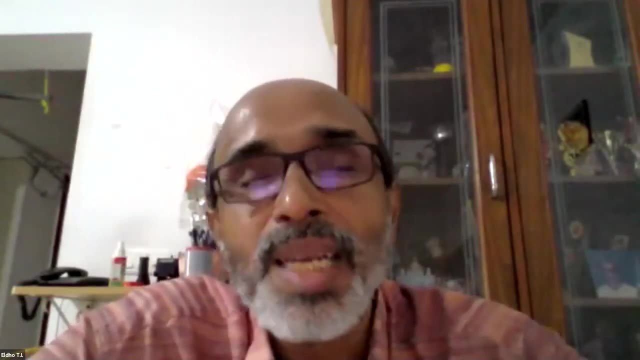 But now, as I already mentioned, CWC has a series of measured data and that is in their portal. It is available, So that way it is not so scarce. Of course, wherever we need it, it may not be available, But whenever we are developing a model on a river basin, 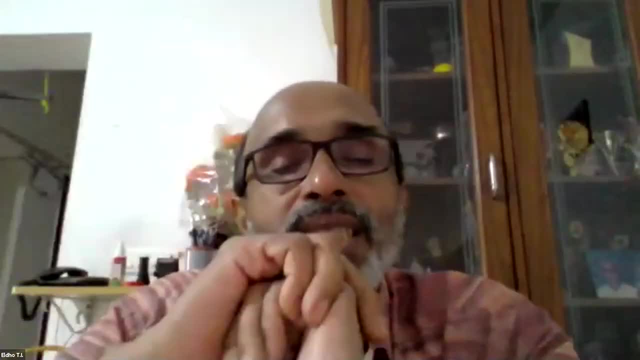 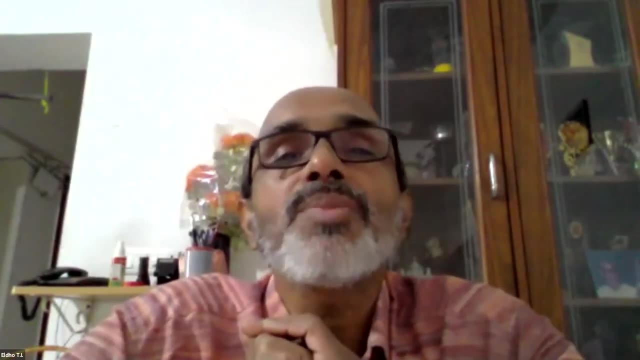 scale, then at least one or two gauging stations will be available in that river basin. So based upon that, we can calibrate the model And then, once you prove that, yes, your model is working fine, then you can extend your model to the area which you are calculating. 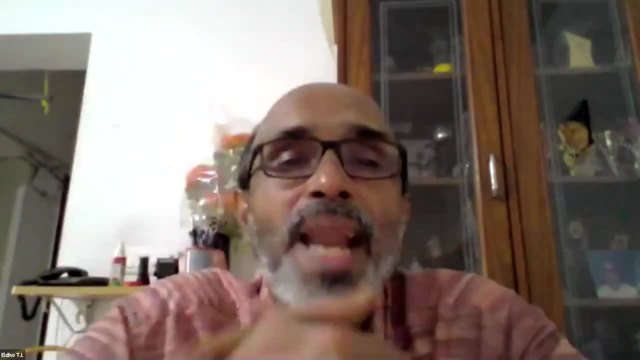 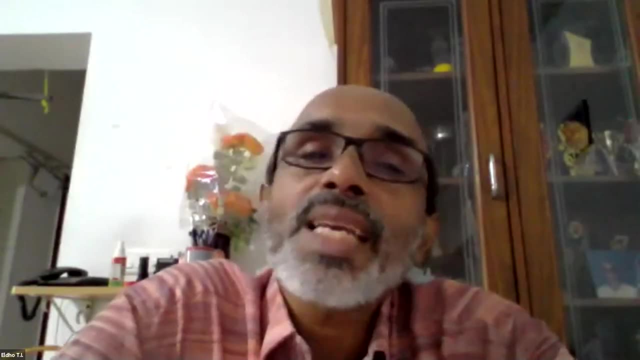 So, as you can see, that even SWAT model or BIC model, number of parameters to be calibrated. For calibration, of course the observed data is required, But we are lucky to say that now, all these generations of modelers, a lot of data is available. And then that with 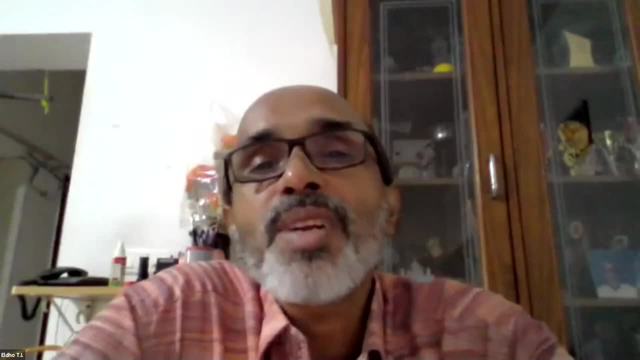 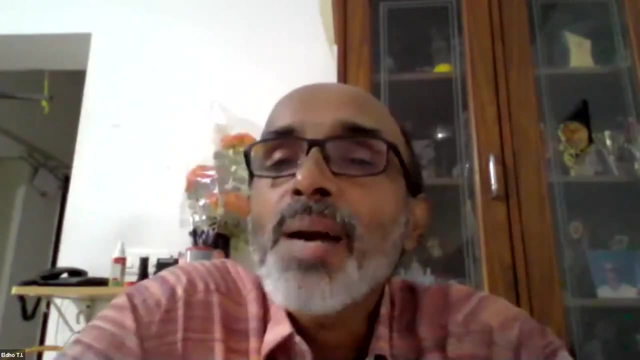 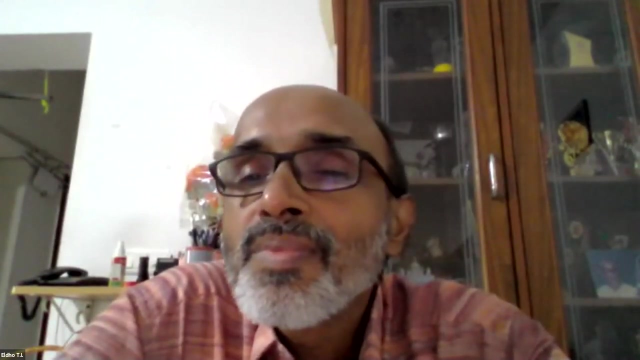 the hydrology project. as I mentioned, phase one, phase two are over Now phase three is going on. I'm sure that we have got a good feature with the data, where it will be much better later. Yeah, Okay, Thank you, sir. There are basic questions. I'm not going into that. We will answer them. 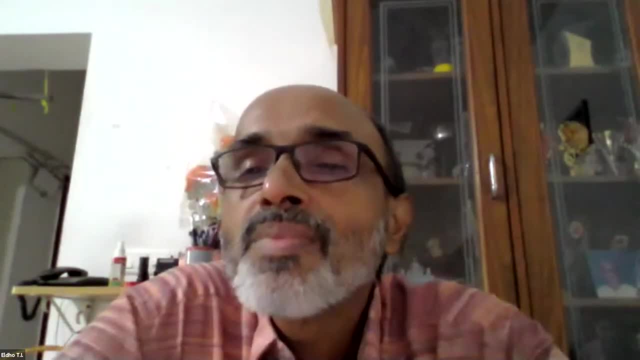 later on. The question is Dr Prasad, who is learning: Why do you think secondary data for designing technological models? How do you make sure that a future city can correct the appropriate school data? So secondary data means- I hope you may be talking about the subject data directly- what 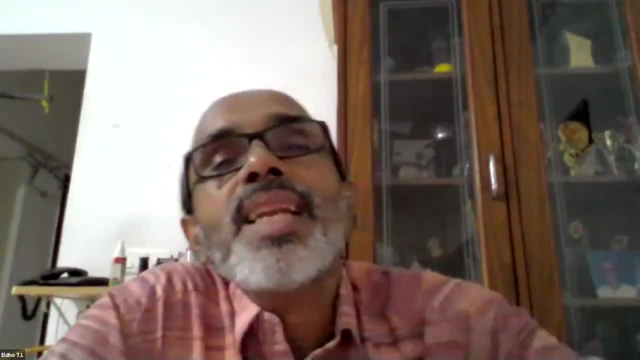 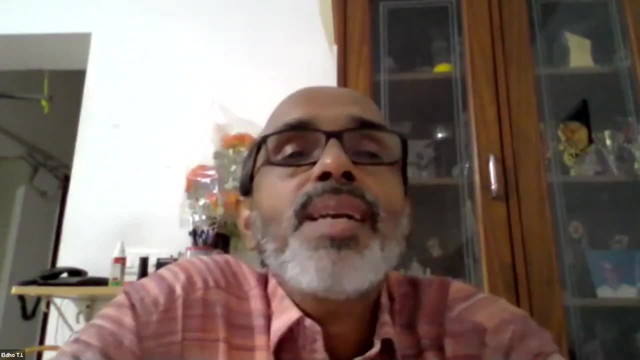 is coming. So it is secondary data, dot, field measured data. So secondary data, that is where we need to, also then, based upon the field measured data, we do there also, like you see, that one important area, what is now taking place, is called a. 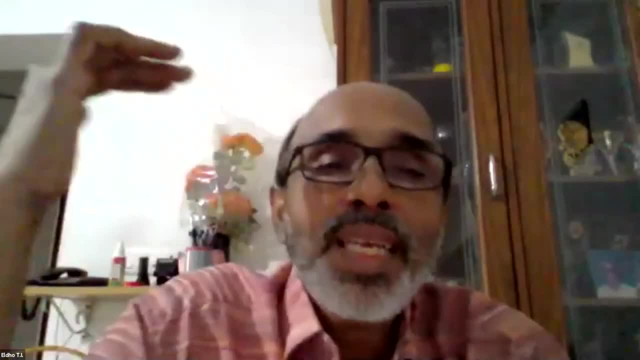 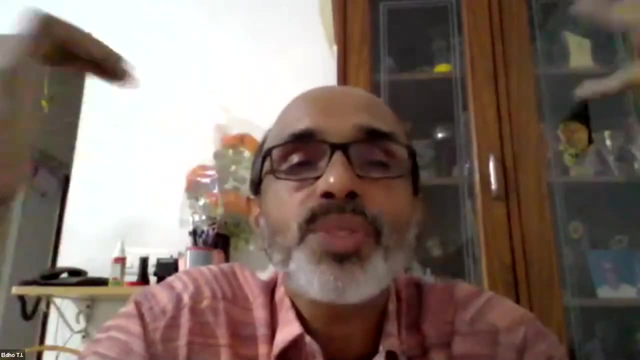 data simulation. So data simulation means with respect to the various satellite data that is available. So, with respect to available field data, we are comparing and then we, if we get a good match or to certain level with respect to past data, we are getting a very 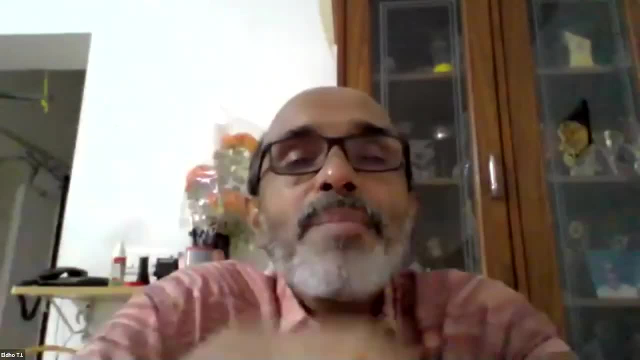 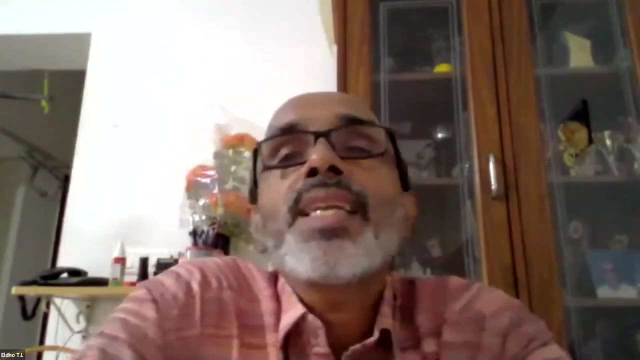 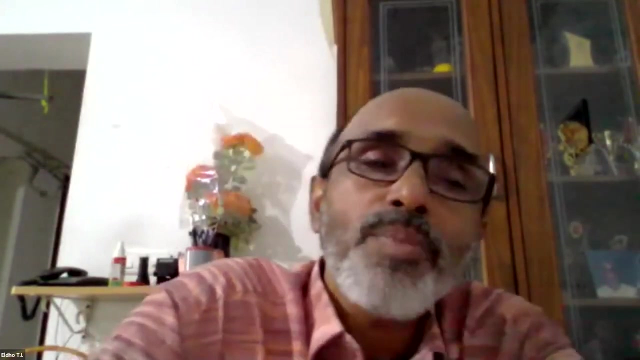 reasonable fit with respect to various parameters or consent, Then we can utilize that secondary data. So, for example, now even some of the satellites directly. you see that one of the most difficult part of this hydrology is getting the field data for the soil moisture, So soil. 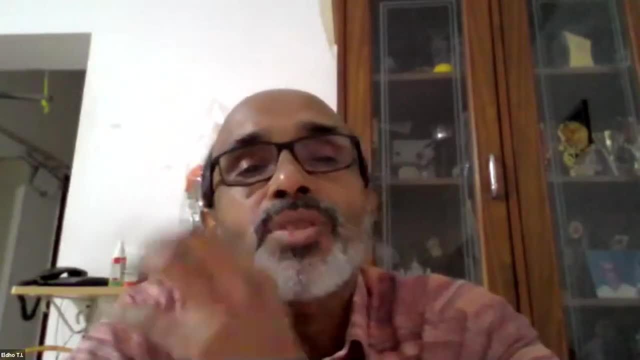 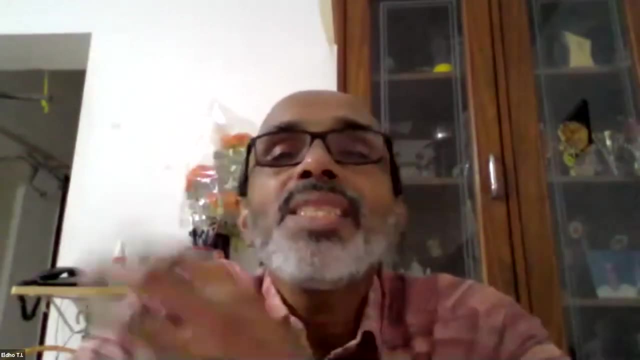 moisture is concerned, as all of you know that, even if you have some props or this thing, I'm sure that Professor Gaurandeepa and his team is measuring in various locations, But that is very, very scarce data is available, especially soil moisture is concerned, But then 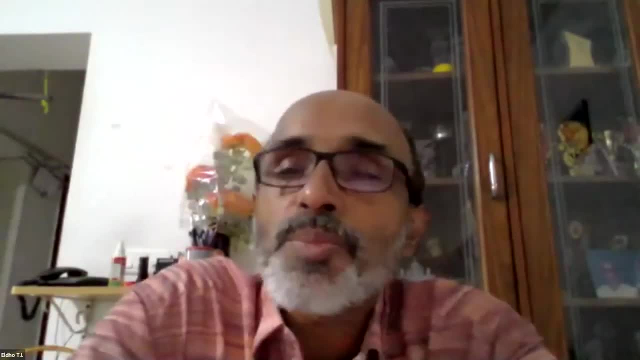 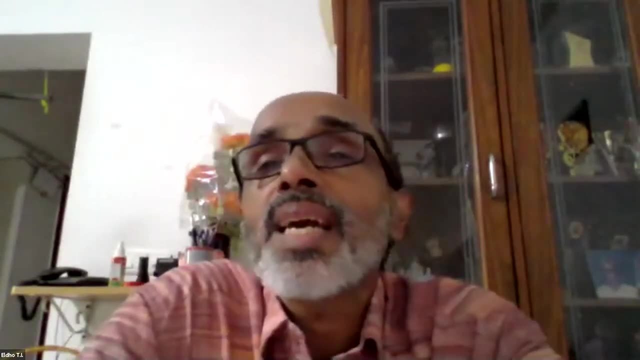 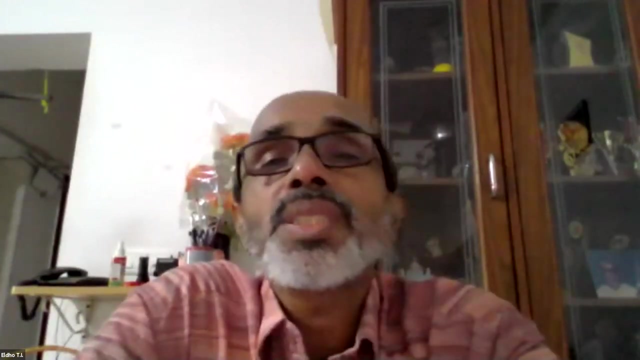 nowadays some satellites are coming for soil moisture. even specific satellites are available and some of my colleagues' studies show that this the satellite data. to a certain extent they are reliable And then through data simulation techniques we can directly utilize this data for especially soil moisture and other kinds of data. we can directly secondary data. we 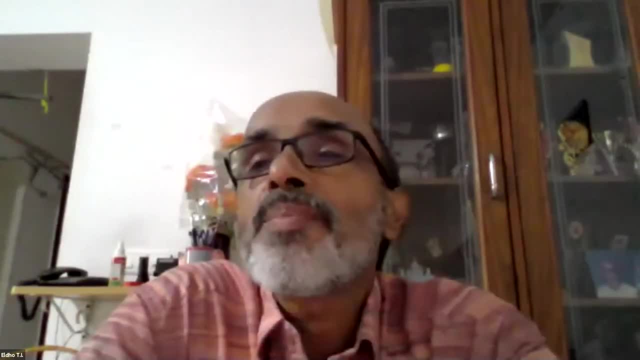 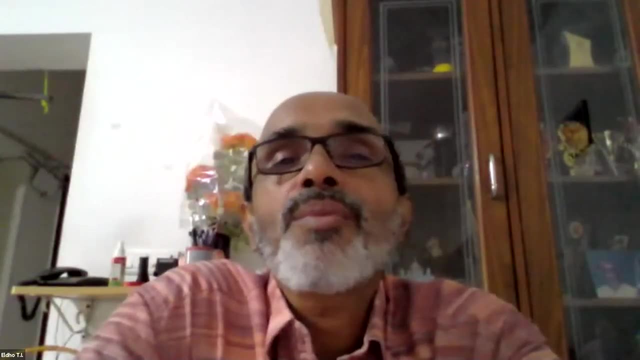 can utilize for hydrology models. So that is already that branch is going in, that studies are going in a very hectic way throughout the world And I'm sure that within a few years, of course, most of the satellite data will be very, very, very, very, very very. 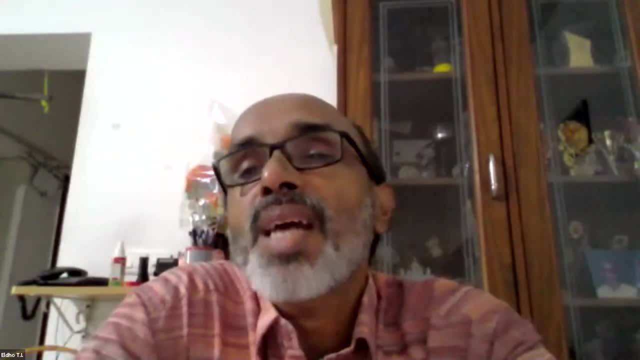 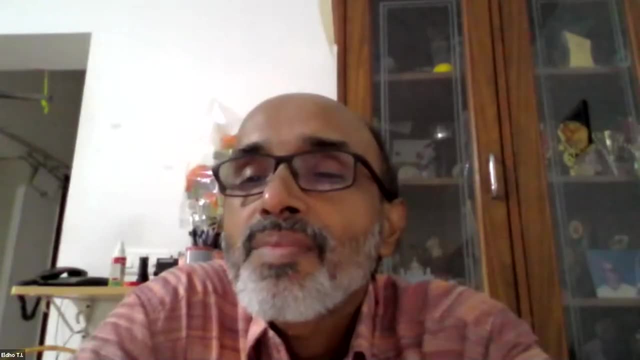 useful, So that is a very effective way we can utilize for a hydrology model. Thank you, sir. I will simply just take two questions only. Next question from Rahul Orman: As the hydrological structures are designed for stationary hydrology but due to climate, 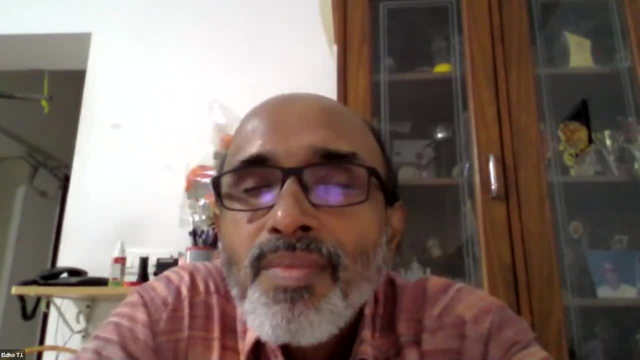 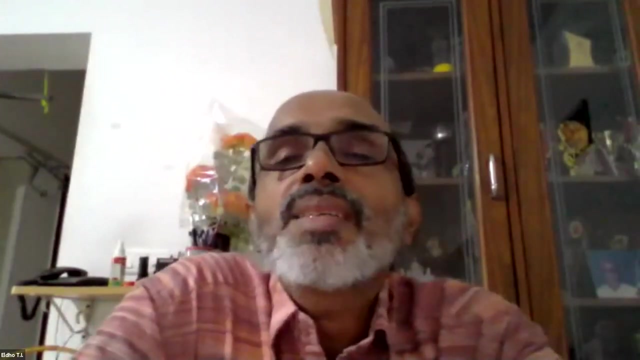 change, the parameters are affected. So is that necessary to revise the operations, as many places in the world that the hydrological structures are not able to fulfill their purpose to its fullest? Yeah, so that is obvious. So I think you see that this is a major challenge with respect to the climate change impacts. what 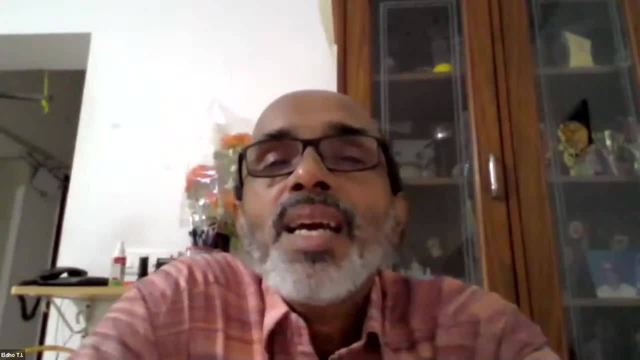 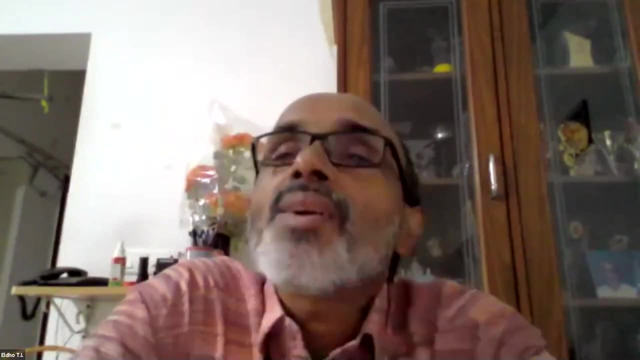 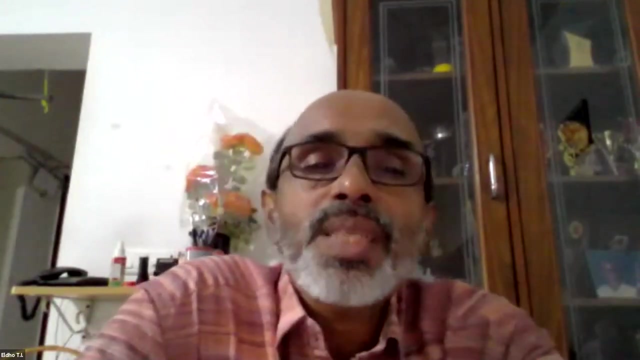 is observed. You can see that though we construct very, very large reservoirs, very large dams like Sardar, Sarovar or even Jaikavadi, all those things are available. But now the problem is that if these kinds of changes taking place, then we cannot store. say what I understand. 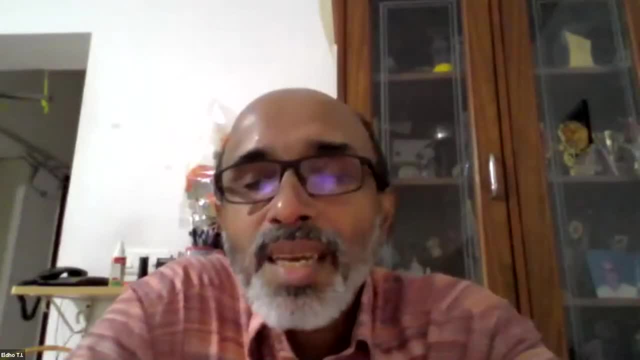 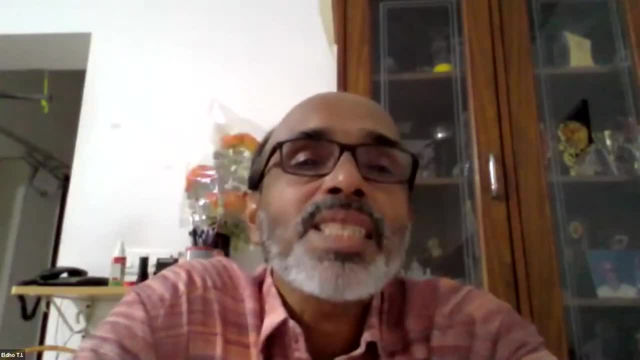 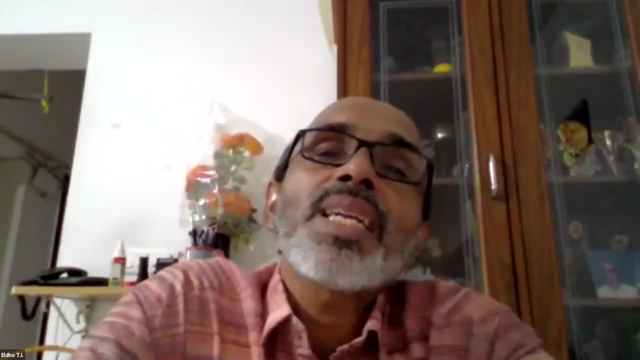 Yeah, There is a lot of work going on. I think there's some hard work happening, Like now, say, for example, Jaikavadi is concerned. I understand that last year they could fill that entire reservoir to certain extent, But so many years this may be happening after 30 years. 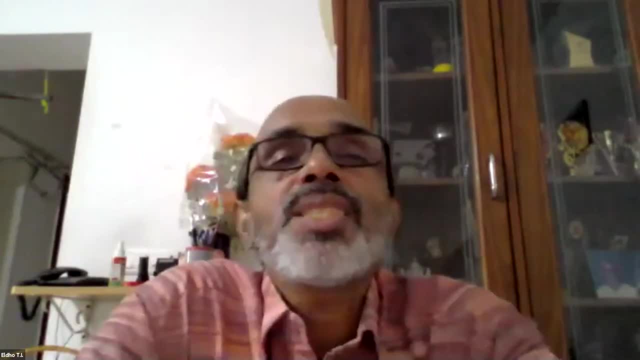 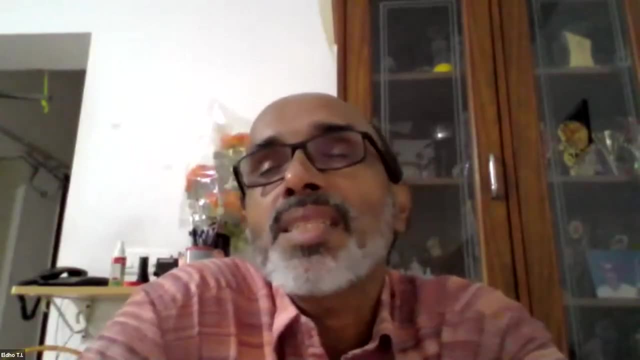 or 40 years. So that way sometimes it is happening, But now the climate change study shows that this is going to happen. I mean, these kinds of discrepancies, or many times these kinds of uncertainty is happening. So that way we cannot overlay upon that. So that way. 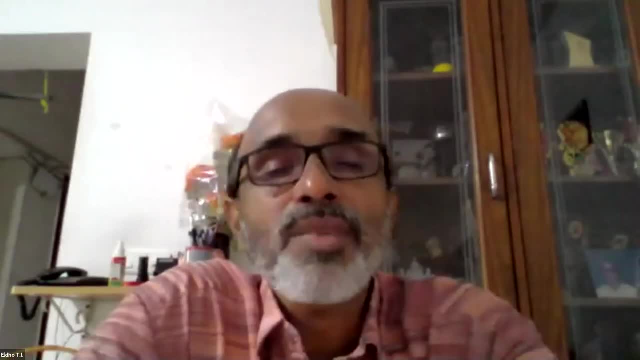 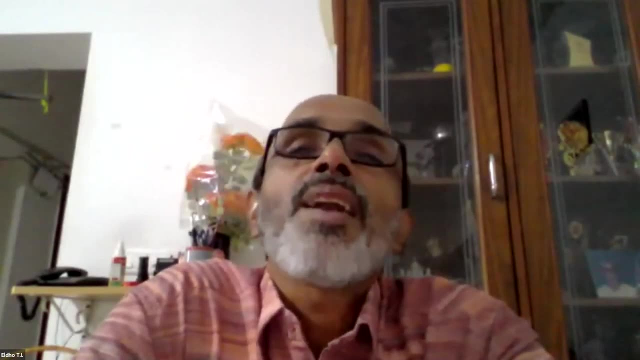 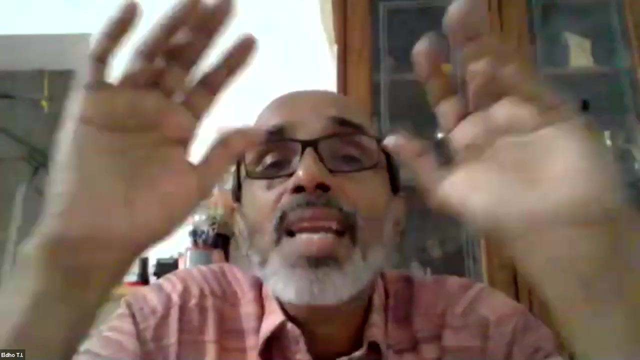 another solution is that locker scheme Like this is an early scale. This is what our government is also promoting. We need to go for rainwater harvesting, local, village level or small watershed scale. development needs to be taking place So that way. we need to wherever water is available, wherever the rainfall is happening, So that area at least. 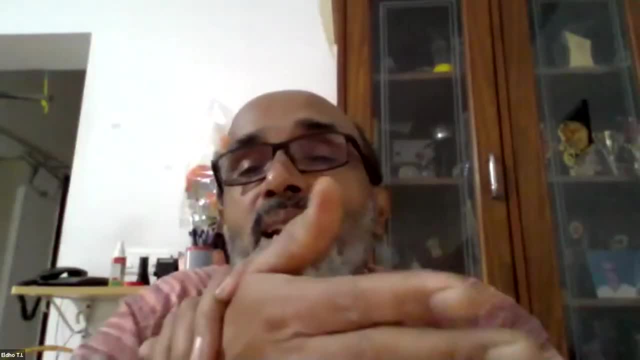 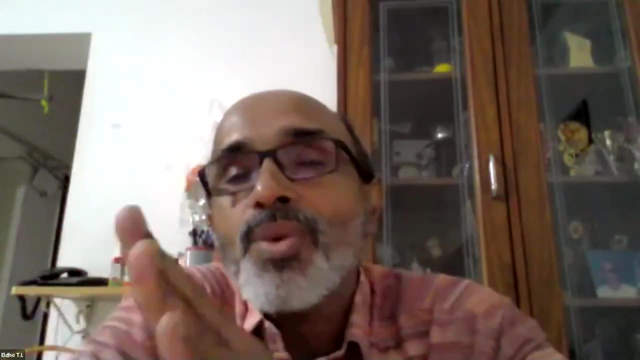 we make a self-sufficient, like many typical cases are there in Maharashtra, like Raleigh and Sydney, or many, many areas are there. So there we have to go for local solution. Of course, local solution will not be sufficient for a long-term solution, So we need to have a mix of like rainwater. 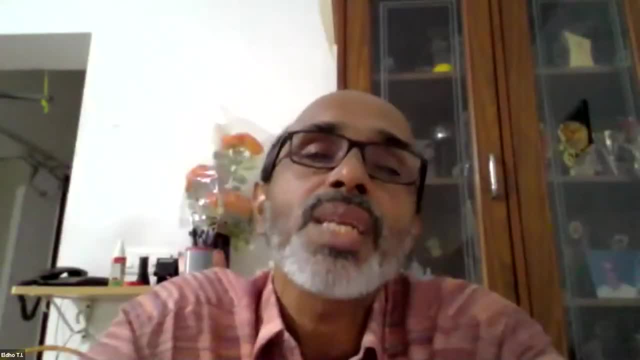 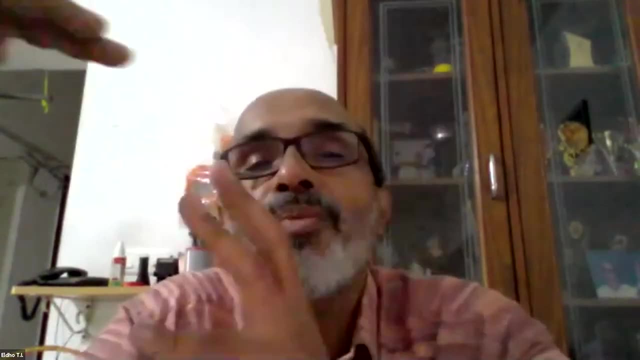 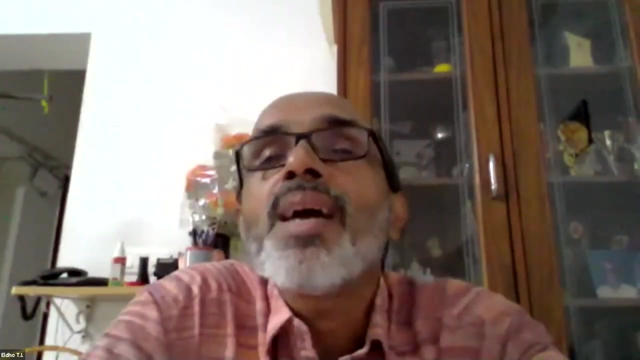 harvesting, watershed management, all those things, and simultaneously we also need a storage, like major storage structures are also needed, So that combining of both these solutions in as part of water management or water source management is concerned. So that way there is a lot of uncertainties are there, since hydrology is uncertainty, Hydrology itself. 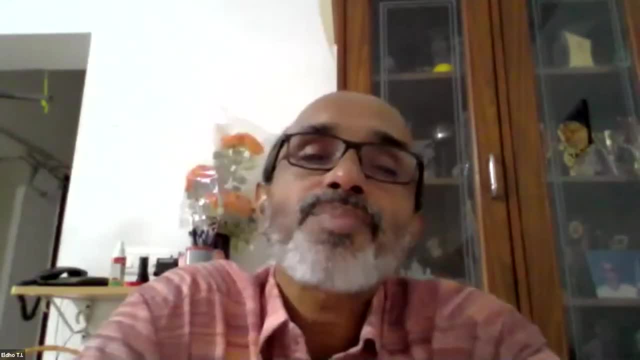 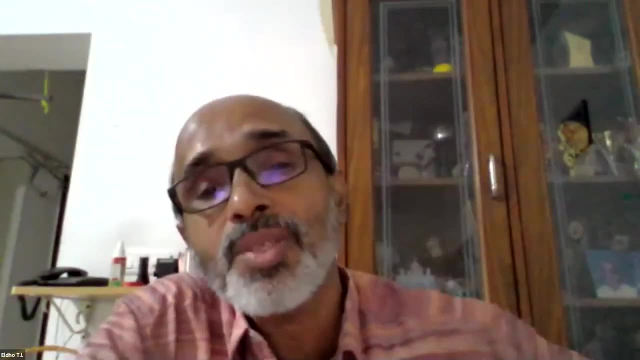 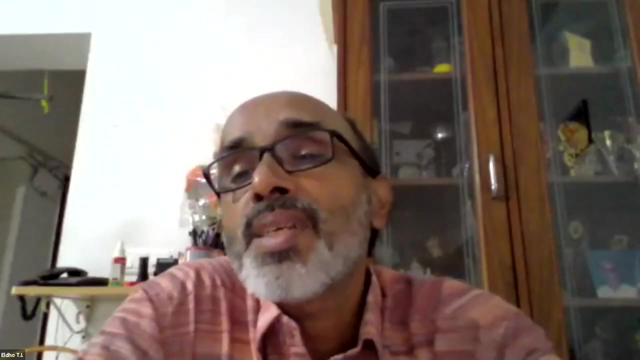 I call it as uncertainty. So that way we need to look into this and then local solutions to global solutions. So we cannot say from global to local is not possible. We need to first see the local solution and then global solution. So that way both of us come together to deal with the water source problems and then 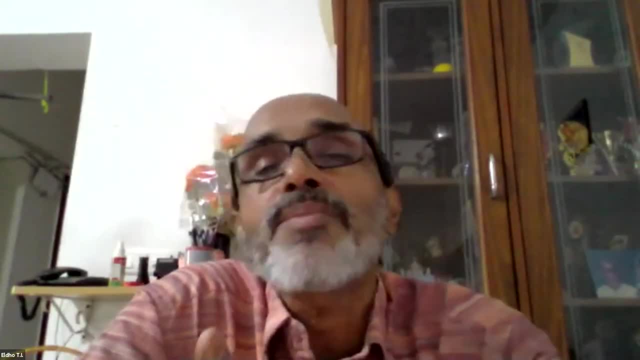 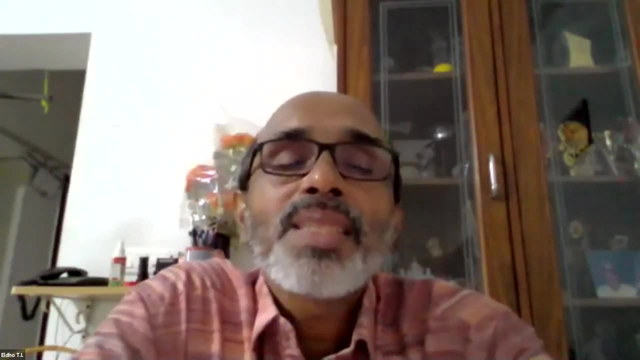 many of the dams or reservoirs may become empty, even after a few years. We do not know. So that is some of the projections are showing, But then that's what I told. an example. Take a example: Whenever heavy rainfall takes place in 2018, Kerala flooding is concerned. First, the Dikhi reservoir, which has filled in last 30 years only once. So that means 1990 and now 2018.. So 2018. by August itself it was full, and then we have to release the water. Then by September or October. 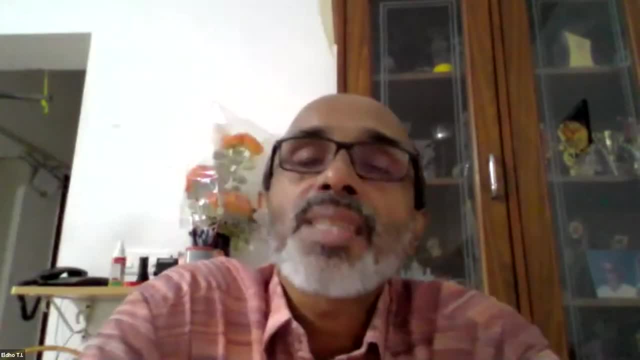 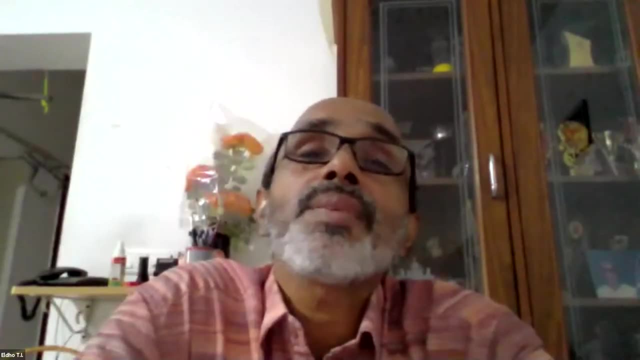 there was no water at all. So I mean even the Dikhi reservoir, which is used for power generation. so there it was affected. So that is the problem. So whenever heavy rainfall due to climate change takes place in few events, and then flooding takes place and then we are forced to release the water, 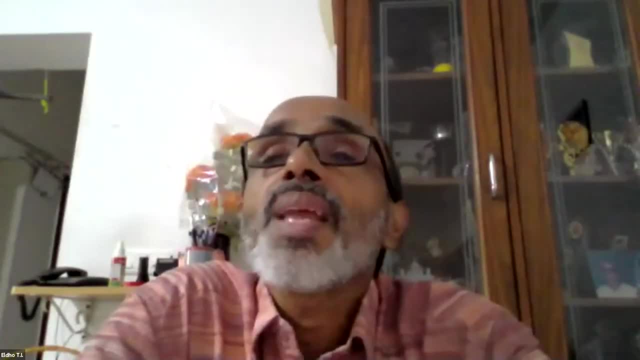 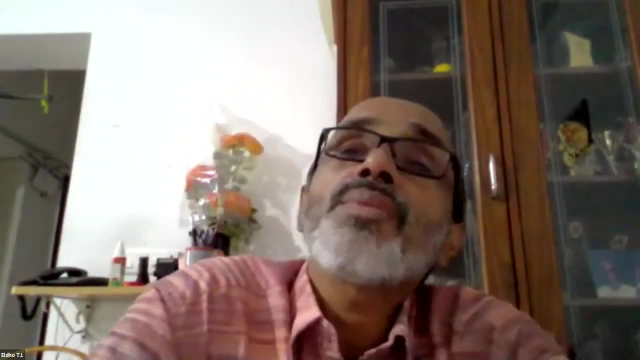 Then later we will not be able to store or we cannot utilize. So that way, local solutions are also very essential and I am sure that the Arashakti ministry is nowadays taking so much of money they are putting for rainwater harvest structures and rainwater harvesting or water. 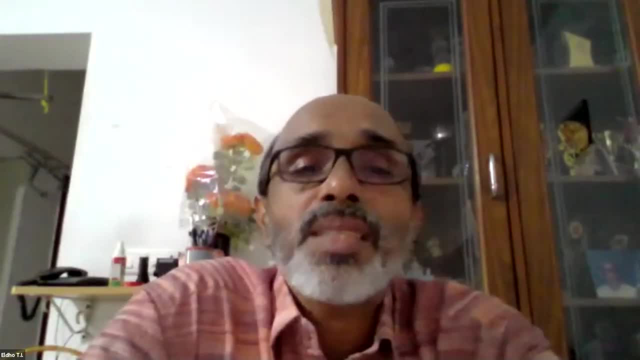 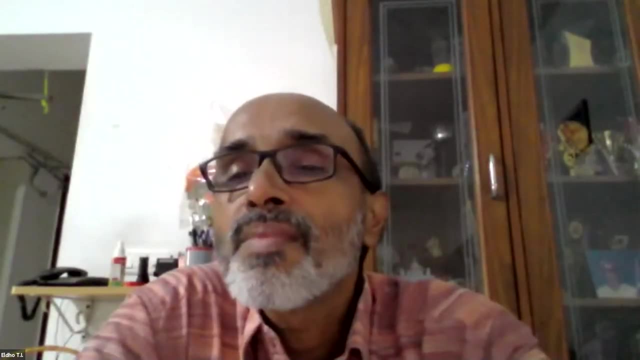 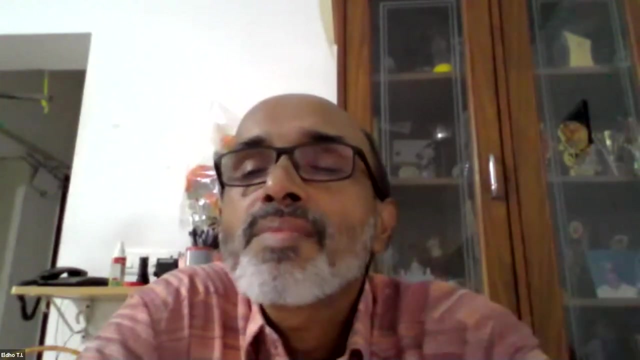 management aspects are also concerned. So that way, a mixed approach, is the best way, as a hydrologist, we can propose. Yeah, Thank you, sir, Because of time. thank you, I am just taking last question from Bhavin Rang. Actually, he is extending his thanks to you, sir, for giving a nice answer. The question is: 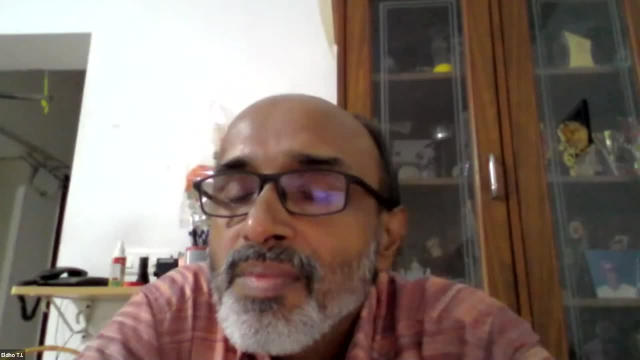 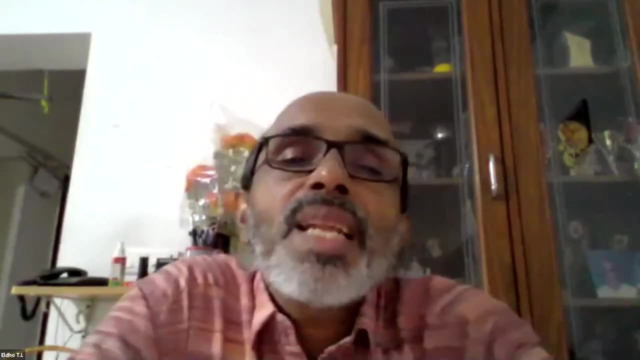 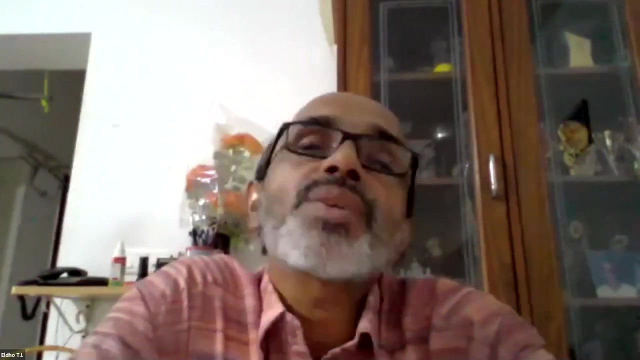 can we use satellite field precipitation product as input for hydrological modeling when we don't have all the data at final table level for particular species? So sediment deal is also concerned. Luckily the sediment is. you see that Roshnan sedimentation is very challenging, probably even compared to hydrology. This is very, very, I mean depending. 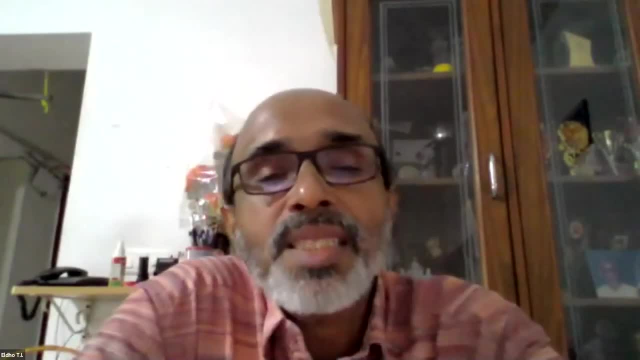 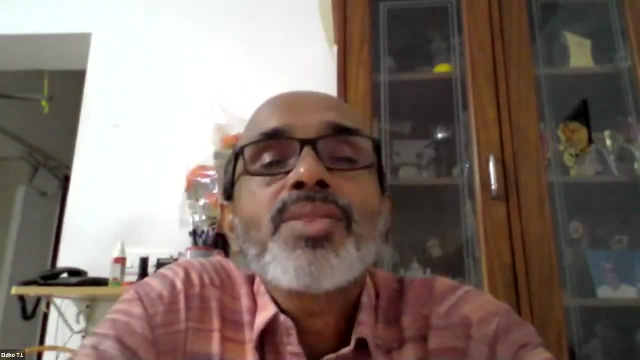 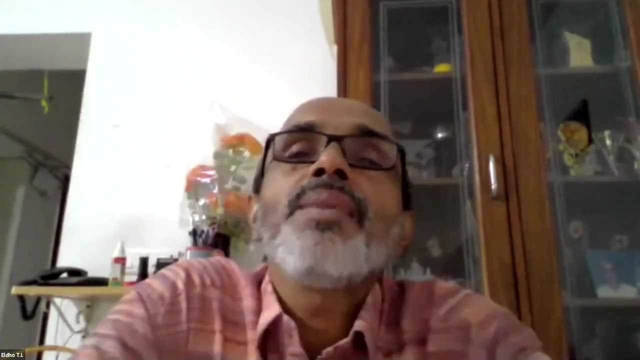 upon so many parameters and geomorphological parameters are concerned. So luckily some measured data is available, So its correctness of course we need to validate. So we have also done sedimentation studies are concerned, and then you see many of the CWC stations, what is available? 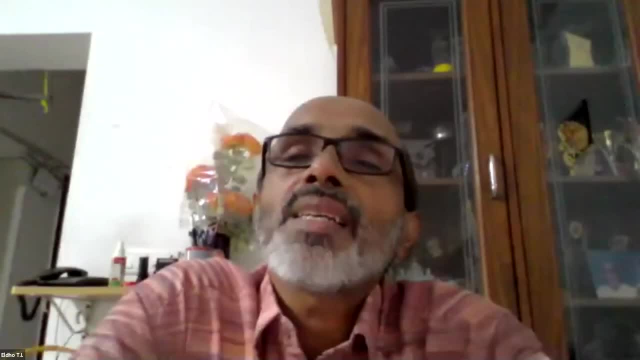 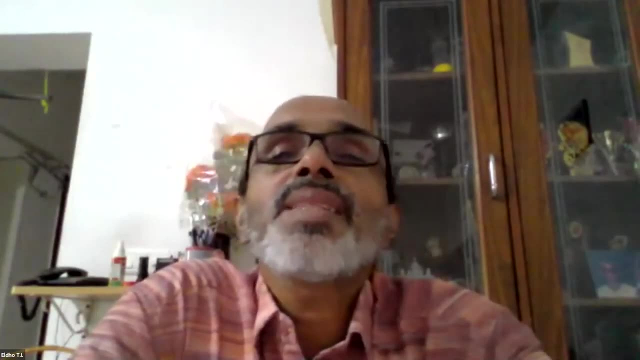 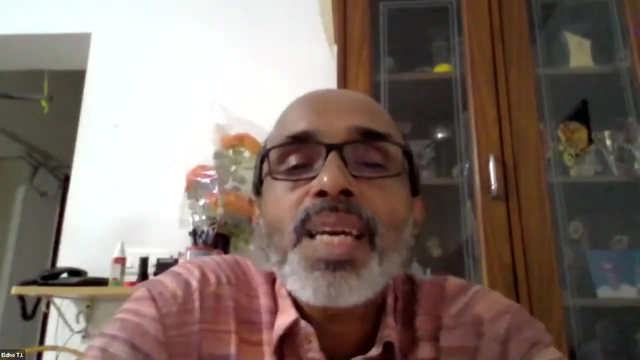 there also. they measure the sedimentation and then its parameters are put. But that way it is not complete. many discrepancies are there in the data. But the thing is that it is so quality I mean we cannot get quality data. it is so difficult even for we cannot blame that those 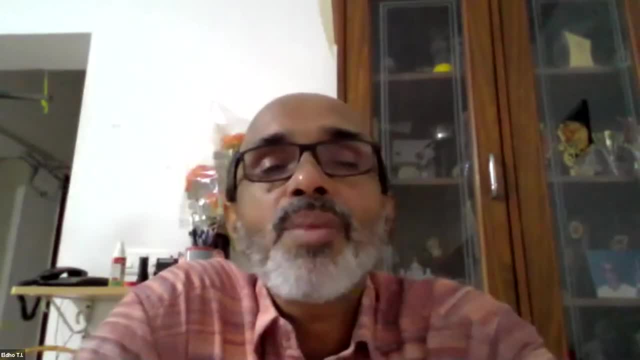 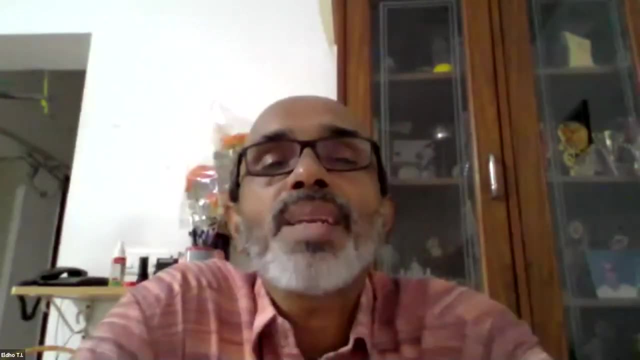 are collecting the data. But since it is a very localized phenomena and then it is, getting that kind of data is very, very difficult. But with respect to the physical models, like here the the sediment transport equations are concerned. So this, some of these data found to be useful and 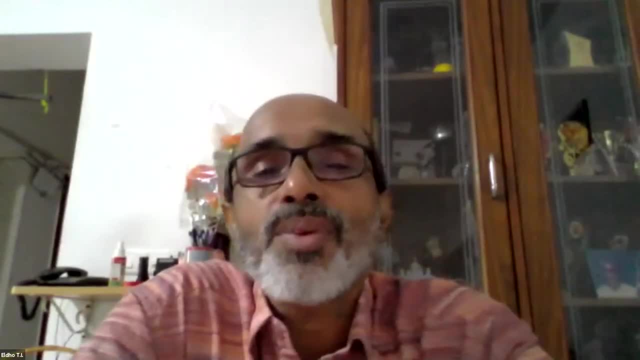 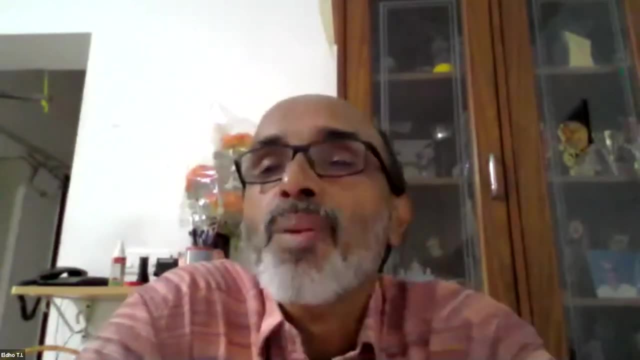 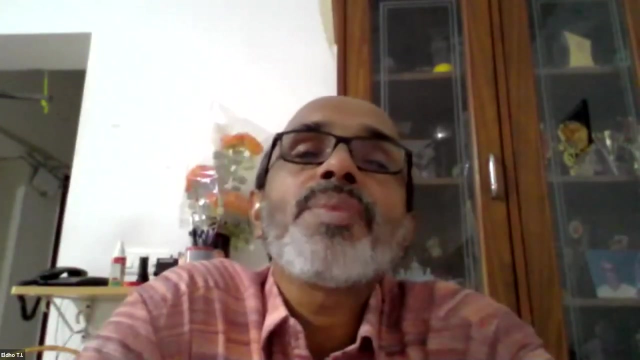 then of course, to certain prediction levels we can say that and then of course we can say a proposed like, like rainwater harvesting or watershed management structures we can propose. But the sedimentation or sediment studies is a very challenging area. There are lot of data is required and data availability is very scarce. 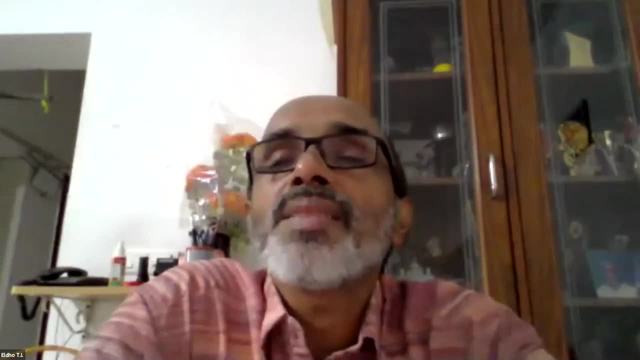 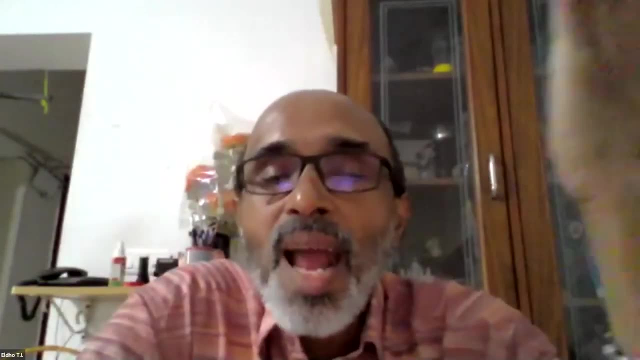 That way I fully agree. But currently some of the the gauge stations by CWC, they also measure the sedimentation that is happening. But if you get one like 5,000 or 10,000 square meter one location, if you get that, is very much inadequate. but our 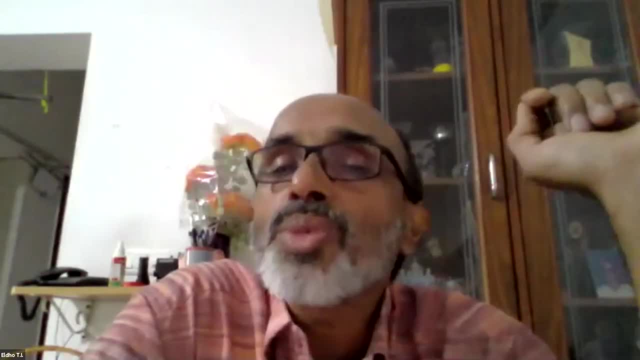 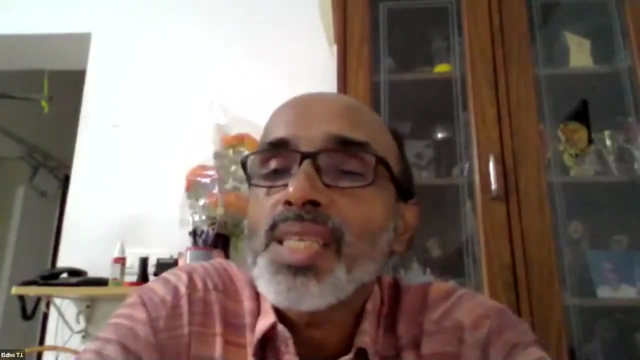 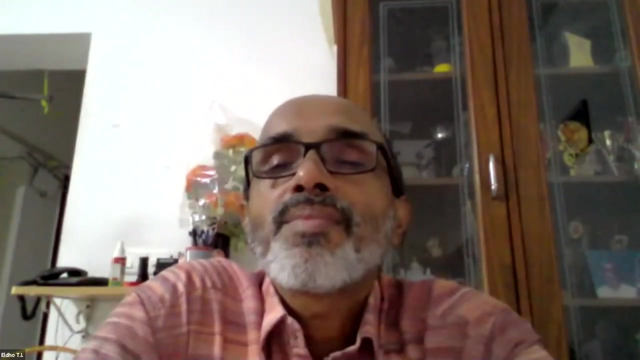 models. if you use it to calibrate it and then you use for a sedimentation map or erosion map you can prepare and that will be used for these kinds of studies. Thank you, sir. hope the participants got their answers fulfilled. because of time we have to wind up this session and other question. 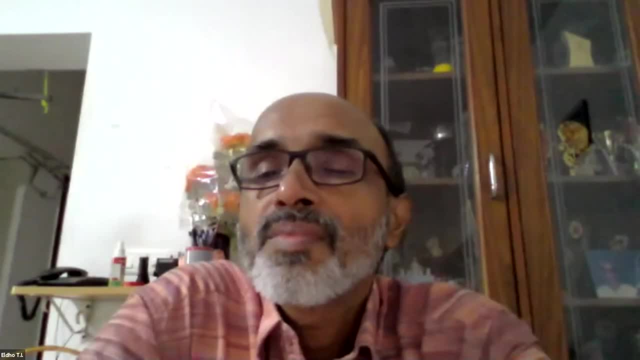 basics. we will take and answer and we will try to answer them in person. Thank you, sir, once again. now I request Dr Atul Alkareesat, Professor Kuala Lumpur Engineering and Bocan Enology State Programme, to present the book of thanks, Sir, please. 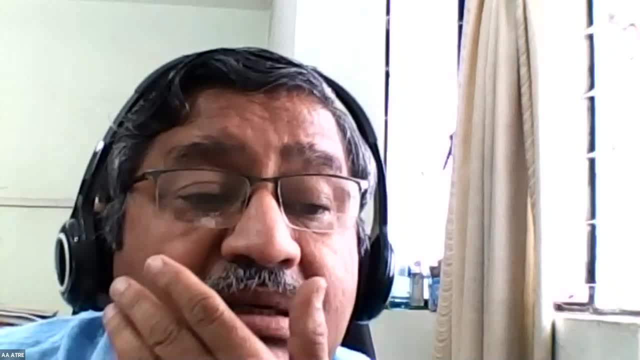 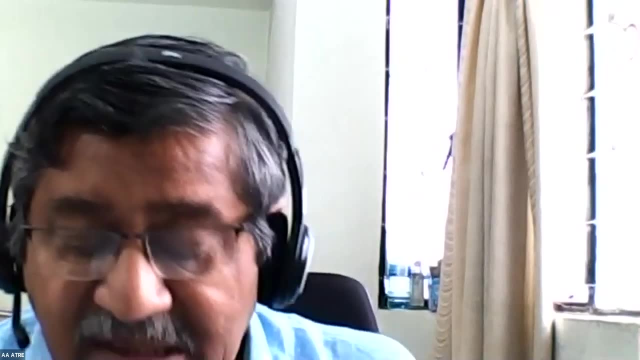 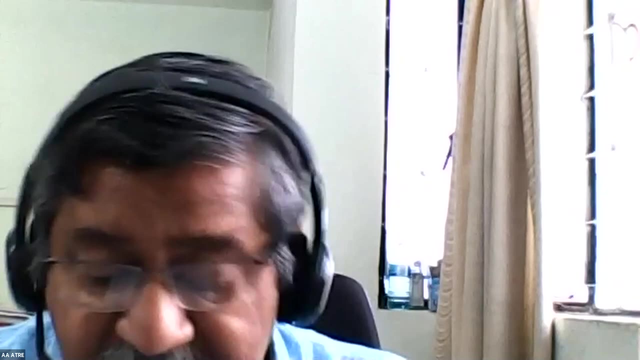 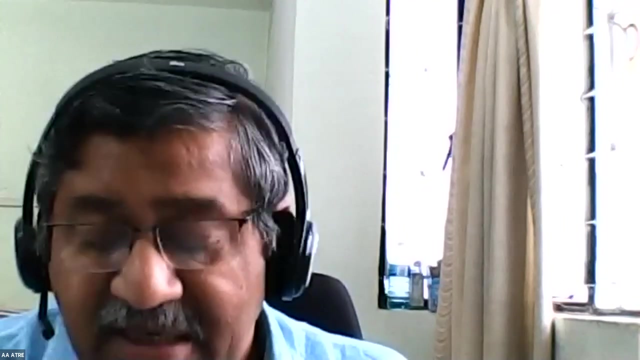 Hello, am I audible? Yes, sir, Okay, thank you, Professor Indu. He has touched on important topics like hydrology, political modeling, then climate change and some case studies showing the effect of climate change on water resources of India. within the constraint of time, Really difficult task. and then he has also given insight of various 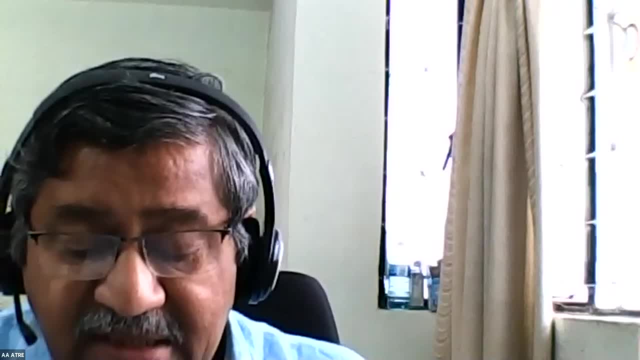 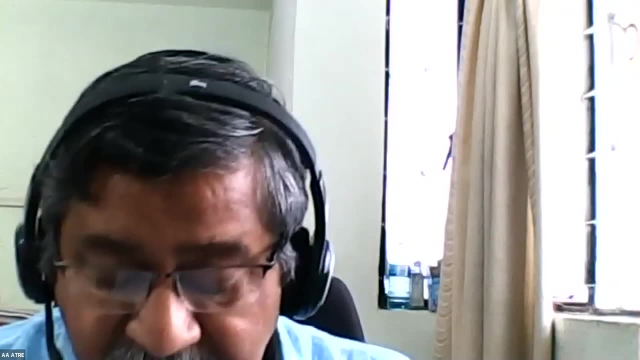 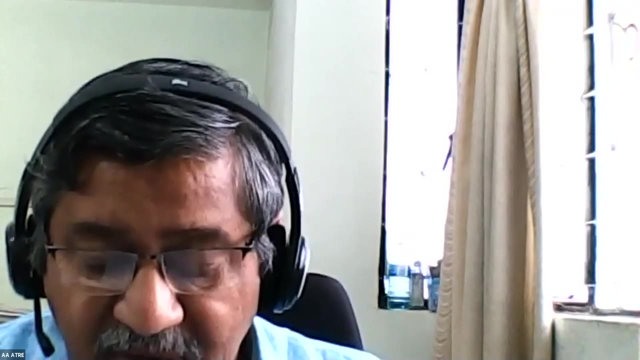 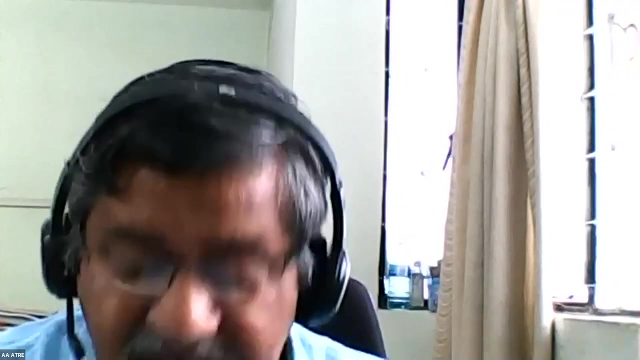 models through questions and answers. I am really thankful to Professor Indu for accepting our invitation and for his nice presentation. I am also thankful to our Honorable Vice Chancellor, as well as Director of Instructions, who have continuously encouraged us to organize such programs for especially young scientists, and I am also thankful to all the 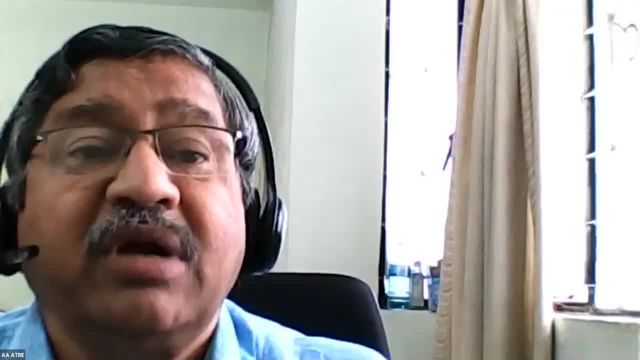 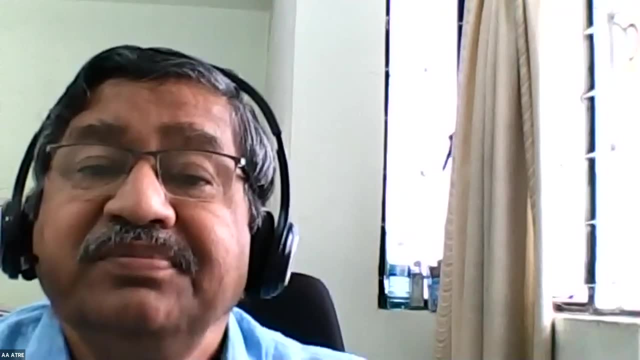 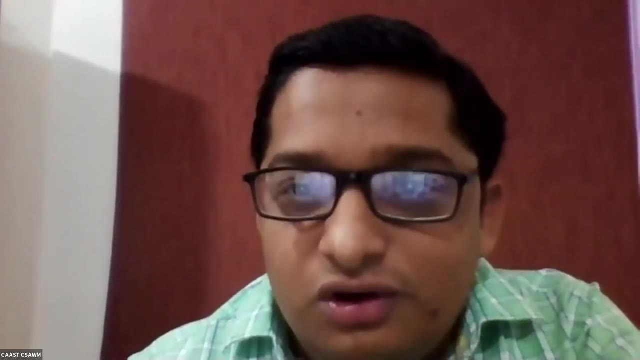 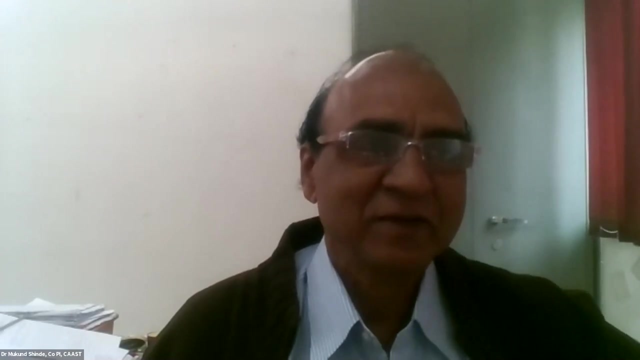 participants who have shown their interest in this particular training program. Thank you one and all. Thank you very much. Now over to Kalpesh. Thank you, sir. This was a Ahh. IT lives now HuNiya. Dr Srinde, could I have a dialogue with Dr Eldo? 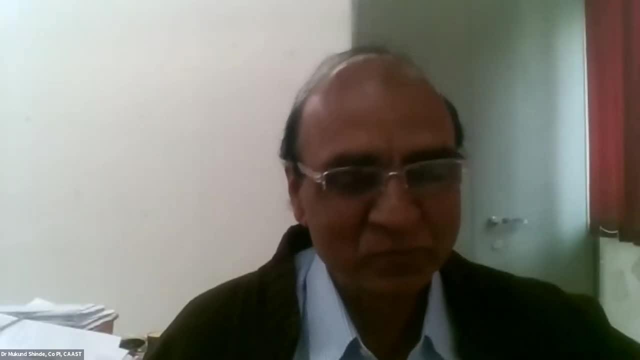 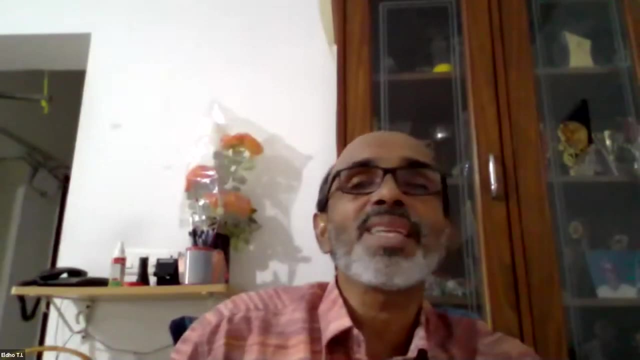 No, it's okay. again from organizing committee. Thank you, Professor Eldo. thank you for spending your valuable time and hope we will have continuous interaction in future. Yes, yes, Okay, thank you very much. Thank you, Professor Kakkoh pozos, Professor Gorandewar and all the team members. Thank you very.